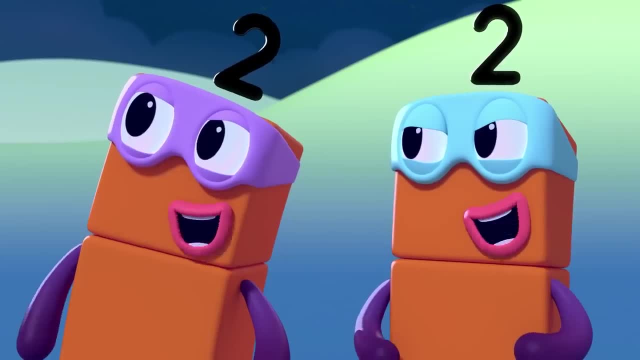 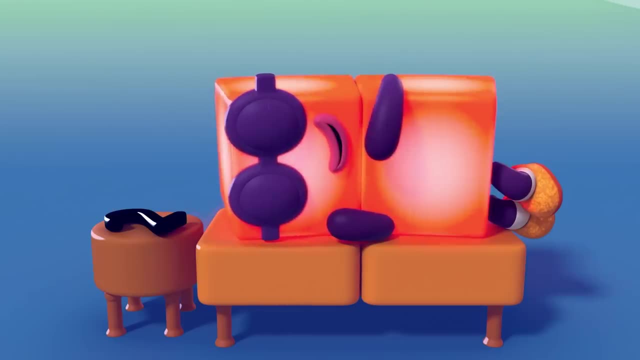 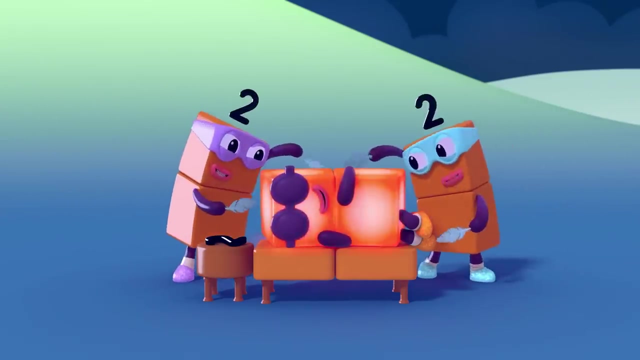 Oh, Oh, That was fun. Let's do it again. Yeah, Oh, Oh, Hee-hee. He reminds me of someone- Amigo Can't think who, Amigo, Tickle, tickle, Tickle tickle. 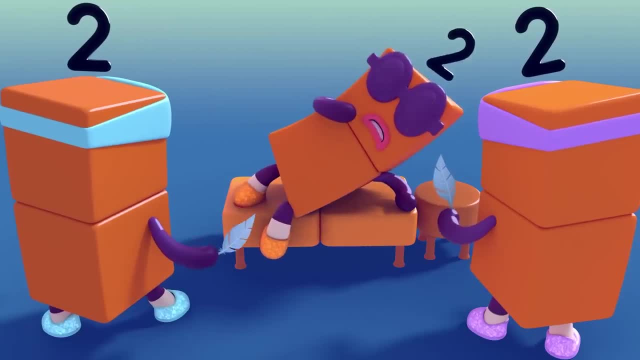 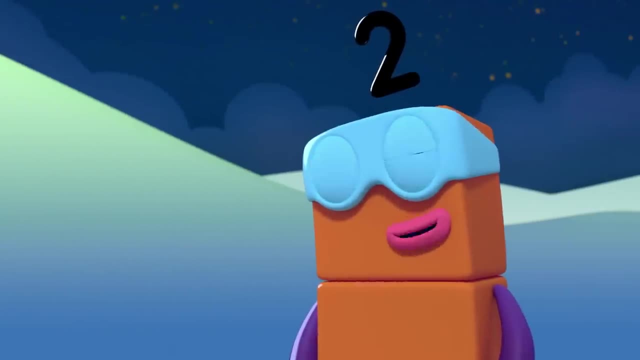 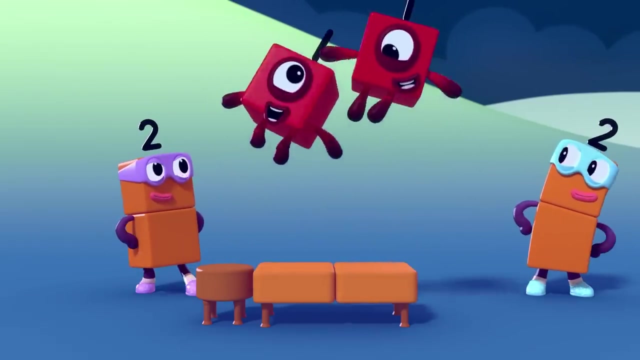 Oh, Another me, Doubler, Another, another me, Him me and you are too many twos. So it's time for the both of us to say Boo, Oh, Oh, Oh Oh. Two twos, two ones. It's time to be gone. 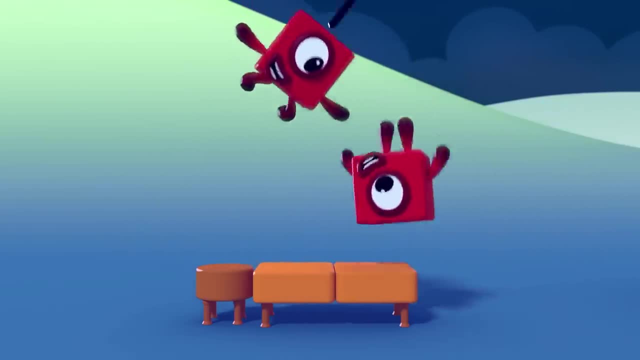 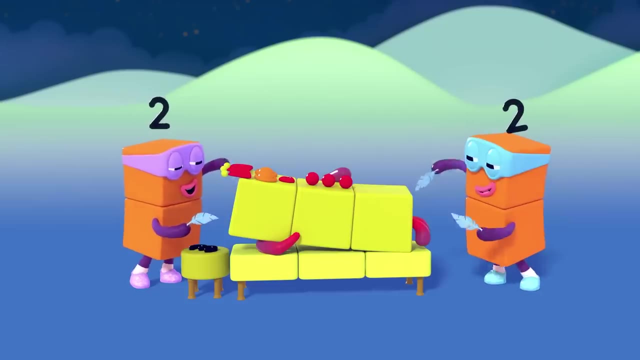 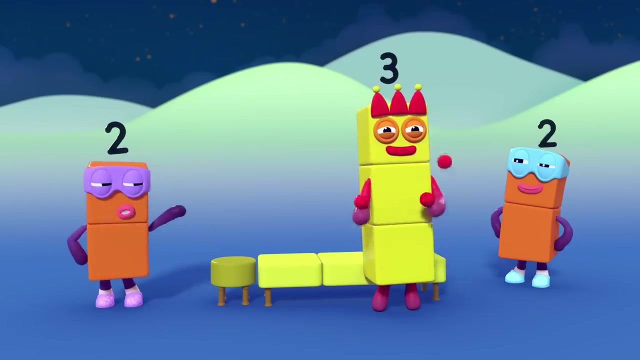 Yeah, Oh, Oh, Oh, Oh, Oh, Oh Oh. One, two, Three Bum, bum, bum. Looks like fun, Let's try it too, Just as soon as we both say: Boo, Oh. 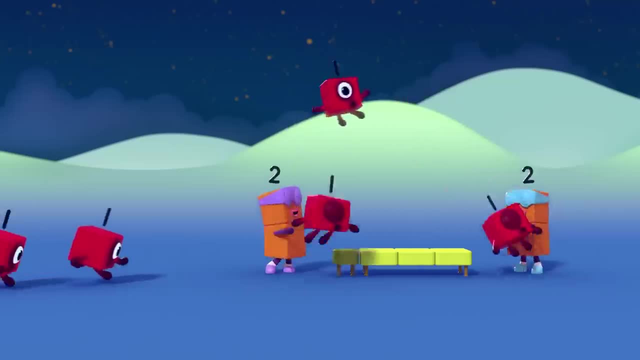 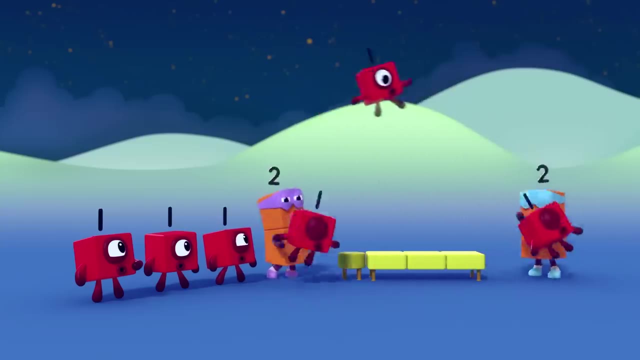 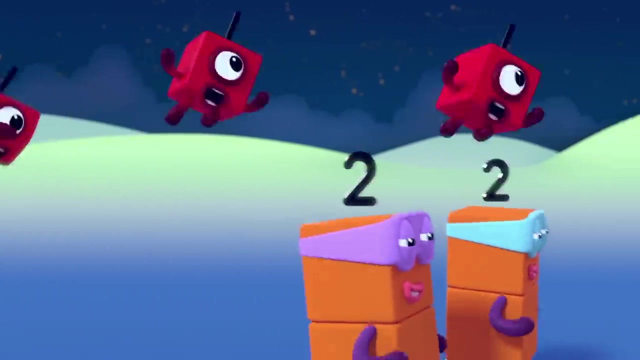 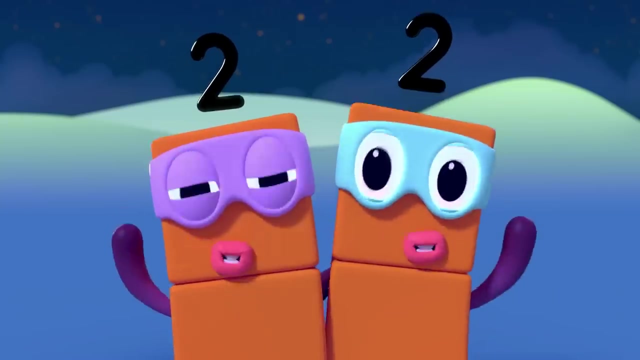 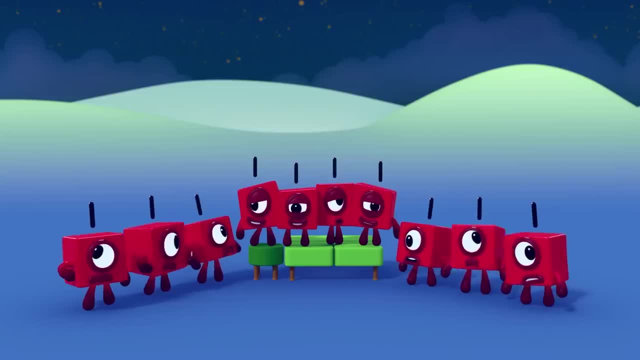 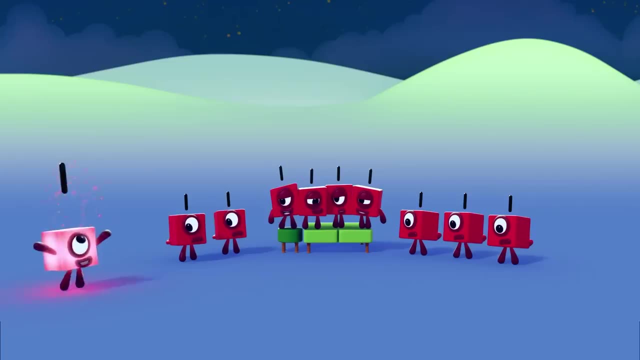 Oh, Everyone, pull yourselves together. One One block. One plus one equals Two. Two is two ones. One plus one plus one equals three, Three. Three is three ones. One plus one plus one plus one equals Four. Four is four ones. 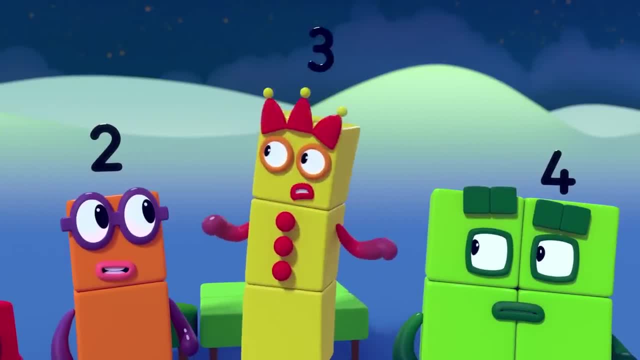 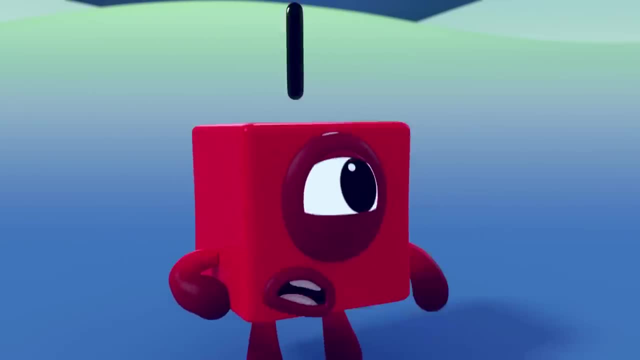 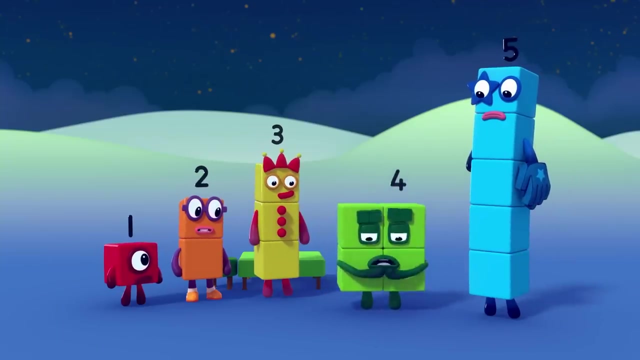 Where are they? Where did those terrible twos go? Don't look at me. What's all of the noise? The terrible twos are playing tricks on us, And where are they now? I have to be square with you. They made me. 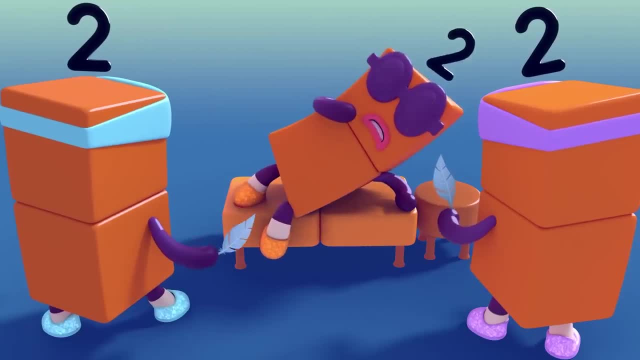 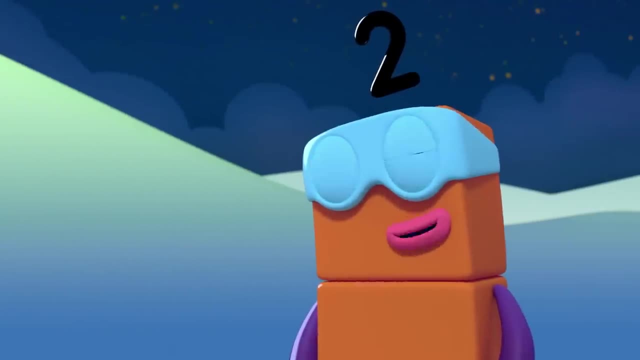 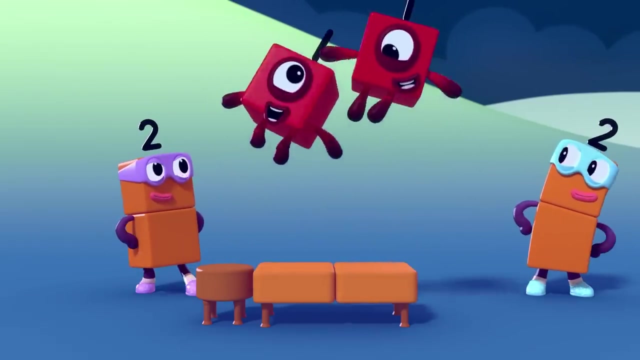 Oh, Another me, Doubler, Another, another me, Him me and you are too many twos. So it's time for the both of us to say Boo, Oh, Oh, Oh Oh. Two twos, two ones. It's time to be gone. 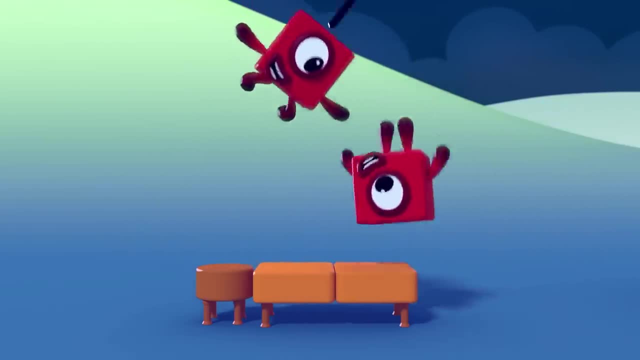 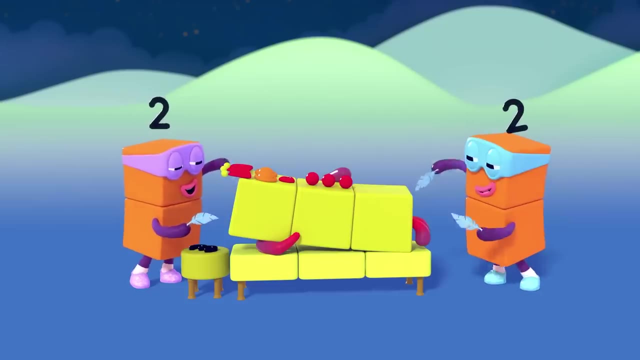 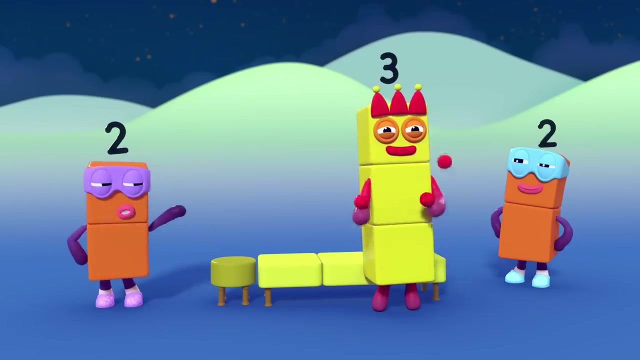 Yeah, Oh, Oh, Oh, Oh, Oh, Oh Oh. One, two, Three Bum, bum, bum. Looks like fun, Let's try it too, Just as soon as we both say: Boo, Oh. 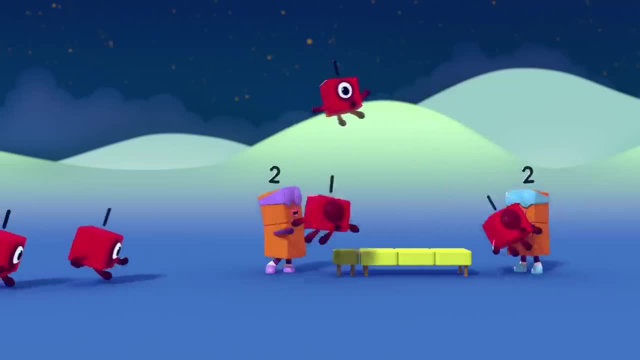 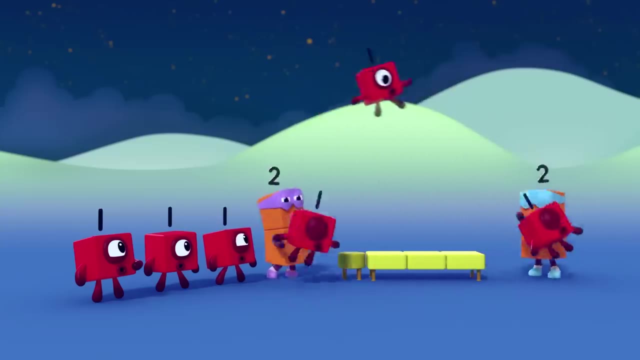 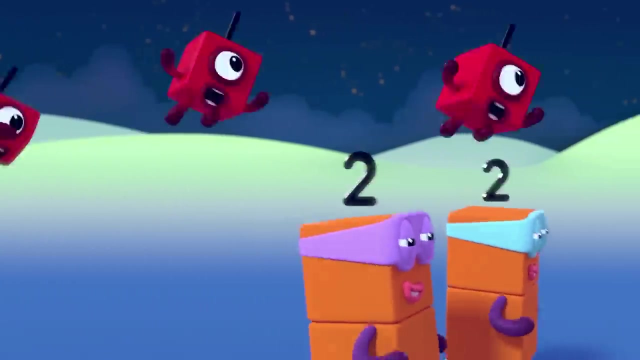 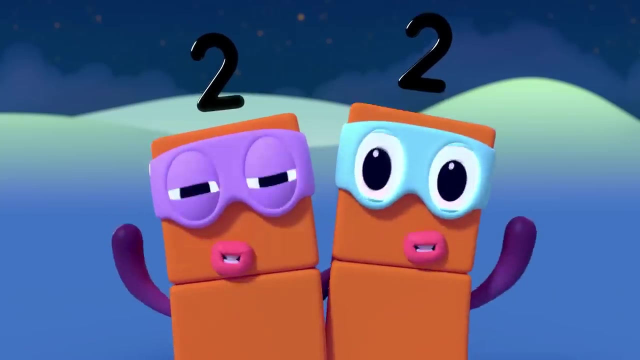 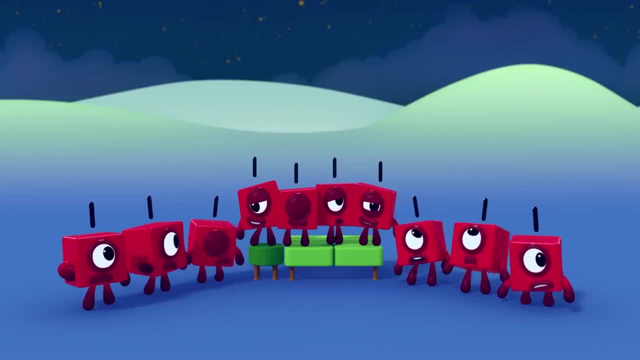 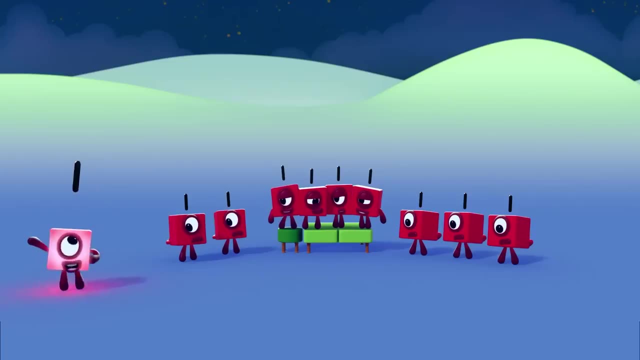 Boo, Boo. Oh, Everyone, pull yourselves together. One one block. One plus one equals two Too two is two ones. One plus one plus one equals three: 3. is three ones: One plus one plus one plus one equals. 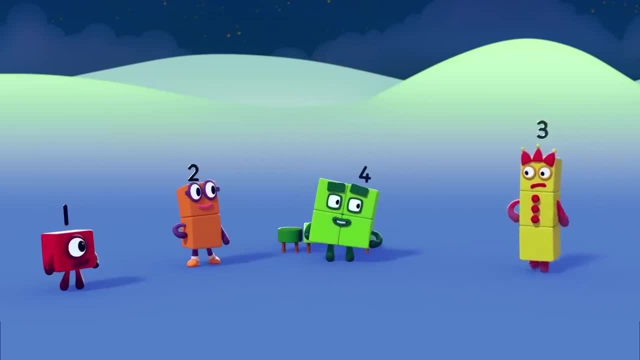 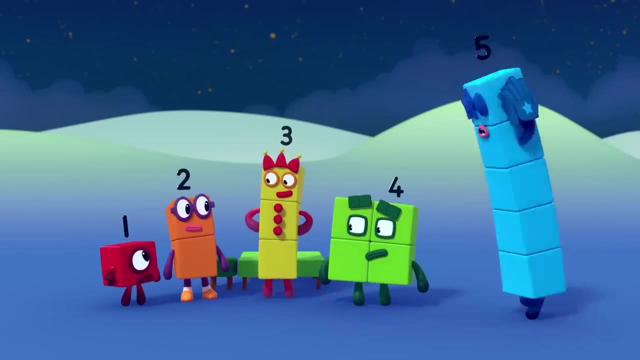 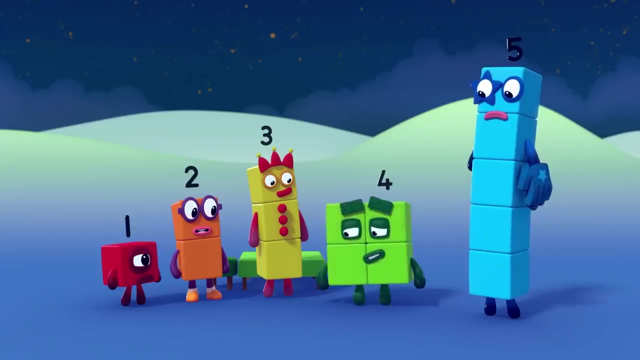 four. Four is four ones. Where are they? Where did those terrible twos go? Don't look at me. What's all of the noise? The terrible twos are playing tricks on us, And where are they now? I have to be. 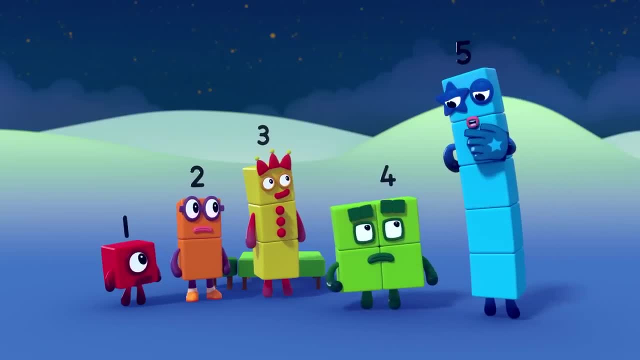 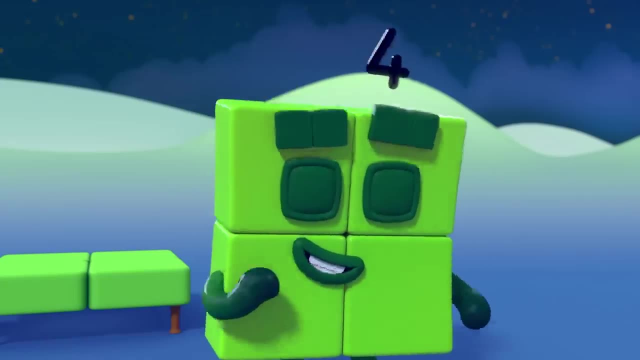 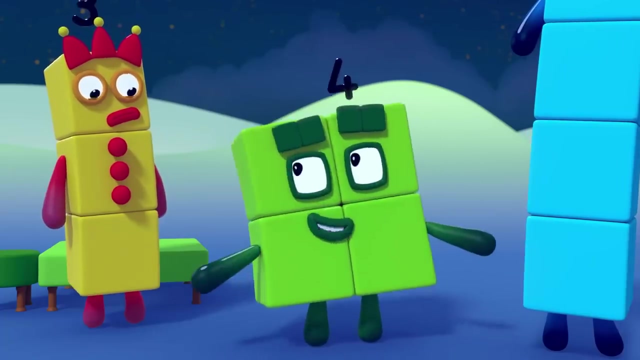 square with you. They made me. What did they make you? You can tell us Four. No, they made me. Well, I made them. Then they made me: Huh, I'm the terrible twos, I'm four. 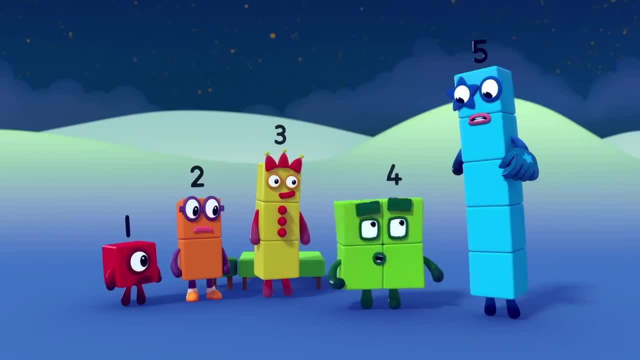 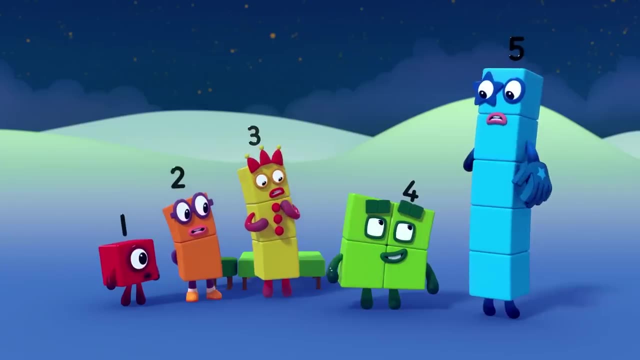 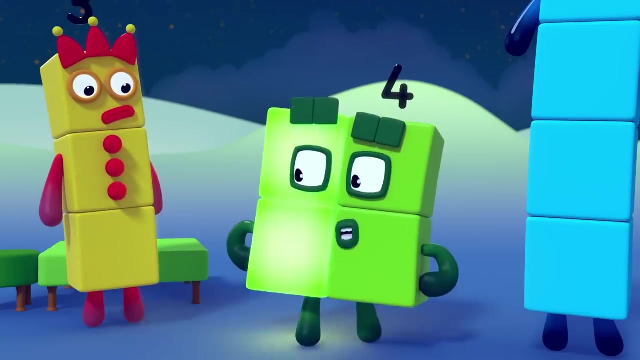 What did they make you? You can tell us Four. No, They made me. Well, I made them. Then they made me. Huh, I'm the terrible twos. I'm four lots of one, but I'm also two lots of two. 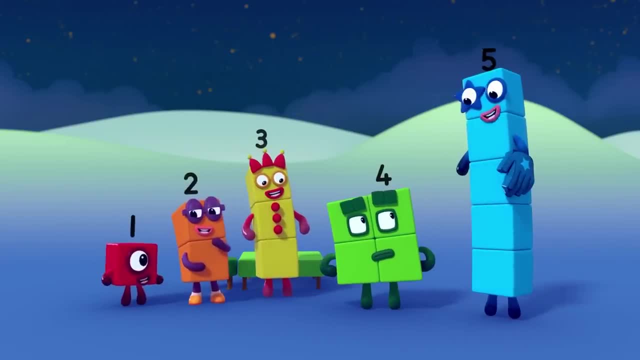 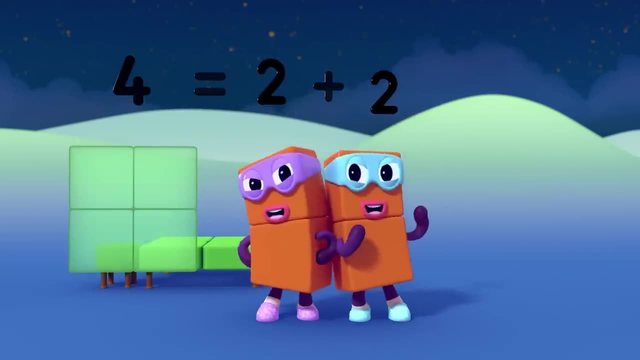 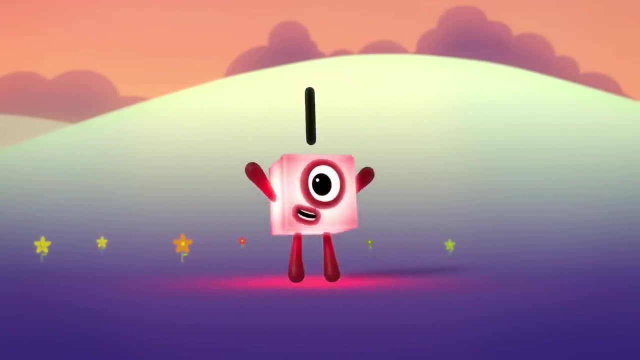 You're funny. Don't be silly, That's a very funny joke. Four equals two plus twos- The terrible twos. I'm number one, And this is fun. I've got one block to play with and the whole of me is one. 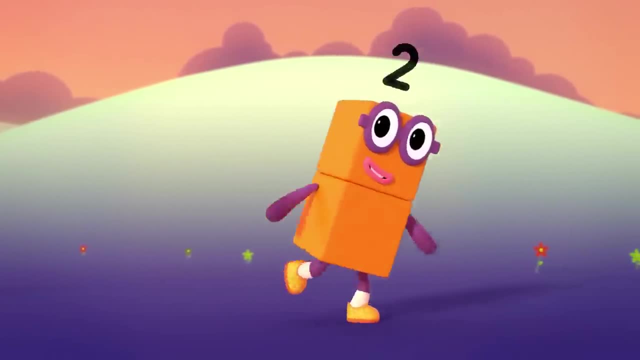 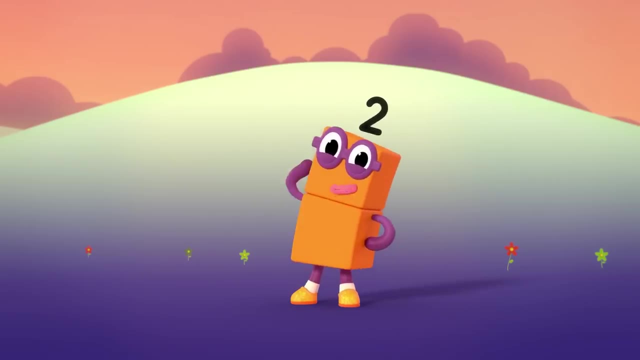 One, One, two, one, two. I'm number two. How do you do? I've got two, I've got three blocks to play with and the whole of me is two, One, two, One is a part of me and one is a part of me and the whole of me is two. 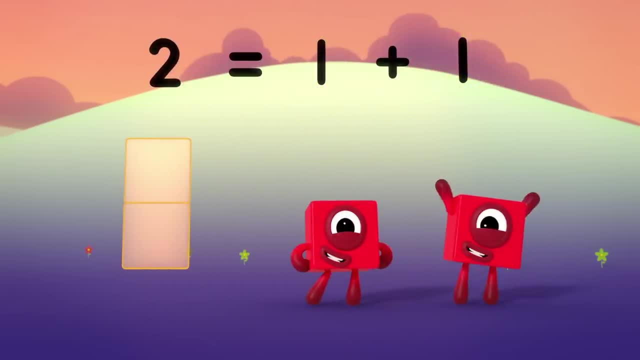 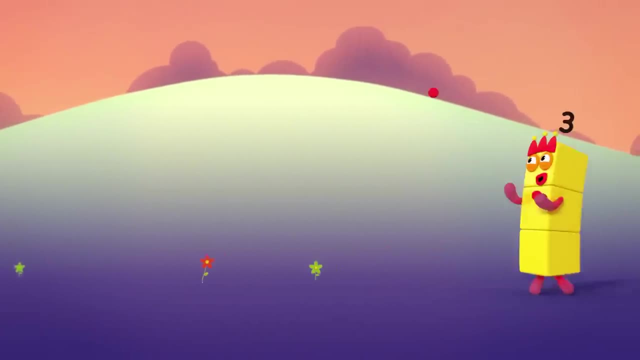 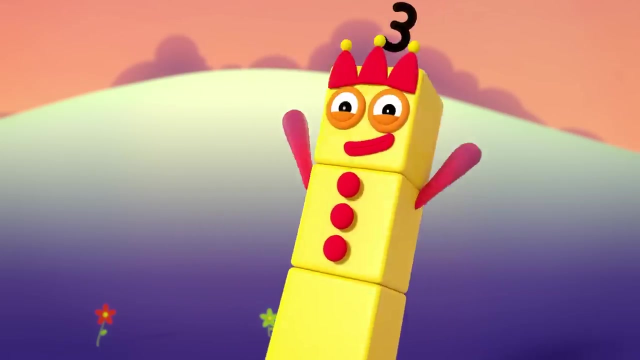 Watch. I'm one and I'm a part, I'm one and I'm a part, And the whole of me is two, One, two, three, One, two, three, One, two, three. I'm number three. 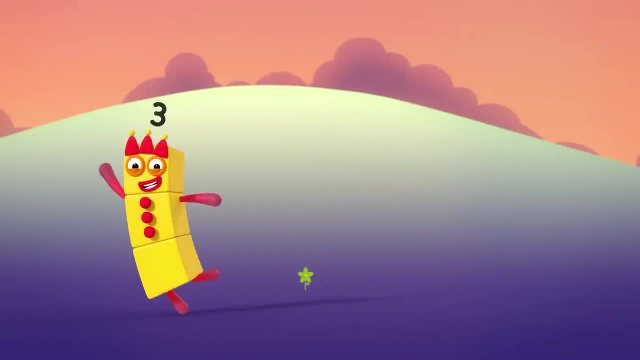 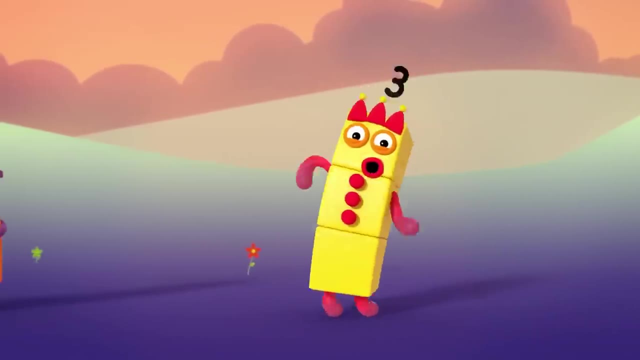 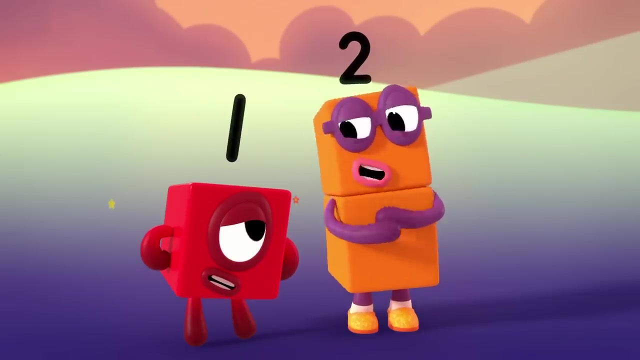 I'm number three. Now look at me. I'm the best of all the number blocks, as you can plainly see. The whole of me is amazing. The whole of me is so great. The whole of me is Sorry. Three, Try again. 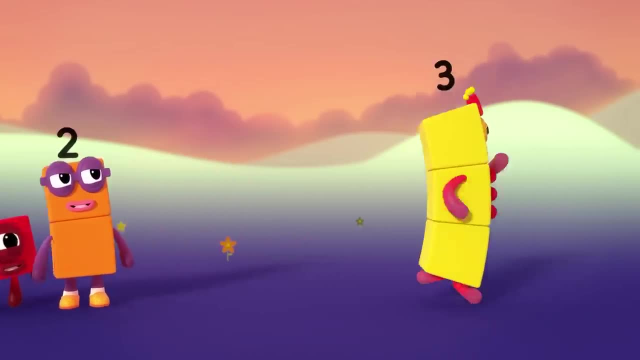 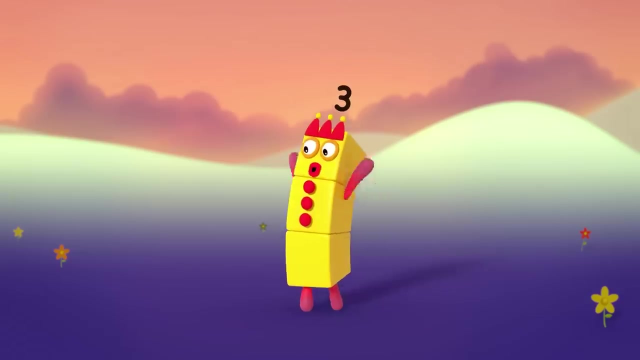 Okay, I'm number three. Yes, look at me. I'm the best of all, the number. Oh, you can't do it like that. You can't do it like that. I am, I'm number three. Now, look at me. 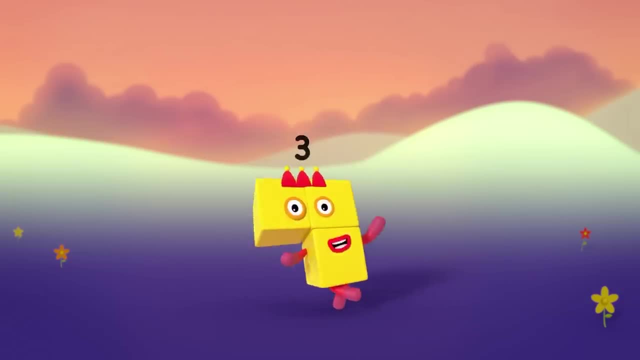 I've got three blocks to play with and the whole of me is three: One, two, three. One is a part of me and two is a part of me, and the whole of me is three. Watch, I'm two and I'm a part. 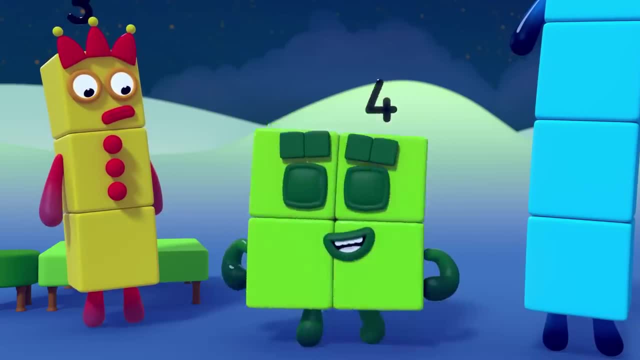 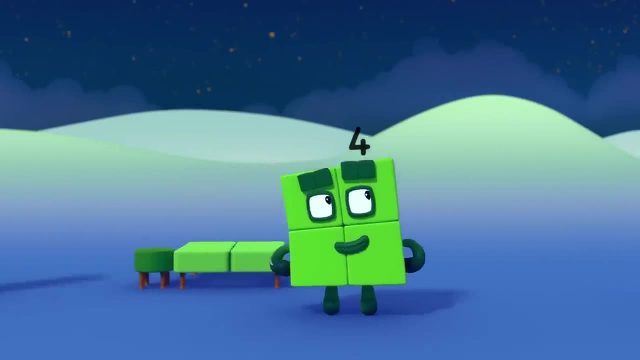 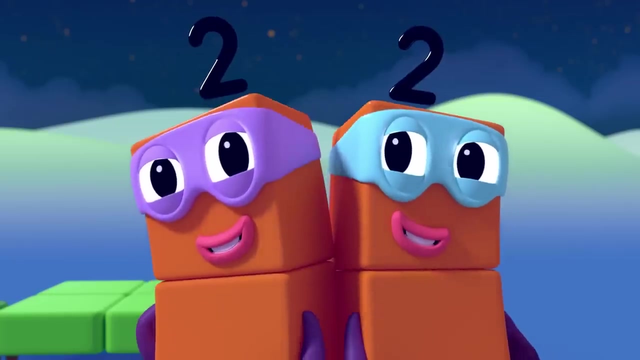 lots of one, but I'm also two lots of two. You're funny, Don't be silly, That's a very funny joke. Four equals two plus two, The terrible twos Shh, I'm number one And this is fun. 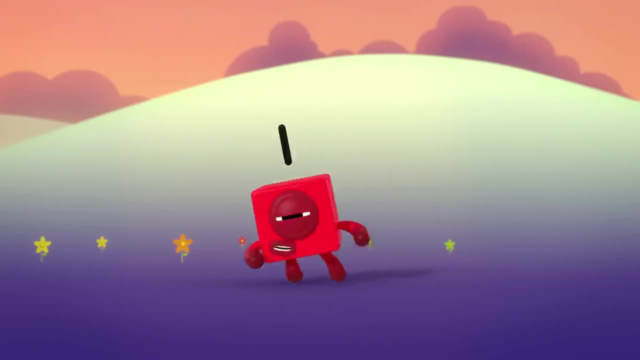 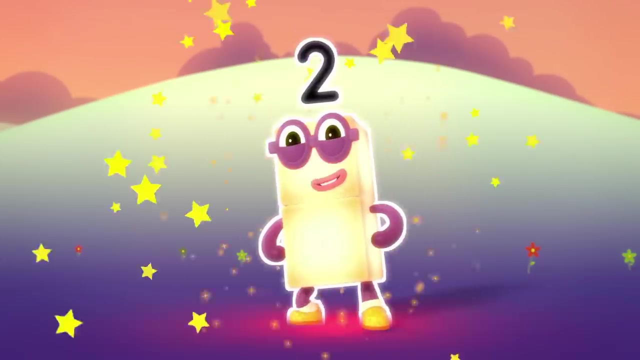 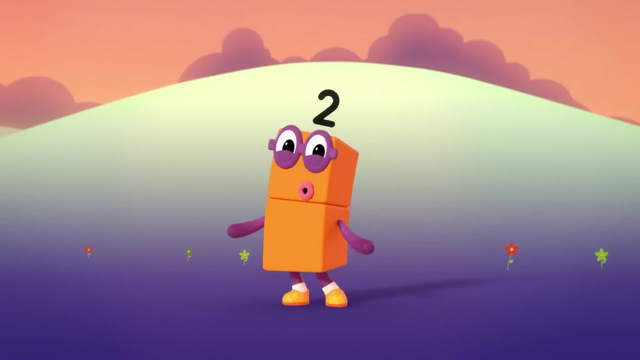 I've got one block to play with and the whole of me is one. One, One, two, one, two. I'm number two. How do you do? I've got two blocks to play with and the whole of me is two. 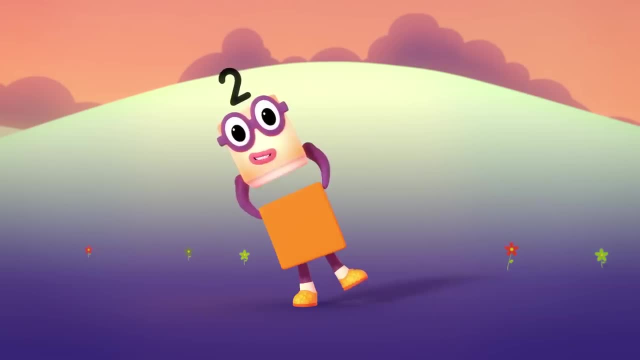 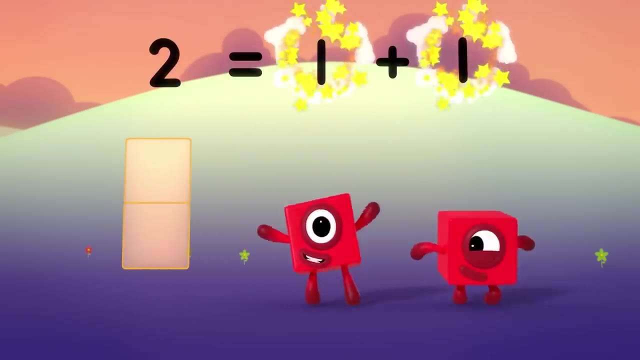 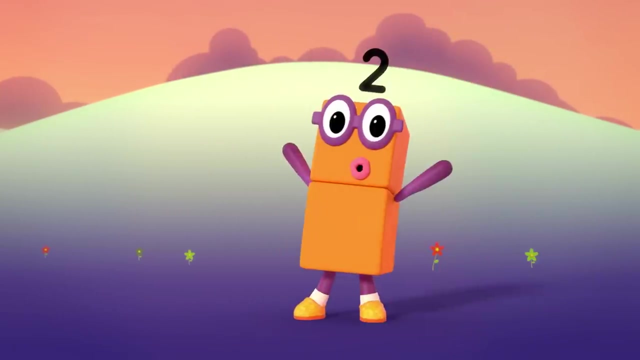 One, two. One is a part of me and one is a part of me, and the whole of me is two. Watch, I'm one and I'm a part. I'm one and I'm a part, And the whole of me is two. 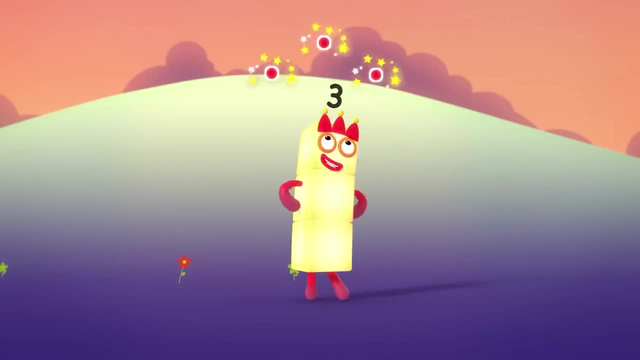 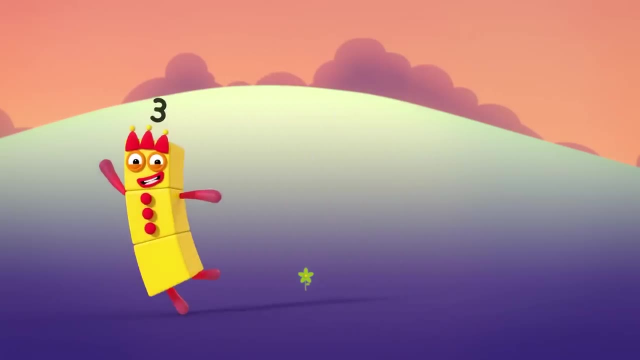 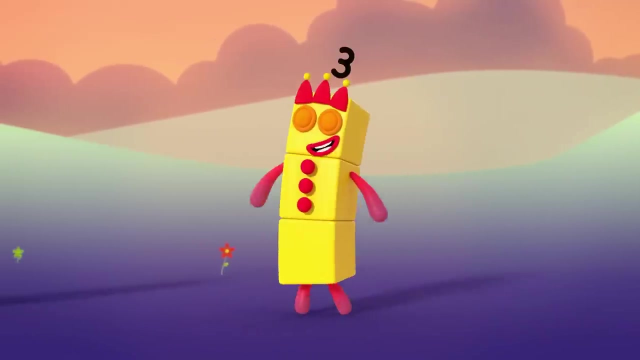 One, two, three, One, two, three, One, two, three. I'm number three. Now look at me. I'm the best. I'm the best of all the number blocks, as you can plainly see. The whole of me is amazing. 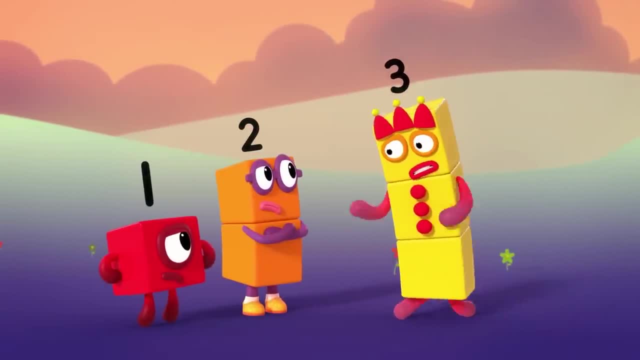 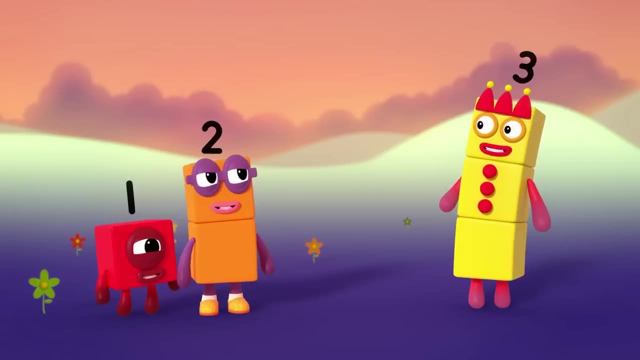 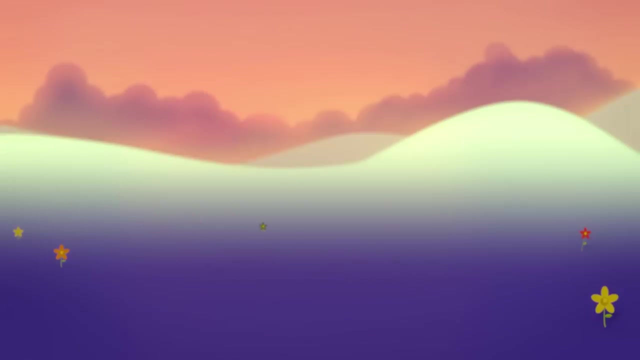 The whole of me is so great. The whole of me is Sorry. Three, Try again. Okay, I'm number three. Yes, look at me, I'm the best of all, the number. Oh, you can't do it. 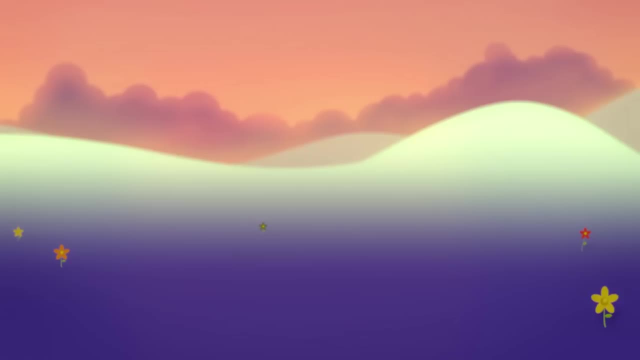 You can't do it. You can't do it. I am number three. One more time, I'm number three. Now look at me. I've got three blocks to play with and the whole of me is three. One, two, three. 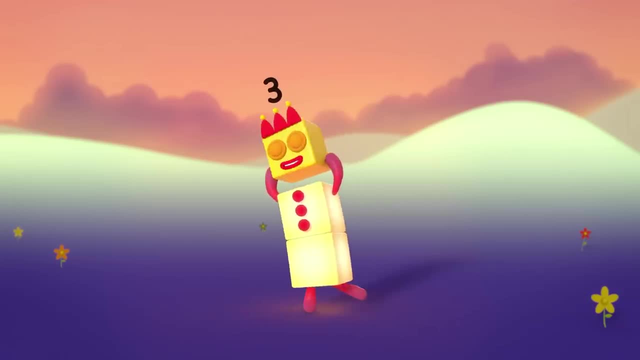 One is a part of me and two is a part of me, and the whole of me is three. Watch, I'm two and I'm a part. I'm one and I'm a part And the whole of me is three. One, two, three. 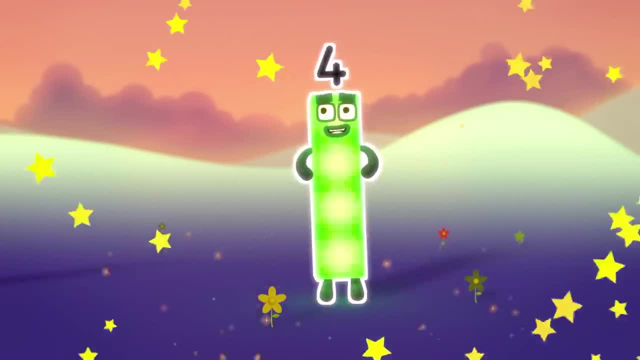 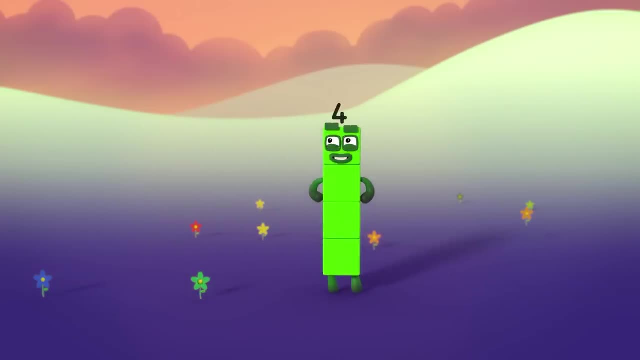 I'm number four And I am sure that I've got four blocks to play with, and the whole of me is four: One, two, three, four. One is a part of me and three is a part of me, and the whole of me is four. 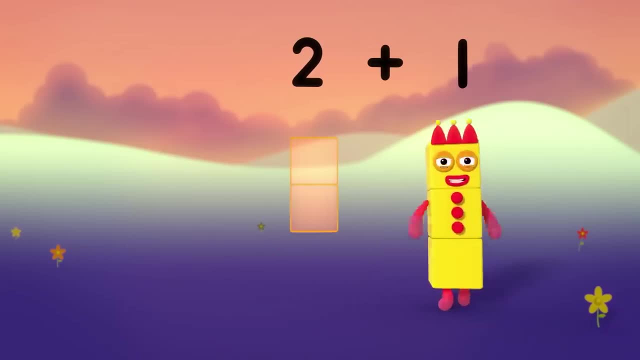 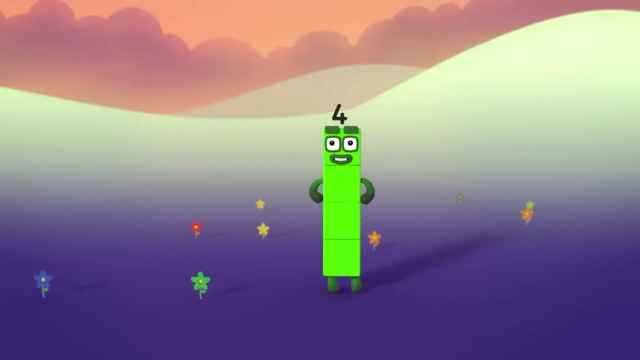 I'm one and I'm a part, And the whole of me is three. One, two, three. I'm number four And I am sure that I've got four blocks to play with, and the whole of me is four. One, two, three, four. 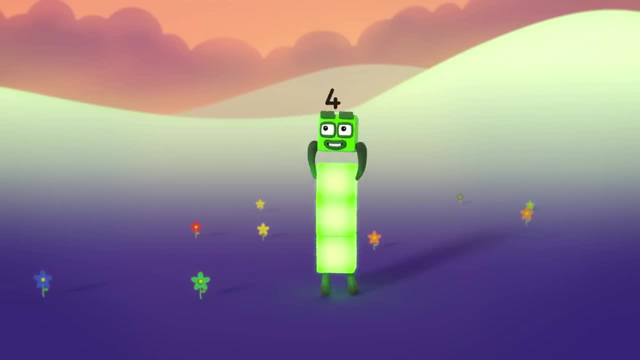 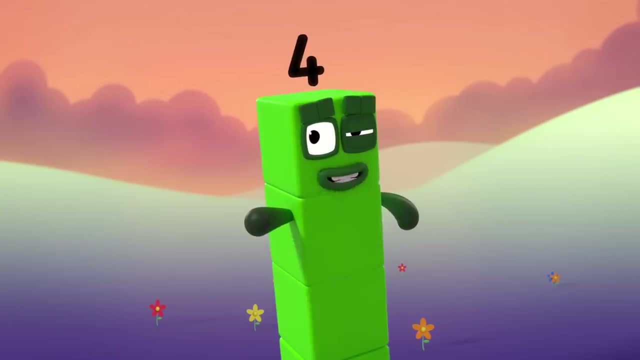 One is a part of me and three is a part of me and the whole of me is four. Watch, I'm three and I'm a part, I'm one and I'm a part And the whole of me is four. Now, here is something more that's different from before. 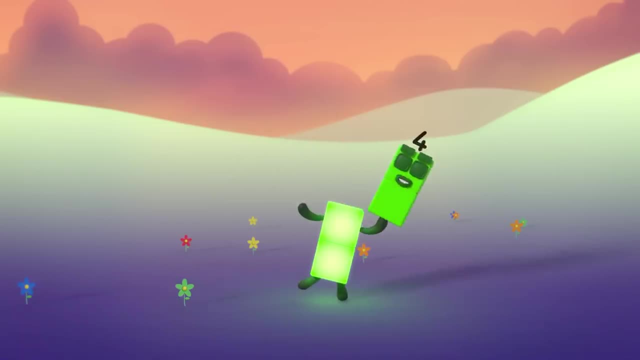 Two is a part of me, and two is a part of me, and the whole of me is four. Watch, I'm two and I'm a part. I'm two and I'm a part, And the whole of me is four. I'm a square, look. 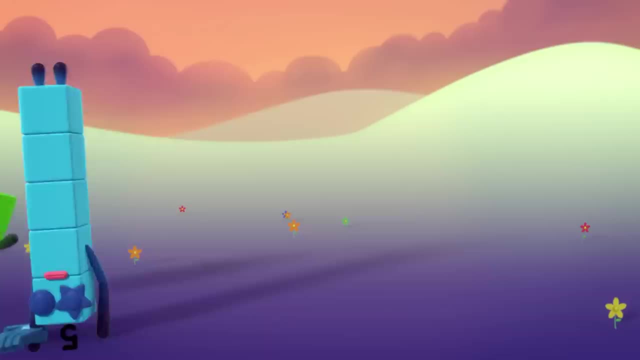 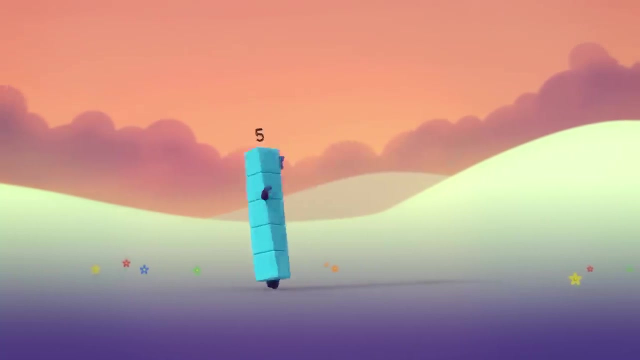 Four sides, four corners. I'm number five. I am alive. I've got five blocks to play with and the whole of me is five. One, two, three, four, five. One is a part of me and four is a part of me, and the whole of me is five. 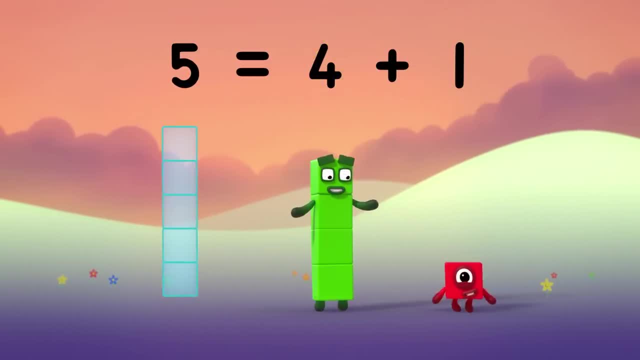 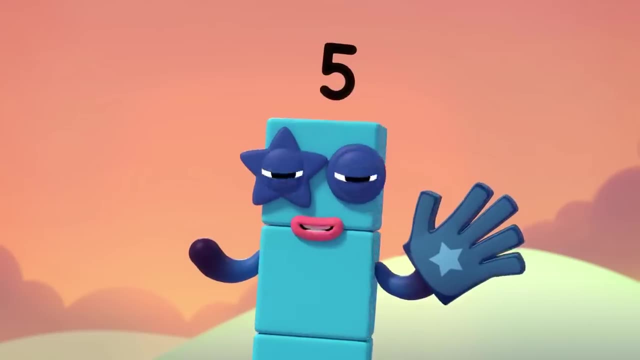 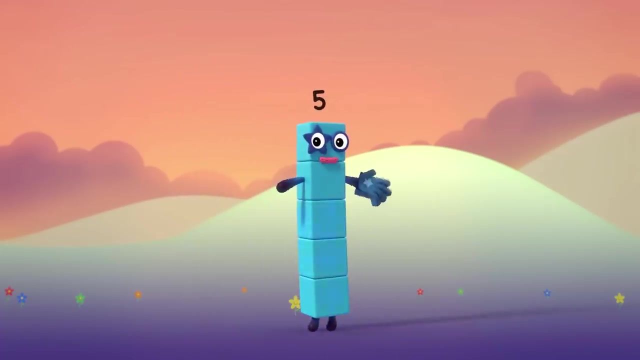 Watch. I'm four and I'm a part, I'm one and I'm a part, I'm two and I'm a part, And the whole of me is five. But now I feel alive, going into overdrive. Two is a part of me and three is a part of me, and the whole of me is five. 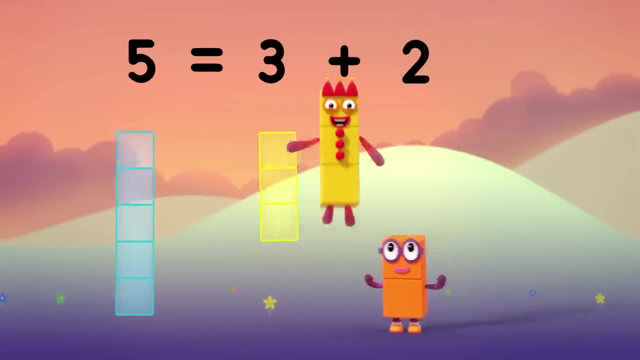 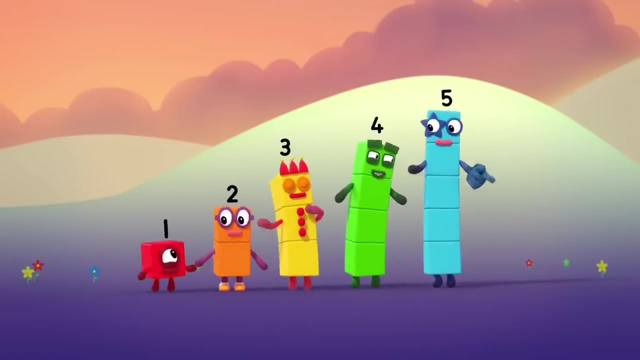 One and three, and I'm a part, I'm two and I'm a part, And the whole of me is five High five. Making friends is easy when you can come apart. Making love is not so hard. it won't break your heart. 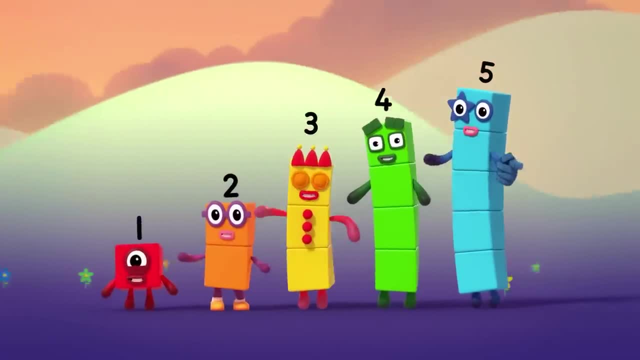 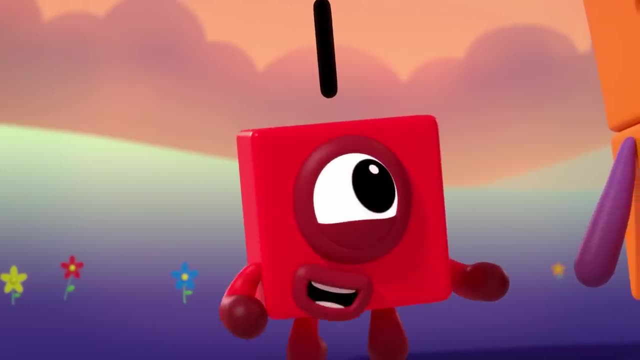 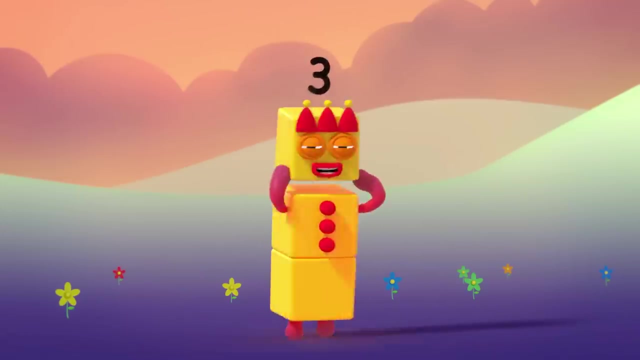 So when we fall to pieces, we have lost control. A whole is made of all its parts and the parts they make a whole. Just remember that One is a part of me and one is a part of me. One is a part of me and two is a part of me. 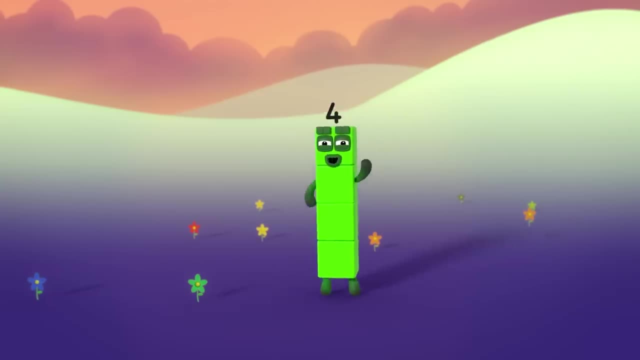 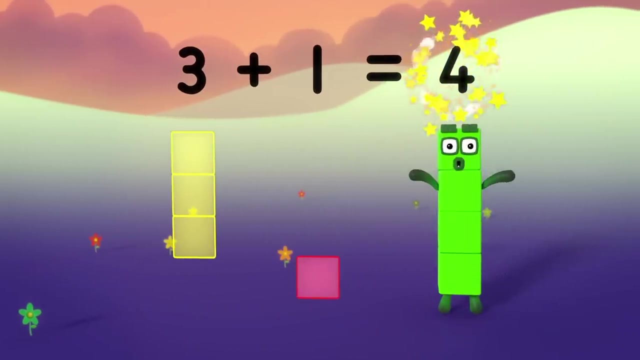 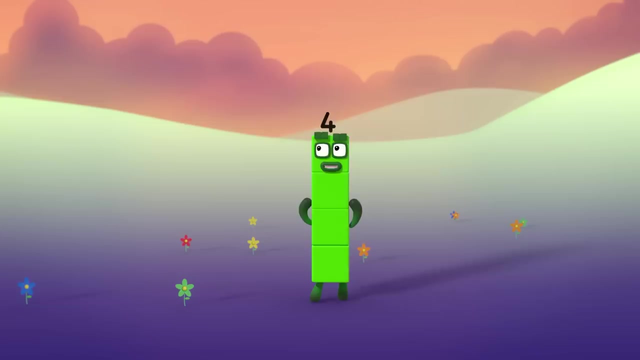 Watch. I'm three and I'm a part, I'm one and I'm a part, And the whole of me is three And the whole of me is four. Now here is something more that's different from before. Two is a part of me. 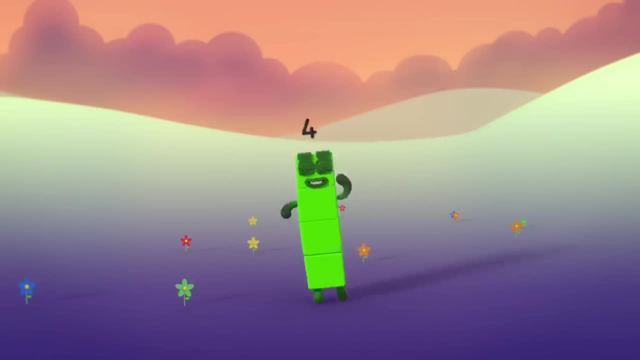 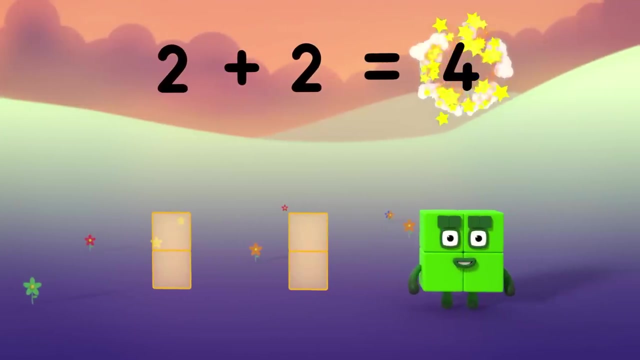 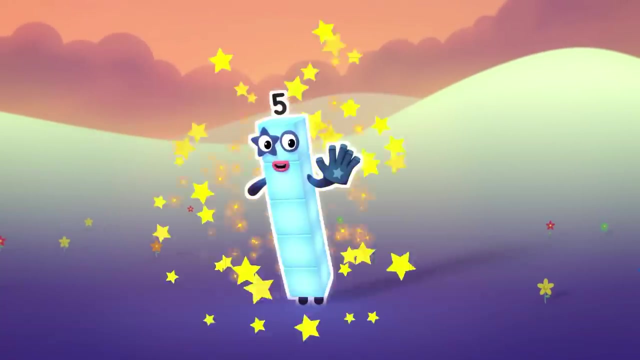 and two is a part of me and the whole of me is four. Watch, I'm two and I'm a part. I'm two and I'm a part, And the whole of me is four. I'm a square. look Four sides, four corners. 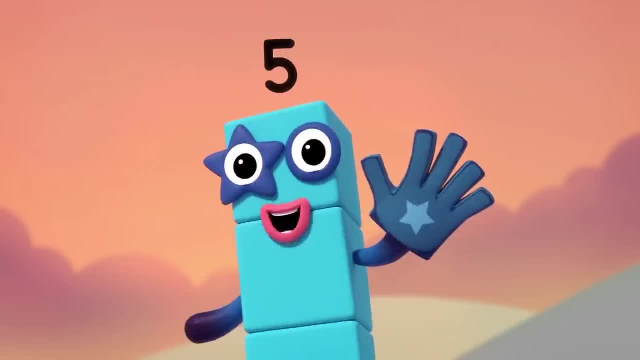 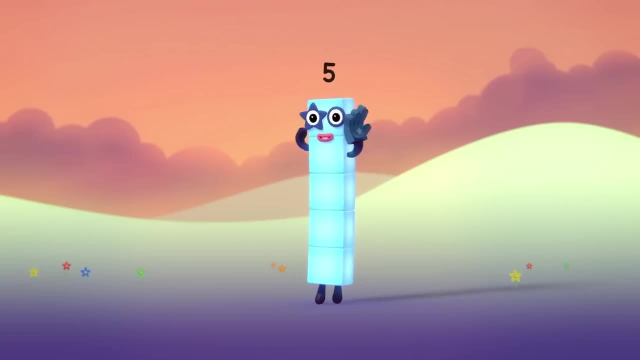 I'm number five. I've got five blocks to play with and the whole of me is five. One, two, three, four, five. One is a part of me and four is a part of me, and the whole of me is five. 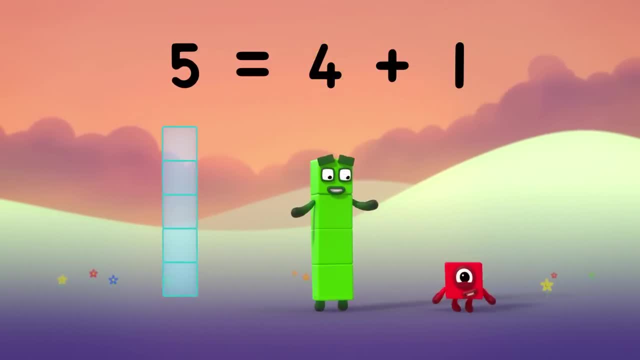 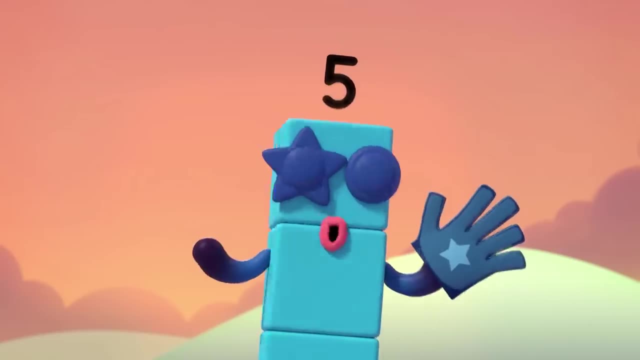 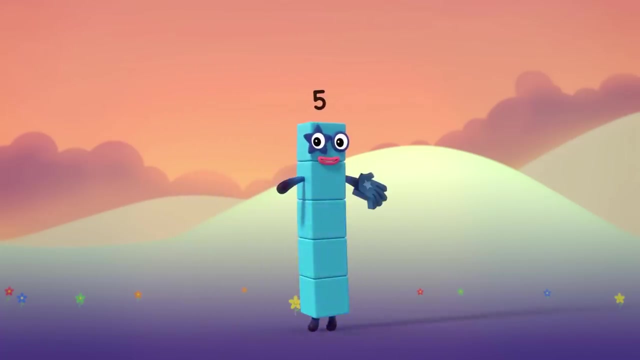 Watch. I'm four and I'm a part, I'm one and I'm a part, And the whole of me is five. But now I feel alive going into overdrive. Two is a part of me and three is a part of me. 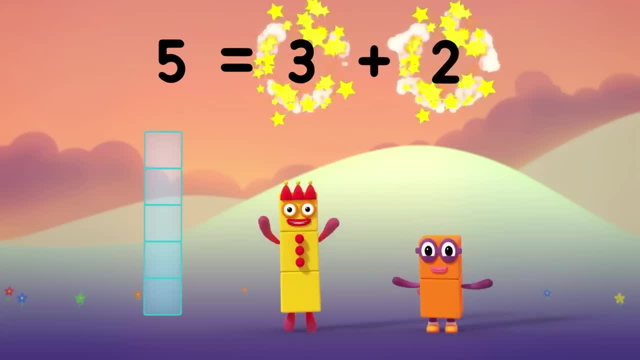 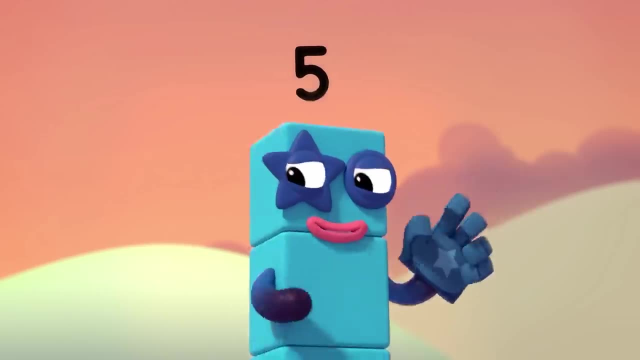 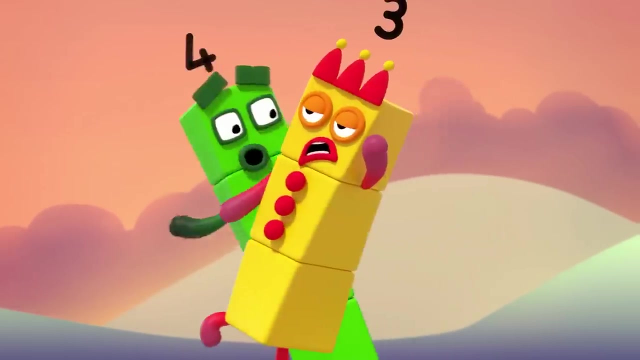 and the whole of me is five. One and three and I'm a part, I'm two and I'm a part, And the whole of me is five High five. Making friends is easy when you can come apart. Splitting up is not so hard. 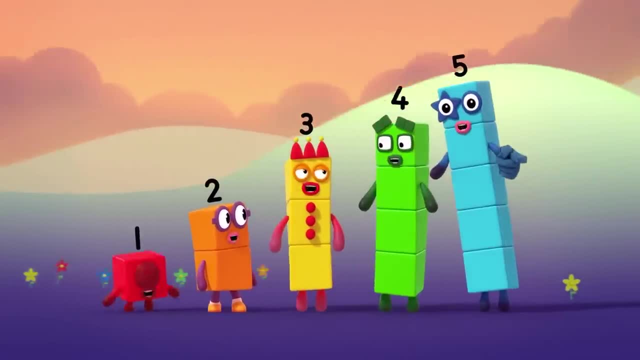 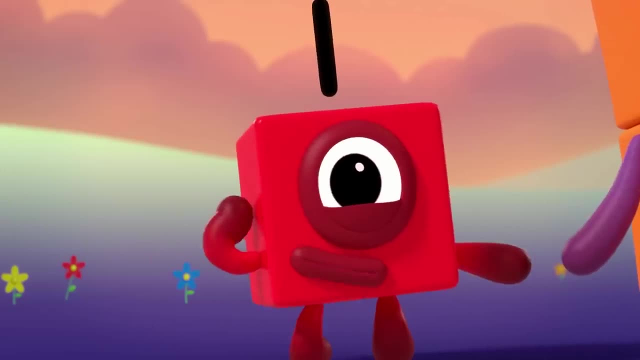 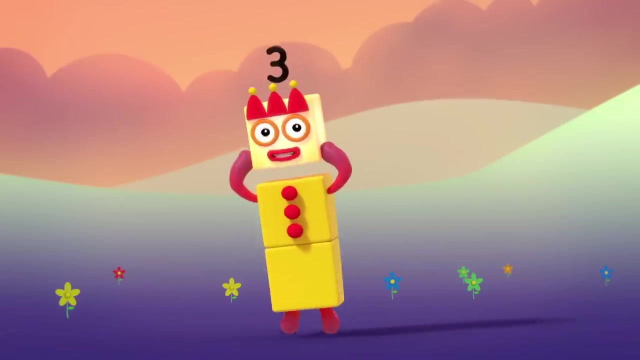 it won't break your heart. So when we fall to pieces, we have lost control. A hole is made of all its parts and they make a hole. Just remember that. One is a part of me and one is a part of me. One is a part of me. 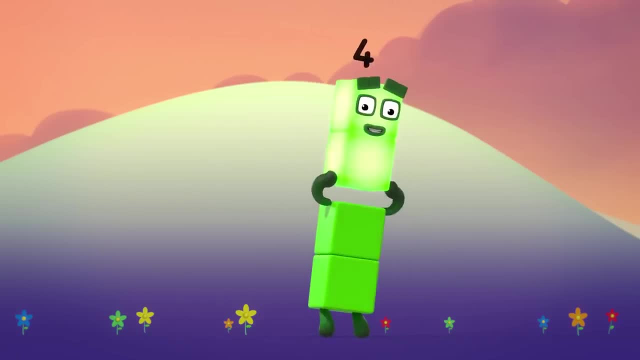 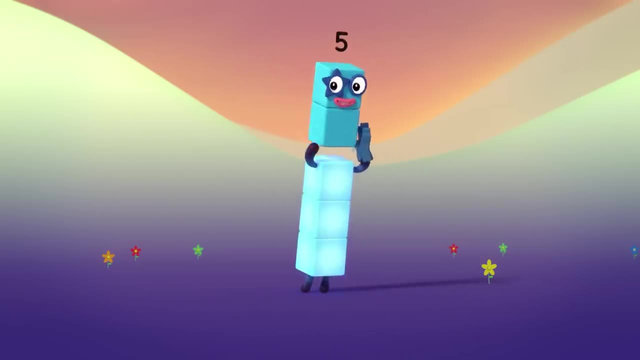 and two is a part of me. One is a part of me and three is a part of me. Two is a part of me and two is a part of me. One is a part of me and four is a part of me. Two is a part of me. 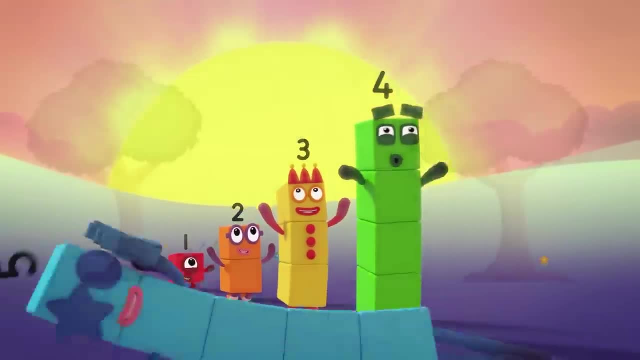 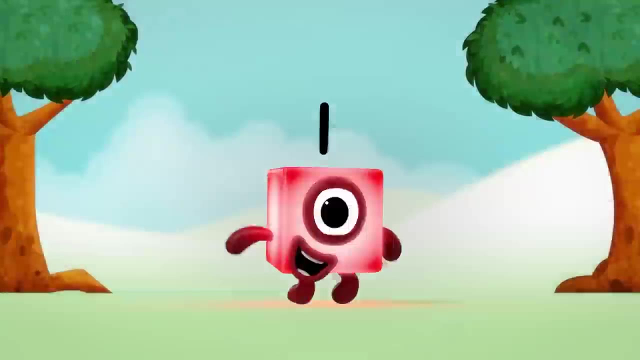 and three is a part of me, Two is a part of me and four is a part of me. If there's nothing going on, no one's there and it's no fun. you can get the party started with a bang by adding one. I am one. 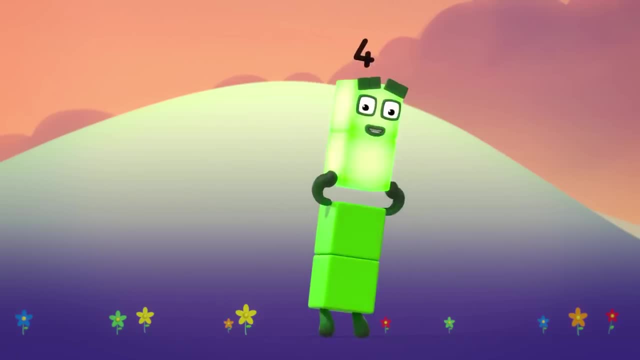 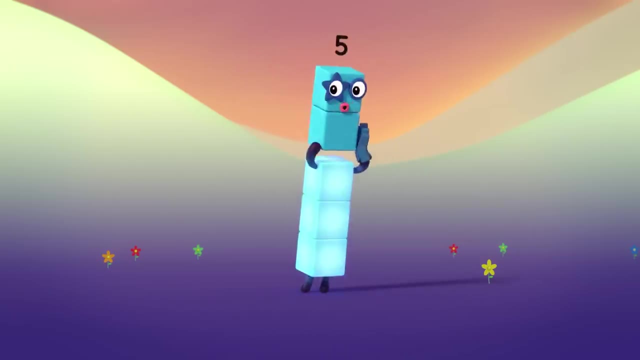 One is a part of me and three is a part of me. Two is a part of me and two is a part of me. One is a part of me and four is a part of me. Two is a part of me and three is a part of me. 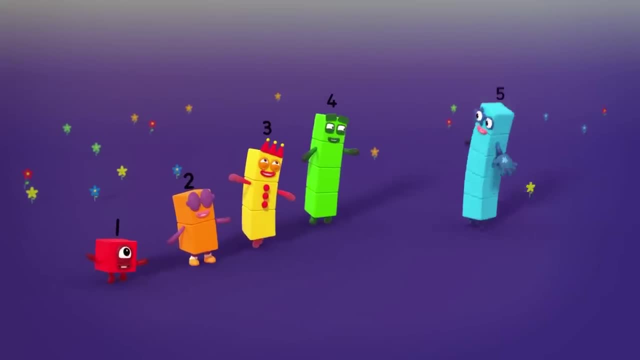 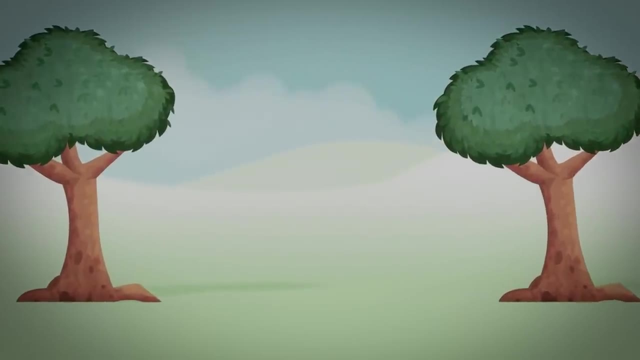 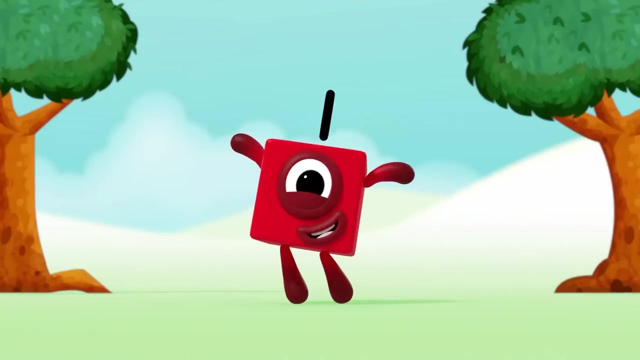 And the whole of me is one, two, three, four. If there's nothing going on, no one's there and it's no fun. you can get the party started with a bang by adding one. I am one and I'm playing in the sun. 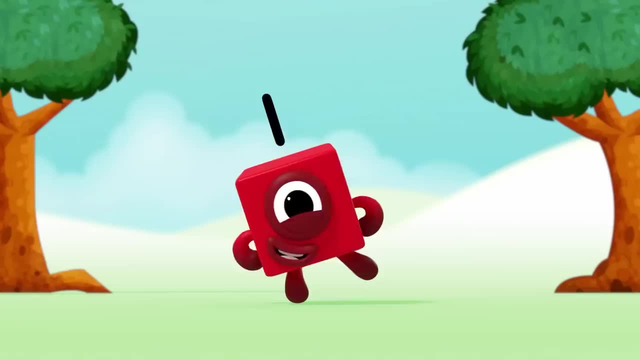 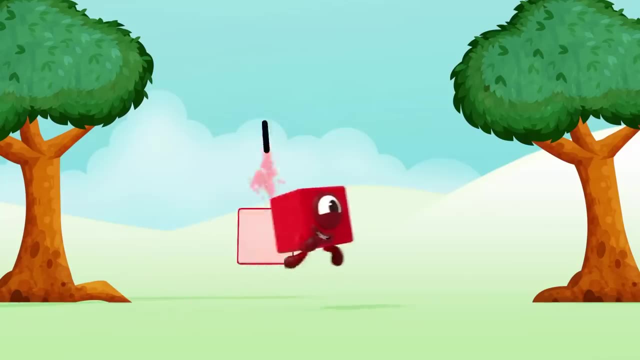 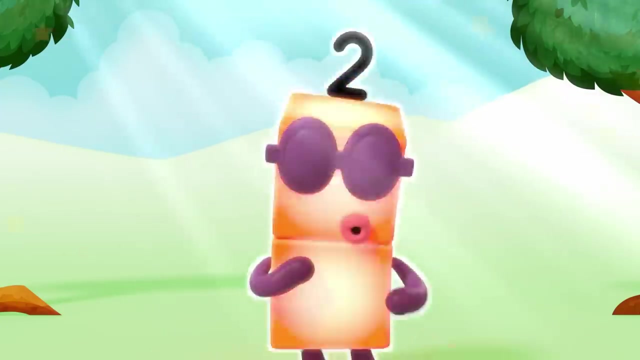 Being one is my idea. One is my idea of fun. One, One little block. Now let's add another one. One plus one equals two. I am two and I'm playing in the sun. A song and dance is my idea of fun. 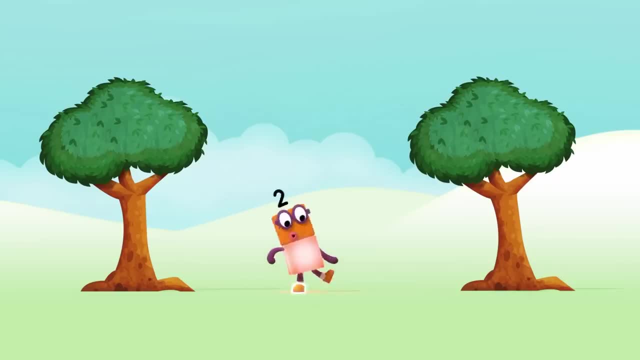 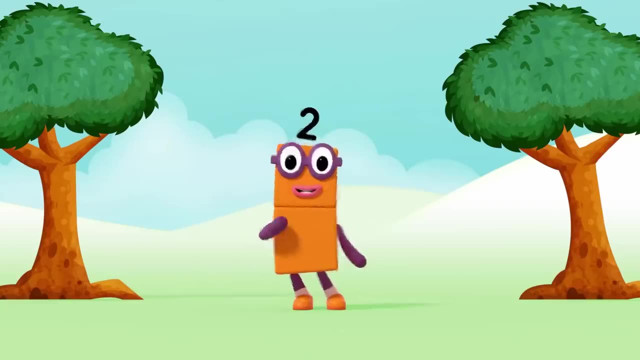 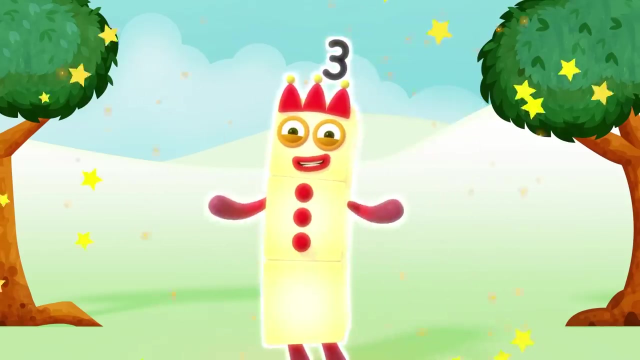 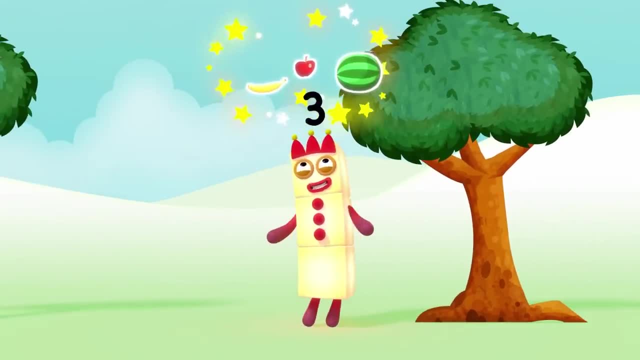 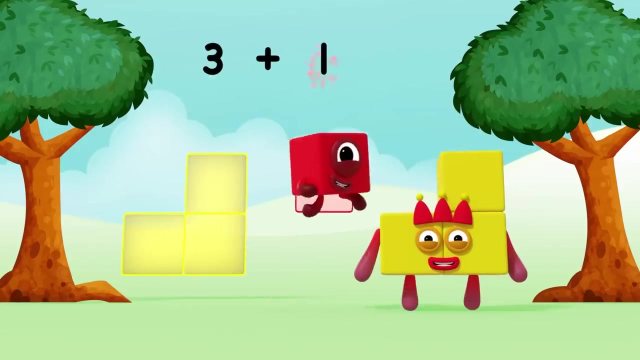 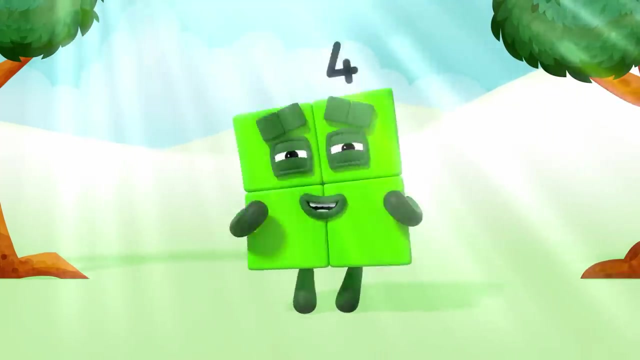 One, two, three, Three things. Look at me: One, two, three. Now let's add another one. Three plus one equals four. I am four and I'm playing in the sun. Being square is my idea of fun. 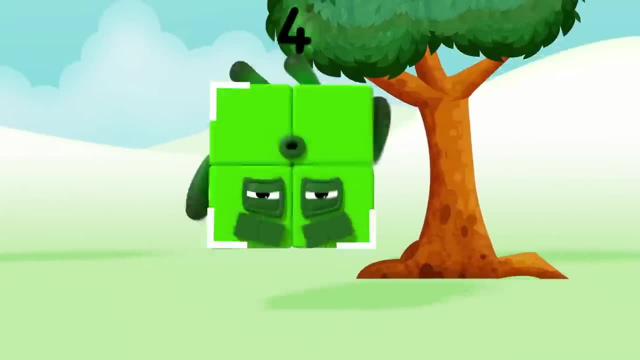 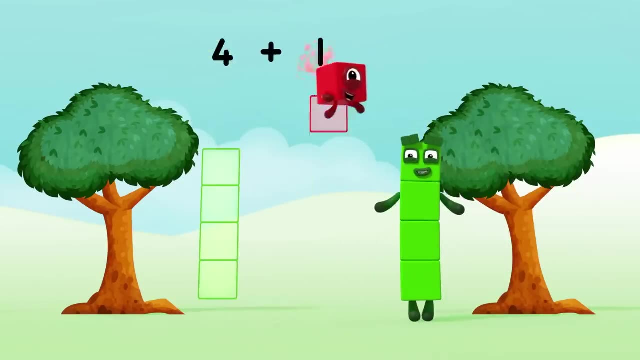 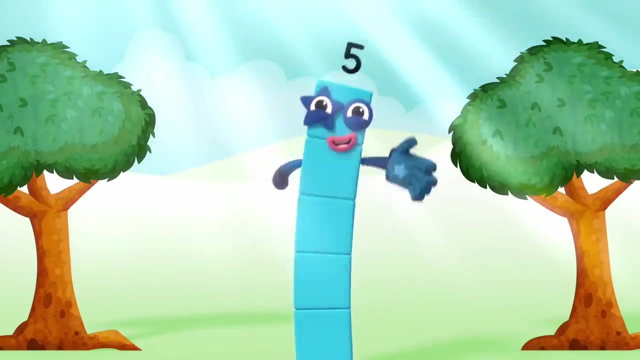 One, two, three, four, Four sides. Ouch, ouch, ouch, ouch, Four corners. Now let's add another one. Four plus one equals five. I am five and I'm playing in the sun. High five are my idea of fun. 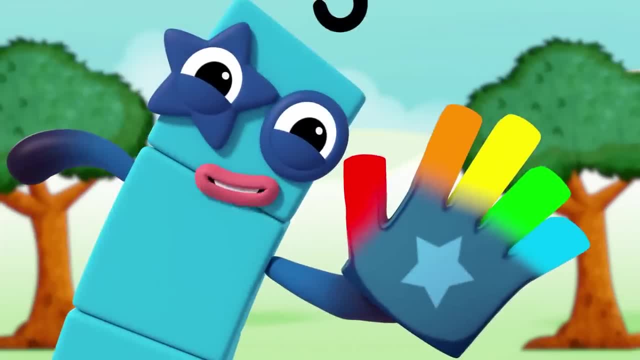 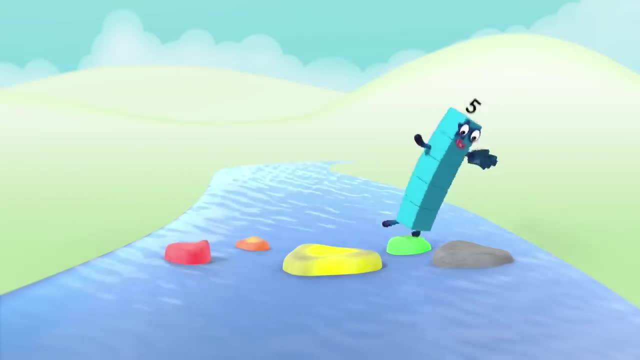 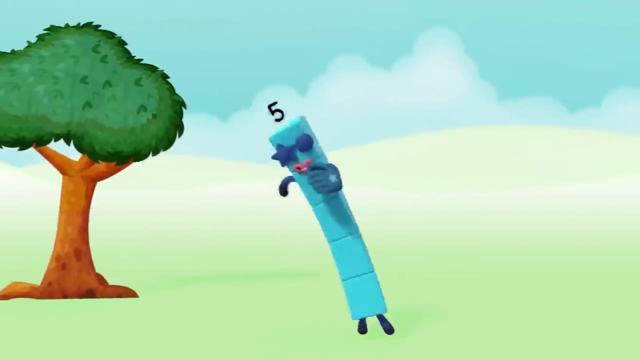 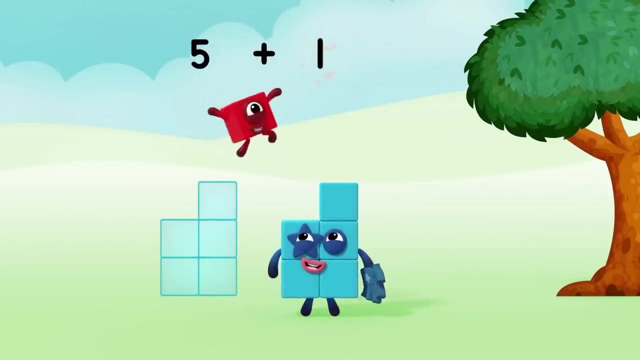 One, two, three, four, five, Five fingers. If you add another one, the number gets one bigger, And if you keep on adding one, you can get to any figure. Now let's add another one. Five Plus one equals six. 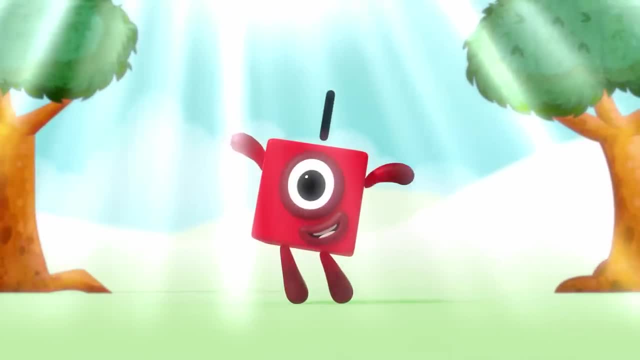 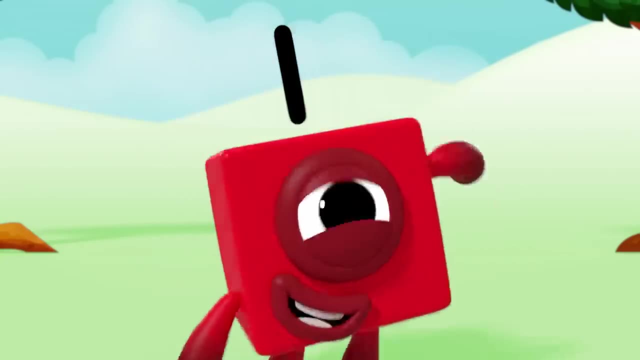 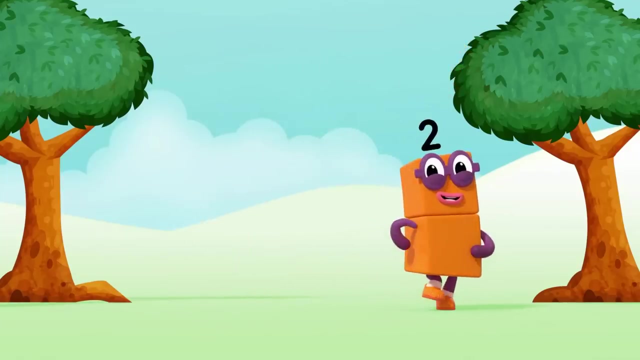 and I'm playing in the sun. Being one is my idea of fun. One, One little block. Now let's add another one. One plus one equals two. I am two and I'm playing in the sun. A song and dance is my idea of fun. 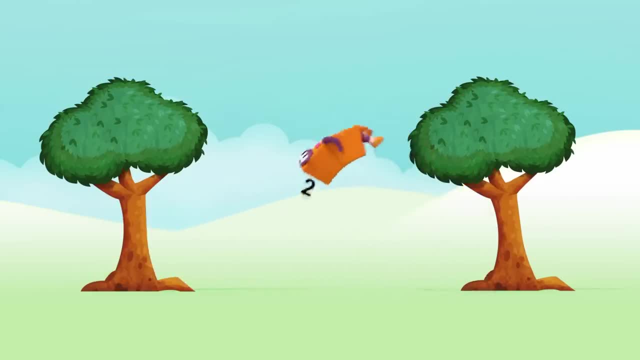 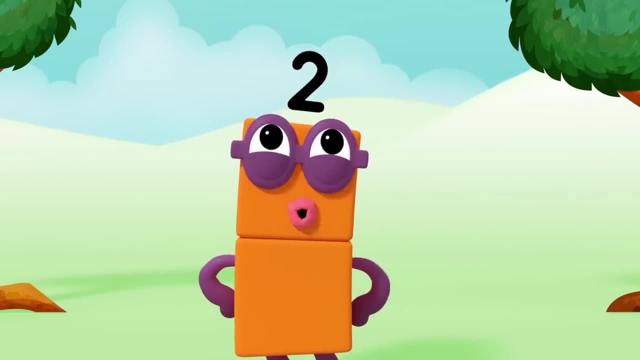 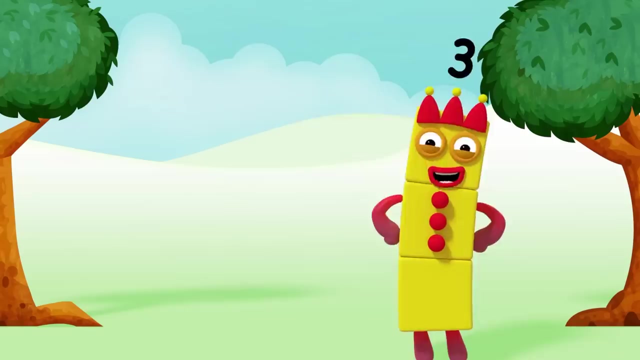 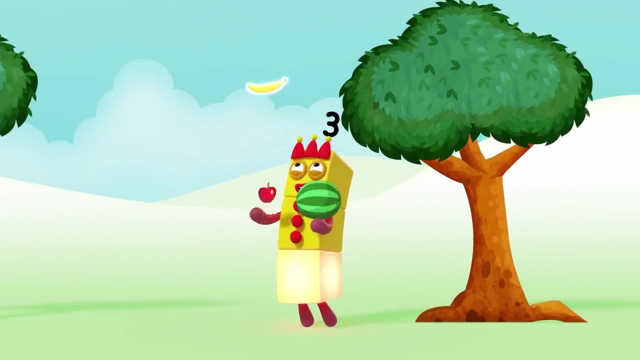 One, two, One, two, One, two, Two dancing shoes. Now let's add another one. Two plus one equals three. I am three and I'm playing in the sun. Juggling things is my idea of fun. One, two, three. 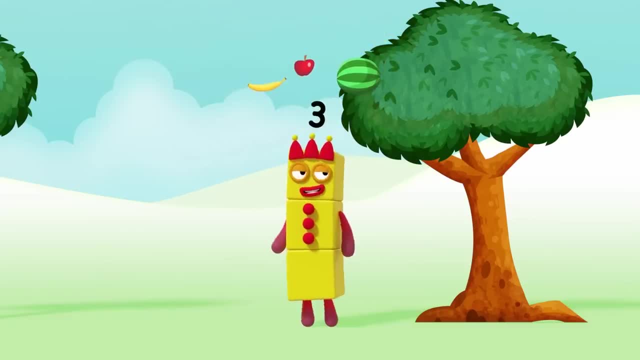 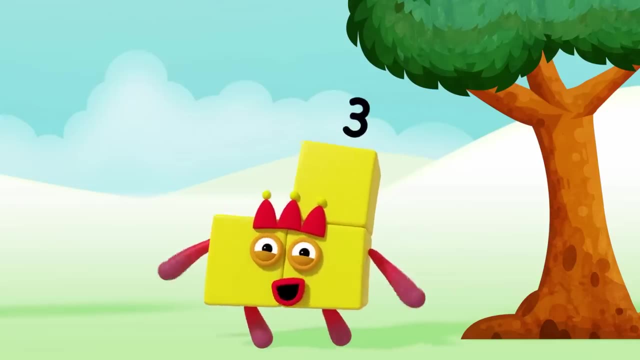 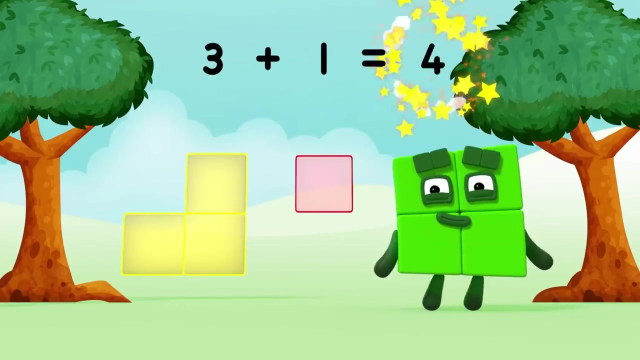 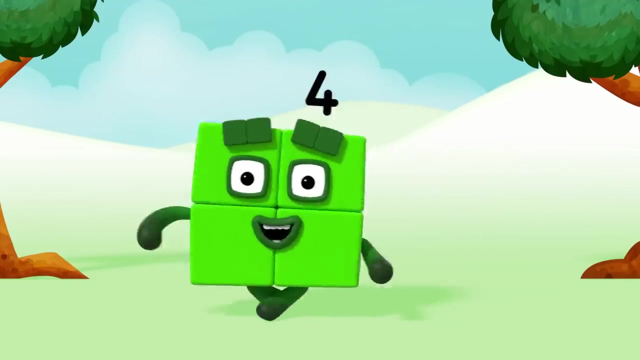 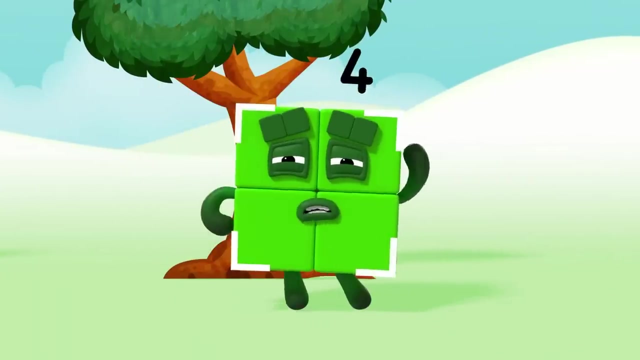 Three things. Look at me: One, two, three. Now let's add another one. Three plus one equals four. I am four and I'm playing in the sun. Juggling things Is my idea of fun. One, two, three, four, Four sides. 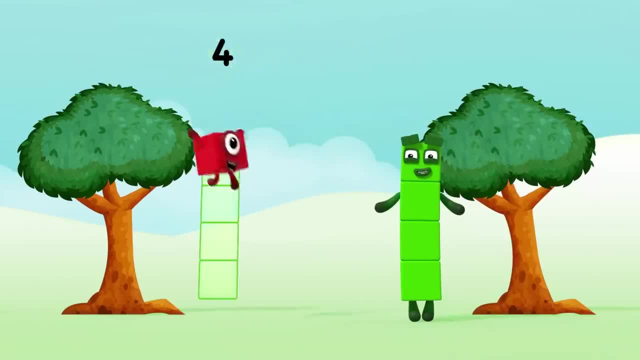 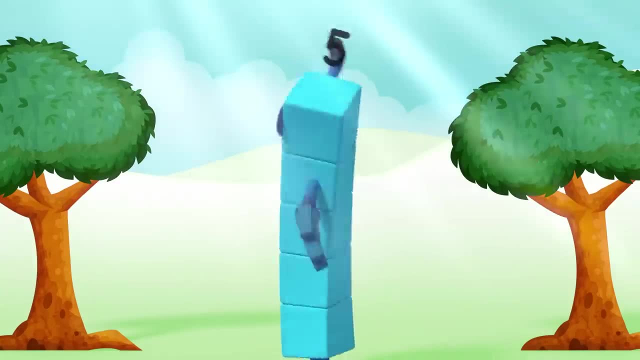 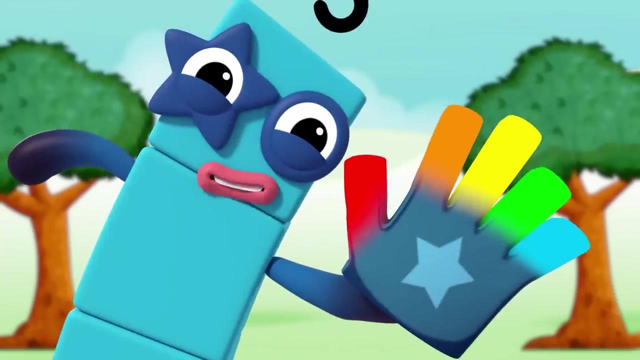 Out, out, out out Four corners. Now let's add another one. Four plus one equals five. I am five and I'm playing in the sun. High five are my idea of fun. One, two, three, four, five If you add another one. 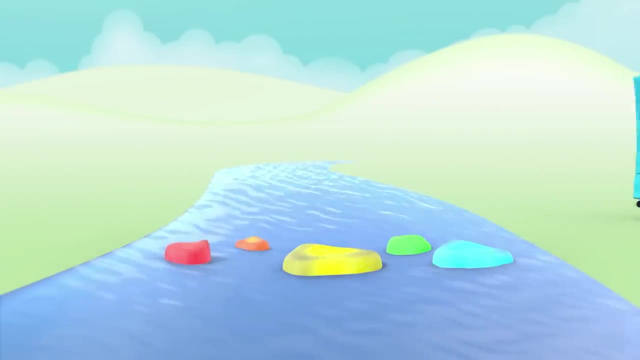 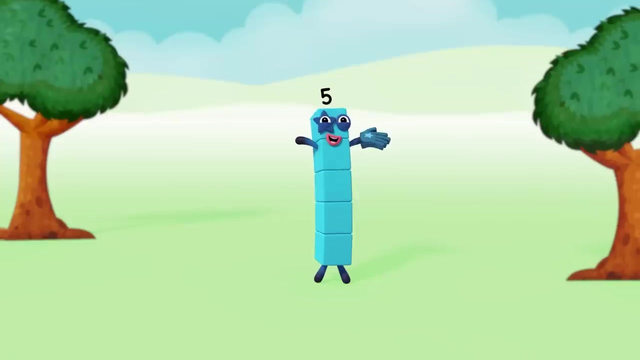 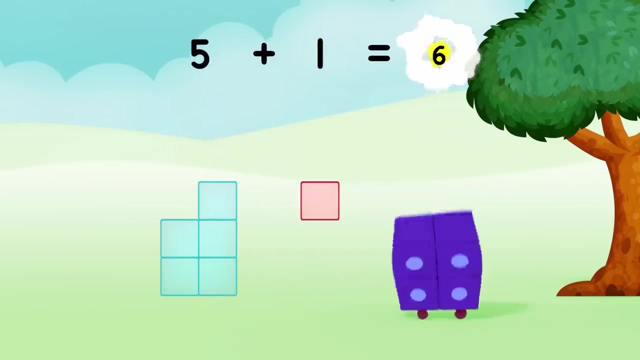 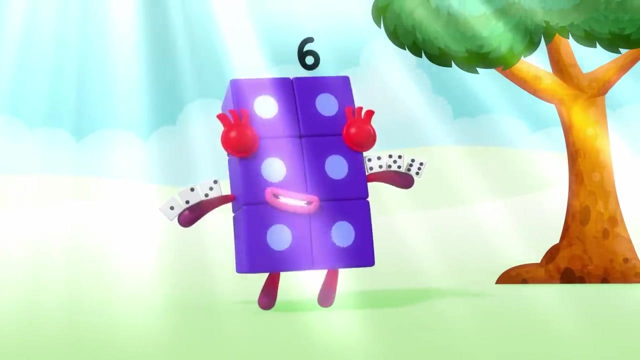 the number gets one bigger, And if you keep on adding one you can get to any bigger. Now let's add another one. Five plus one equals six. I am six and I'm playing in the sun. Playing games is my idea of fun. 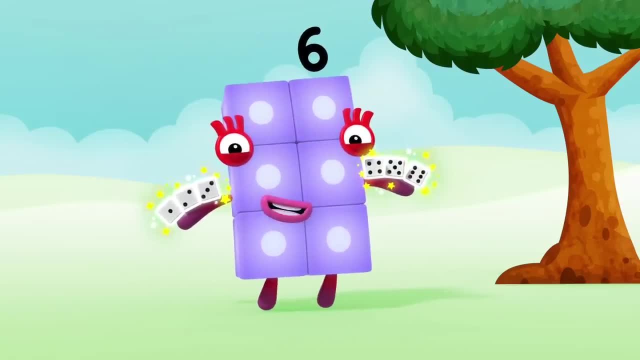 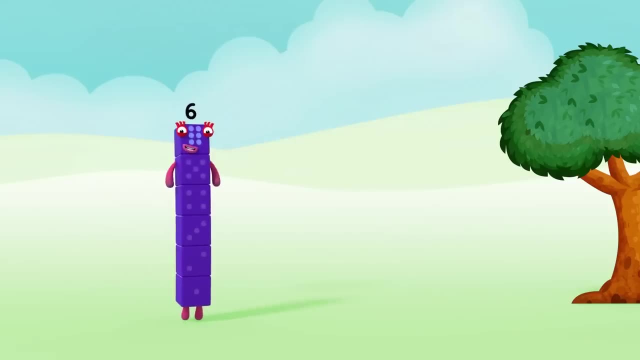 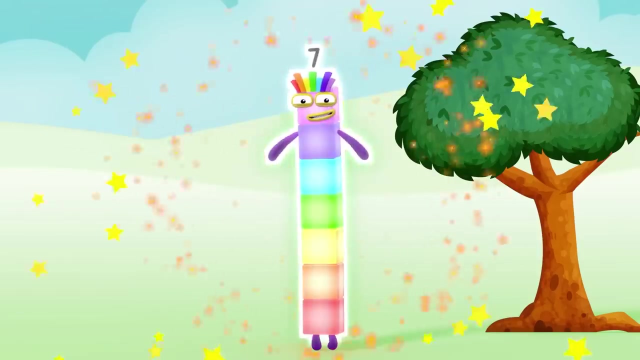 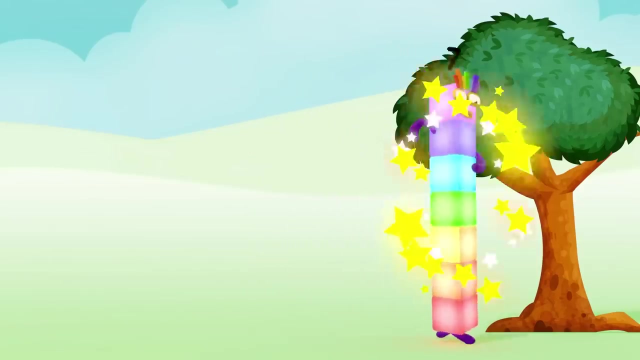 One, two, three, four, five, Six, Six dice. Now let's add another one. Six plus one equals seven. I am seven and I'm playing in the sun. Making rainbows Is my idea of fun. One, two, three, four, five, six, seven. 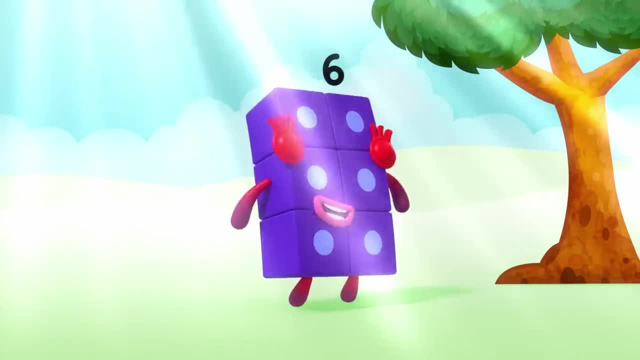 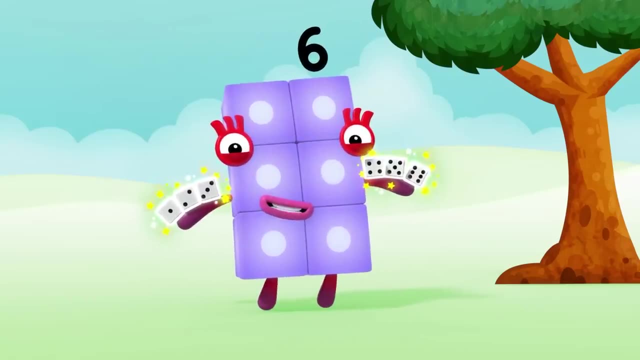 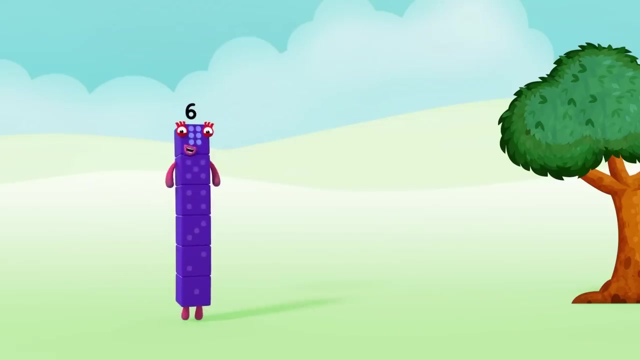 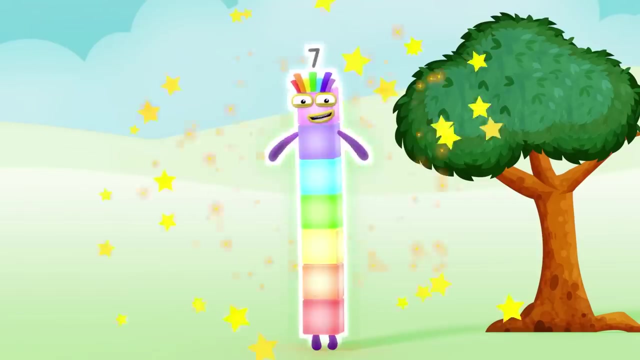 I am six and I'm playing in the sun. Playing games is my idea of fun. One, two, three, four, five, six, Six dice. Now let's add another one. Six plus one equals seven. I am seven and I'm playing in the sun. 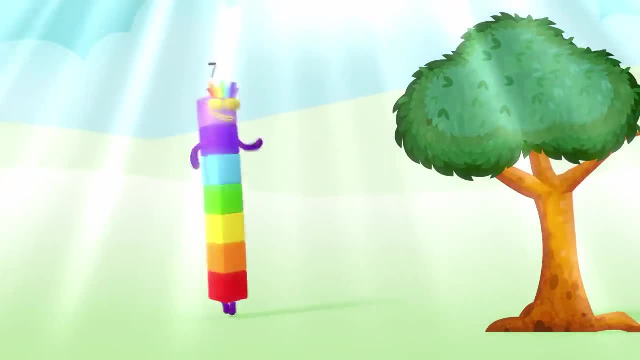 Making rainbows Is my idea of fun. One, two, three, four, five, six, seven, Seven colors. Now let's add another one. Seven plus one equals Seven plus one equals eight. I am eight and I'm playing in the sun. 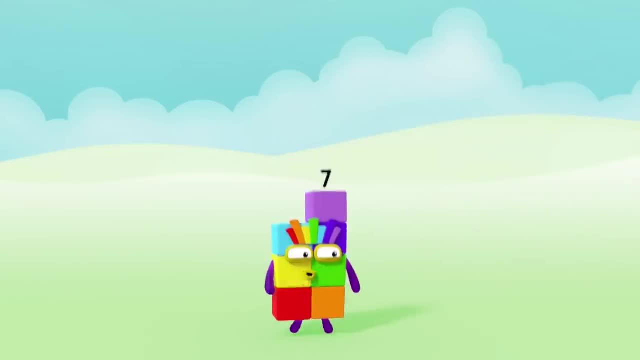 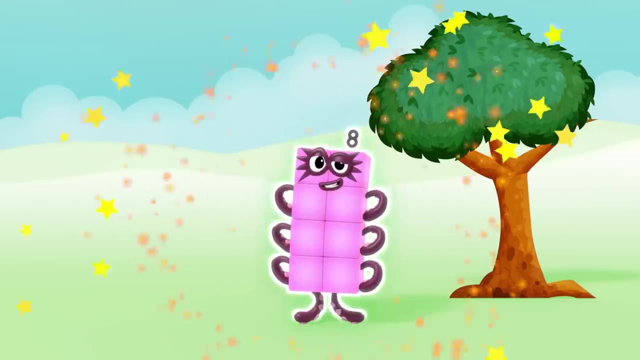 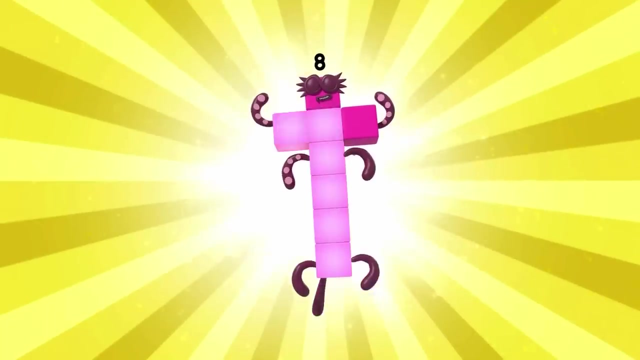 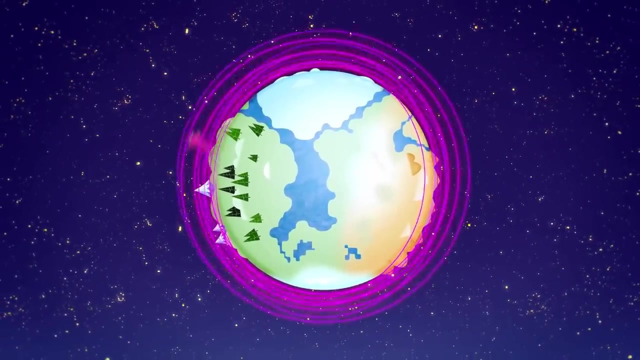 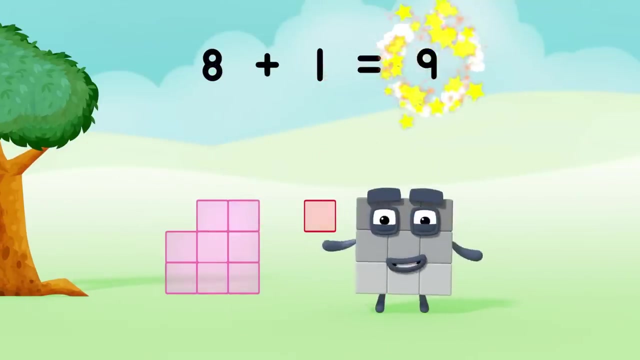 Being octoblock is my idea of fun. Octoblock run: One, two, three, four, five, six, seven, eight run. Now let's add another one. Eight Plus one equals Nine. I am nine. 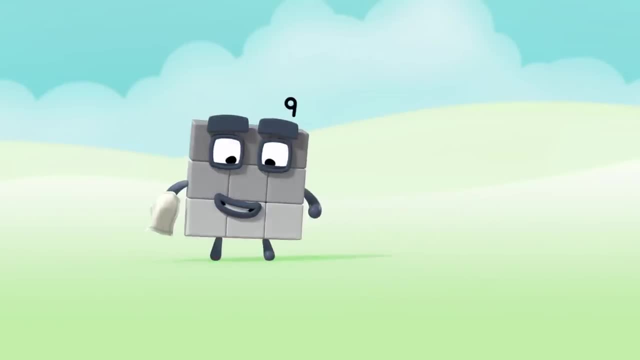 I am nine And a playing in the sun, not sneezing, is my idea of fun. One, two, three, four, five, six, seven, eight, nine, Nine hankies. Now let's add another one. 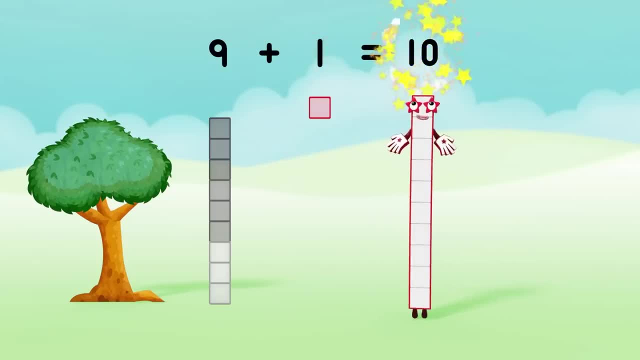 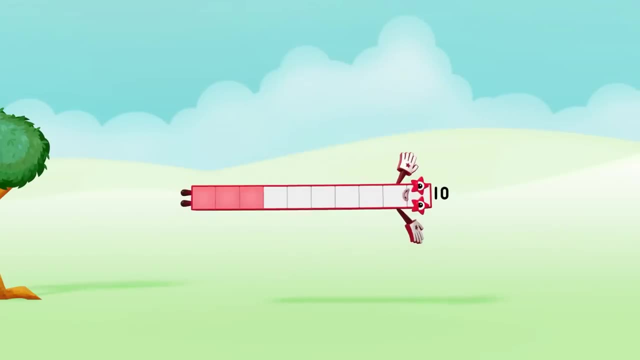 Nine plus one equals ten. I am ten And a playing in the sun. being ten is my idea of fun. One, two, three, four, five, six, seven, eight, nine, ten, Ten blocks: We're ten ones. 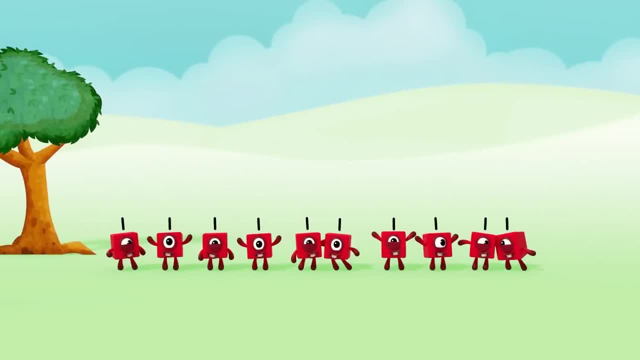 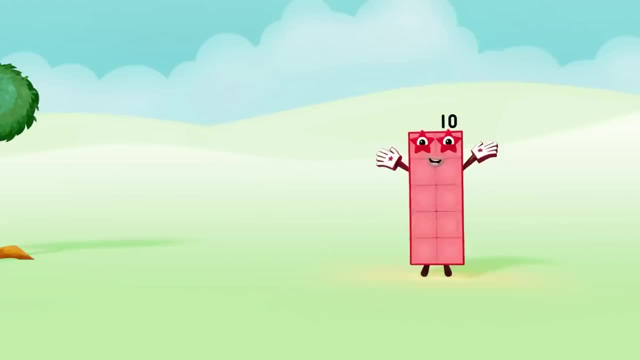 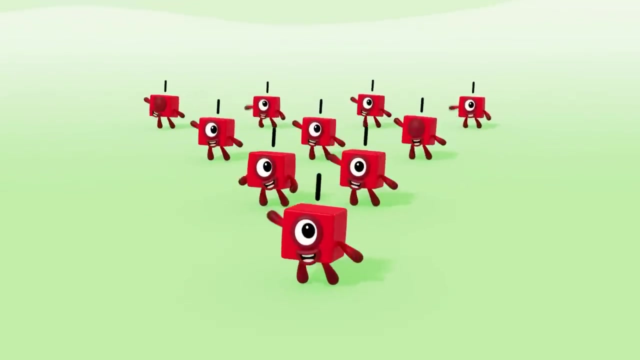 And we're playing in the sun. making friends is our idea of fun. One, two, three, four, five, six, seven, Nine, eight, nine, ten. Remember this forever. You can do what we've just done. 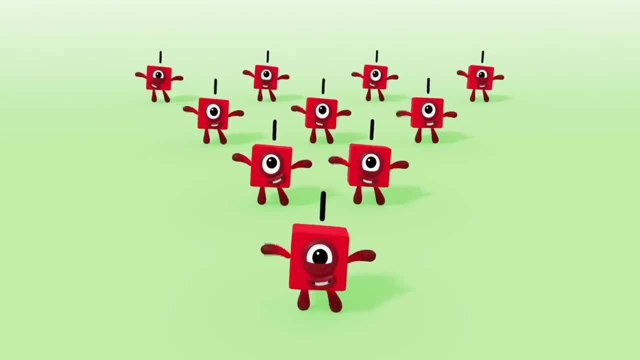 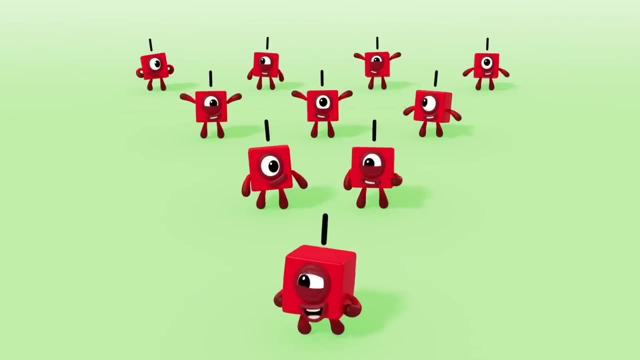 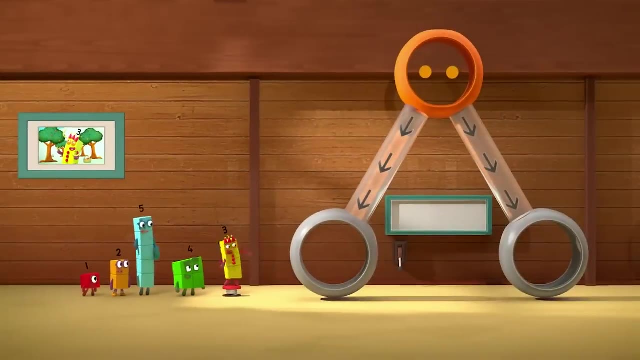 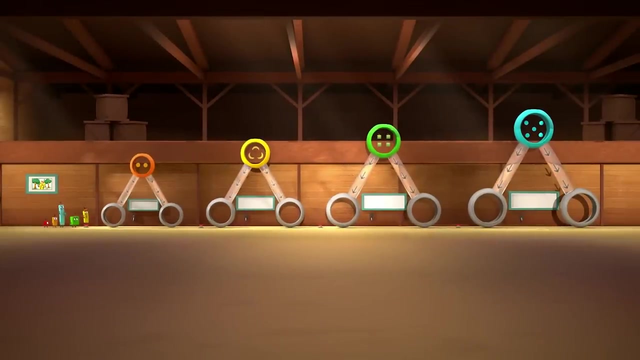 You can make any number, Then you'll keep on adding one. That was fun, Yay, Welcome, welcome. welcome to my fantastic Fun Fruit Factory Where we serve up fresh fruit all day. Ooh, Wow, How do they work. 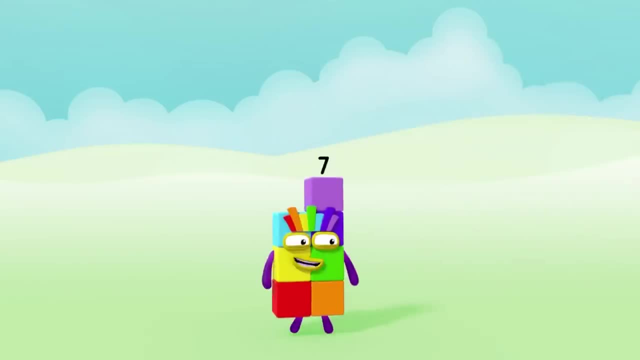 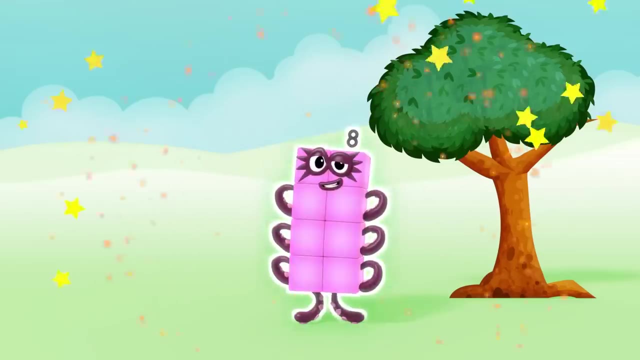 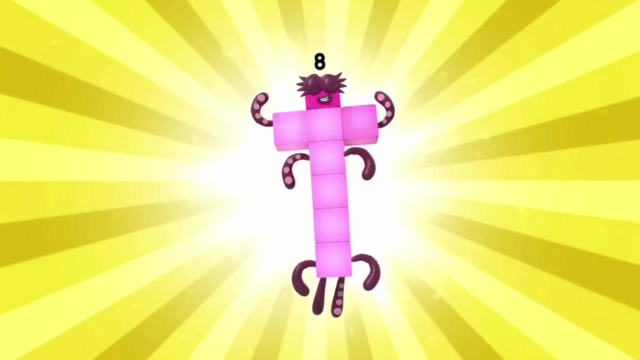 Seven colours. Now let's add another one. Eight plus one equals eight. I am eight and I'm playing in the sun. Being octoblock is my idea of fun. Octoblock run: One, two, three, four, five, six, seven, eight run. 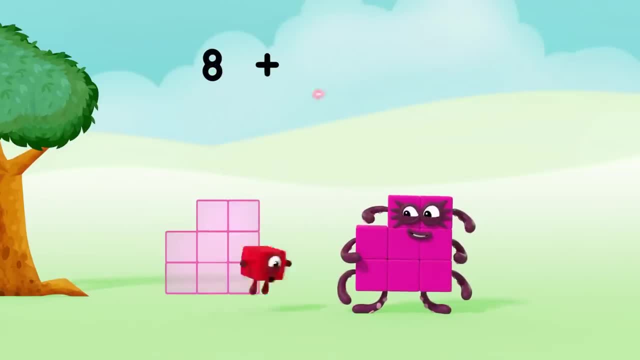 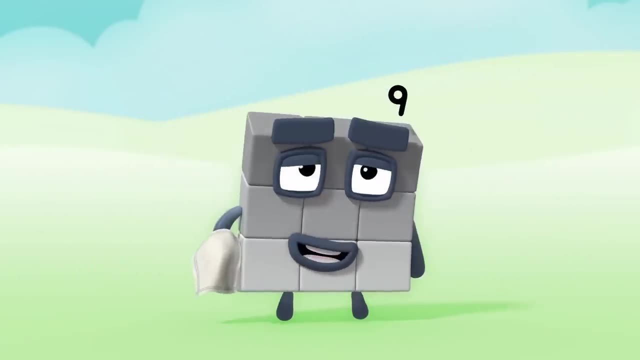 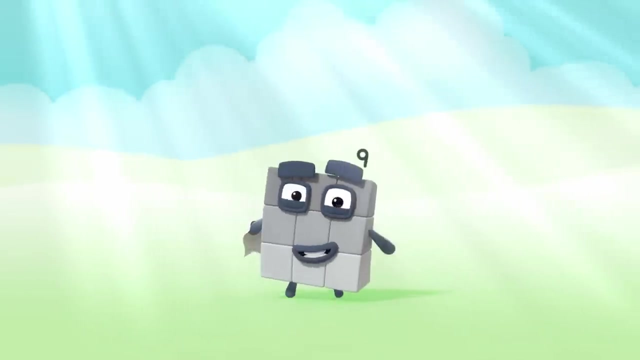 Now let's add another one. Eight plus one equals nine. I am nine, I am nine and I'm playing in the sun. Not sneezing is my idea of fun. One, two, three, four, five, six, seven, eight, nine, Nine hankies. 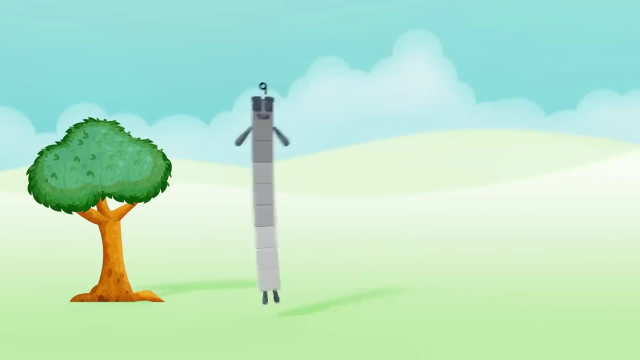 Now let's add another one. Nine plus one equals ten. I am ten and I'm playing in the sun. Being ten is my idea of fun. One, two, three, four, five, six, seven, eight, nine, ten, Ten blocks: We're ten ones and we're playing in the sun. 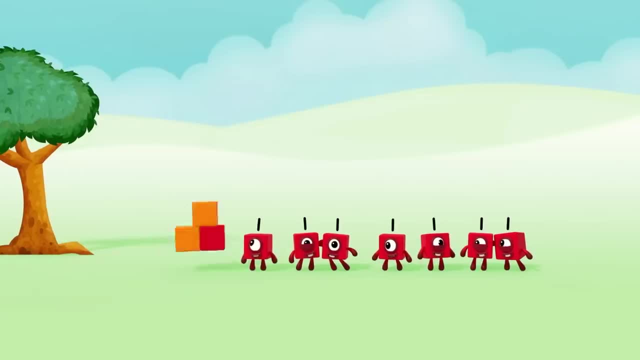 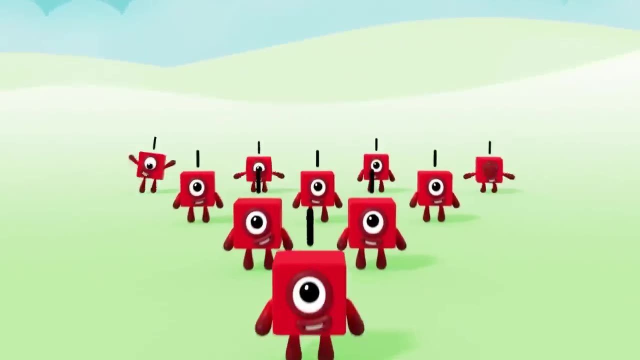 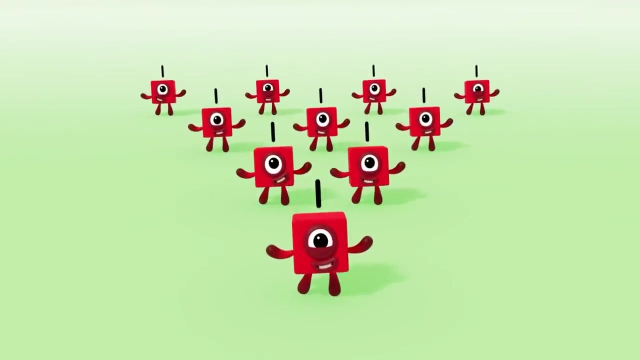 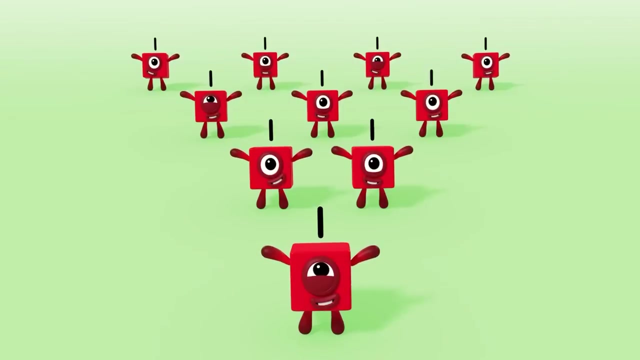 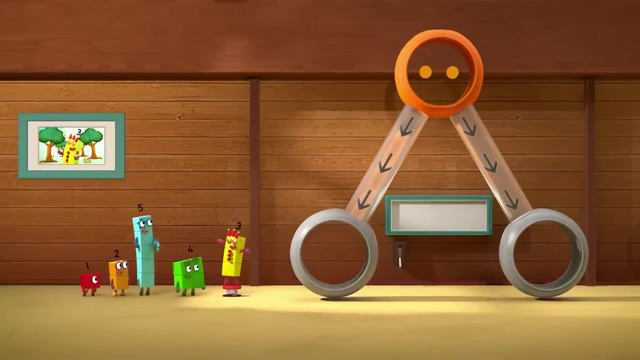 Making friends is our idea of fun. One, two, three, four, five, six, seven, eight, nine, ten. Remember this forever. You can do what we've just done. You can make any number and keep on adding one. That was fun. Yay, Welcome, welcome, welcome. 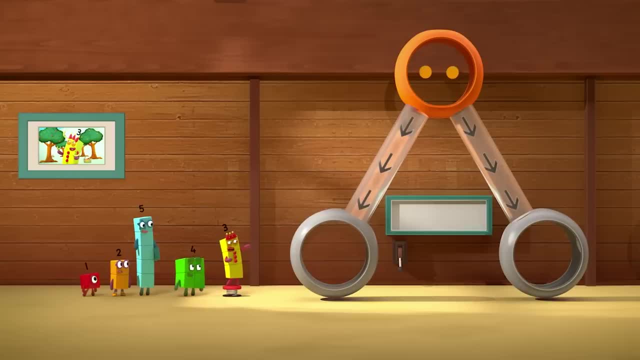 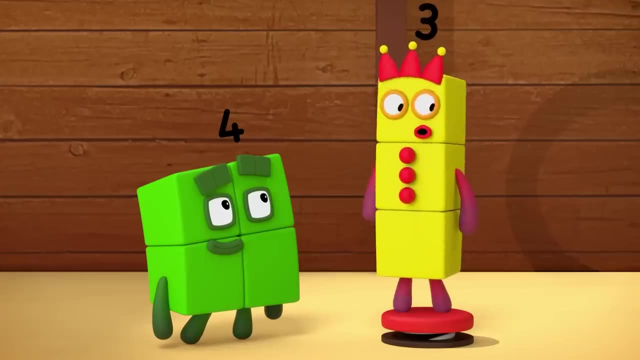 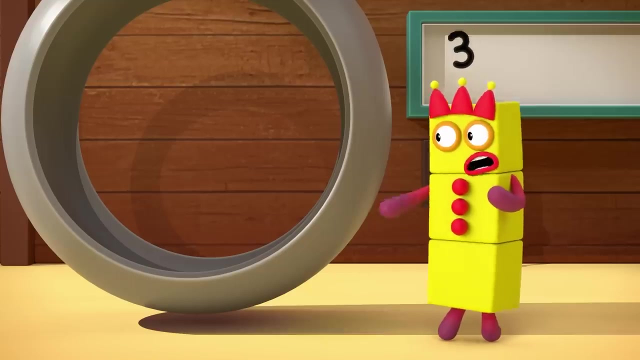 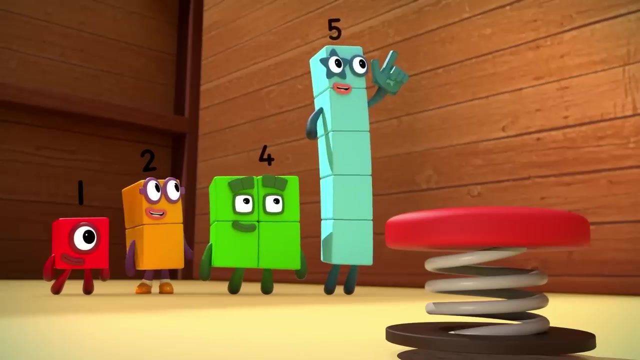 to my fantastic Fun Fruit Factory, where we serve up fresh fruit all day. Wow, How do they work? Oh, easy peasy. lemon squeezy, Obviously. just Silly thing's broken. There are two oranges in there. Maybe if two tries it. 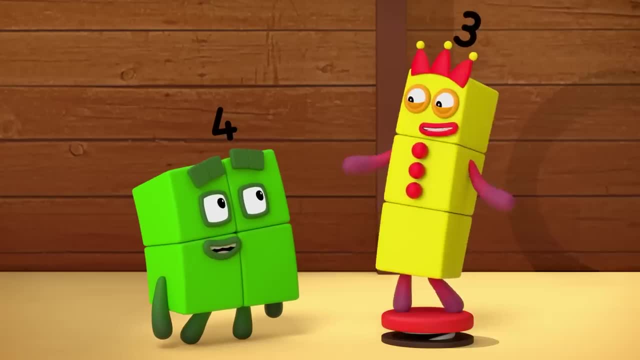 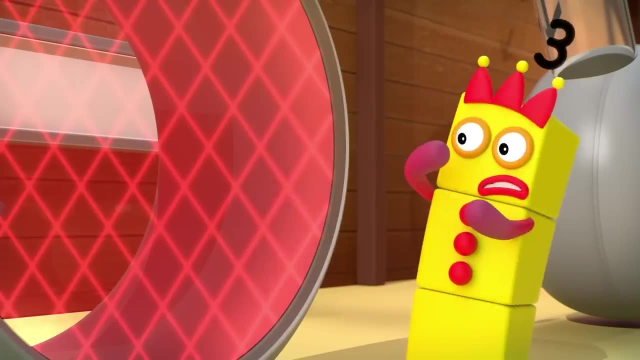 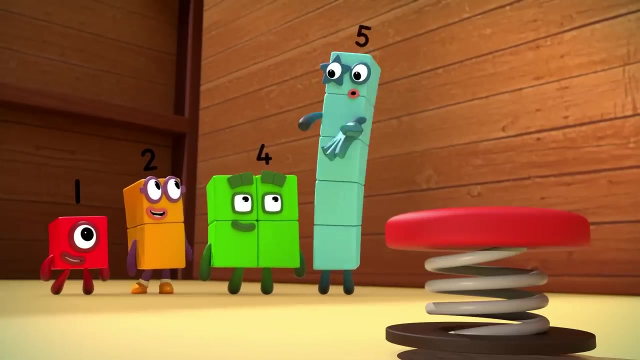 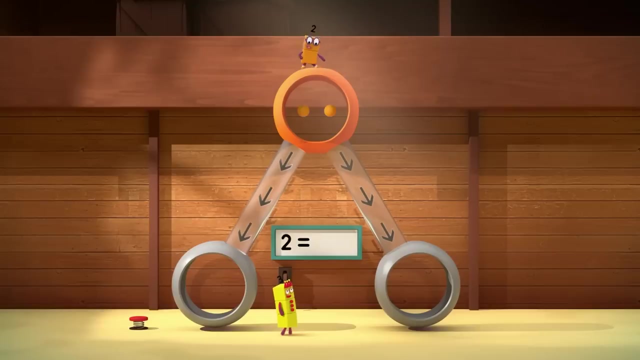 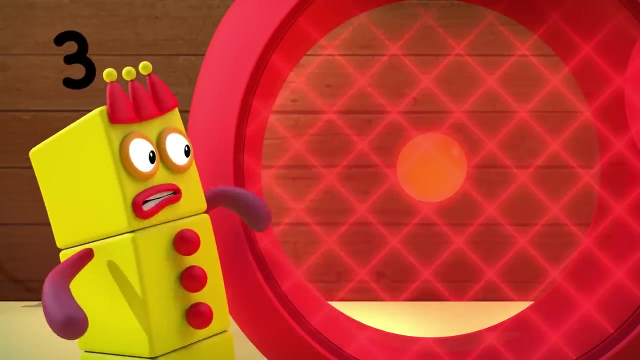 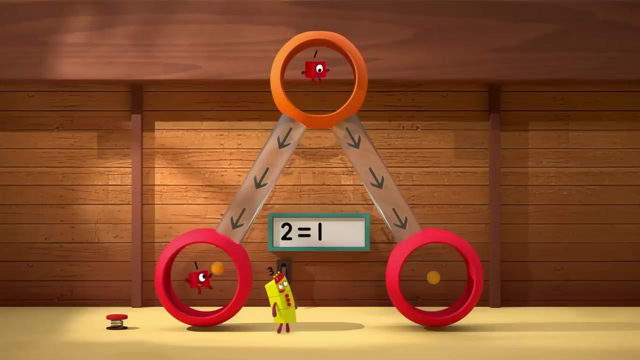 Oh, easy peasy, lemon squeezy. Obviously I just Silly thing's broken. There are two oranges in there. Maybe, if two tries it Two equals one, One plus one. How do I? Two equals one plus one. 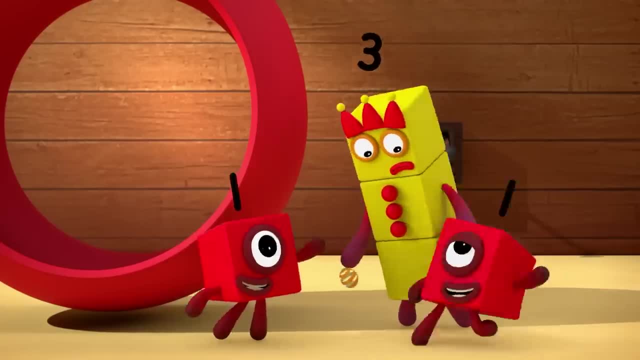 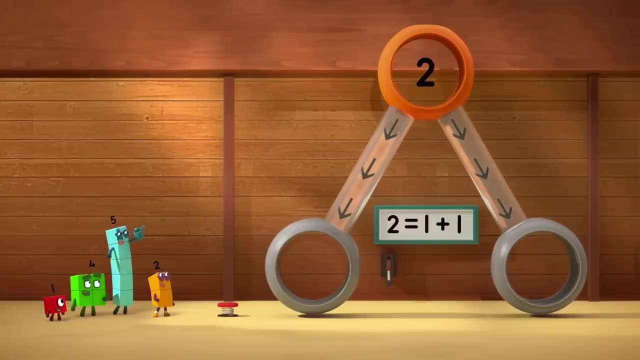 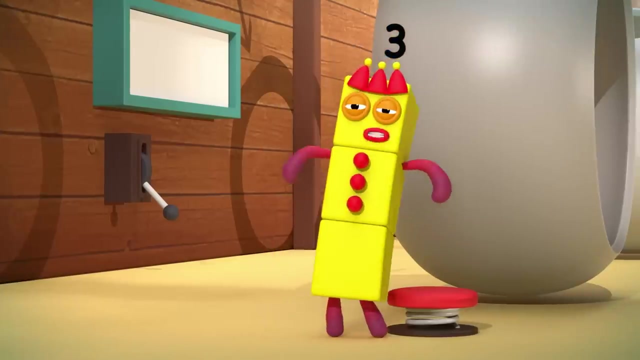 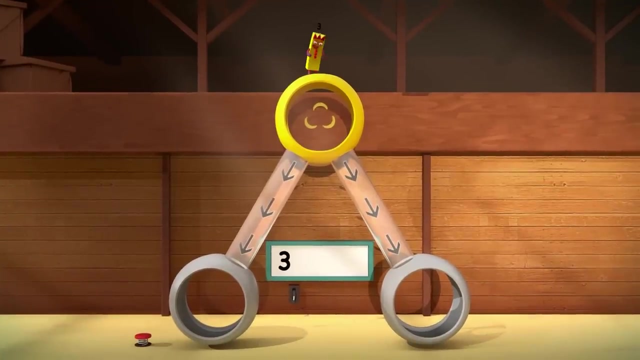 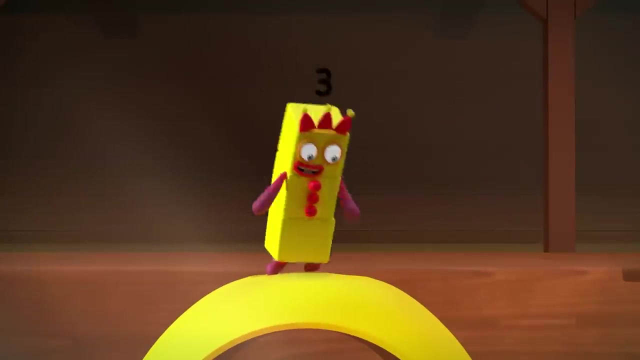 Yum, Ta-da. Oh. look. Two at the top splits in to one and one stacked on top. Ahem, I want fruit. It's my turn. Three equals one plus two. Yummy, yummy, yummy. Three equals one plus two. 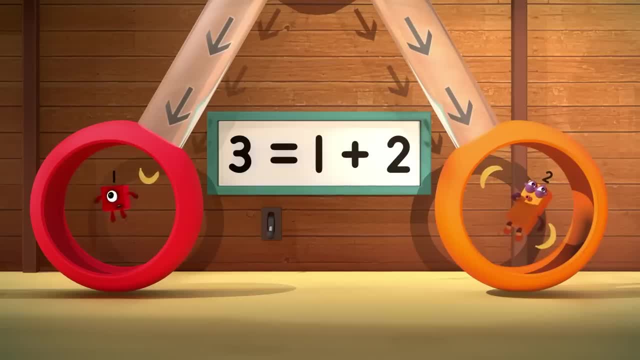 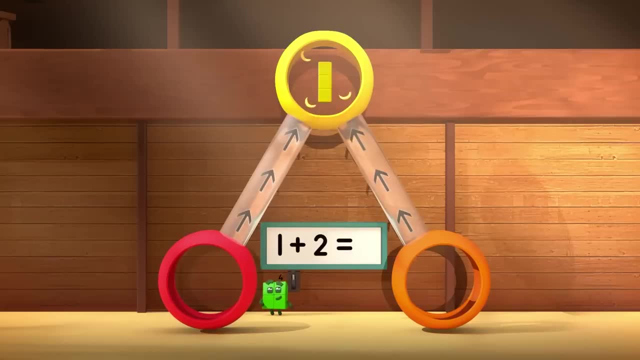 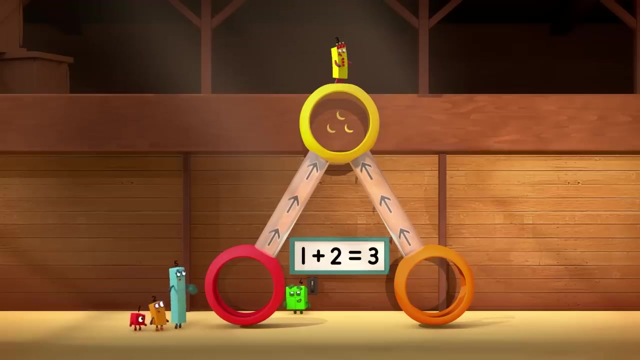 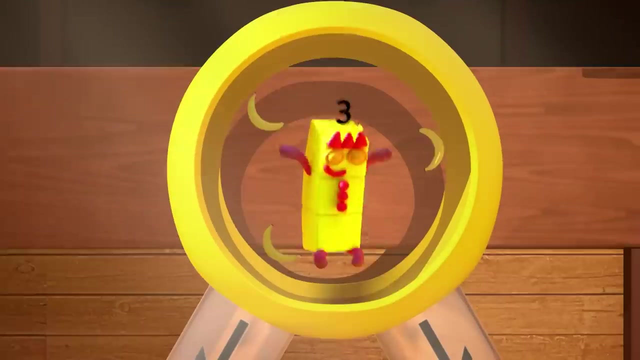 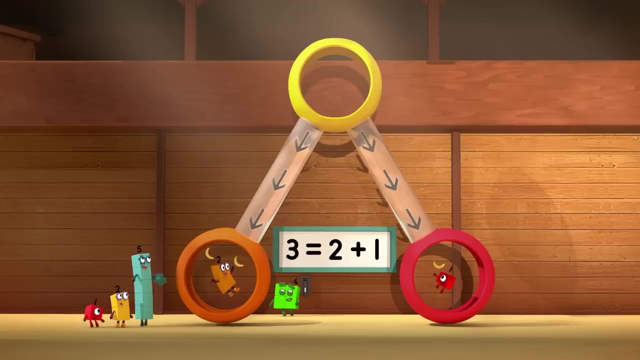 Oh, Where's three? Let's try this lever: One plus two equals three. Oh, it works both ways. Oh Hey, those are mine. Three equals two plus one. Now there's three. There's two over here and one over there. 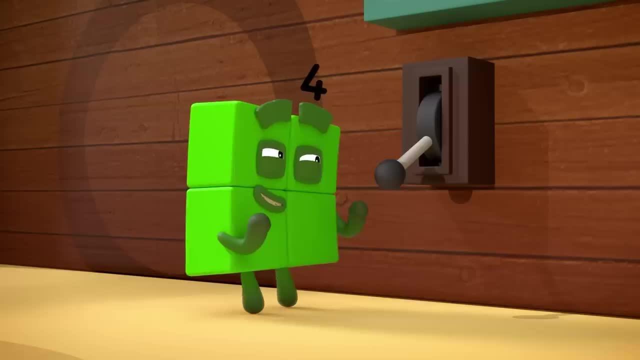 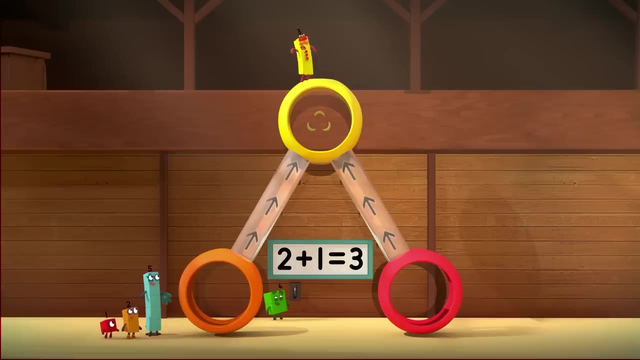 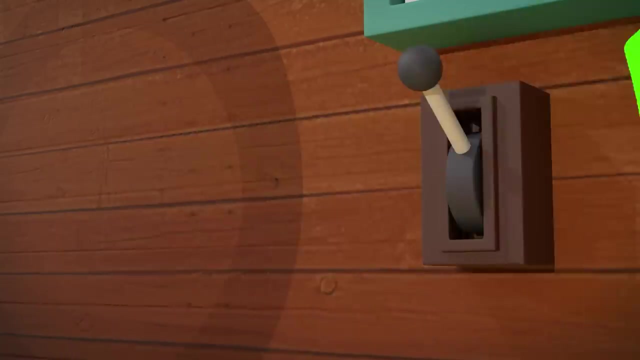 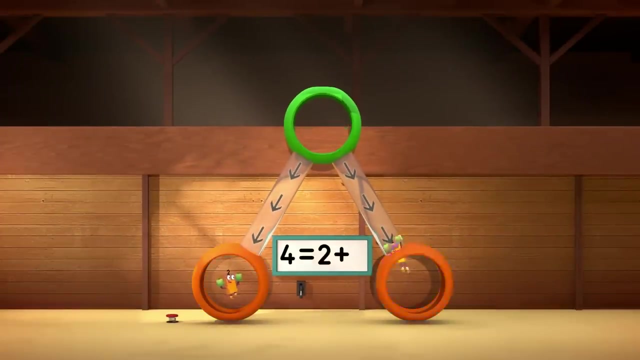 But three doesn't get her bananas again. Two plus one equals three. Hey, I'm still hungry. Look, apples, Square apples. Four equals two plus two. Yum, yum, Yum, yum, Yum, yum. No, no, no, you silly machines. 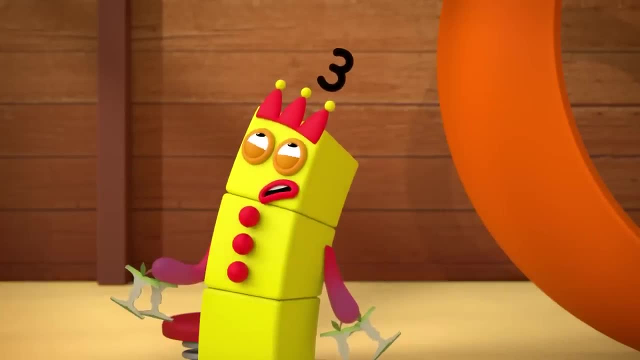 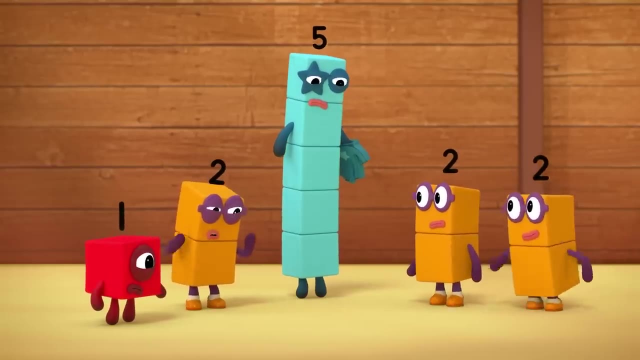 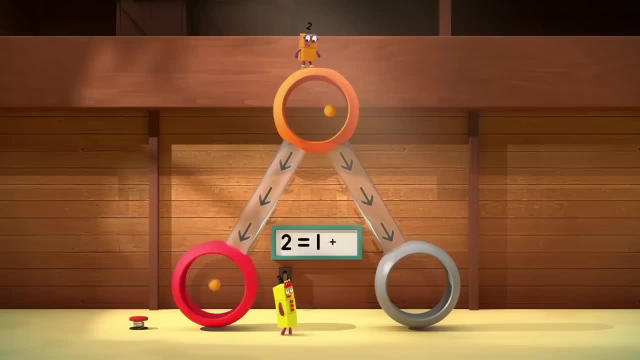 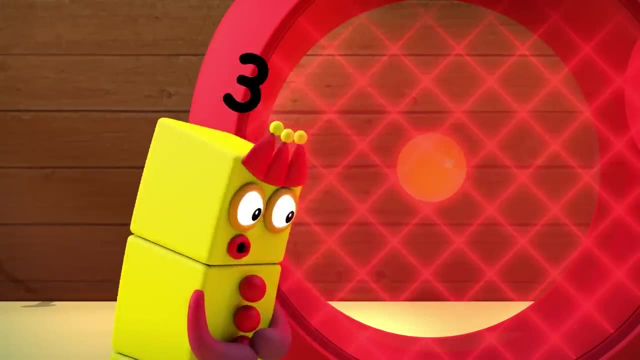 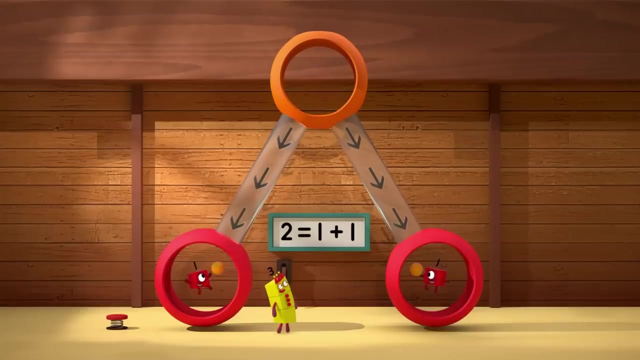 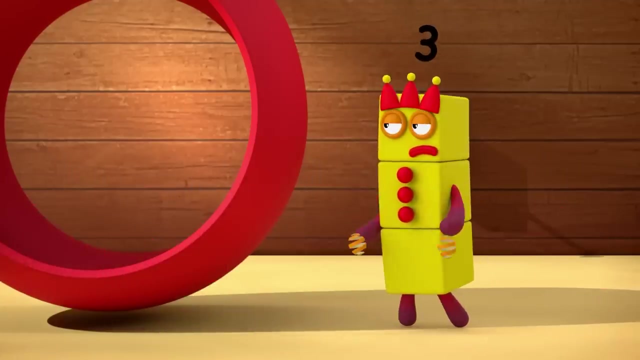 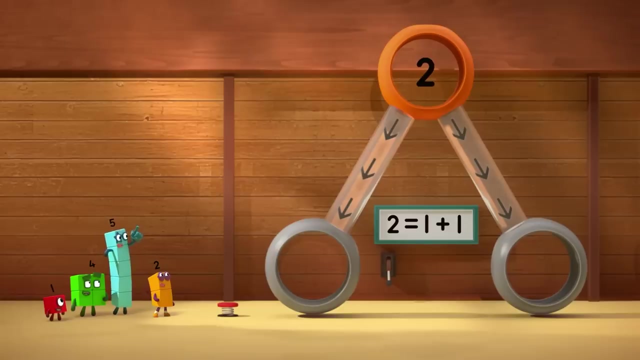 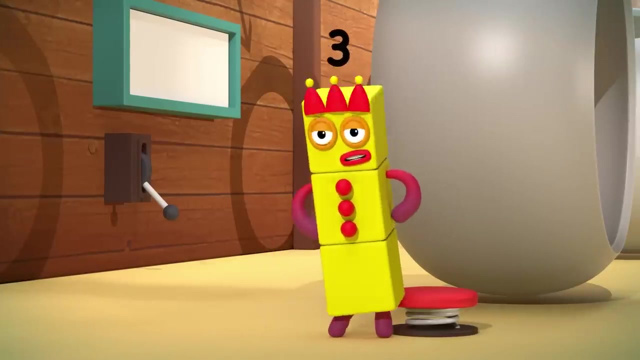 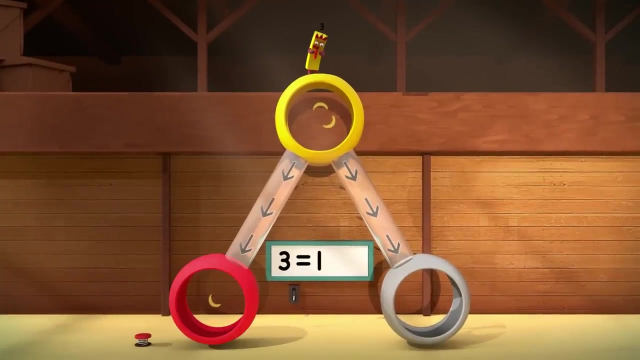 Two equals one plus one. How do I? Two equals one plus one, Yum Ta-da, Look. Two at the top splits into one and one at the bottom. I want fruit. It's my turn. Three equals one plus two. 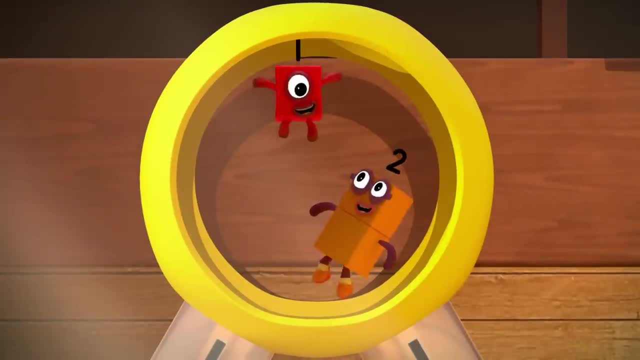 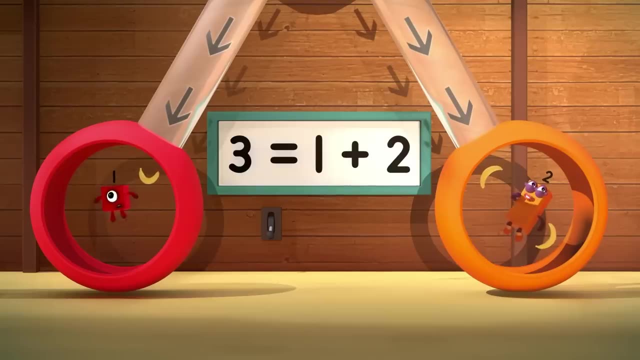 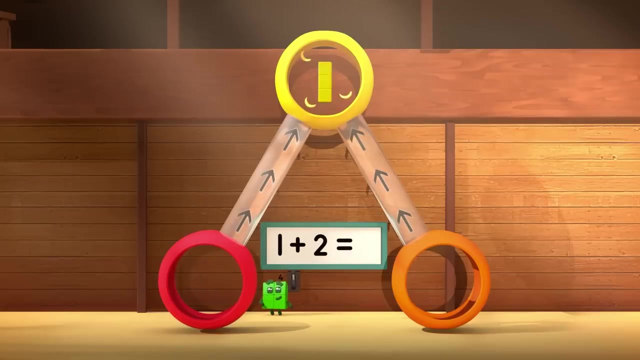 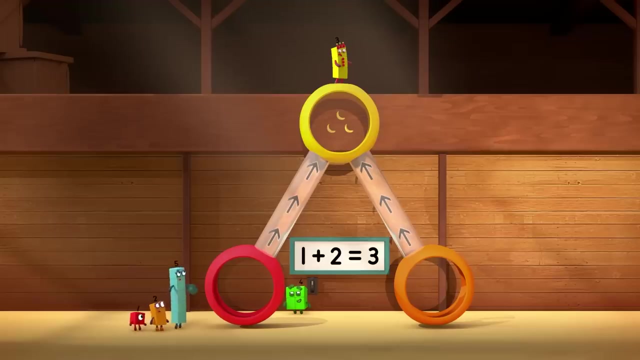 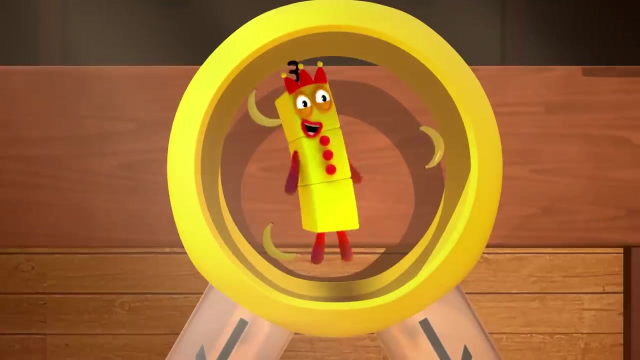 Yummy, yummy, yummy. Three equals one plus two. Oh, Where's three? Let's try this lever: One plus two equals three. Oh Oh, It works both ways. Oh Hey, Those are mine. Three equals two plus. 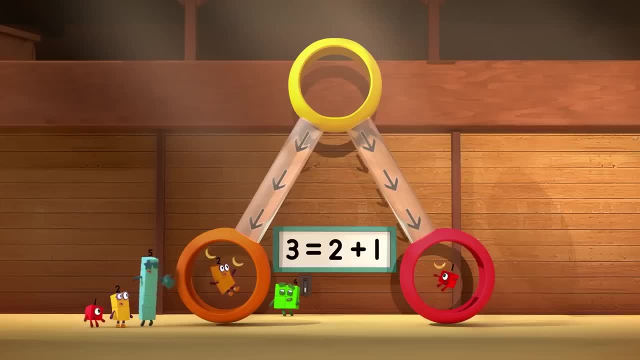 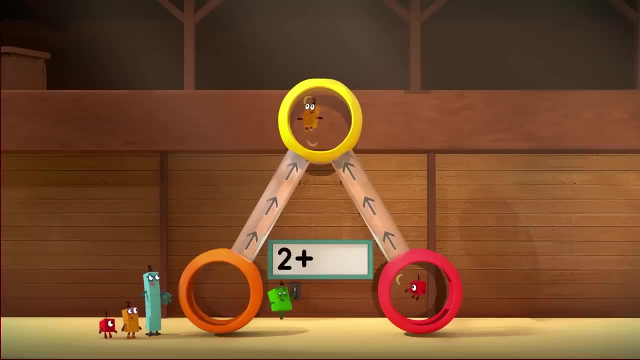 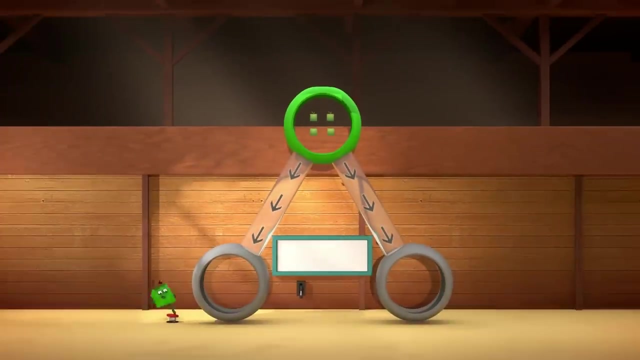 one Now, there's two over here and one over there, But three doesn't get her bananas again. Two equals plus one equals three. Hey, I'm still hungry. Oh Look, Apples, Square, apples, Huh. Four equals. 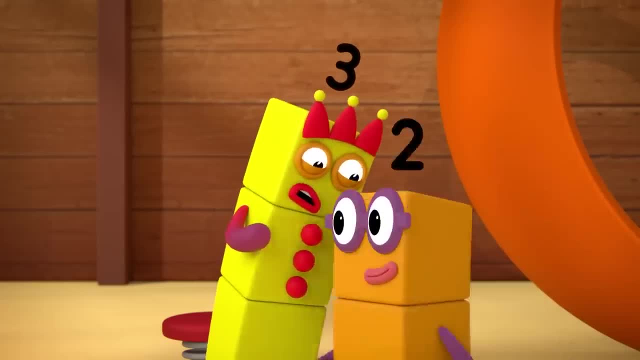 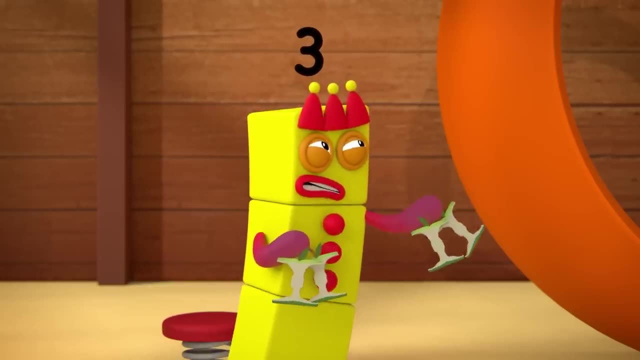 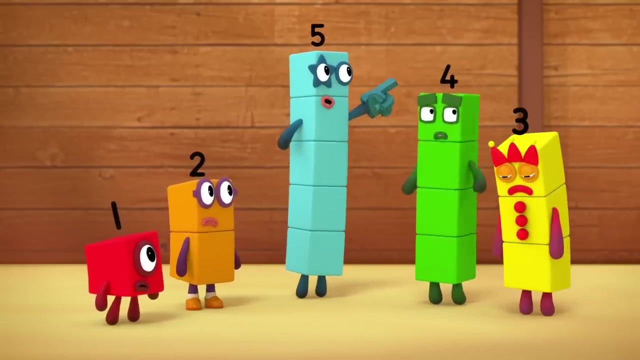 two plus two, Yum yum, Huh, Yum yum. Oh no, you silly machines, Poor three. We need to find a way to make three apples come out. Look, Four new apples are the top. I know how to make three. 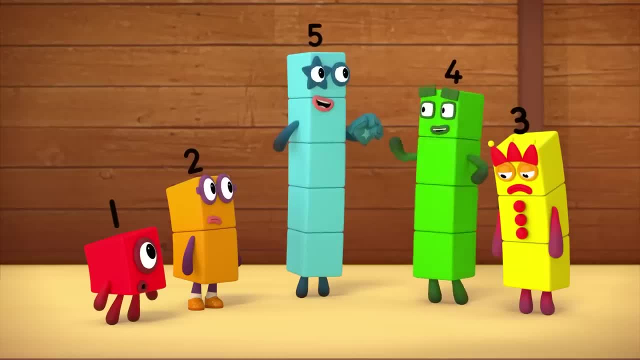 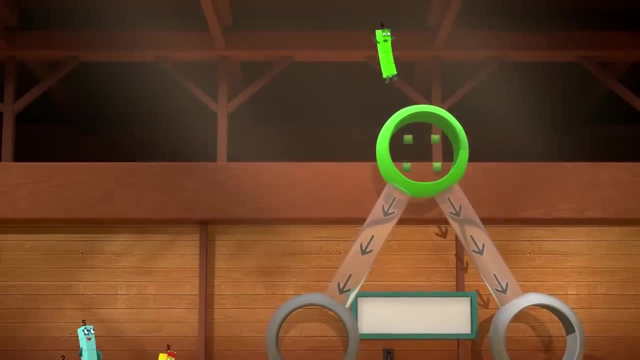 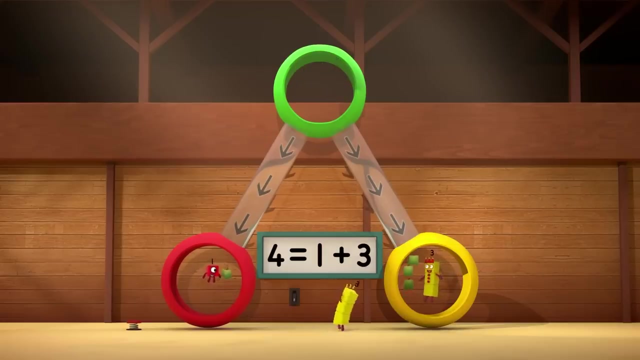 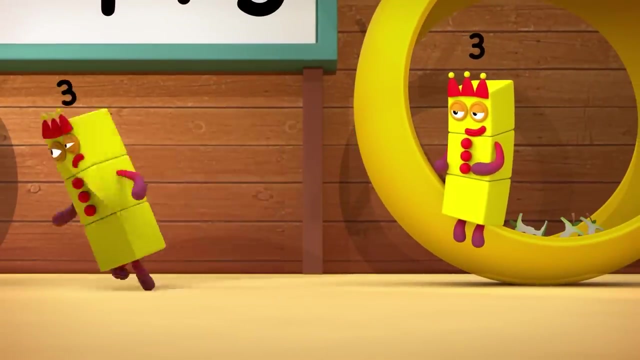 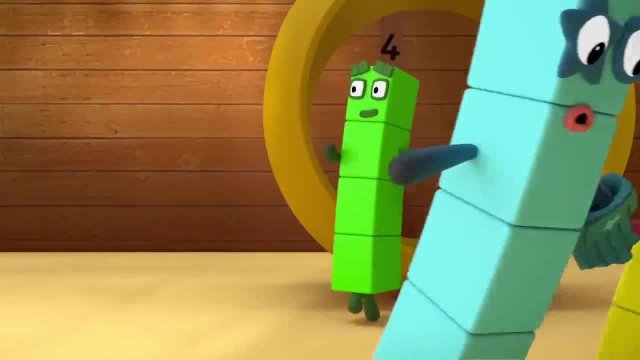 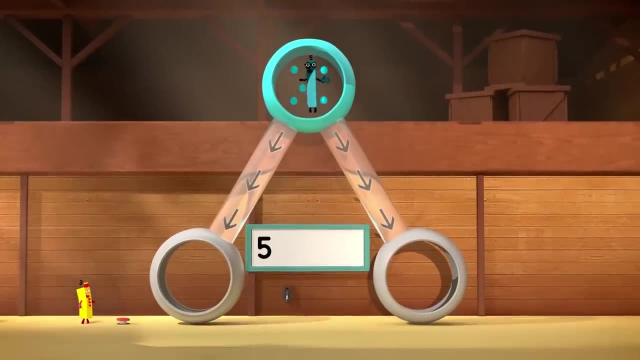 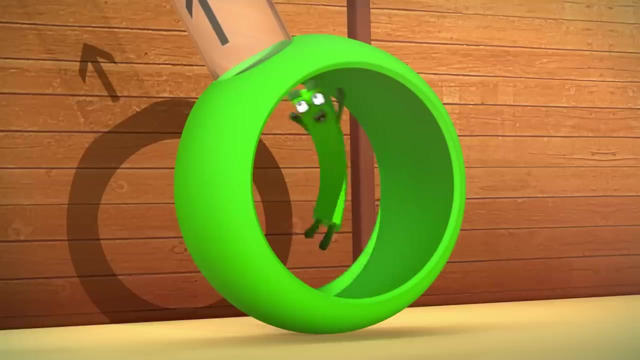 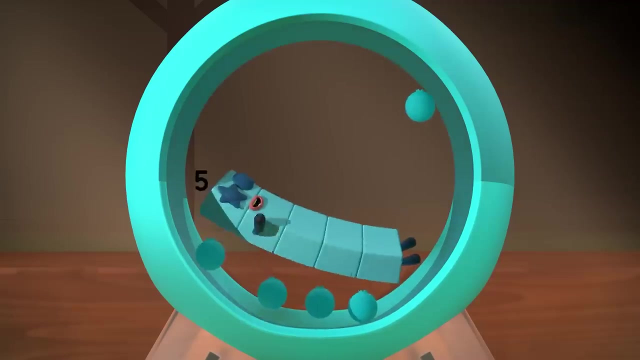 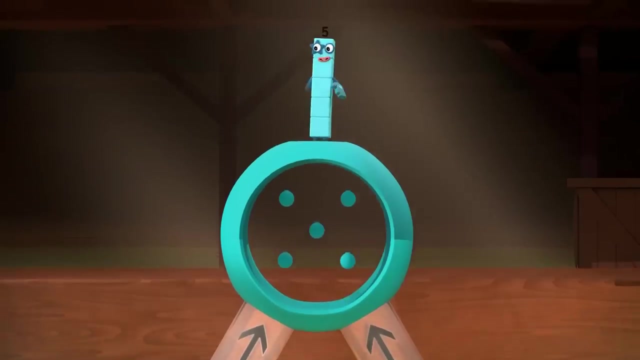 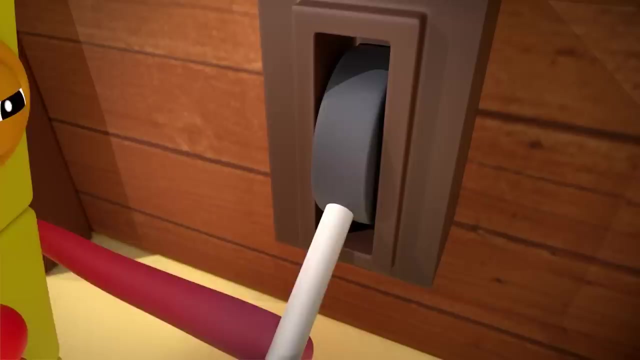 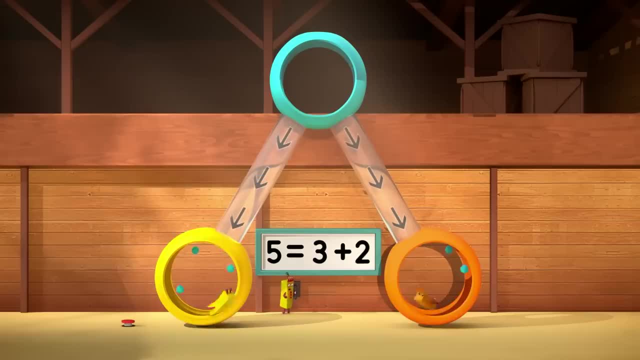 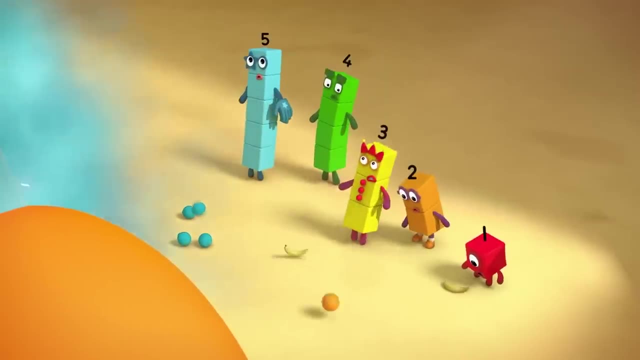 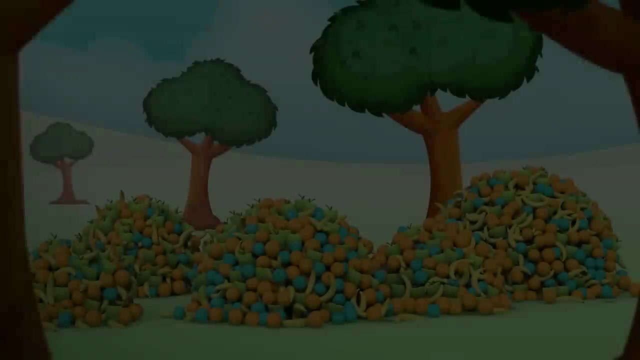 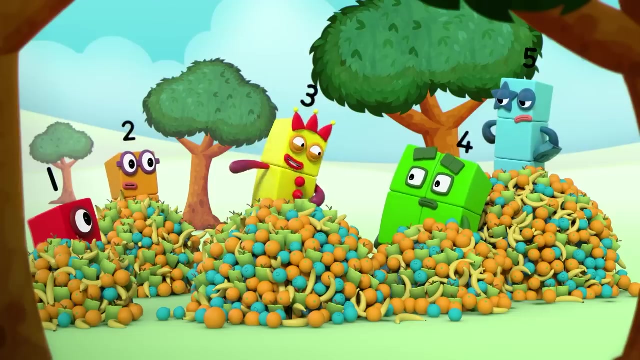 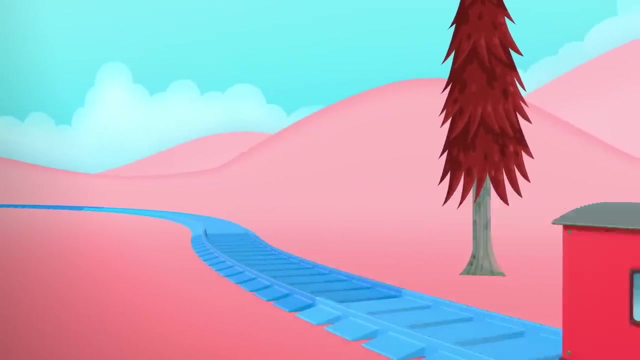 It's going far too fast. Five equals three plus four. One, two, three, Three bloopers. I told you Easy peasy, lemon squeezy. I am five, I feel alive Whenever I can drive my train. Only five, no more, no less. 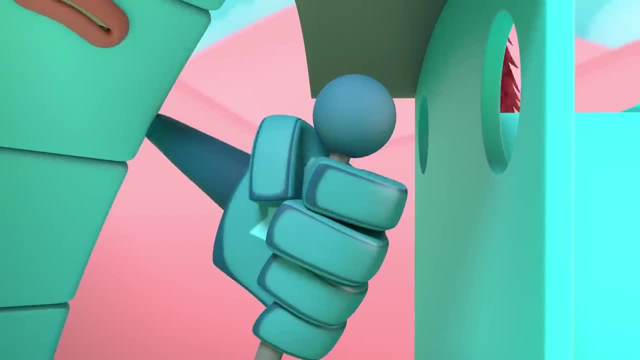 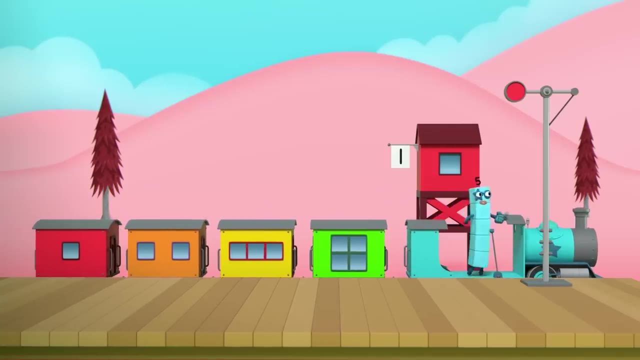 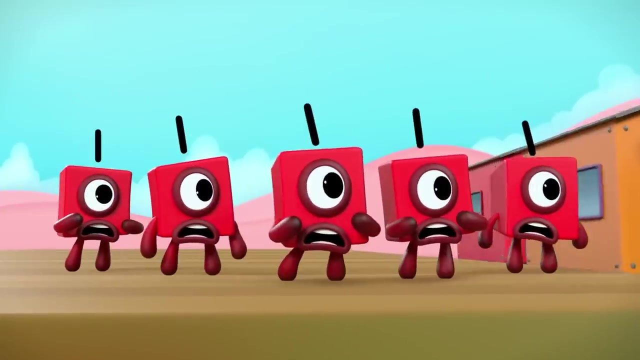 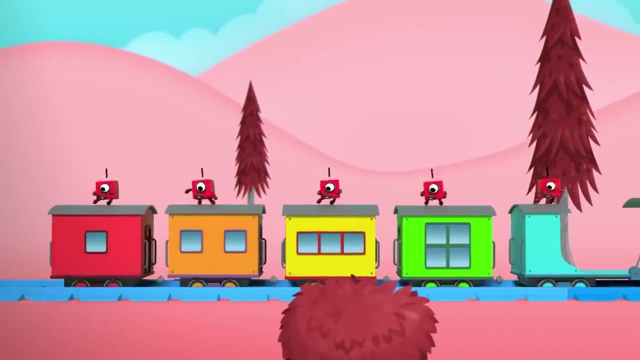 Can drive. the number block six break. Woo-hoo, No one getting on the train. Let's be on our way again. Woo-hoo, We have to get the train to stop. So hop, hop, hop, hop, hop on top. Only five can stop the train. 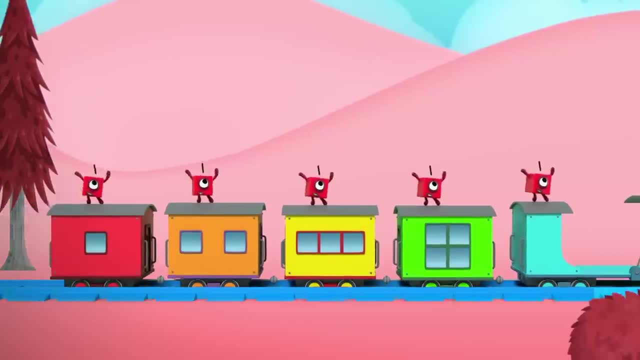 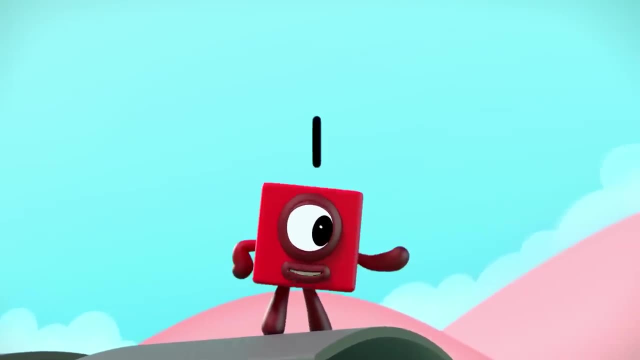 So how do we make five again? Only five, no more, no less. Can stop the number blocks express Woo-hoo. I think I know what must be done. Let's stop the train by adding one. One plus one equals two. Two plus one equals three. 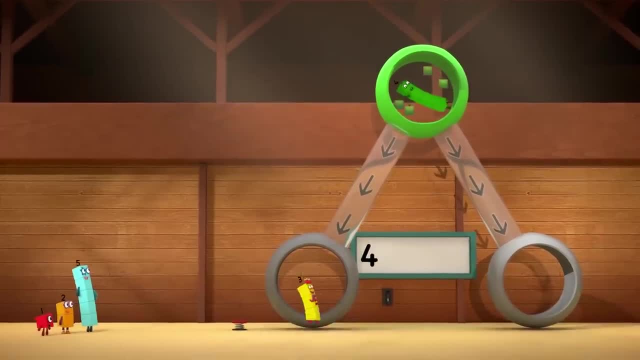 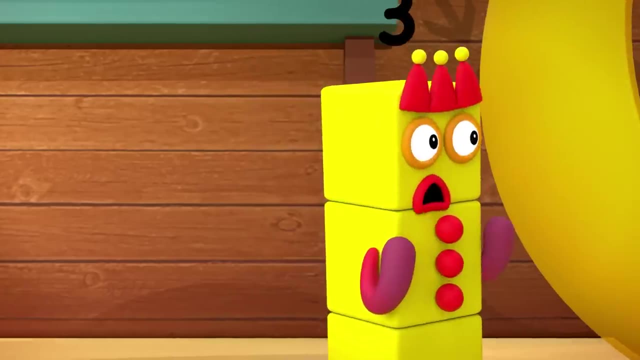 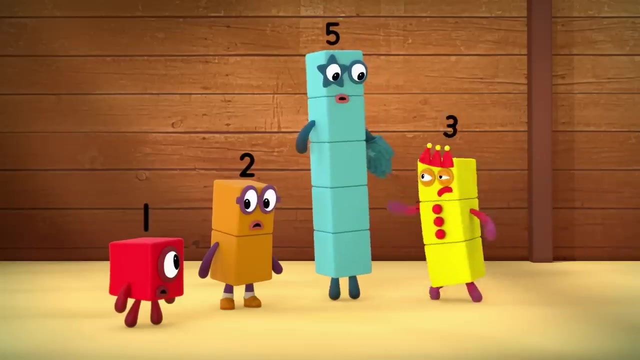 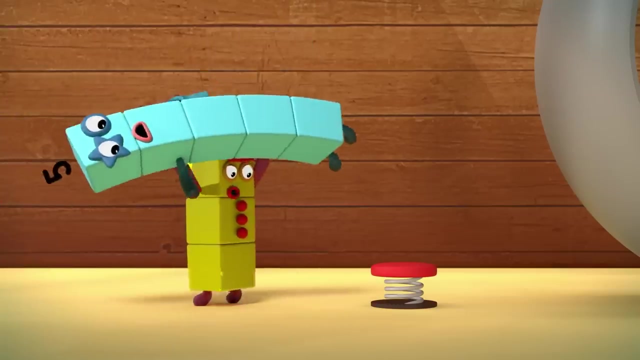 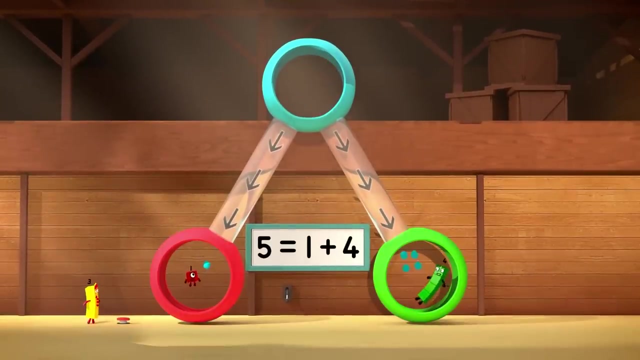 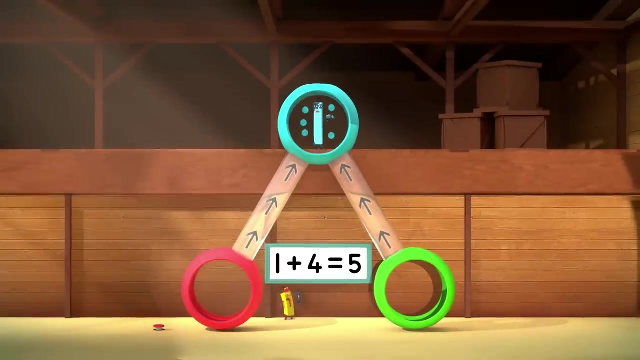 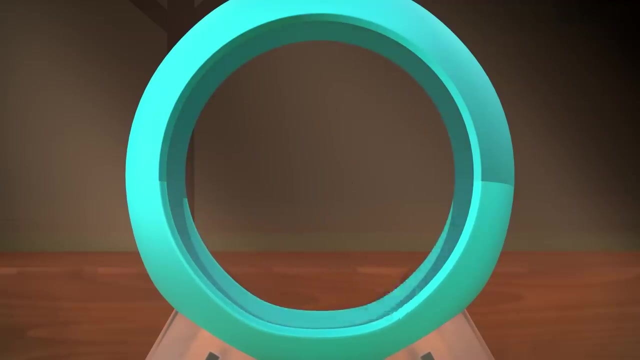 Here I go. Ah, Four equals one plus three. Yes, Yes, Yes, No, no, no, I won't write: Five equals one plus two. One plus four equals five, Two equals five. Yikes, Five equals four plus one. 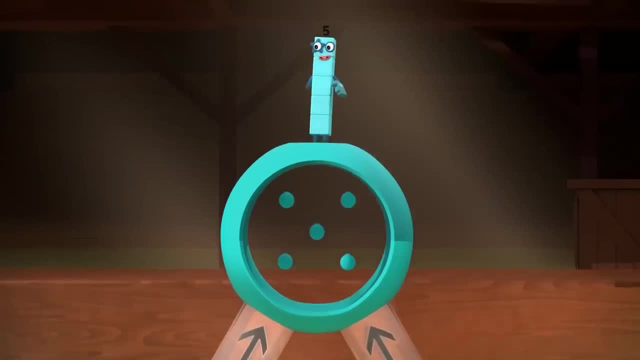 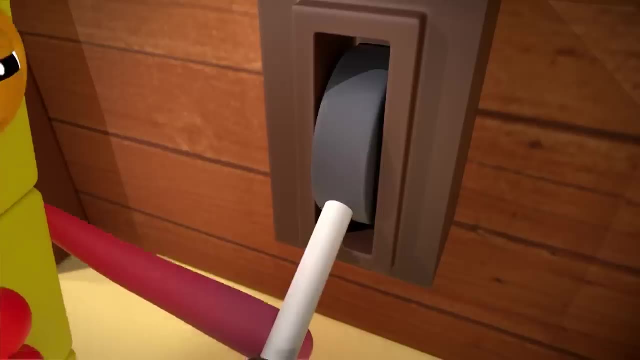 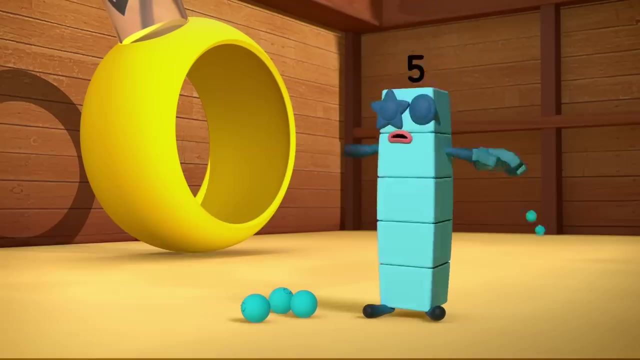 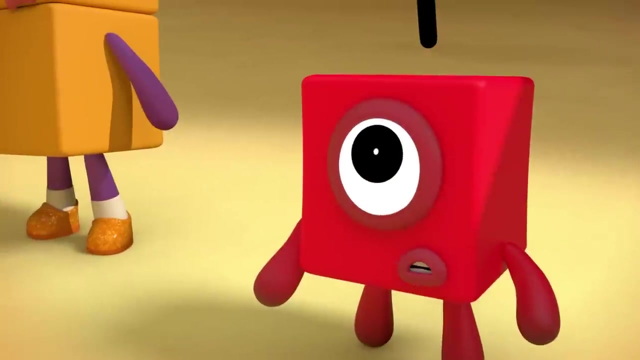 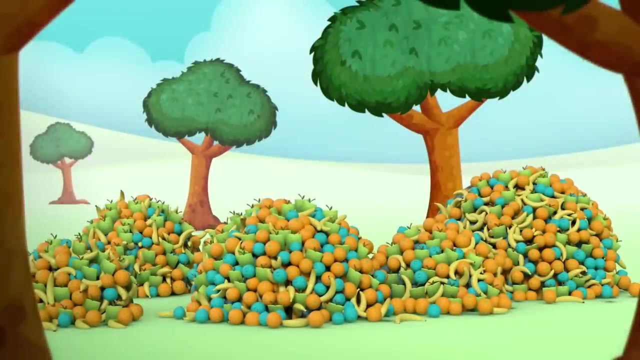 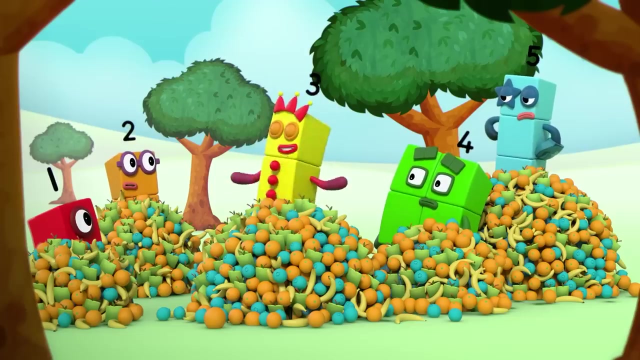 Four plus one equals five. Five equals two plus three. Two plus three equals five. It's going far too fast. Five equals three, One, two, three. Bluebird Run. I told you Easy peasy, lemon squeezy. 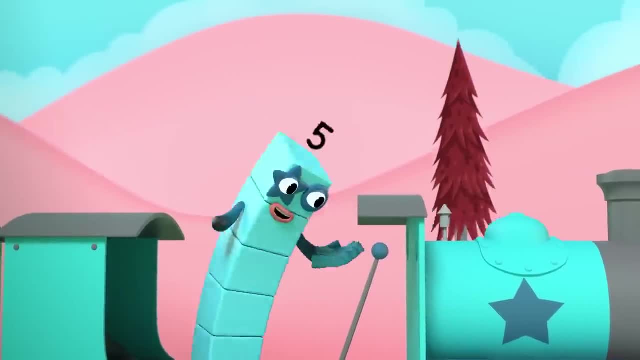 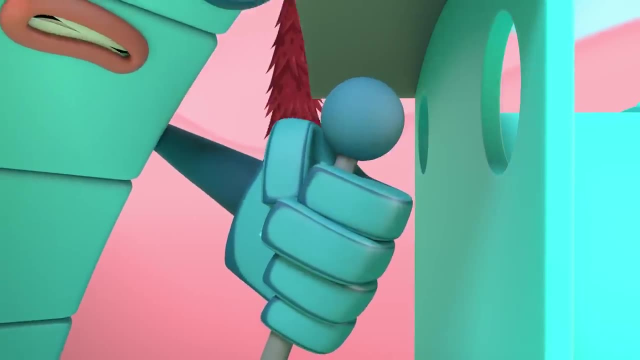 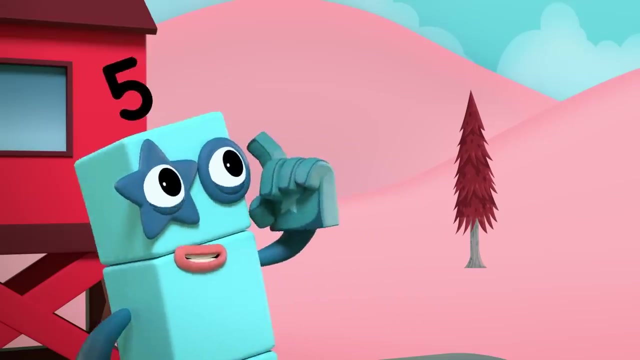 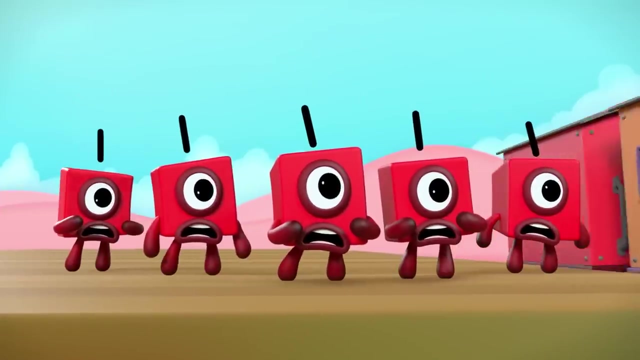 I am five, I feel alive Whenever I can drive my train. Only five, no more, no less, Can drive the number black, six brick. Woohoo, No one getting on the train. Let's be on our way again. Woohoo, We have to get the train to stop. 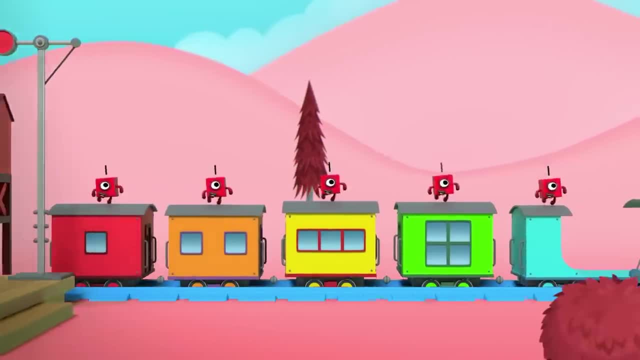 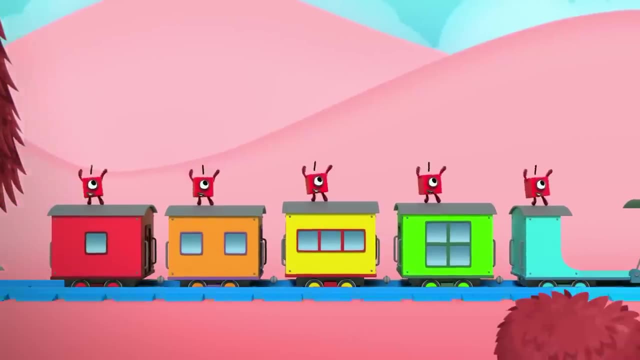 So hop, hop, hop, hop, hop on top. Only five can stop the train. So how do we make five again? Only five, no more, no less, Can stop the number blocks express. Woohoo, I think I know what must be done. 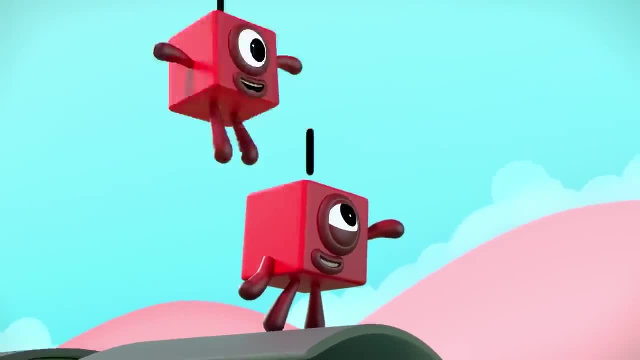 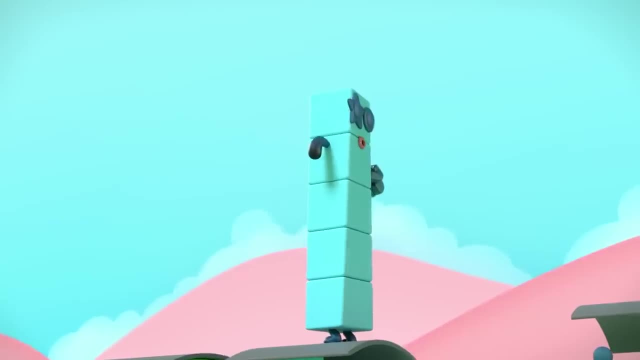 Let's stop the train by adding one. One plus one equals two. Two plus one equals three. Three plus one equals four. Four plus one equals five. Only five can stop the train, And I am back to five again. Five minus one equals four. Four minus one equals three. 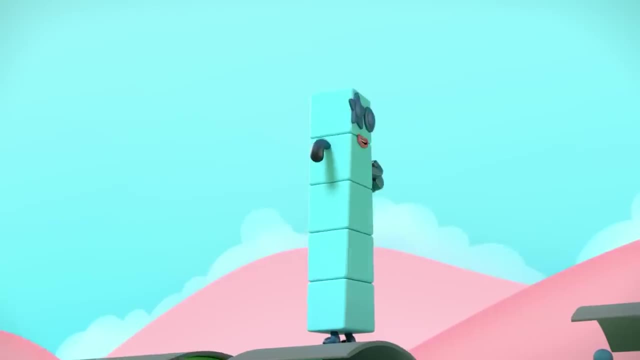 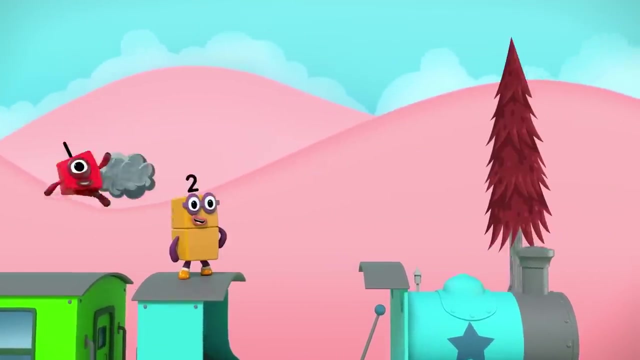 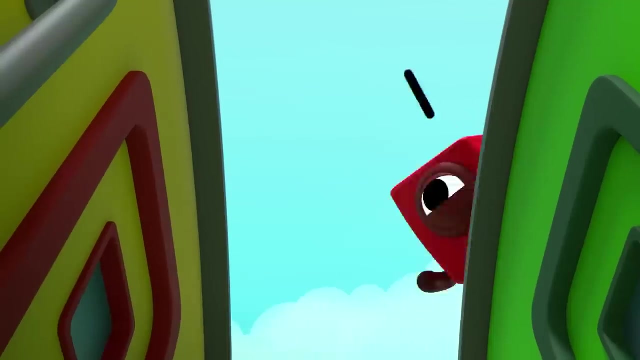 Three plus one equals four. Four plus one equals five. Only five can stop the train, And I am back to five again. Woo-hoo. Five minus five, One equals four. Four minus one equals three. Three minus one equals two. Two minus one equals one. Can you help us pretty please? 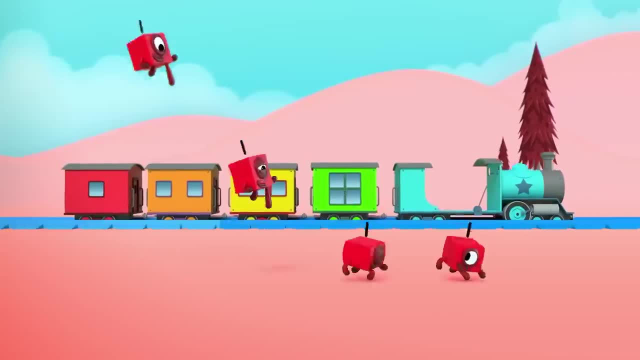 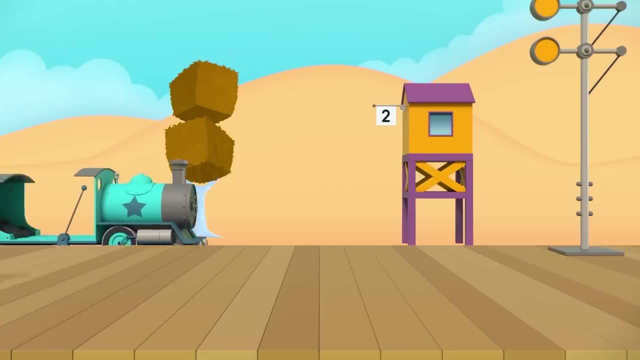 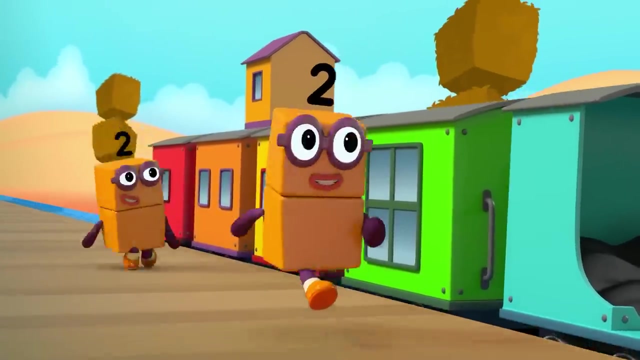 We need to get back on the way. Only five can stop the train. So how do we make five again? Only five, no more, no less, Can stop the number blocks express Woo-hoo. We know what we have to do: Stop the train by adding two. 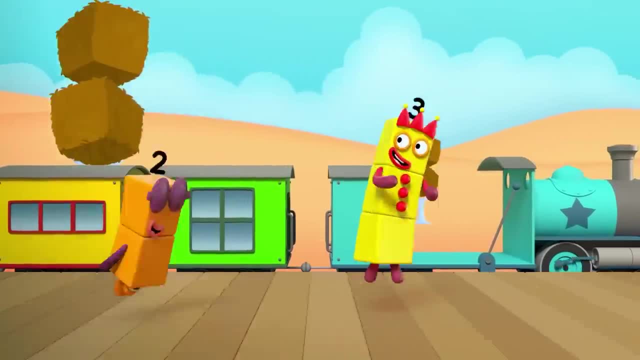 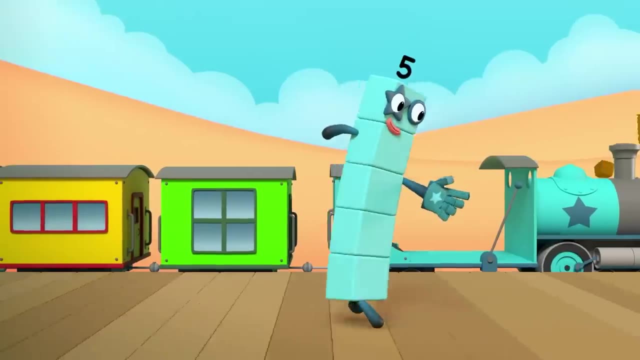 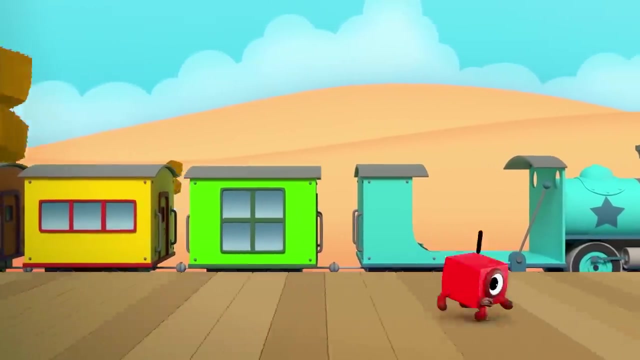 One plus two equals three. Three plus two equals five. Only I can stop the train, So I am back to try again. Five minus two equals three. Three minus two equals one. Ouch Ow, Come on twos Time to act like kangaroos. Hop, hop, hop, hop. 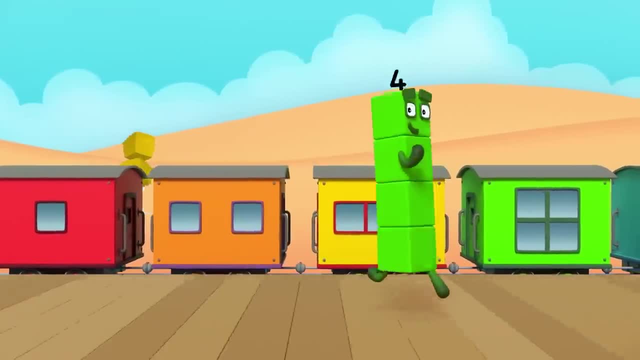 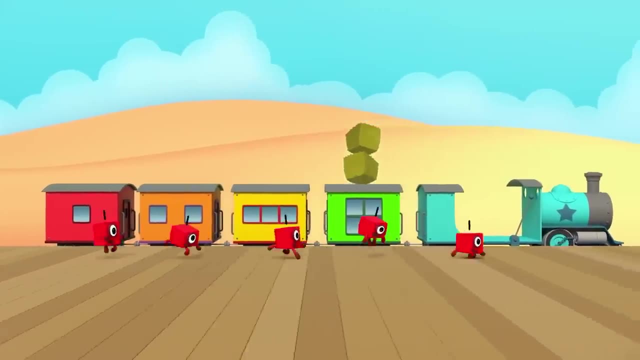 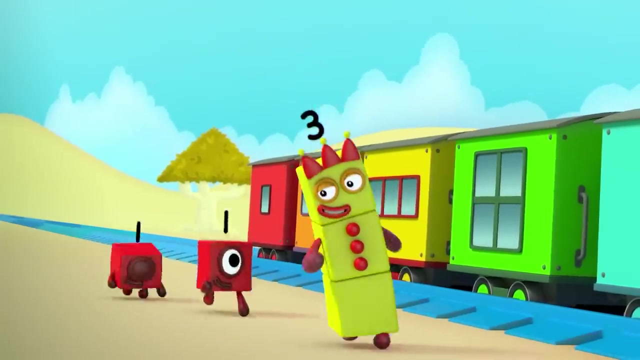 Two plus one equals three. Six plus one. extended. Can we do this again? Three plus two equals four. Six plus two equals four. Five plus two equals three. Three plus one equals three. Four plus one equals three. Hotって, One plus two equals four. Five plus two equals two. 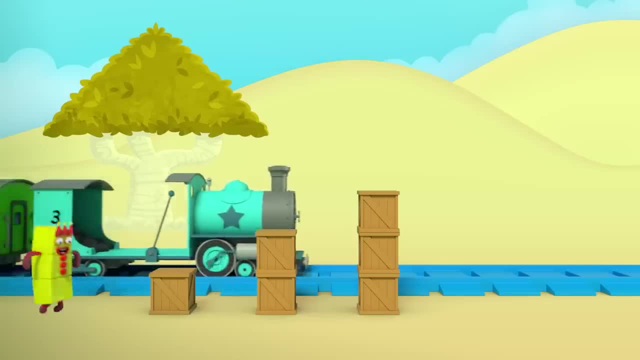 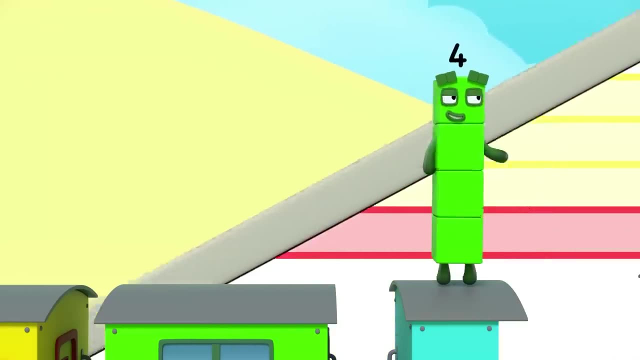 Only five can start the train. So how do we make five again? OK, friends, leave this to me. I'll stop the train by adding three: Hop, hop, hop And hop. One plus four equals three. What does that mean? I'm not quite sure. I don't think I've seen that before. 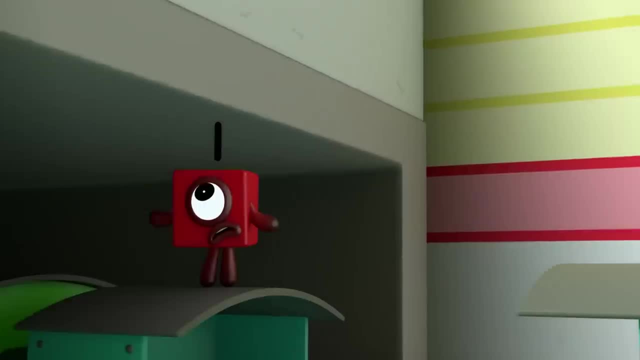 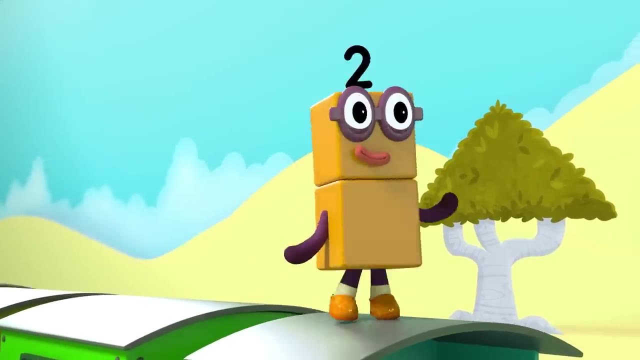 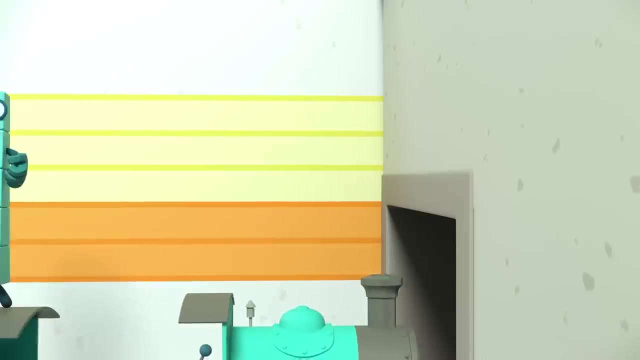 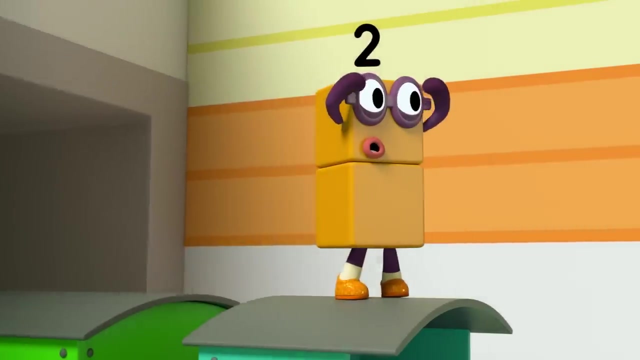 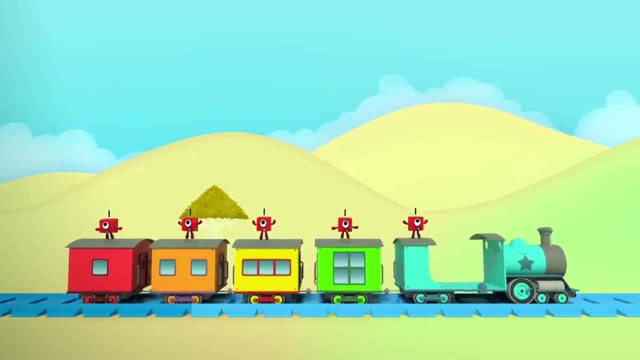 Minus three Equals one, Hey, Two plus three equals five. Only I can start the tree. and I am back to five. Minus three Equals two. Hey, Only five can stop the train. so how do we make five a game? 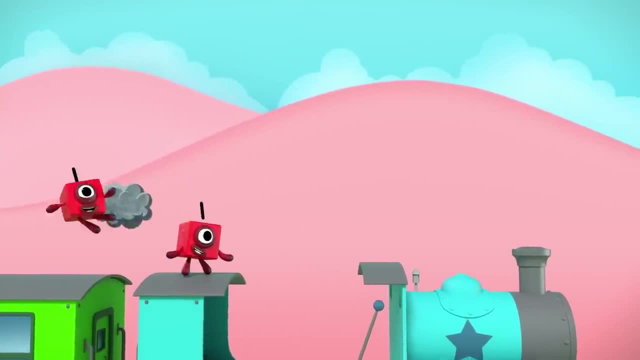 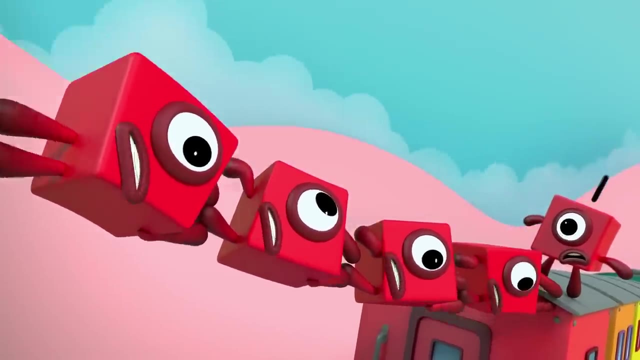 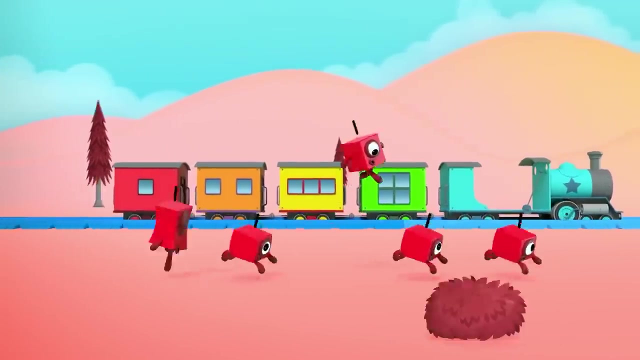 Three minus one equals two. Two minus one equals one. Can you help us, pretty please? We need to get back on the way. Only five can stop the train. So how do we make five again? Only five, no more, no less, Can stop the number blocks express. 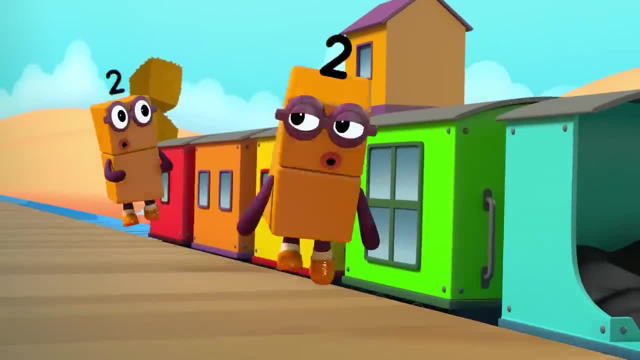 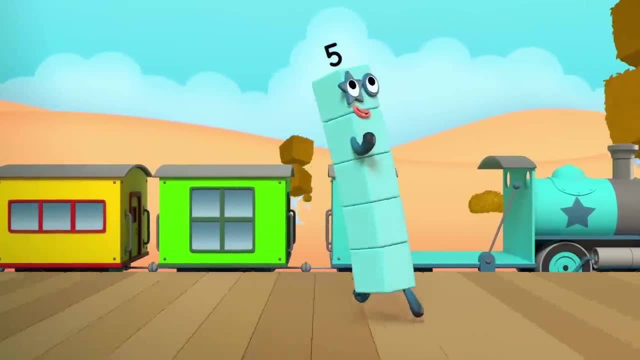 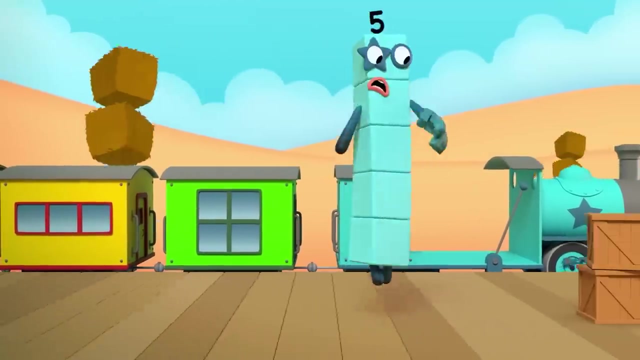 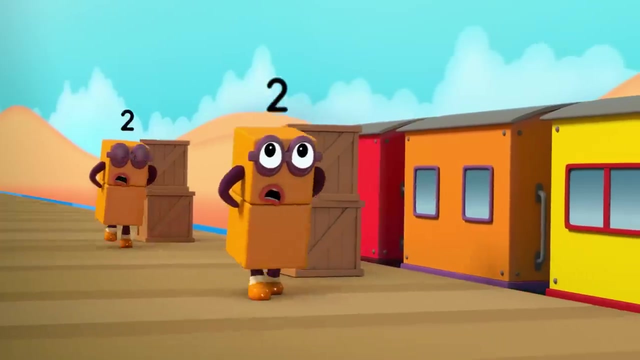 Woohoo, We know what we have to do: Stop the train by adding two. One plus two equals three. Three plus two equals five. Only I can stop the train. So I am back to try again. Five minus two equals three. Three minus two equals one. Ouch ow, come on twos. 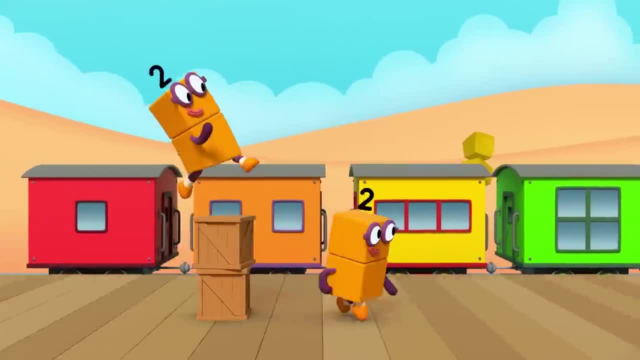 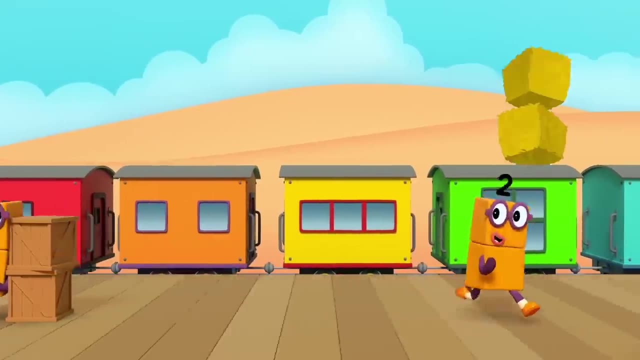 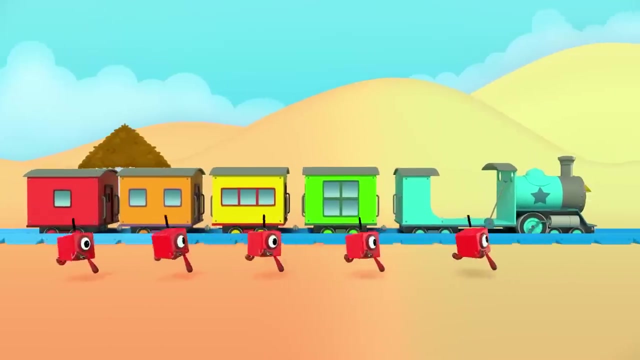 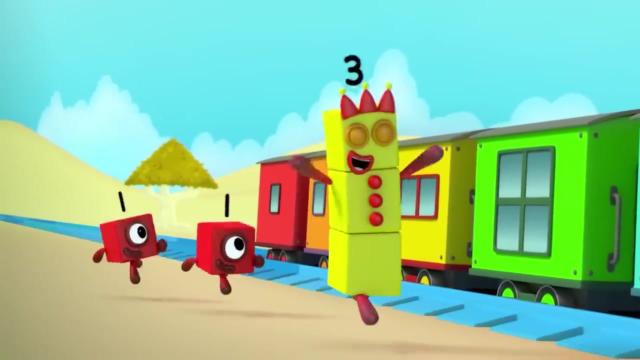 Time to act like kangaroos. Hop, hop, hop, hop, hop. Two plus two equals four. Four minus two equals two. Only five can stop the train. So how do we make five again? Okay, friends, leave this to me. I'll stop the train by adding three. 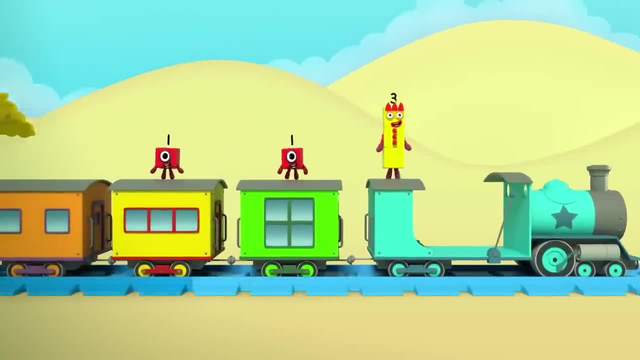 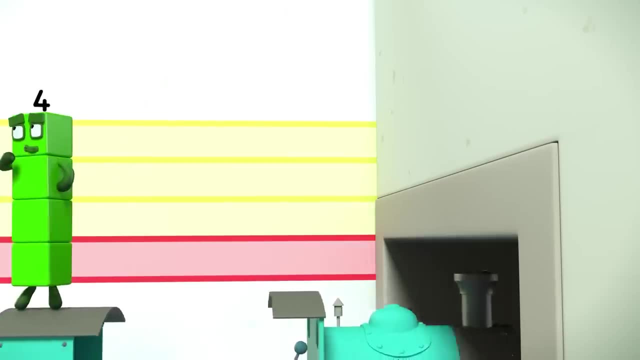 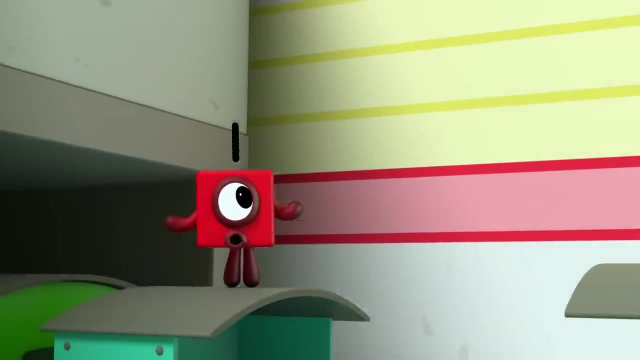 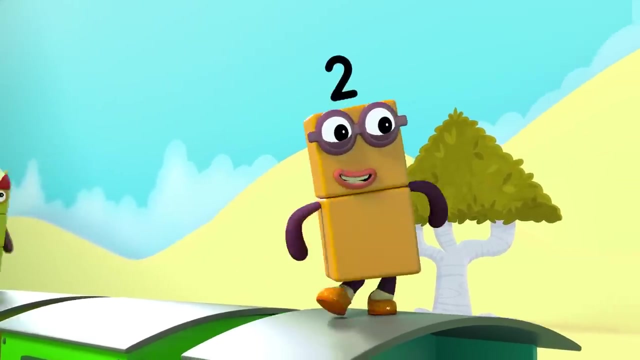 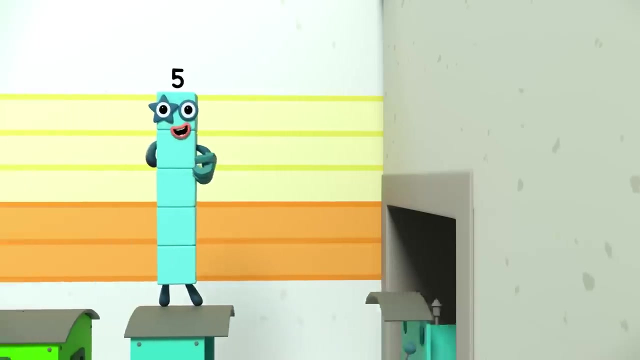 Hop, hop, hop, hop. One plus three equals four. What does that mean? I'm not quite sure. I didn't think. I've seen that before. At minus three Equals one. Hey, Two plus three equals Five. Only I can stop the train And I'm back to five. 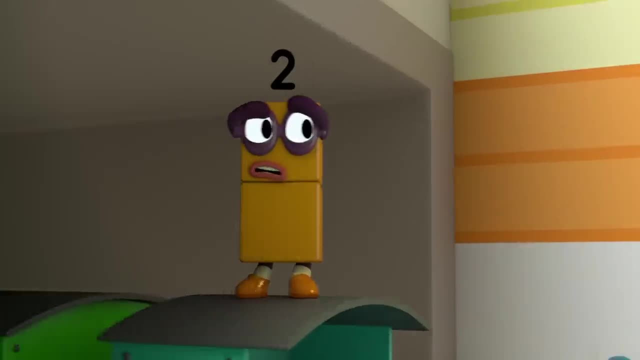 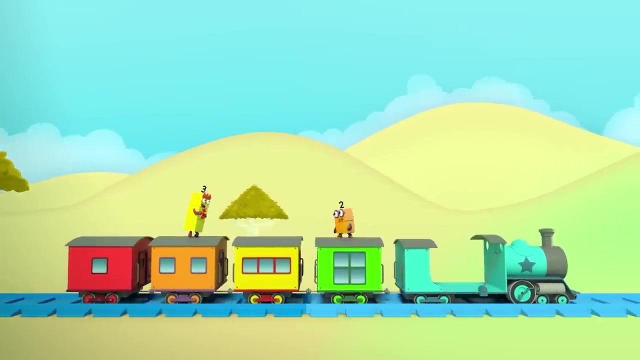 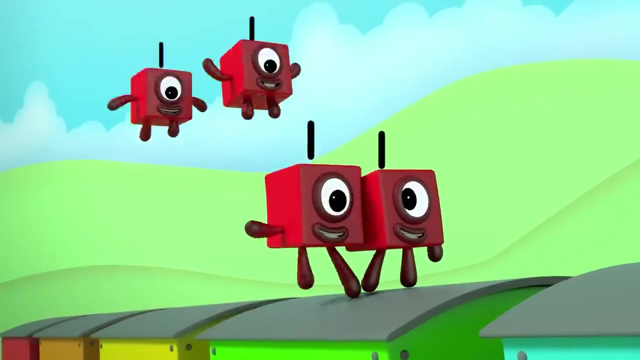 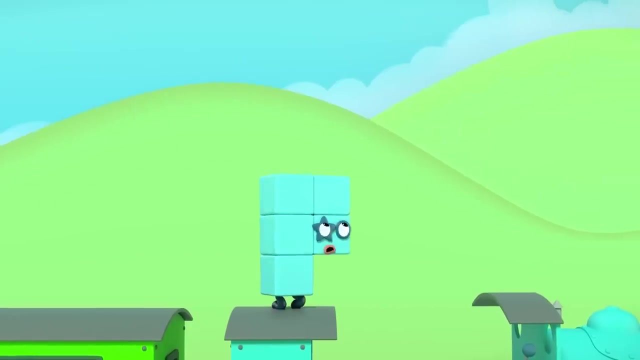 Minus three Equals two. Hey, Only five can stop the train. So how do we make five again? I am square, you be war. Let's stop the train by adding four. One plus four equals five. Only I can stop the train. So here I am to try again. 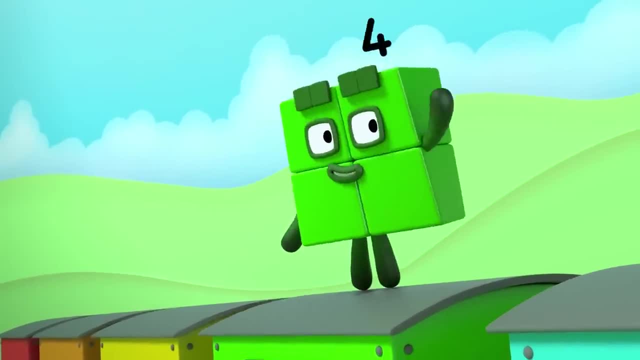 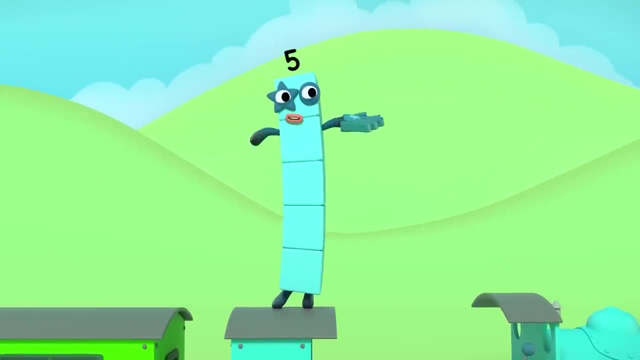 I am square, you be war. Let's stop the train by adding four. One plus four equals five. Only I can stop the train. so here I am to try again. Only five, no more, no less, can stop the number blocks express. 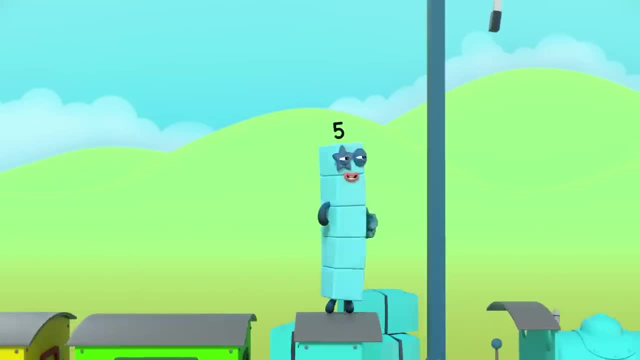 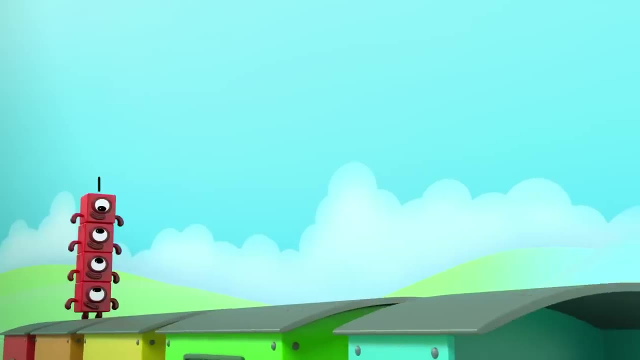 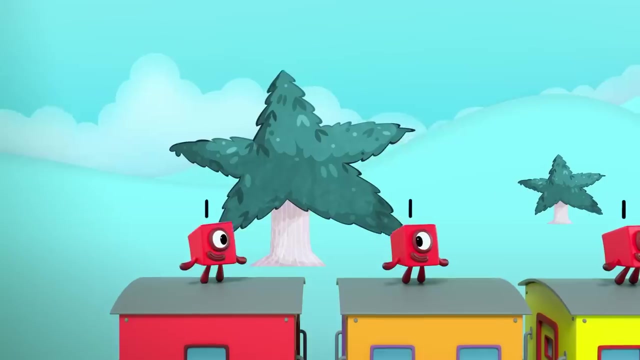 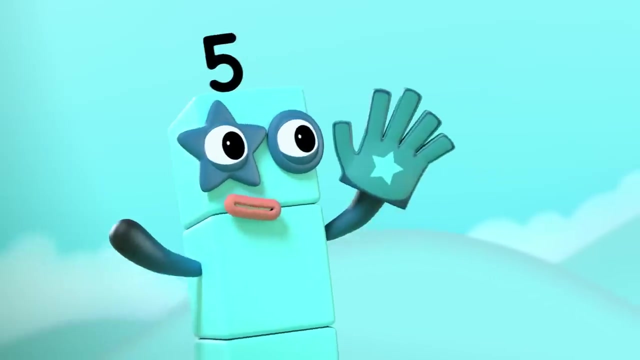 Woo-hoo, Five minus four equals one. Only five can stop the train. so how do we make five a game? One, two, three, four, Hey, Only five can stop the train. so here I am to try again. 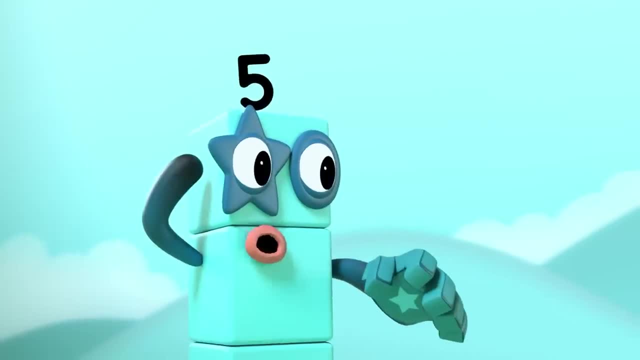 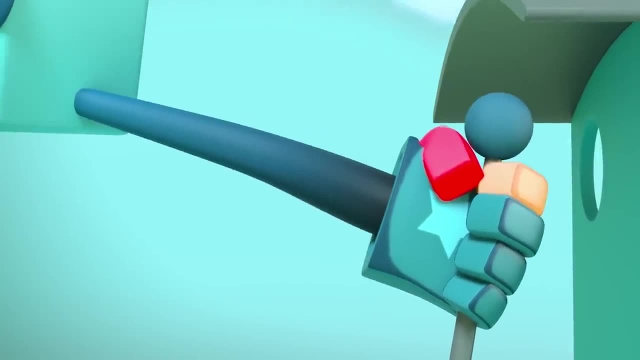 Yeah, Only five can stop the train. so here I am to try again. Yeah, Only five can stop the train, so here I am to try again. Oh no, we're in a mess. Stop the number. blocks express One, two, three, four, five. 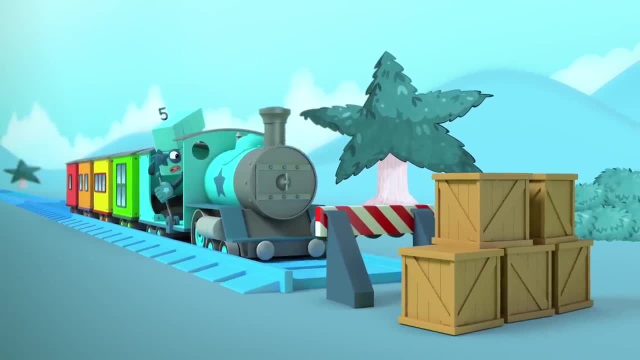 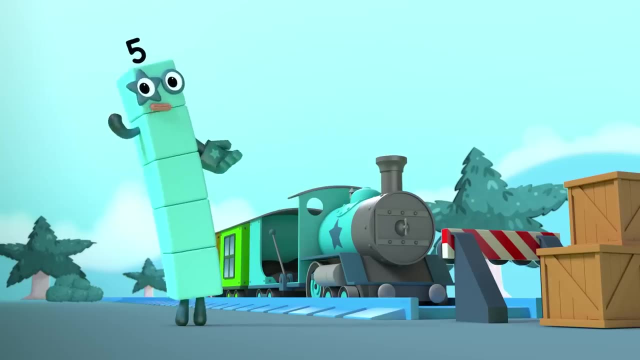 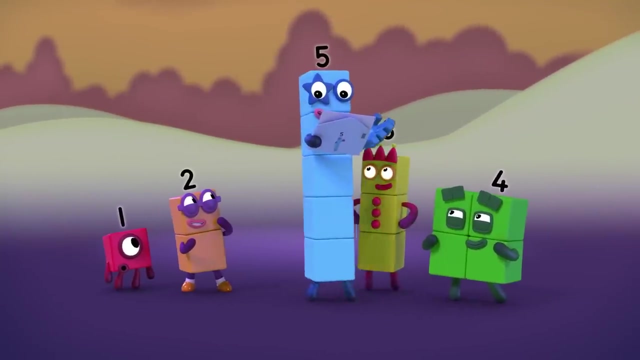 Five, High five, Success. I stopped the number blocks express Woo-hoo. Yeah, Now what could this be? Oh, Five and fresh. The twins are invited to a five-star ball at the Two Palms dance floor. Oh, 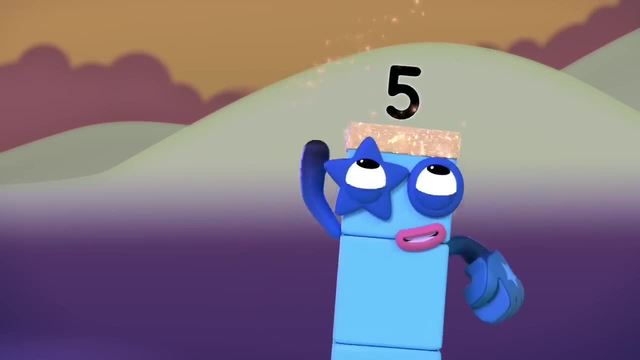 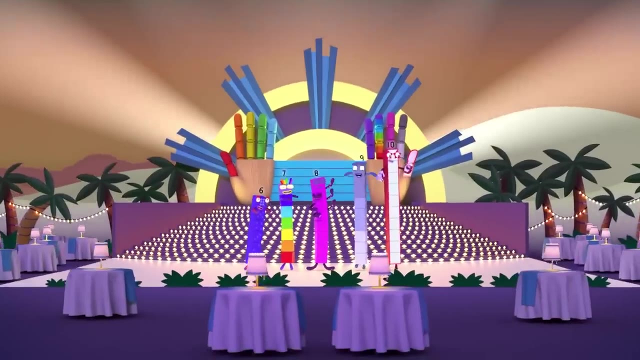 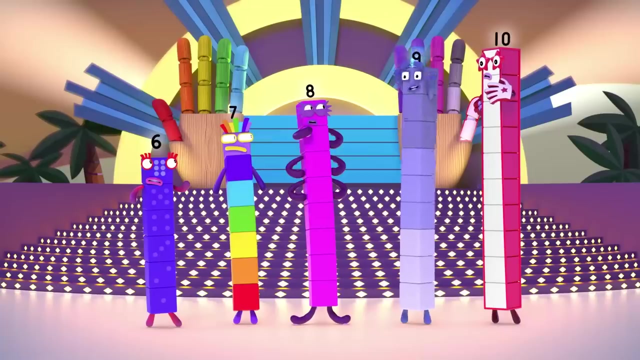 Yes, I can wear my sparkly headband, The Two Palms. Where's that? Um, Um, La-la, Ooh, Doo-doo, Oh, Don, Where's Five? We can't start a Five and Friends dance without Five. 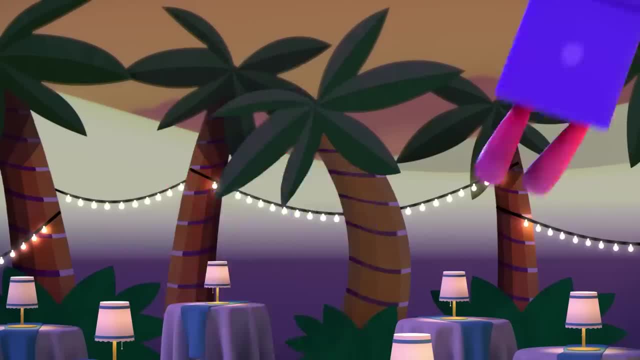 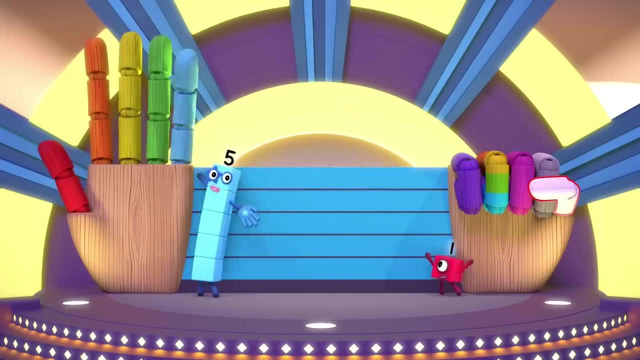 Huh, Why wait? Just look and you will see that Five is here as part of me. Ready, I'm Six. I'm Five. I'm One. Five, I'm Five. I've got a Five in me too. I'm Seven. 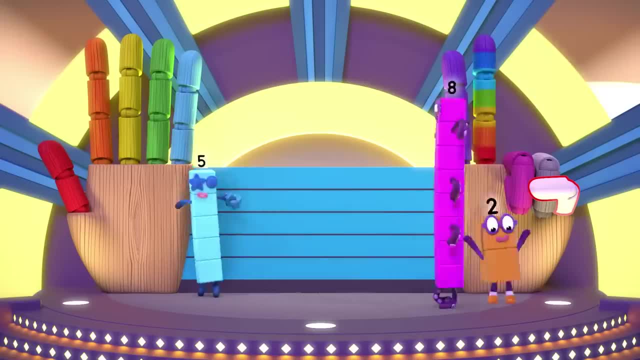 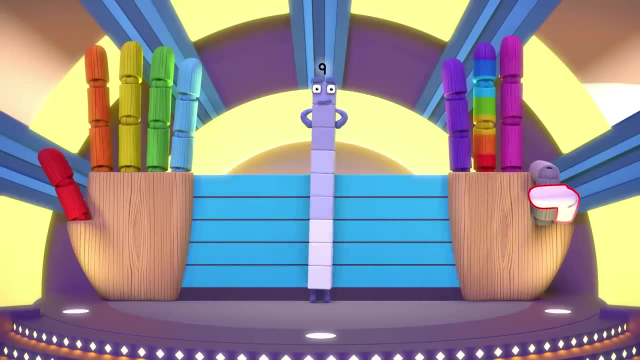 I'm Five And Two, Five And Two. I'm Eight, I'm Five And Three, Five And Three. I'm Nine, I'm Five And Four, Five And Four And Nine And Four And Five. 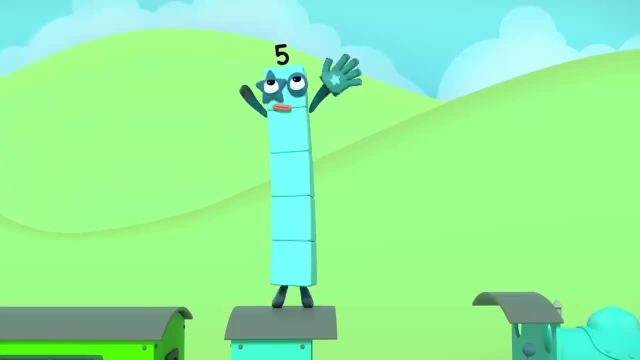 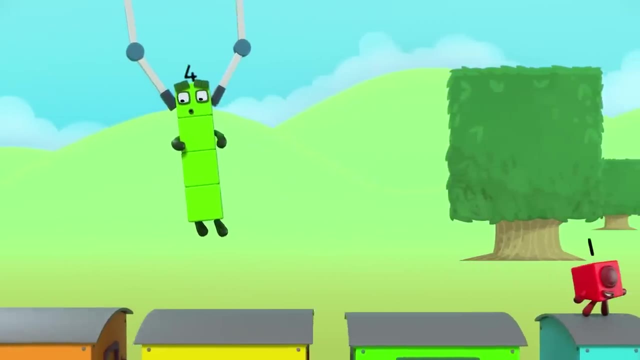 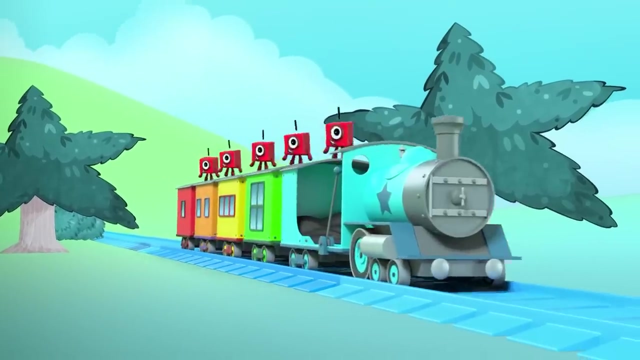 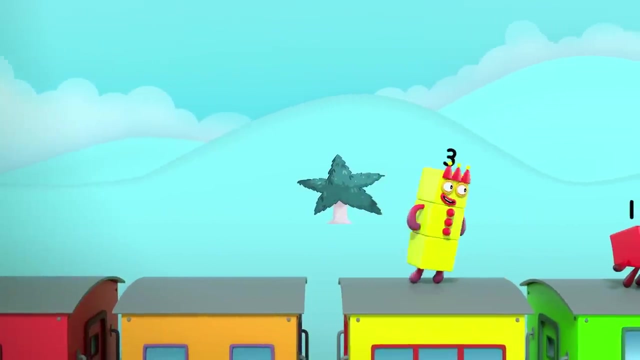 Only five, no more, no less, Can stop the number of lives expressed. Woo-hoo, Five plus four equals one. Only five can stop the train. So how do we make five again? One, two, three, four, Hey, Only five can stop the train. 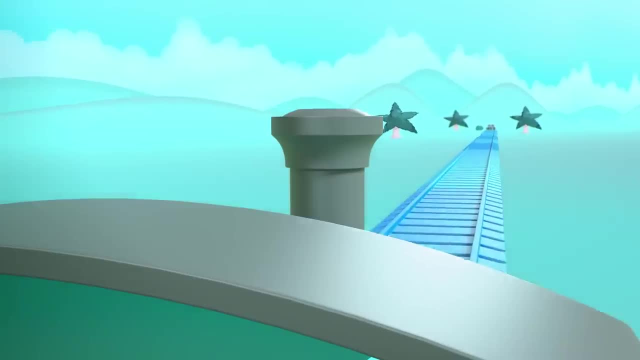 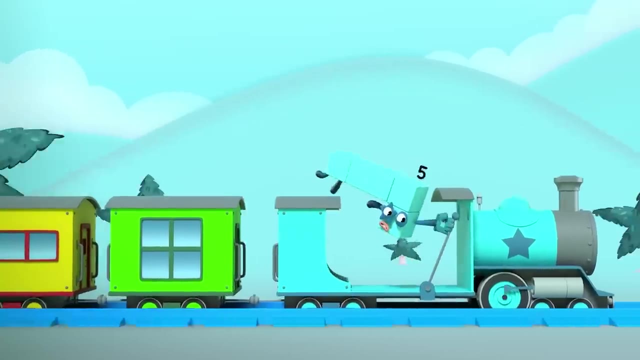 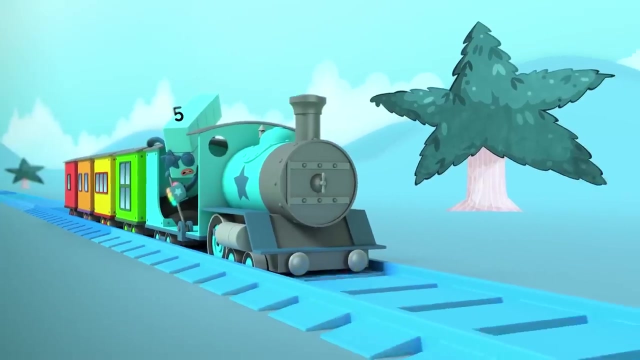 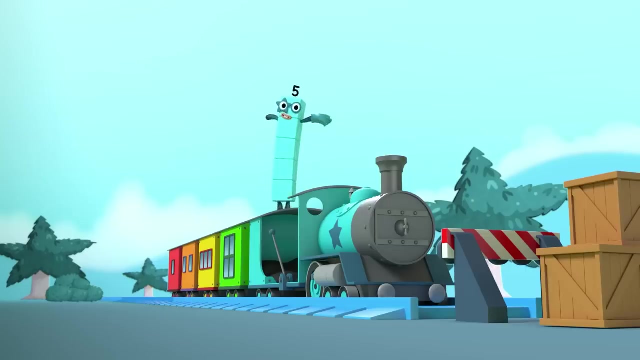 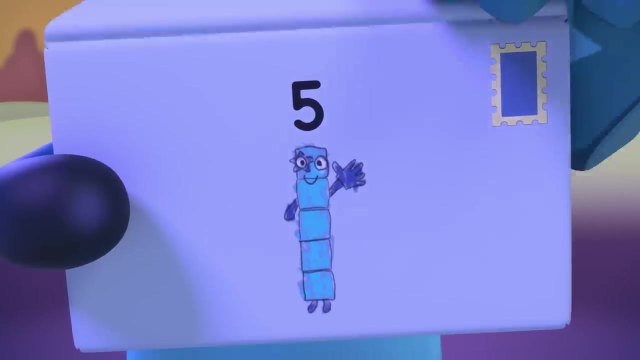 So here I am to try again. Uh-oh, no, we're in a mess. Stop the number blocks express One, two, three, four, five, High five, Success. I stopped the number blocks express Woo-hoo, Yeah. Now what could this be? 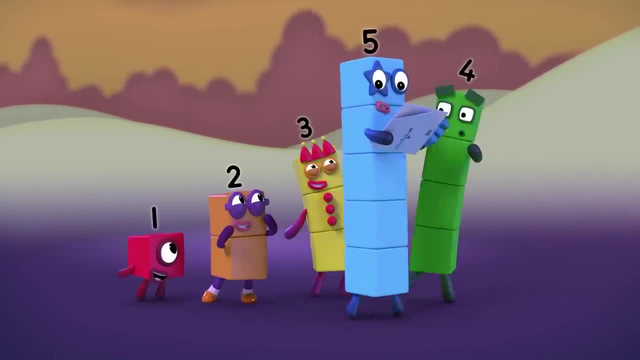 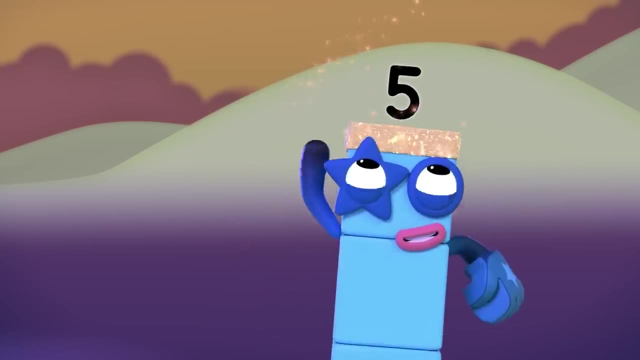 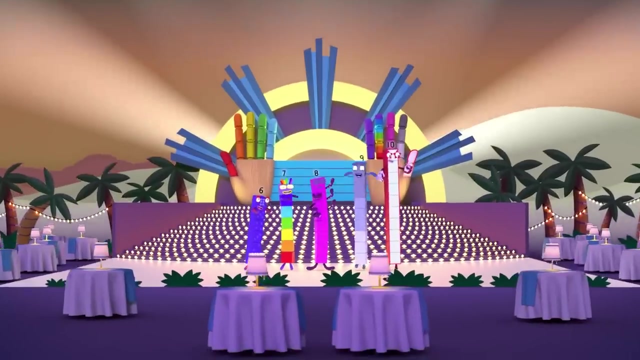 Ooh Five and friends are invited to a five-star ball at the Two Palms dance floor. Ooh, Yes, I can wear my sparkly headband, The Two Palms. Where's that? Um, Um, La-la, Ooh, Doo-doo. 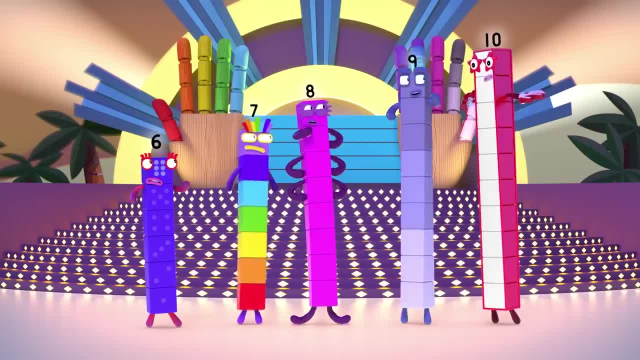 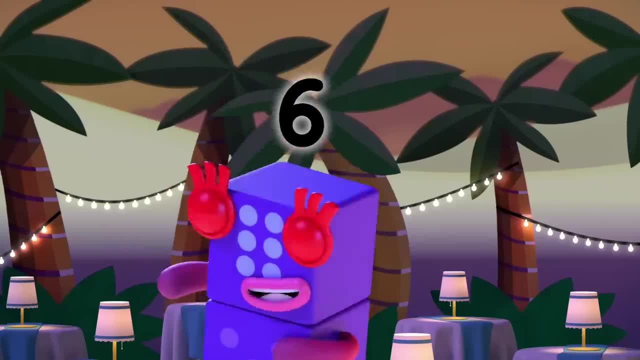 Oh Don, Where's five? We can't start a five-and-friends dance Without five. Huh, Why wait? Just look and you will see that five is here as part of me. Ready, I'm six, I'm five and one. 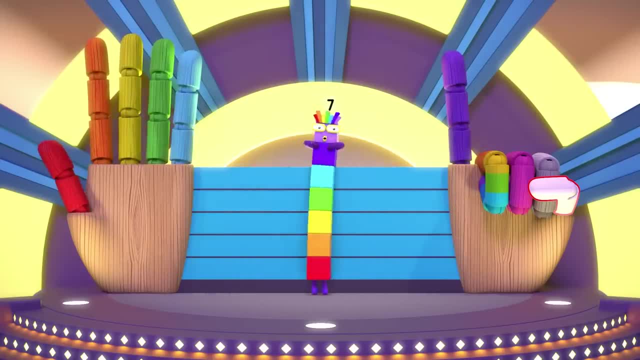 Five and five. I've got a five in me too. I'm seven. I'm five and two. Five and two. I'm eight. I'm five and three. Five and three. I'm nine. I'm five and four. 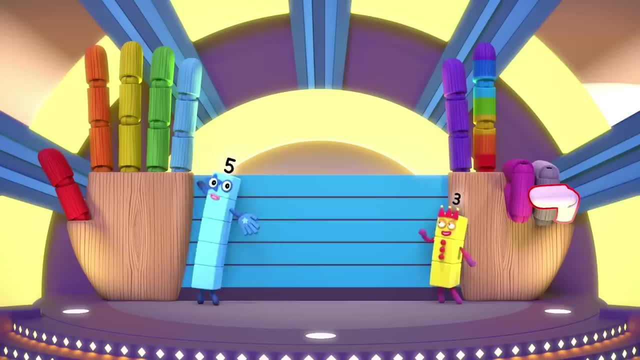 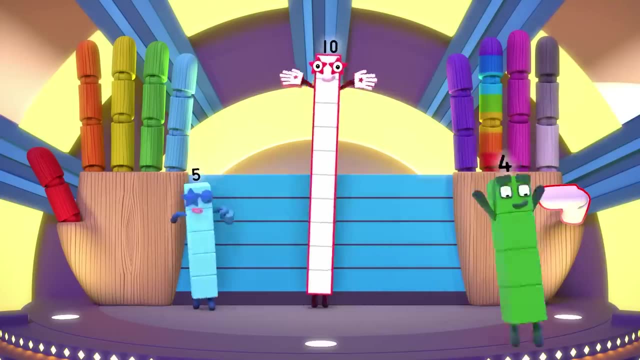 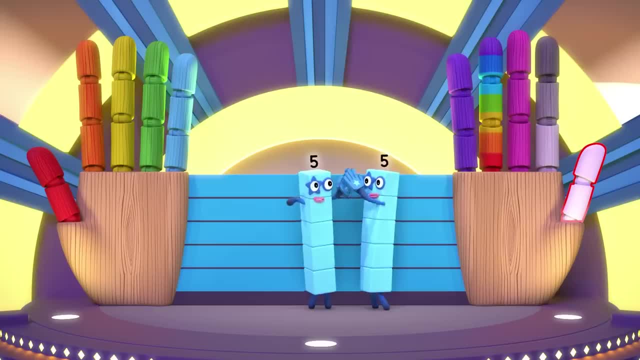 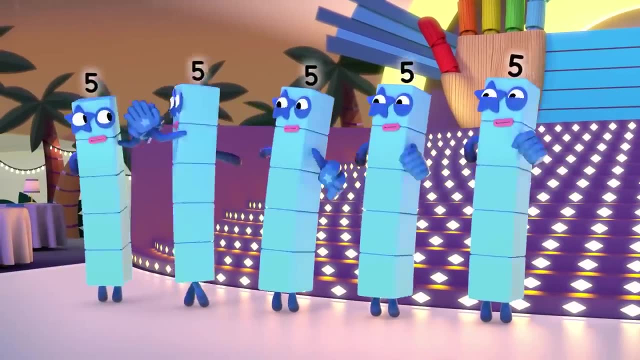 I'm nine And five And five And five And I'm ten, I'm five And another five High-fives, Five and five. Hey look, Five, fives, High-five. Ooh, Up to the side. 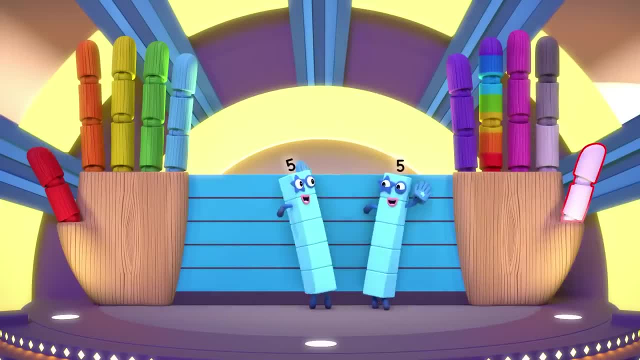 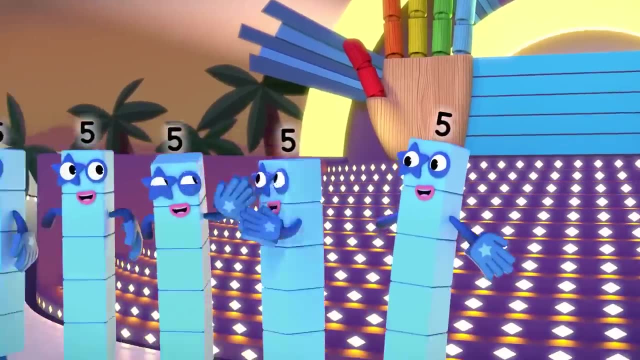 And Ten, I'm Five, And another Five High Five. Five And Five. Hey look, Five Fives High Five. Ooh, Up to the side Up above, Down low, Too slow, Hooray. 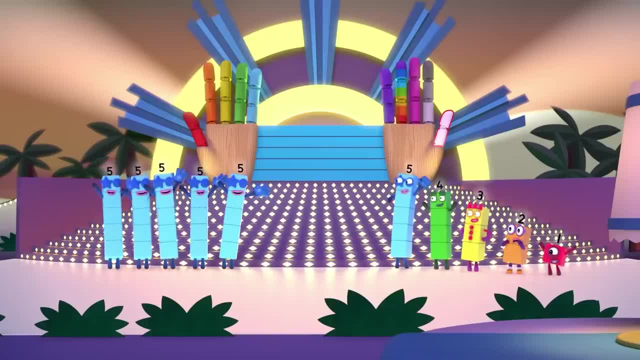 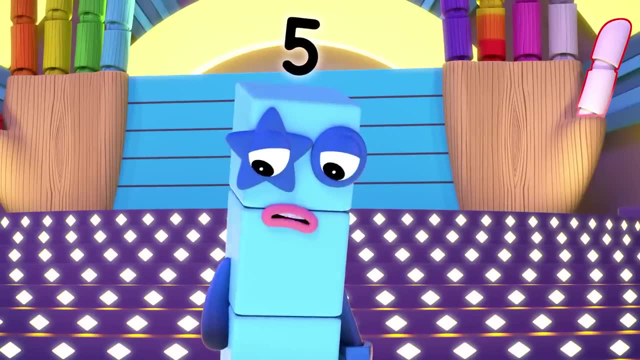 Hey wait, There are loads of Fives here now, but where are Six, Seven, Eight, Nine and Ten? We can't start the dance until all my friends are here. Let's go and find them. Hooray, Hooray. 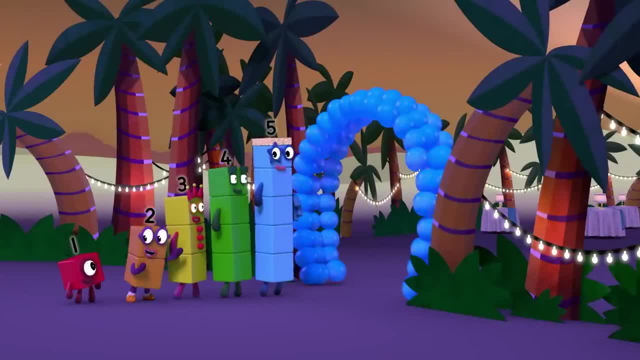 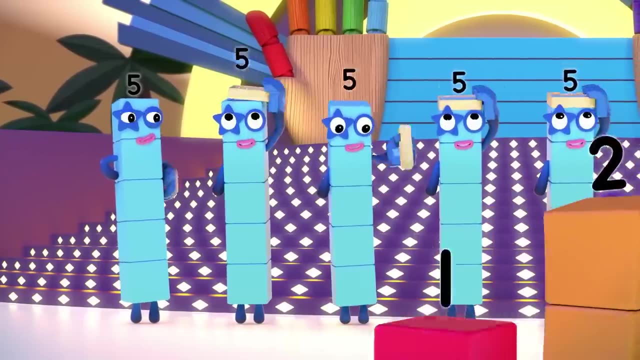 We can make friends, We have to putiji down. Hooray, He's all bugged. He's been in the way. Wahey Ha заключfan van der schijf, All right, Oof All of them's in the way. 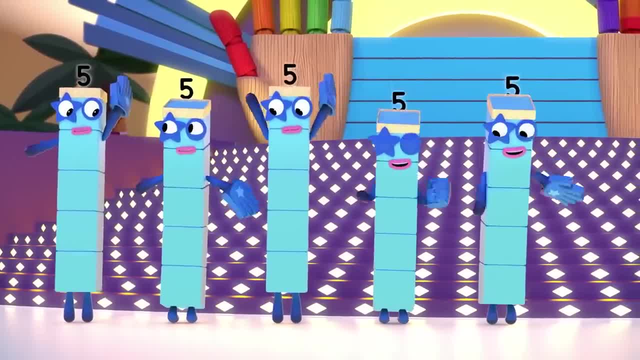 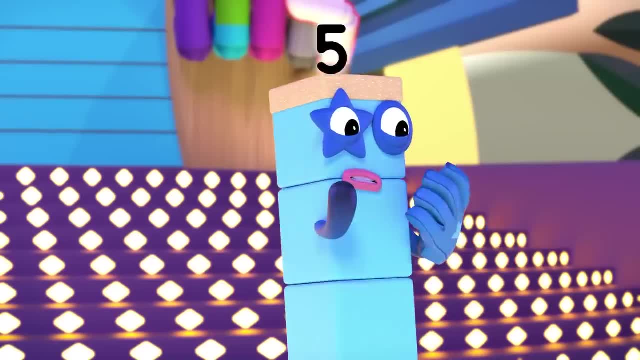 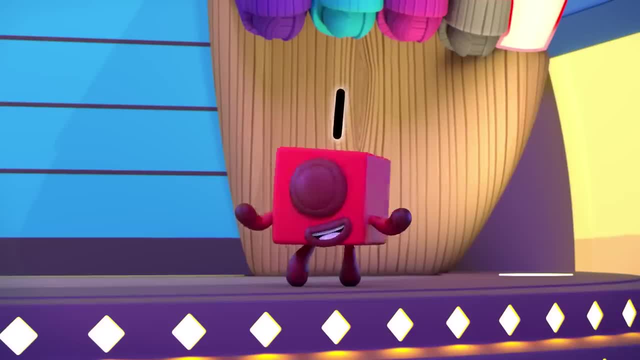 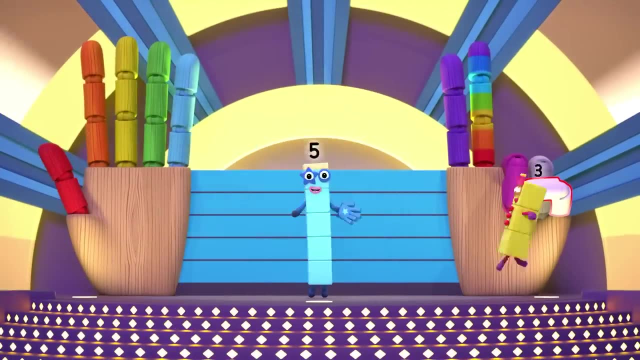 Huh, And you'll tell the truth. Five and one is six. Five and two is seven. Five and three is eight. Five and four is nine. High five, Five and another five is ten. Now let's get this party started. 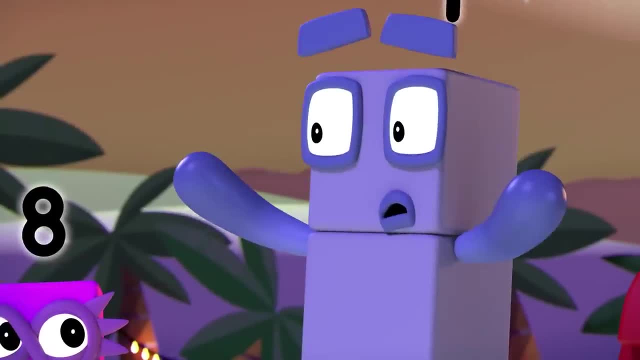 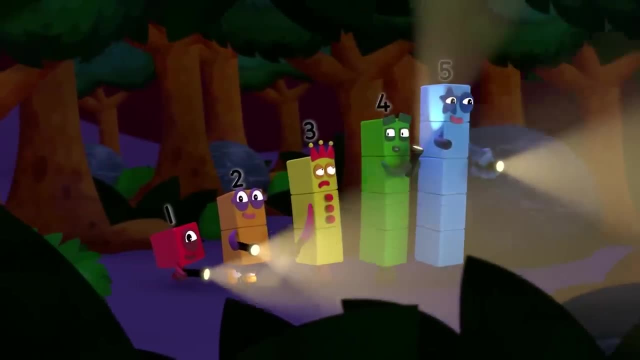 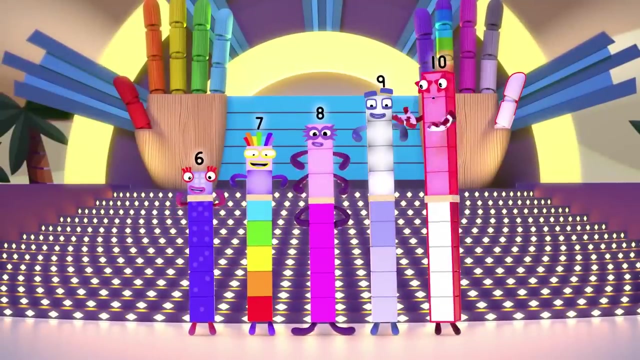 Hold on. We're a one, two, three, four and five. Where are they? Look here, above the sparkly line. Do you see who I see? Ready. I'm six, I'm five, I'm one, I'm seven. 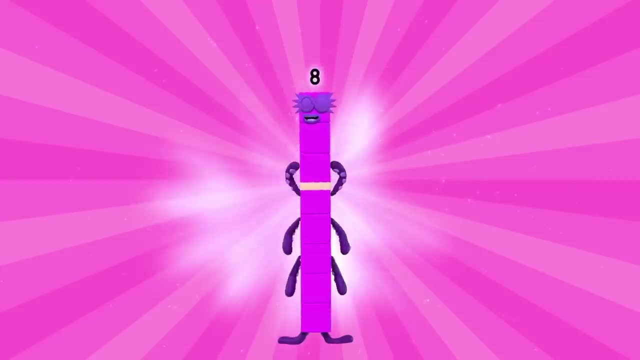 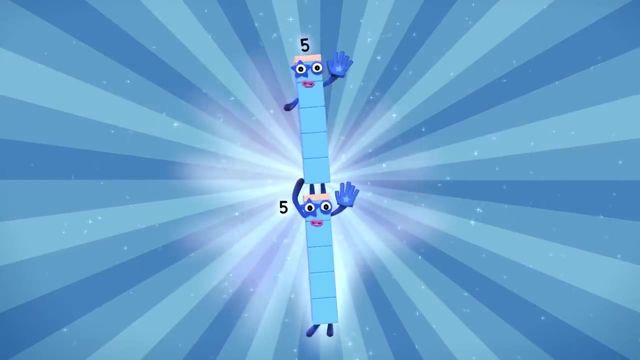 I'm five, I'm two, I'm eight, I'm five, I'm three, I'm nine, I'm five, I'm four, I'm ten, Five and another five, High five. Hey, wait, Where are six, seven, eight, nine and ten? 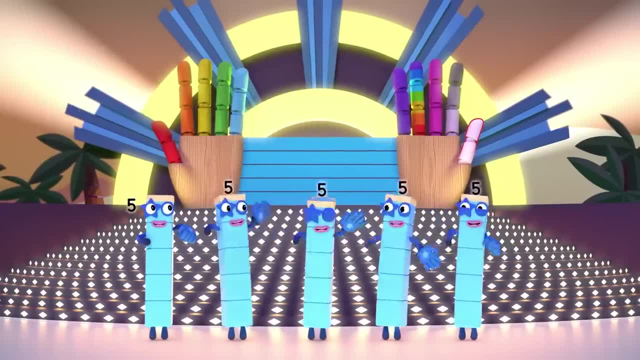 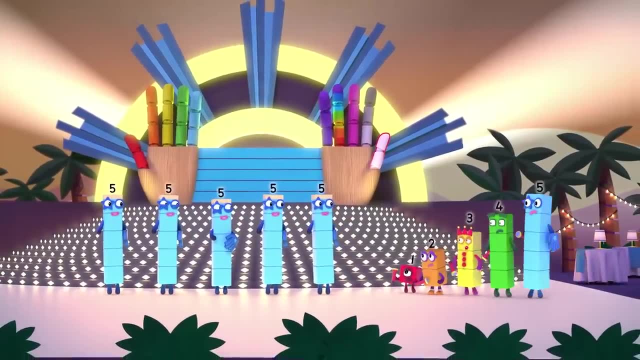 Let's go and find them. High five To the side. Oh boy, Jump up, don't low too slow. Oh, we're going here. We're aware of six to ten. Jump up here, You'll see them, men. 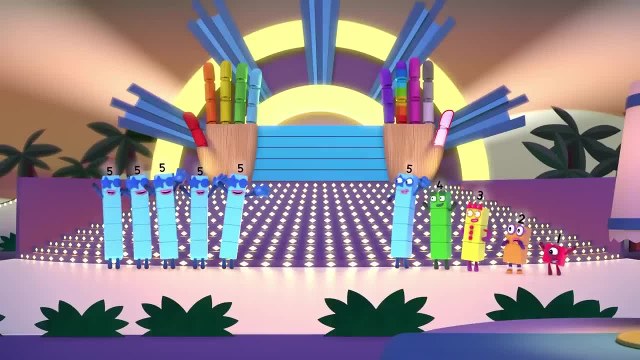 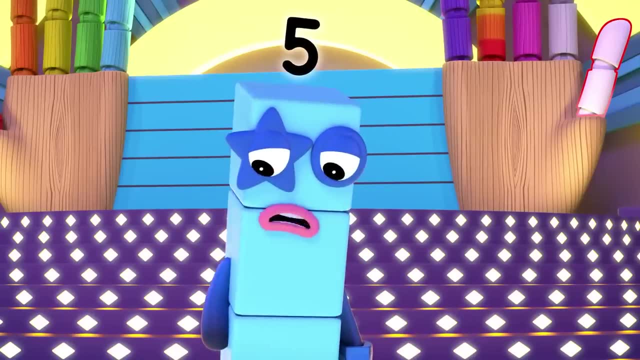 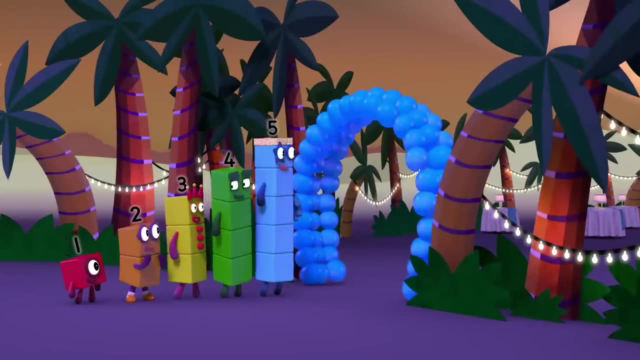 Up above, Down low Too slow. Hey wait, There are loads of fives here now, but where are six, seven, eight, nine and ten? We can't start the dance until all my friends are here, are here, Let's go and find them. Wow, This must be the two palms. Oh, wow And look. 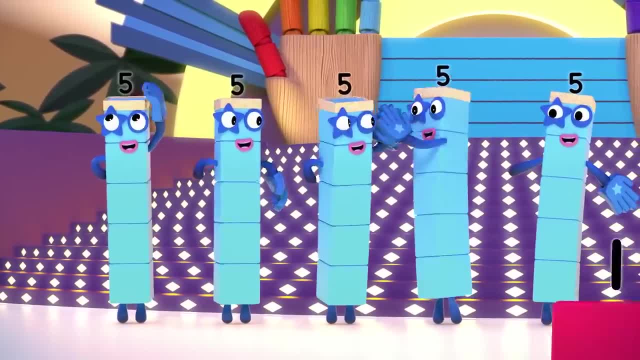 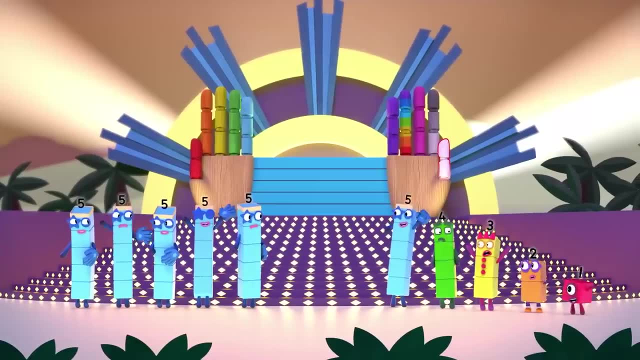 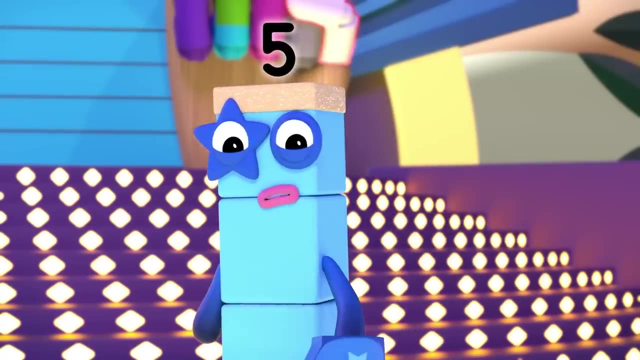 five, fives, Oh, High five. Oh, To the side above, don't go too slow. Wait, wait, wait. Where are six, seven, eight, nine and ten? We can't start until all my friends are here. 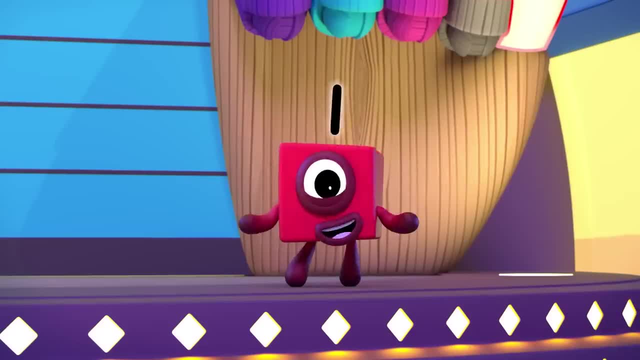 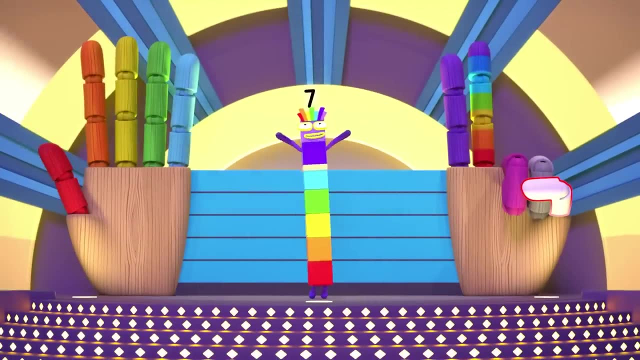 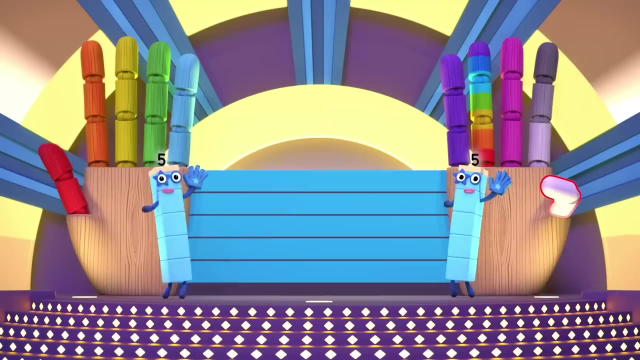 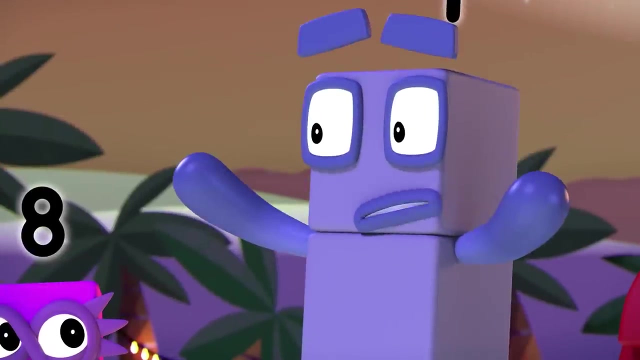 Hey, we can make friends Ready. Five and one is six. Five and two is seven. Five and three is eight. Five and four is nine. High five, Five and another five is ten. Now let's get this party started. Hold on, We're a one, two, three, four and five. 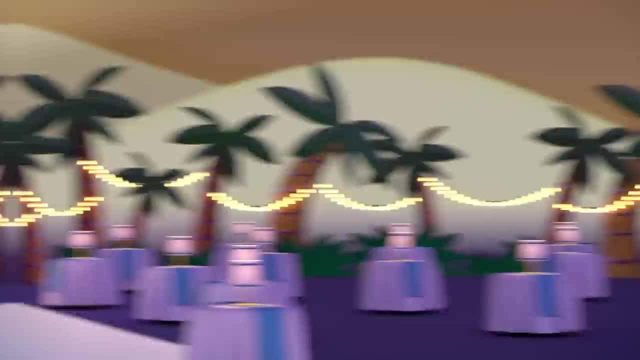 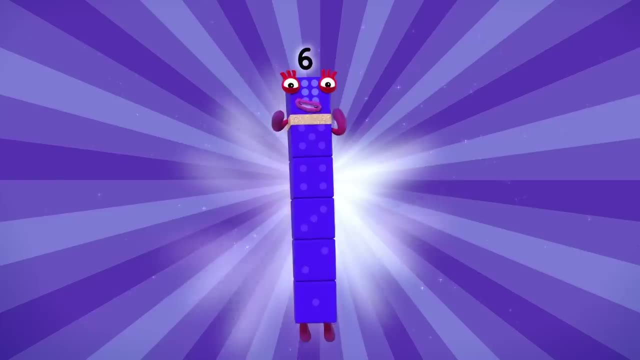 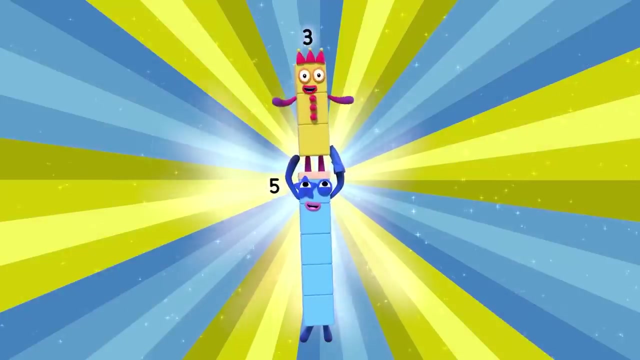 Where are they? Look here, above the sparkly line. Do you see who I see Ready. I'm six, I'm five, I'm one, I'm seven, I'm five, I'm two, I'm eight, I'm five, I'm three, I'm nine. 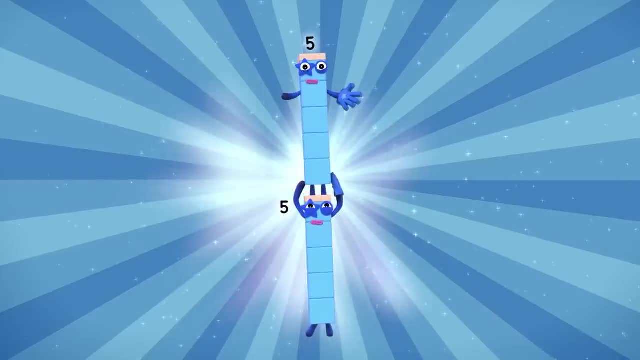 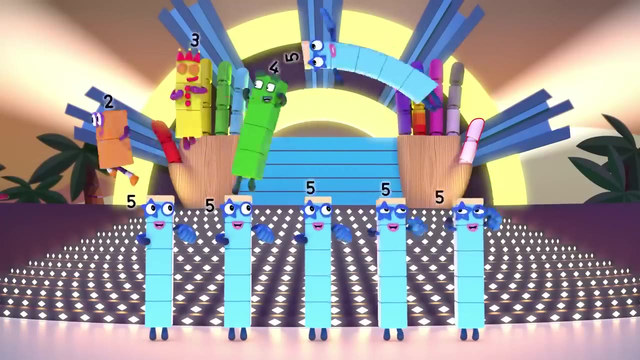 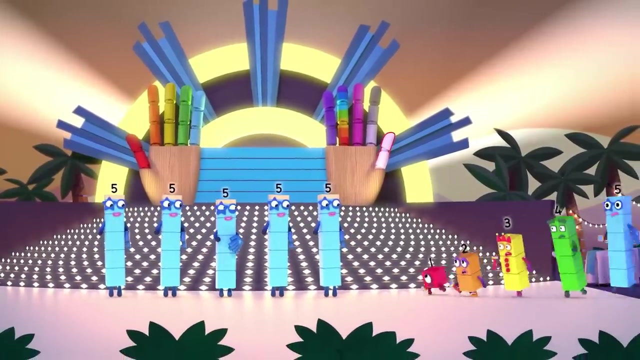 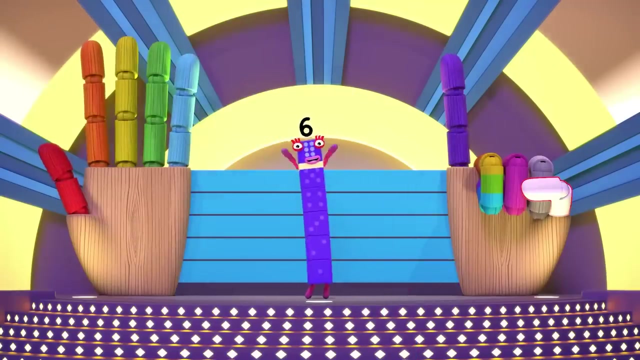 I'm five, I'm four, I'm ten, I'm five, I'm another five, High five. Hey, wait, Where are six, seven, eight, nine and ten? Let's go and find them. Five and one is six. Five and two is seven. Five and three is eight. Five and four is. 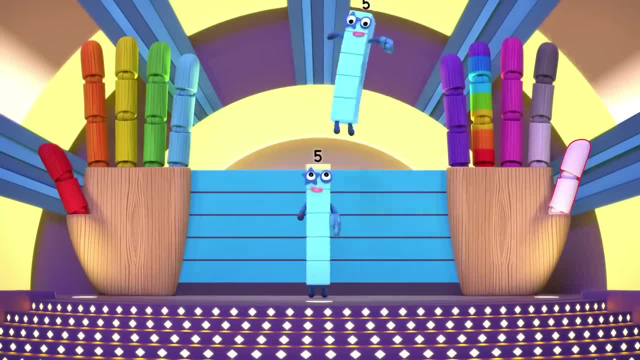 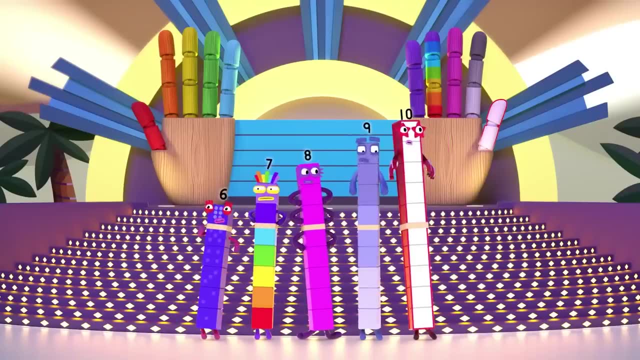 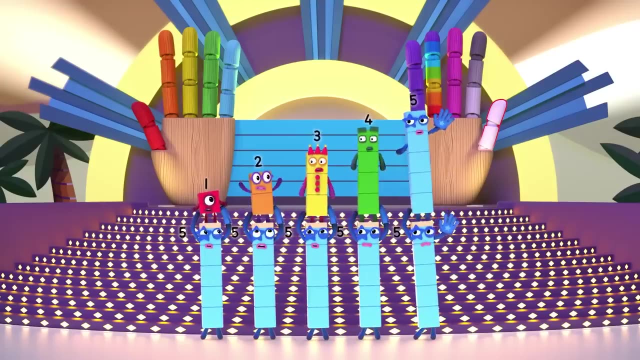 nine High five. Five and another five is ten. Now let's get this party started. Hold on, We're a one, two, five. Ooh, One two, three, four, five and another five High five. Hey wait, Where are six? 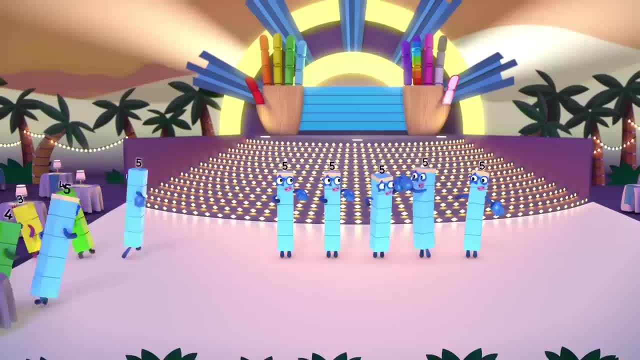 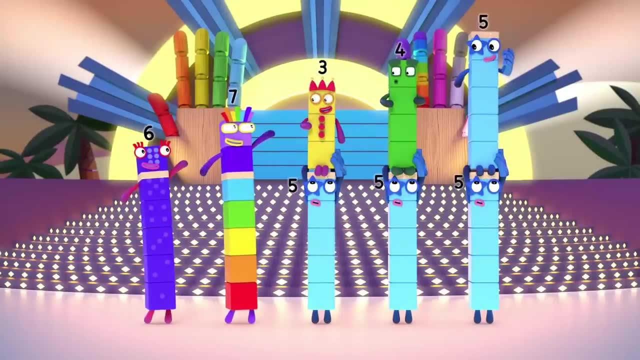 to ten. Let's go look for them again. High five, Ooh, Ooh. Where are we? We're a six to ten. Why don't you jump up again? Six, seven, eight, nine, five and another five. 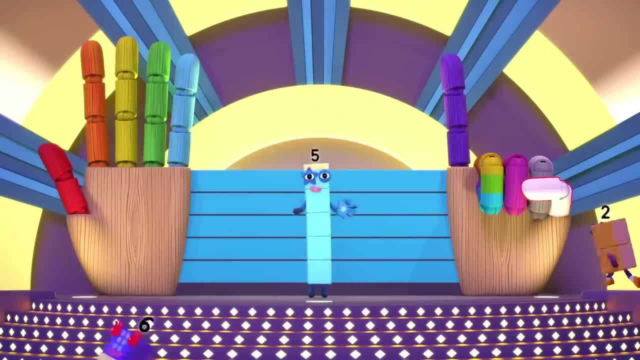 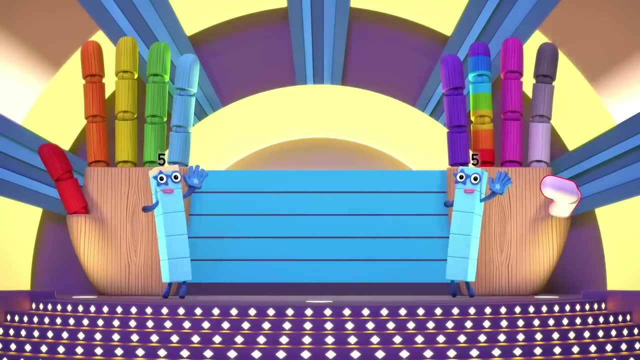 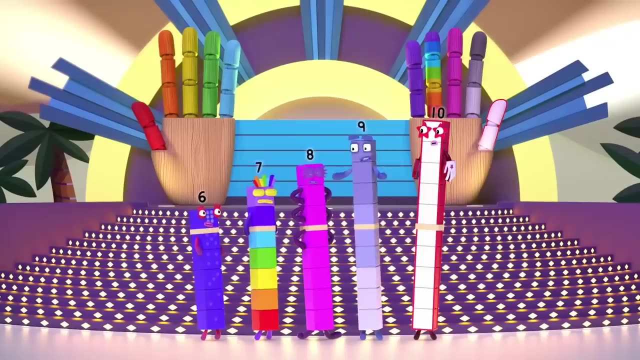 Ready Five and one is six. Five and two is seven. Five and three is eight. Five and four is nine. High five: Five and another five is ten. Now let's get this party started. Hold on, We're a one to five. 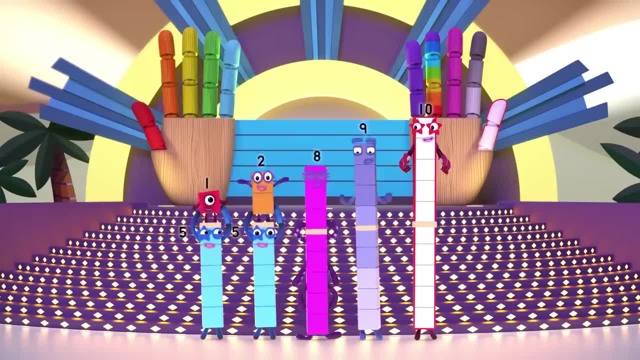 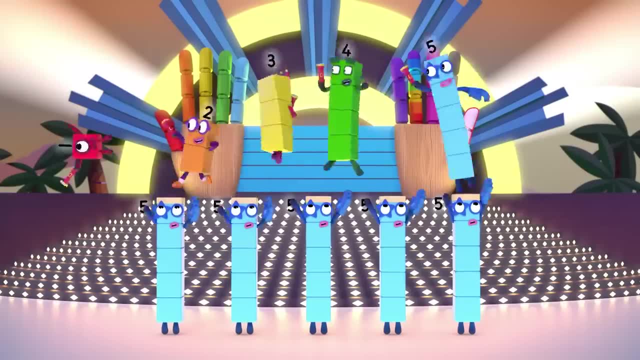 Ooh, One, Two, Three, Four, Five and another five. High five. Hey wait, Where are six to ten? Let's go look for them again. High five. Ooh, We're aware of six to ten. 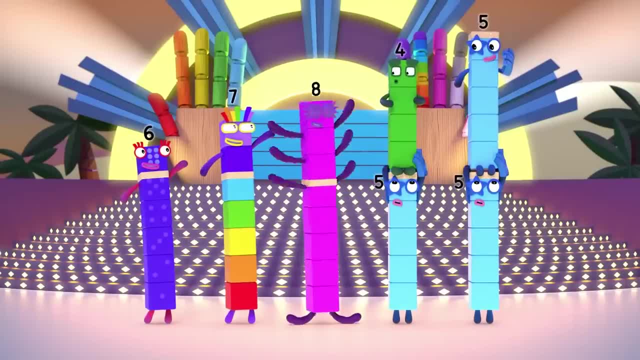 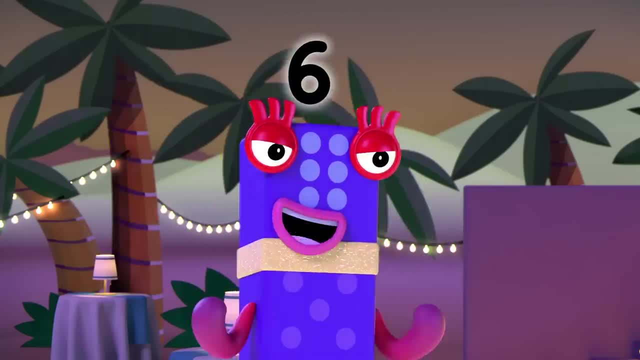 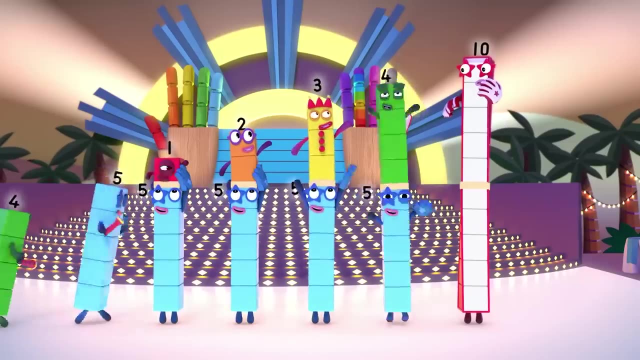 Why don't you jump up again: Six, seven, Eight, nine, Five and another five is ten. Let's get this party started. Hold on, Where are one to five, One, two, two, two? There we are. 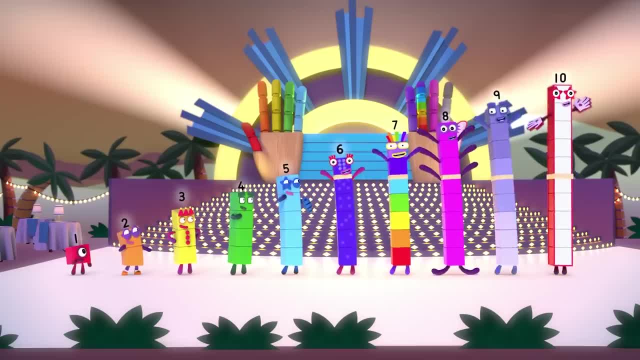 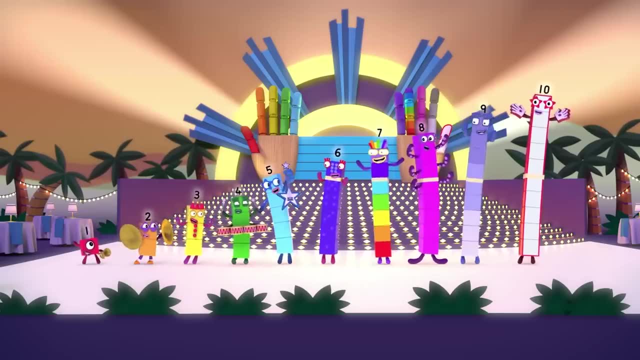 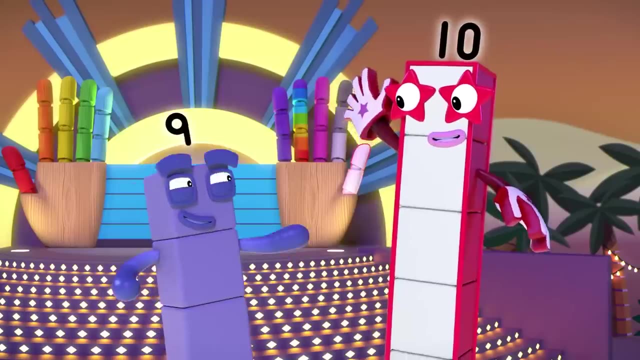 We're aware of six to ten. Here we are. My friends are all here. Let's get this party started. High five Ooh. To the side Up above. Don't low Too slow. High five Ooh. 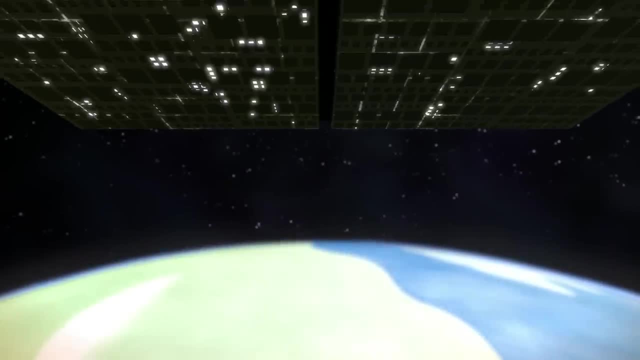 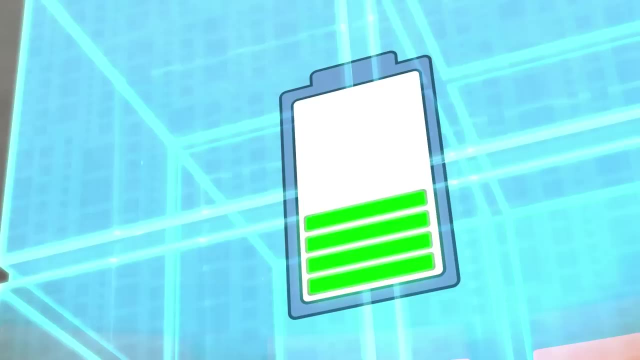 Ooh, Ooh, Ooh, Ooh Ooh. Come in number basis. I'm in position and heading for the Blockstar Careful 12.. The Blockstar's battery's running out. You need to change it before the whole thing drops out of the sky. 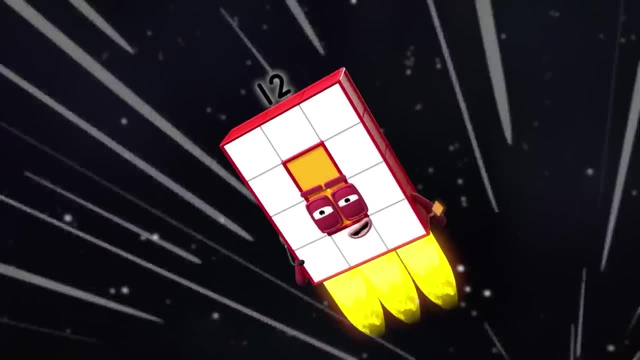 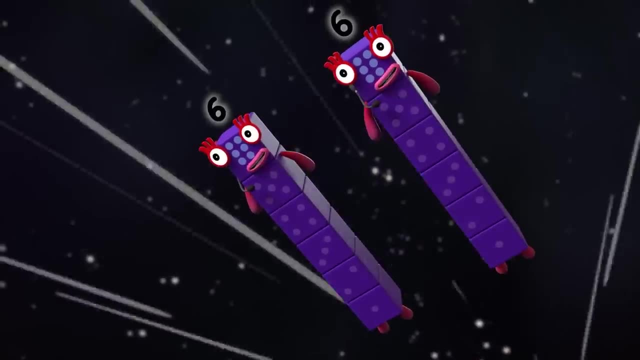 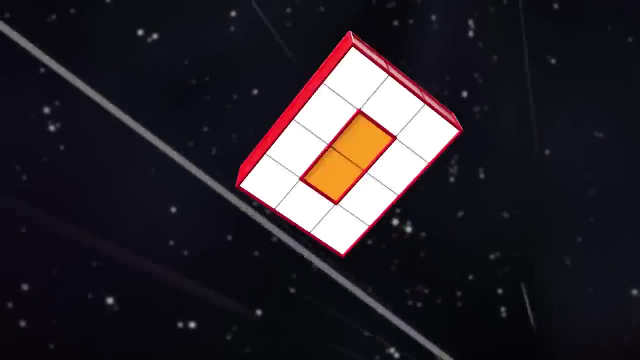 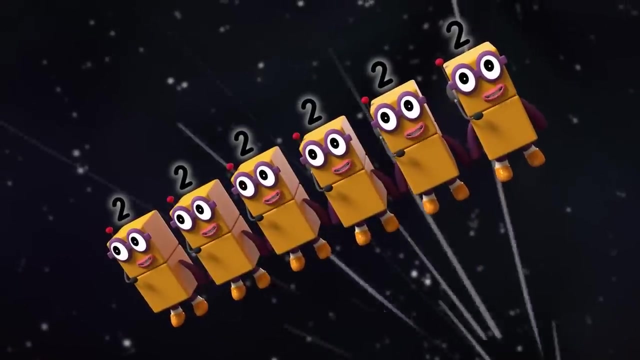 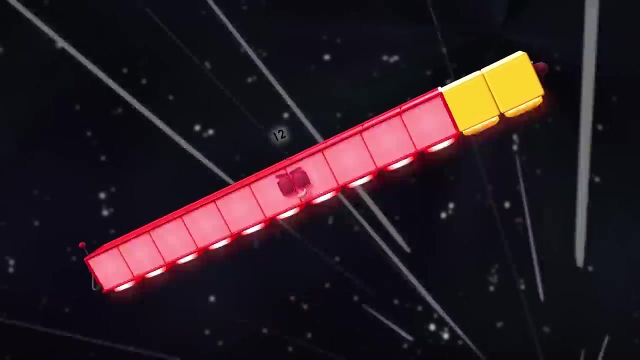 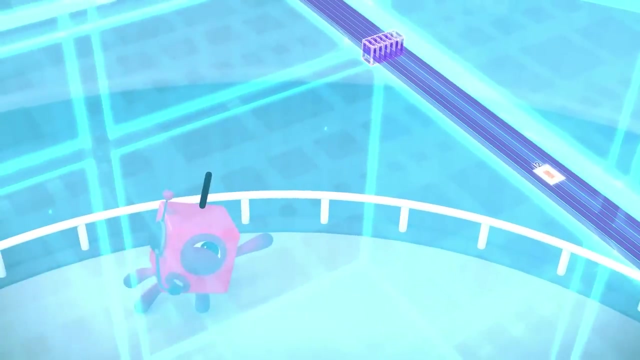 and smashes into Numberland. Oh, That block is no match for a super rectangle like me. All teams report in: Switch Two- sixes standing by. Switch Three- fours standing by. You need to turn off the force field before you can get to the battery. 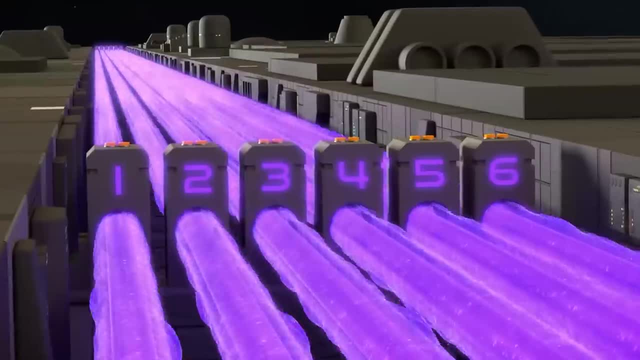 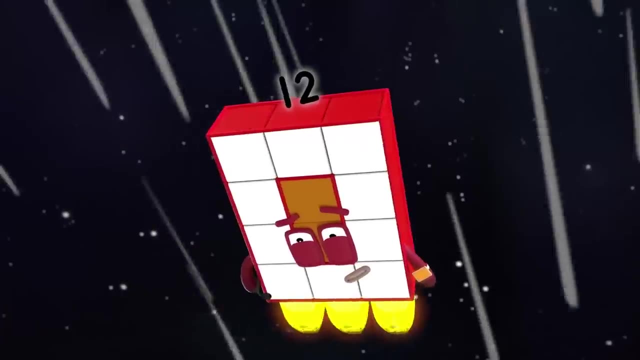 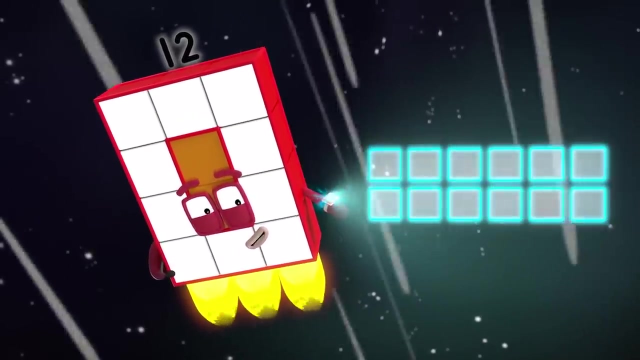 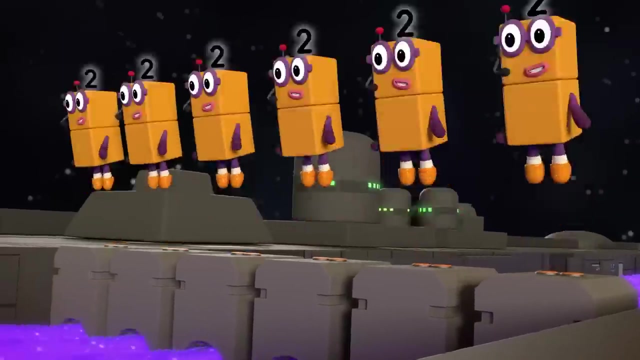 Can you see a line of towers ahead? Yes, six of them. Each has two buttons on top. You need to press all the buttons together. Six towers, two buttons each Array display. This calls for switch Whee, Six days. 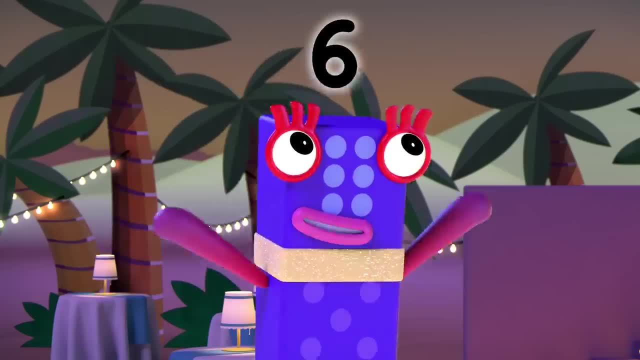 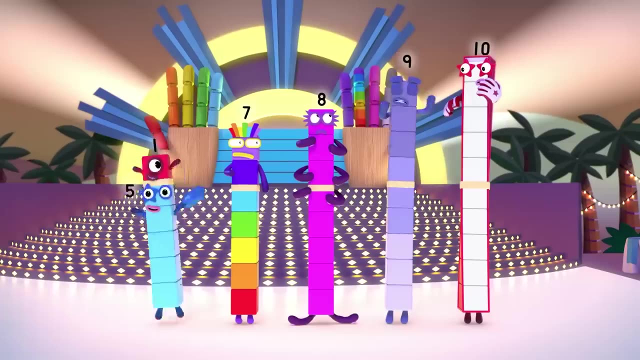 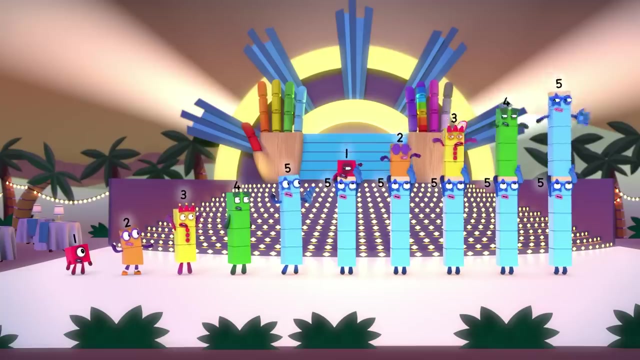 is ten. Let's get this party started. Hold on, Here we are. We're a one to five. There we are, But we're a we're a six to ten. Here we are. My friends are all here. let's get this party started. 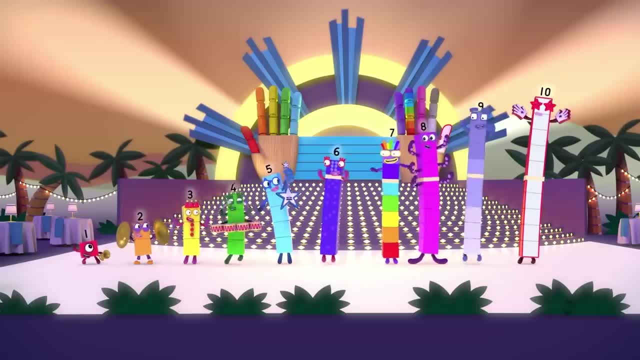 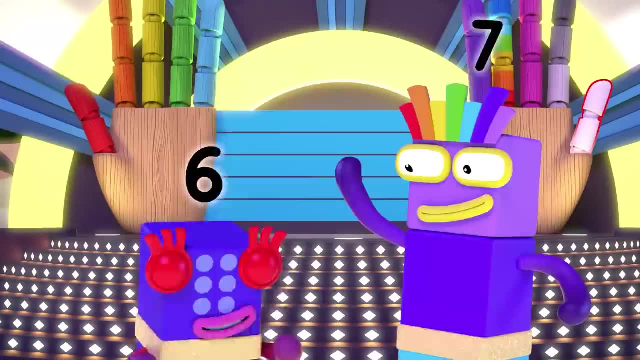 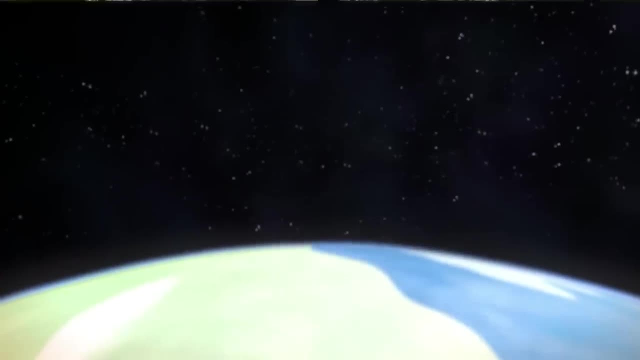 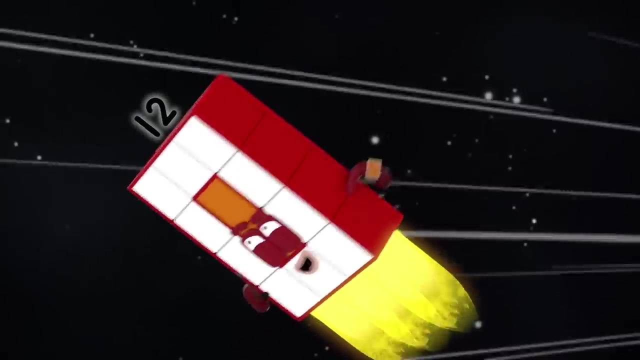 High five: Ooh To the side. High five To the side, Up above, Don't low Too slow. High five, Come in number. basic: I'm in position and heading for the Blockstar, Careful 12.. 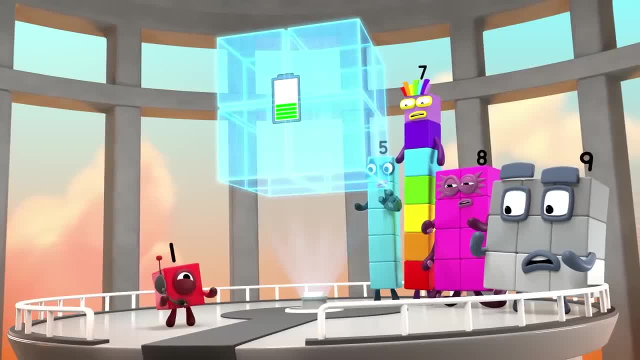 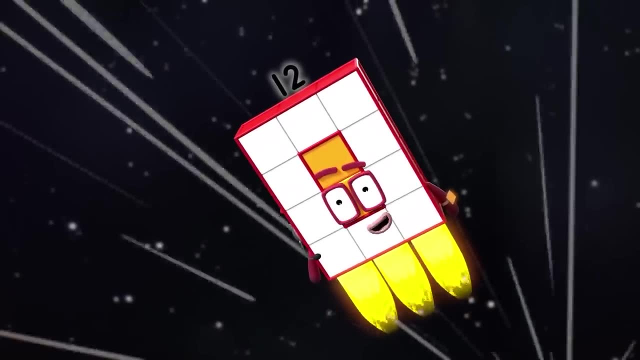 The Blockstar's battery's running out. You need to change it before the whole thing drops out of the sky and smashes into Numberland. That block is no match for a super rectangle like me. All teams report in Switch Two sixes standing by. 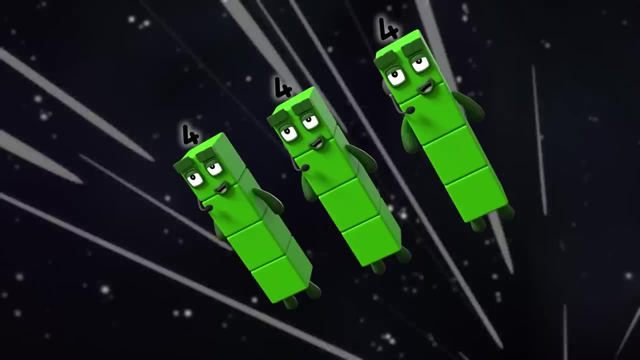 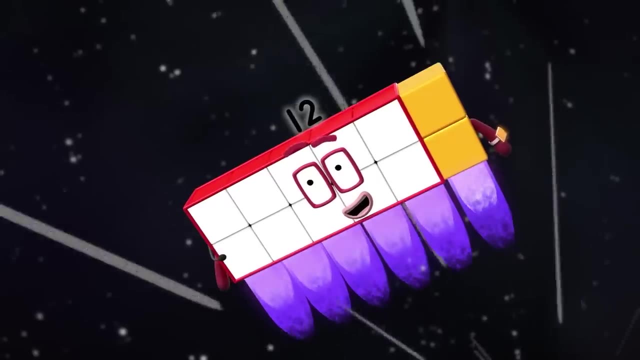 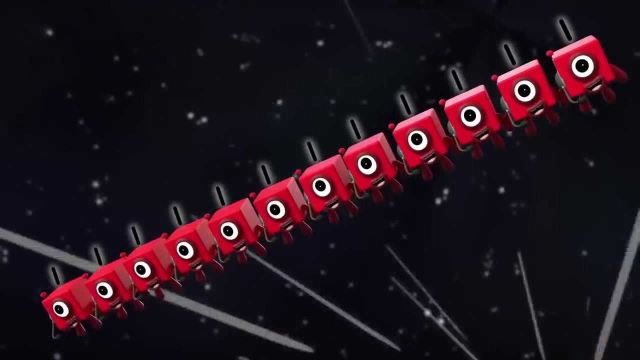 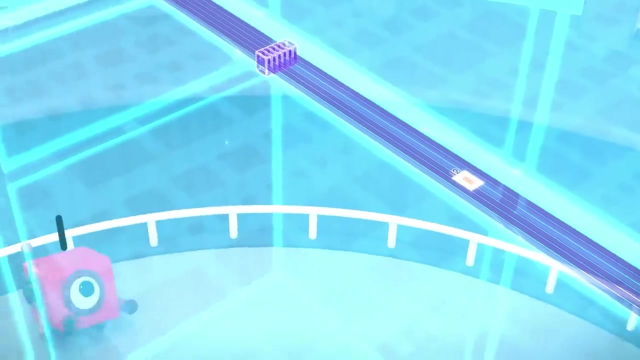 Switch Three. fours standing by Turn Four. threes standing by Switch. Six. twos standing by Switch. Twelve ones standing by Switch. I'm going in. Hold on tight. You need to turn off the force field before you can get to the battery. 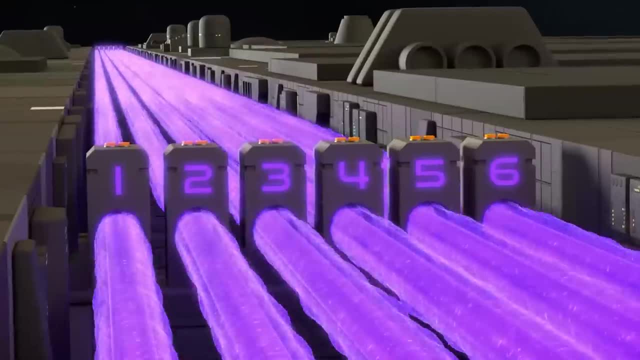 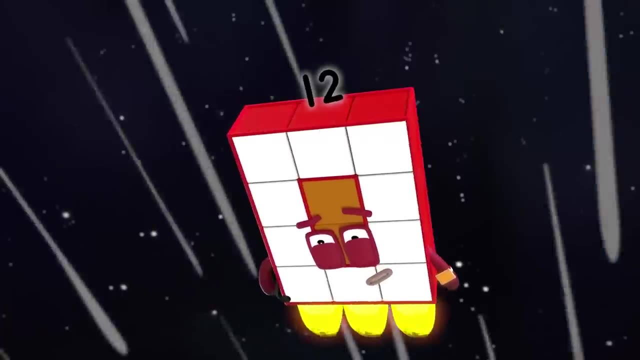 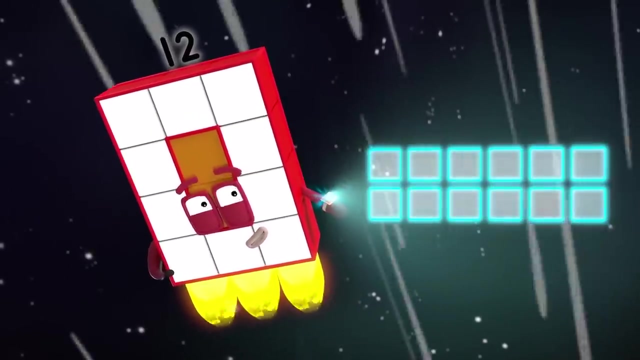 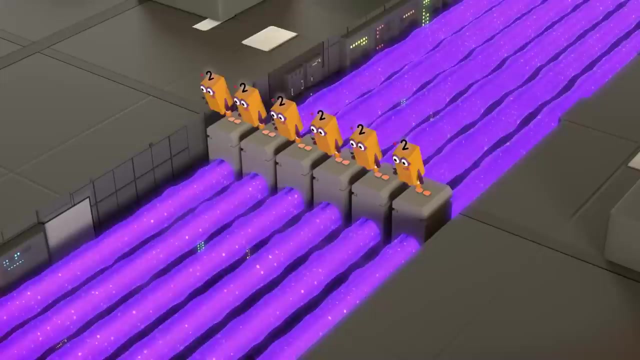 Can you see a line of towers ahead? Yes, six of them. Each has two buttons on top. You need to press all the buttons together. Six towers, two buttons each Array display. This calls for switch Three sixes. Hello. 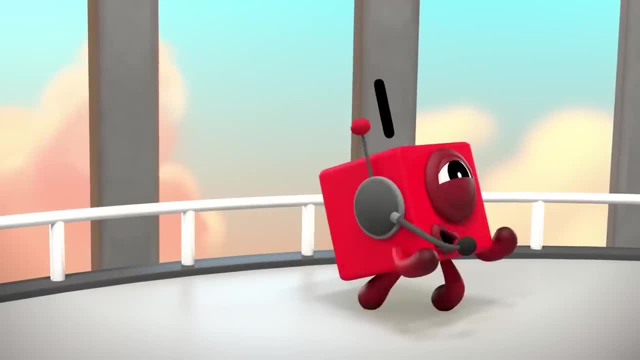 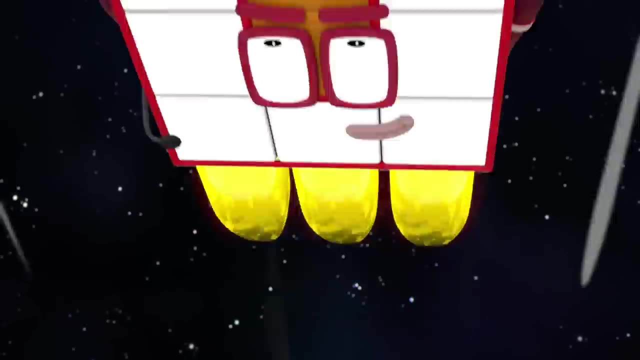 Yes, Lucky, You've done it. 12. Now head for that battery. There's no time to lose, I'm on it. Switch. Two sixes standing by Switch. Two sixes standing by Switch. 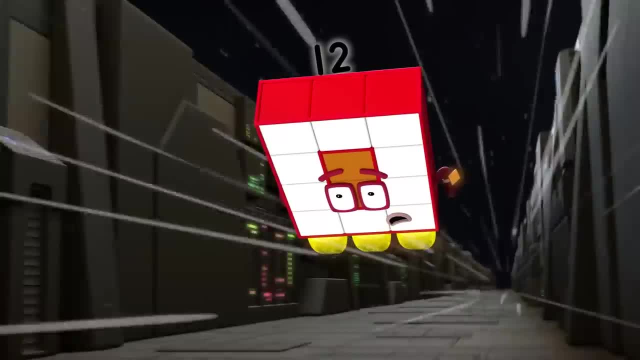 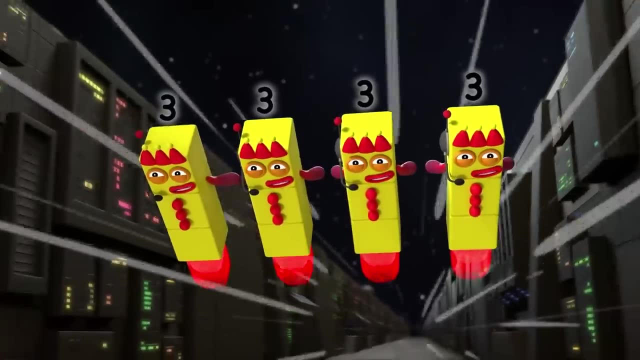 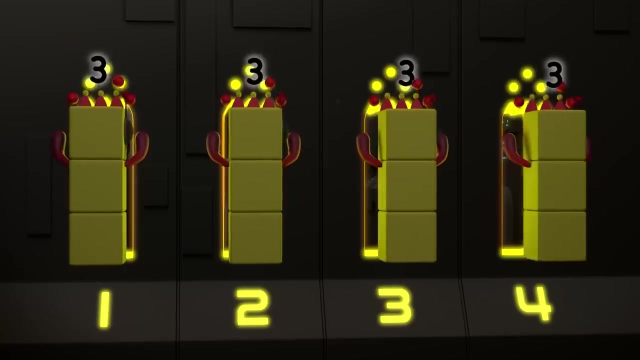 Two sixes standing by Switch. No, Disable the brain. Do this if you become a Nazi party member. Request результат. Pull up 12.. You're going to hit No time, Dire. We're in the trees, Okay. 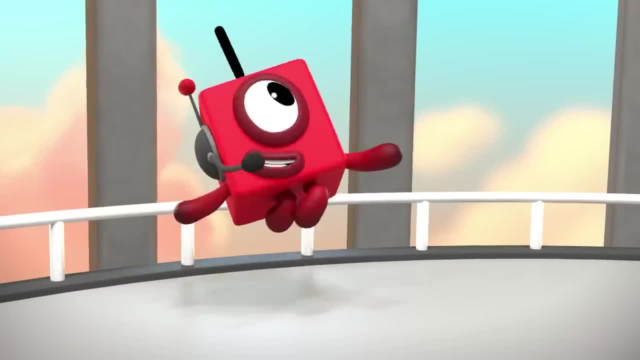 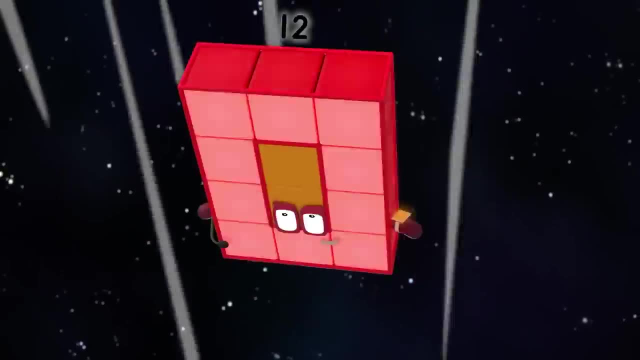 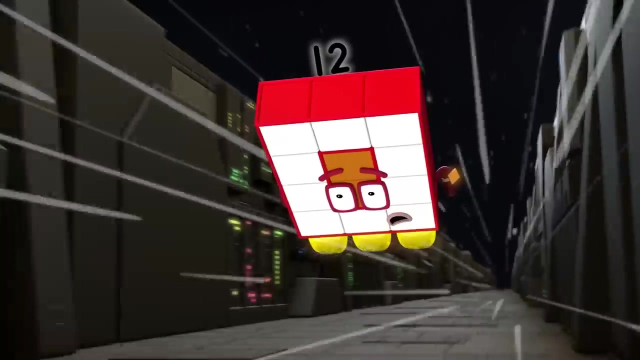 Whoa Lucky. Yes, You've done it. Twelve Now head for that battery. There's no time to lose. I'm on it. Switch, Pull up Twelve, You're going to hit. No time Turn. 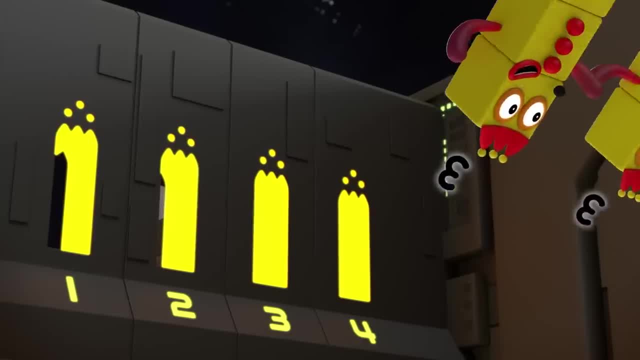 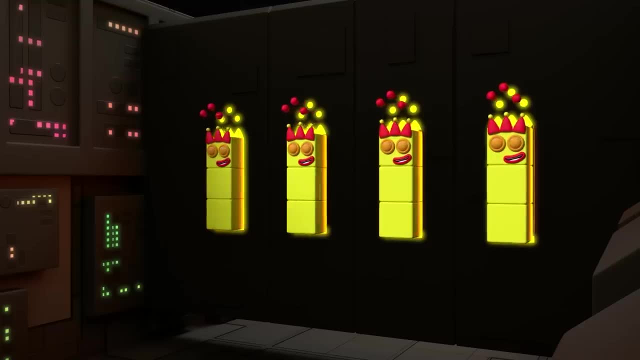 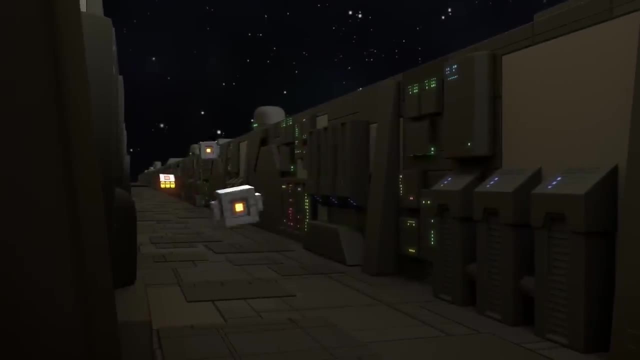 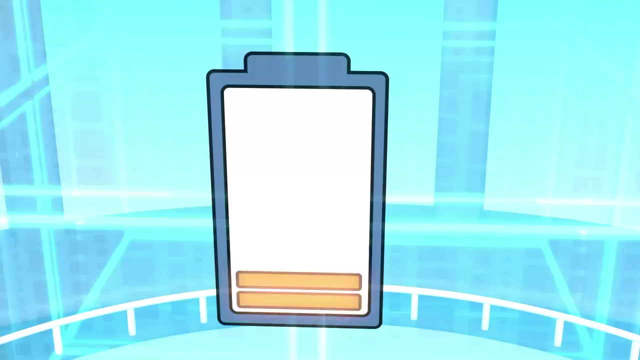 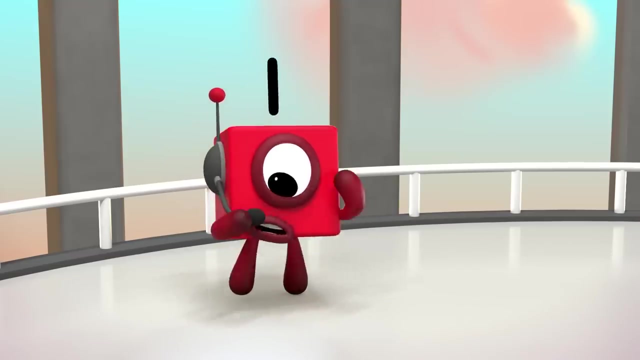 Four, threes, Whoa. Look at me. Look at me. Woo, hoo, Woo. Those blockships have gone haywire. It must be the low battery. Don't let the battery die. No, Don't let them slow you down. 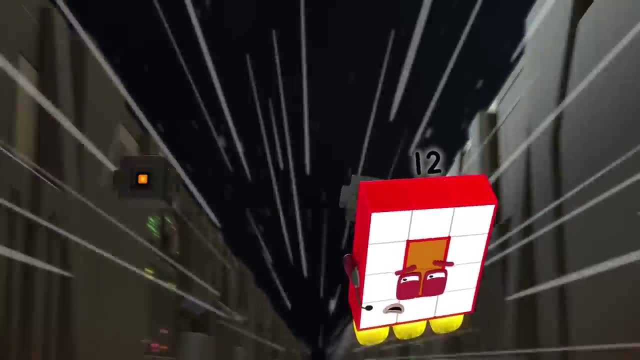 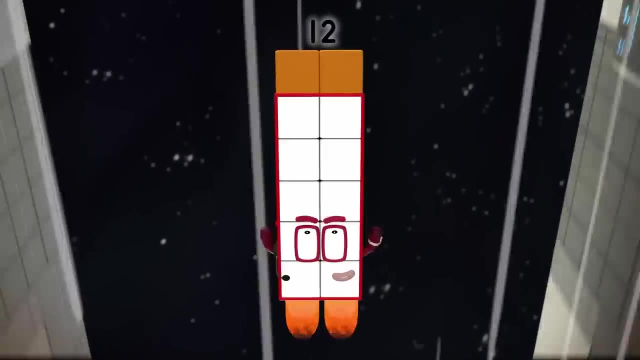 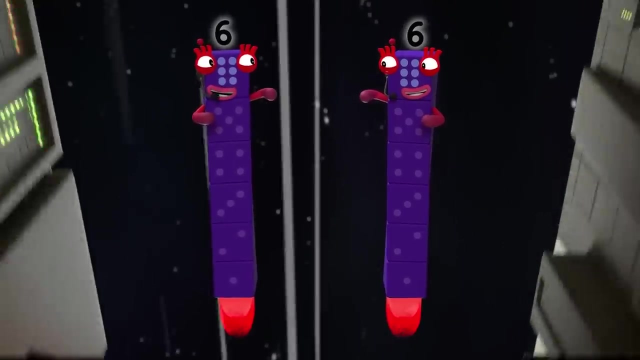 Hup, Hup, Wah, Woo-hoo, Awaited Blake, I've got just the team Switch, Two sixes. We've got a great escape technique. Let's play a game of hide-and-seek Switch. 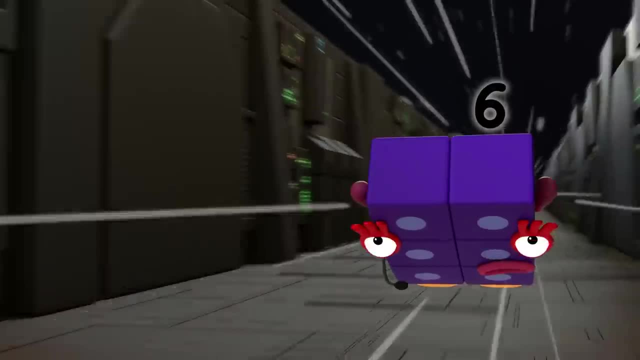 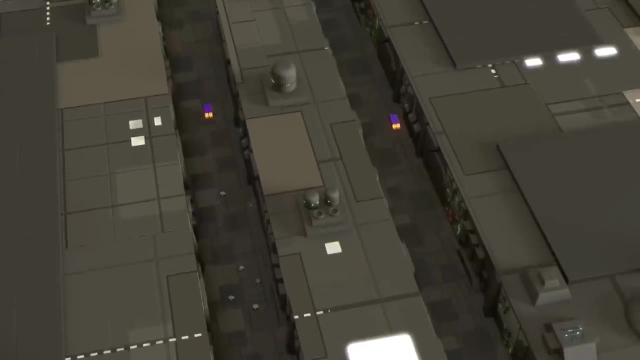 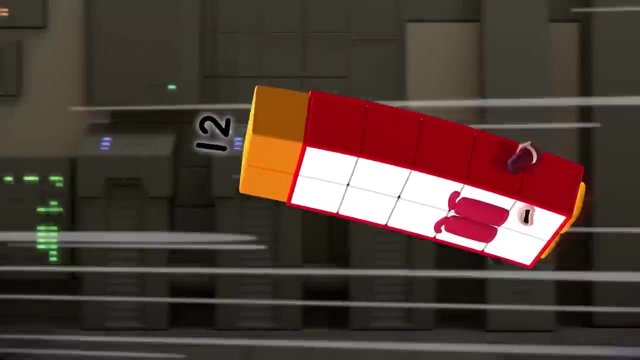 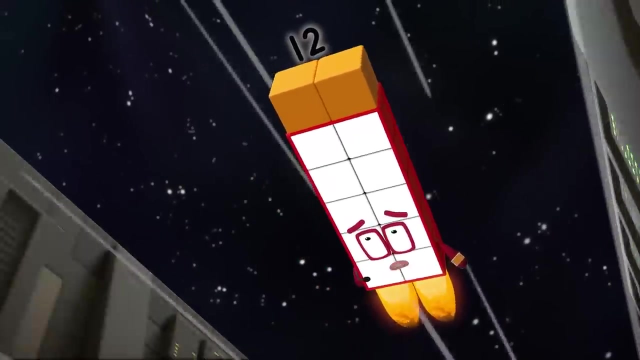 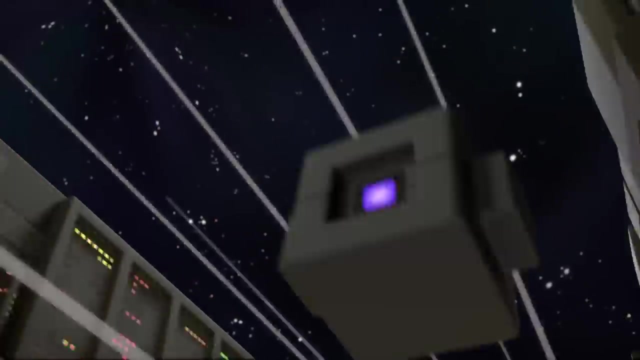 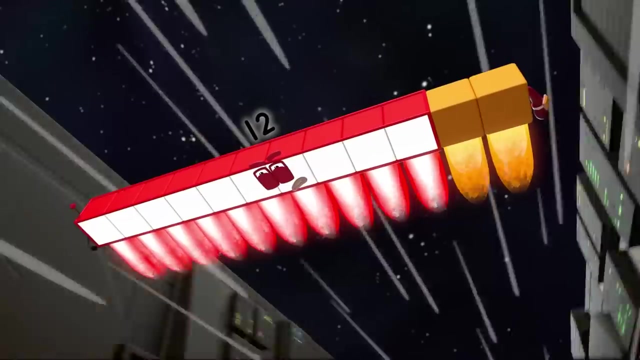 Catch me if you can. Hup, Hup. I've got to lose them Through there. Oh, I've got a bad feeling about this. A razor's blade, Long and low, Switch. Hup, Wah, Look out twelve. Twelve, what Phew Whoa. Battery level almost dead, but you're right on top of it. You need to open the cover, take out the old battery, then put in a new one. Do it as fast as you can. 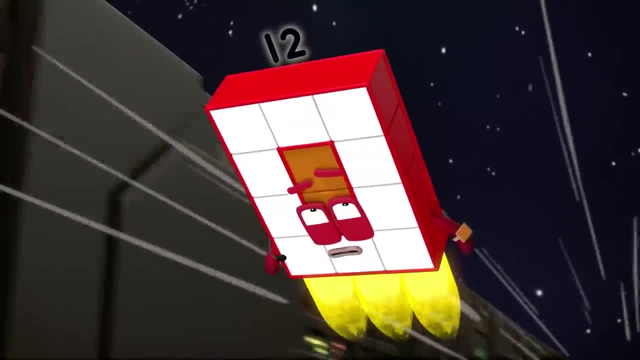 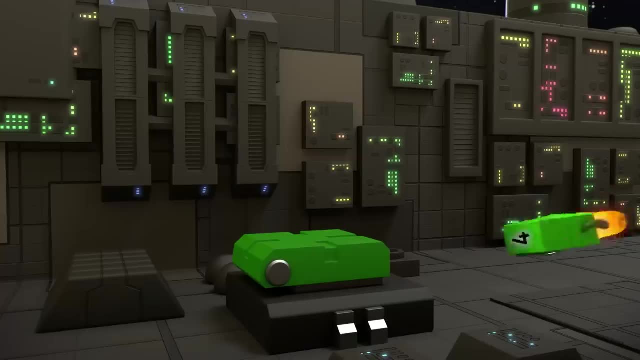 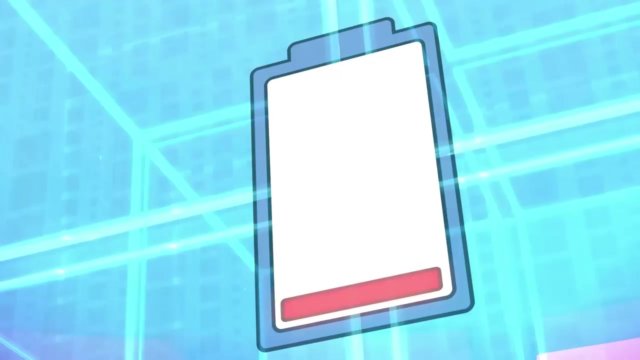 Phew, That's three different tasks, But I can do them all if I use the fours. This is it: Target approaching One, Two, Three, Re-arm. Ha-ha, Yeah, We did it. Oh, you did it. 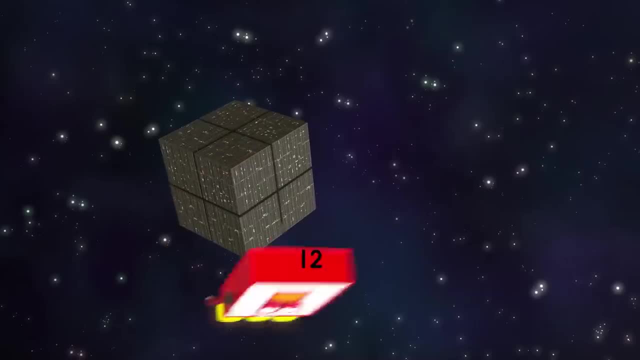 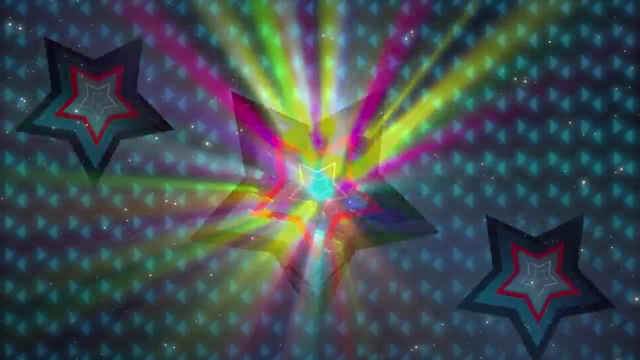 Now witness the power of this fully operational disco cube. Welcome back to Fifteen's Minute of Fame, the show where number blocks show you their tremendous talents. So far tonight we've seen Six and her bobbing number blocks One, two, three, triangle. 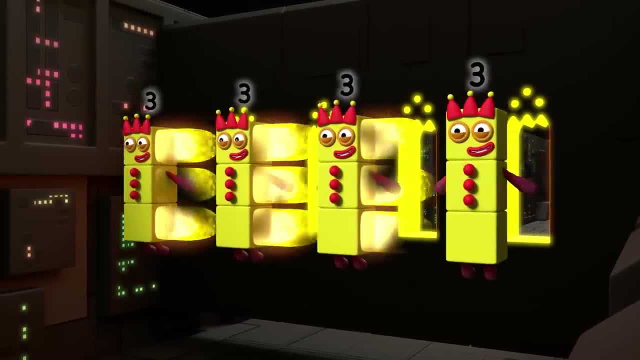 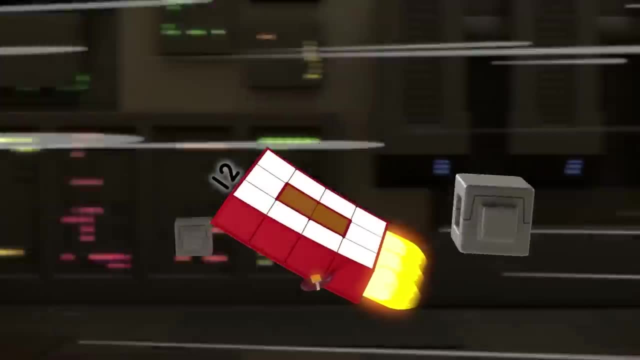 One, two Pop. please Can't Stop. Sorry, All right, now you can come in. By the way, what's your name? Come on out Where, Baby? Yeah, all that balls. we gotta make your way around the room. 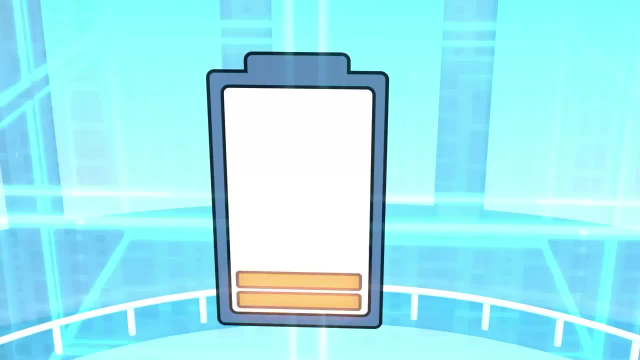 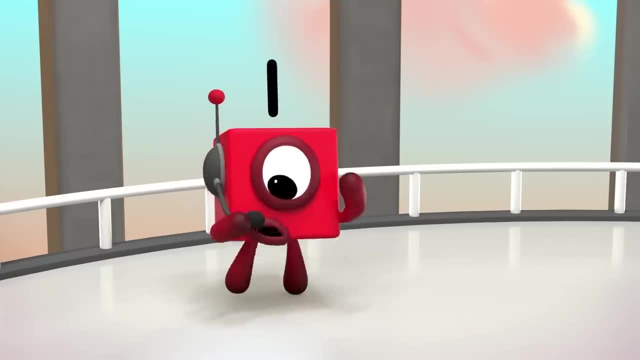 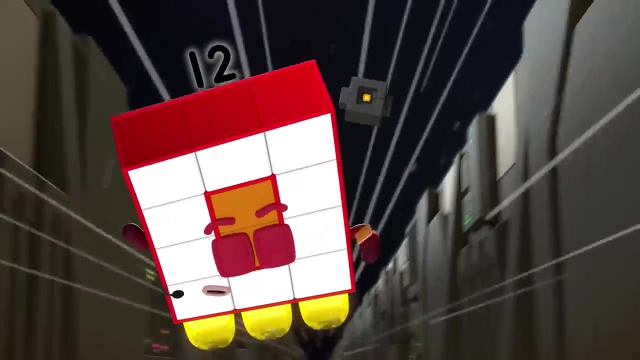 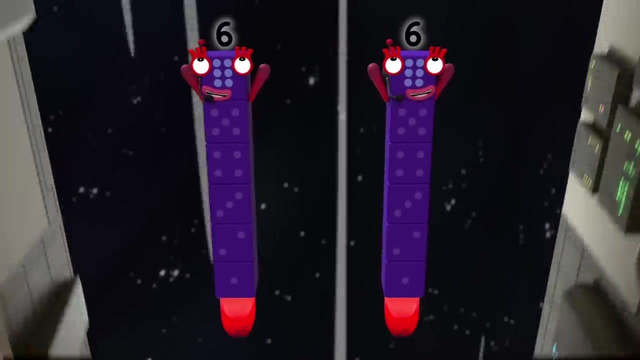 I wanna win. Yay, Those block ships have gone haywire. It must be the low battery. Don't let them slow you down. Wah, Woo-hoo, A latest play. I've got just the team Switch Two sixes. 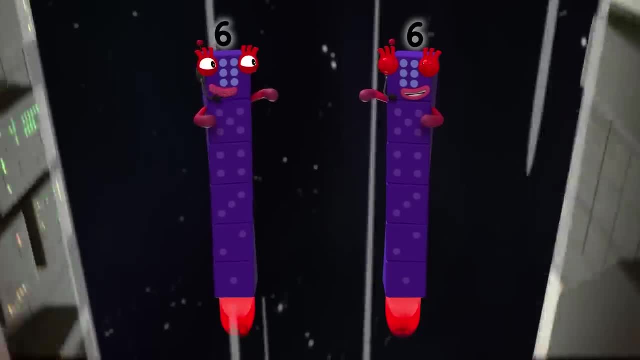 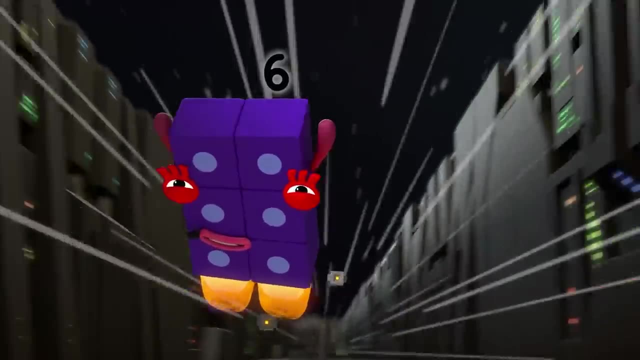 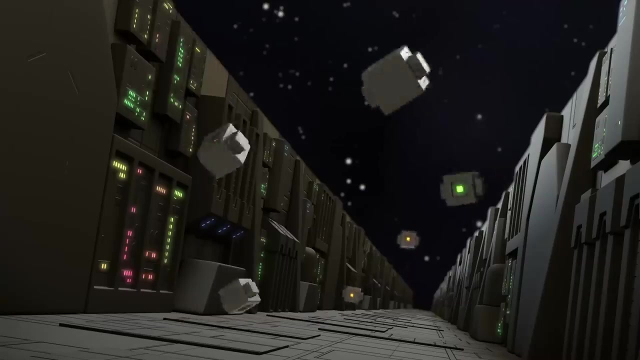 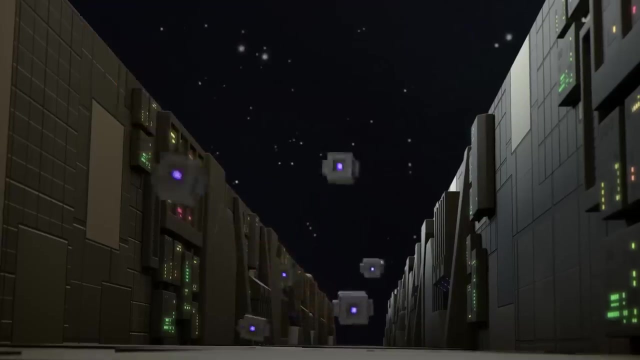 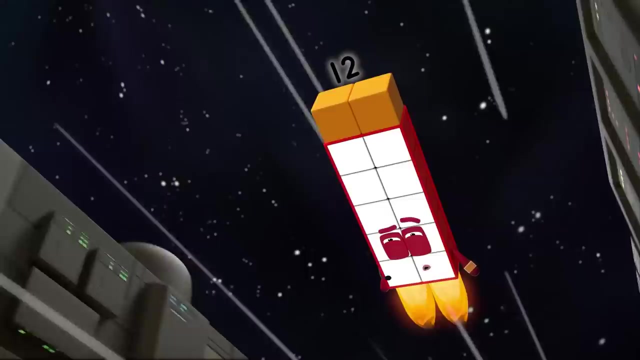 We've got a great escape technique: Let's play a game of hide and seek Switch. Catch me if you can. Ah, Whoa, I've got to lose them Through there. Oh, I've got a bad feeling about this. 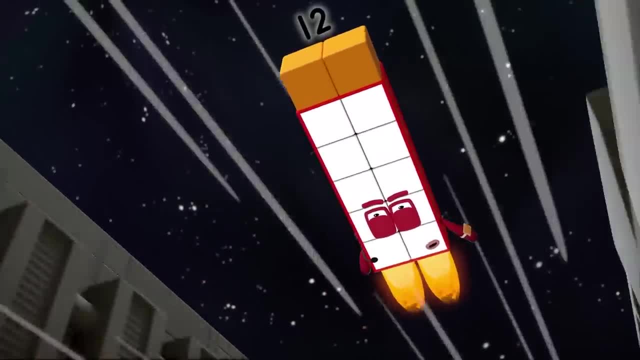 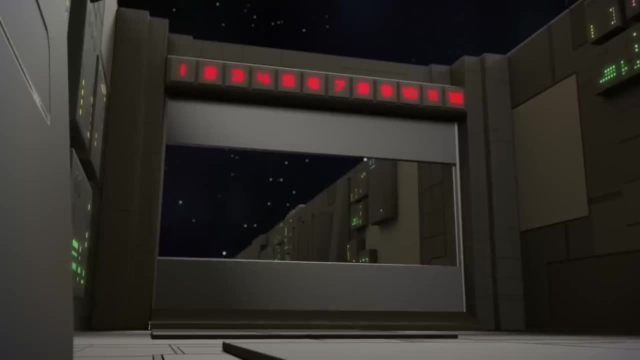 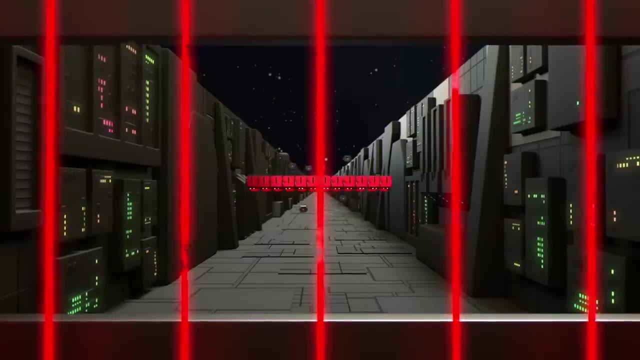 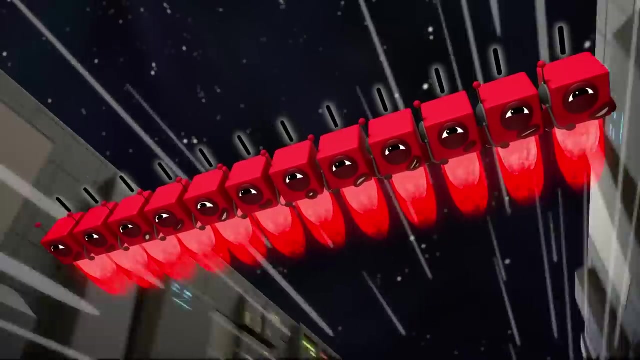 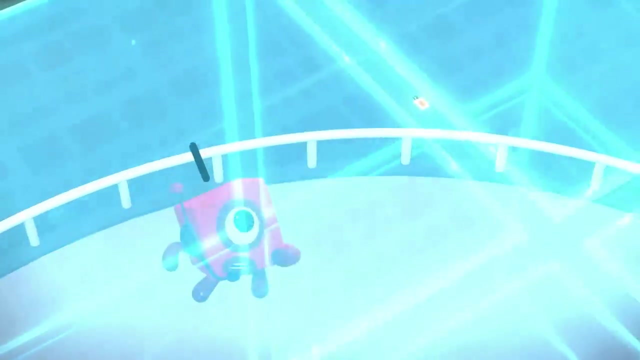 A racist play. Long and low, Switch, Wah, Look out. twelve, Twelve, what Phew Whoa? Battery level almost dead, but you're right on top of it. Switch, Switch, Switch, Switch, Switch, Switch. 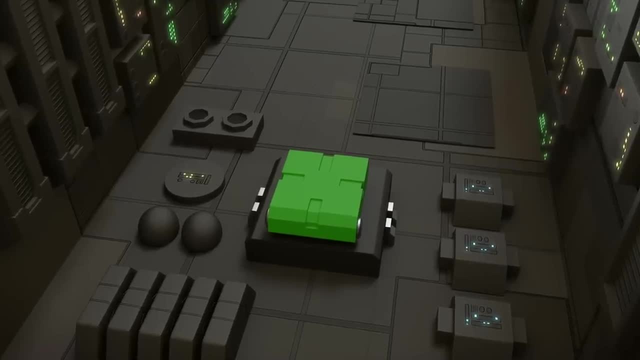 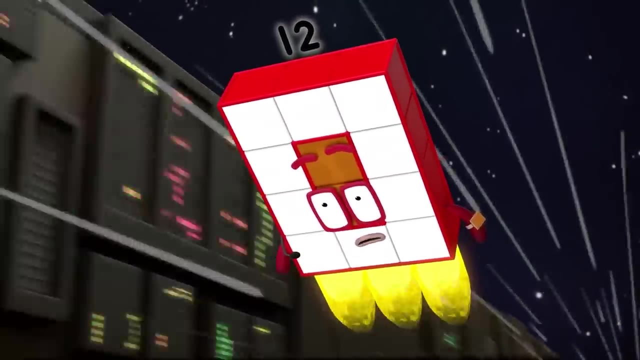 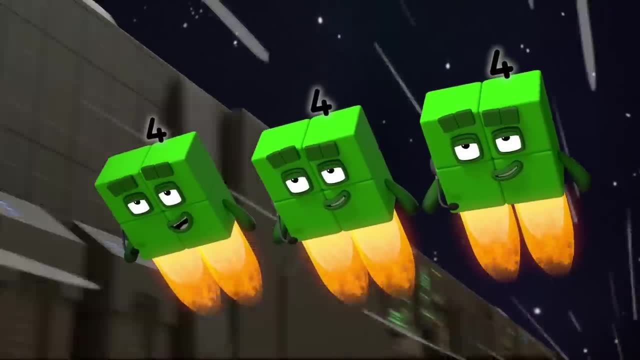 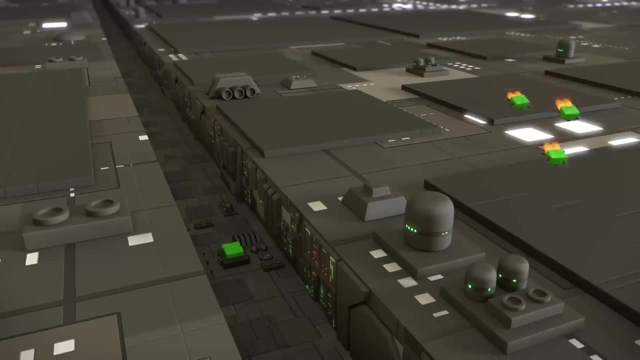 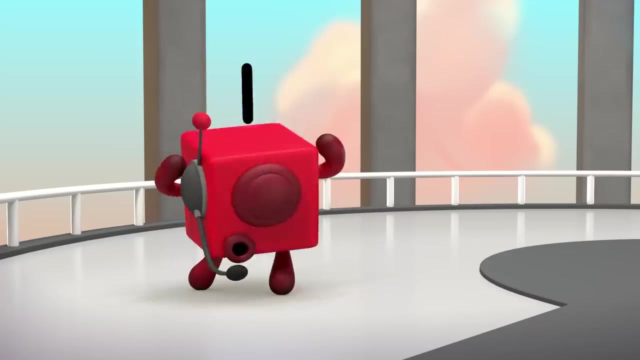 Use the fours. This is it Target, approaching One, Two, Three, Four. Stay armed, Stay armed, Ho ho Yay, Ho, ho, ho, Hoohoo Yay. You did it. Now witness the power of this fully-operational disco cube. 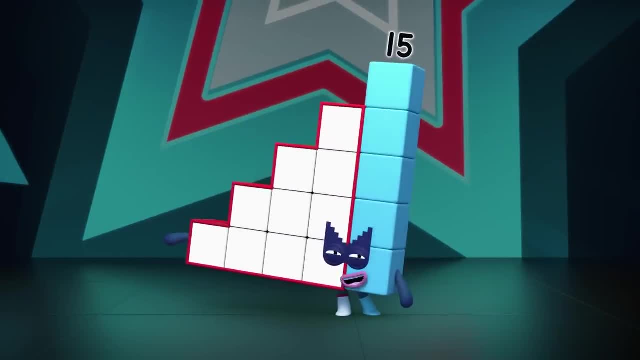 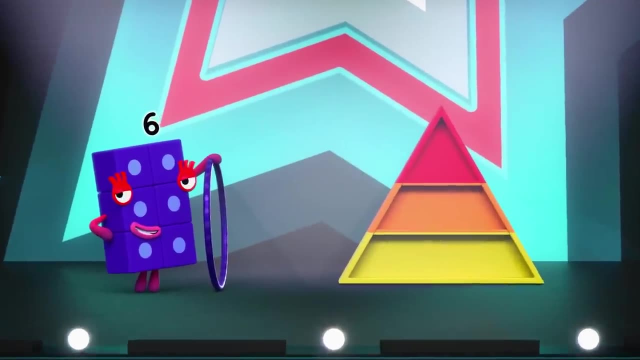 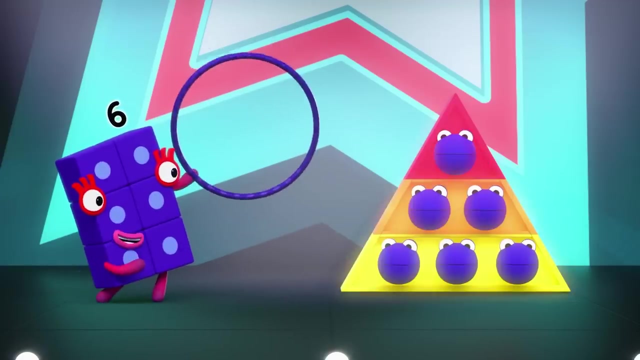 Welcome back to 15's Minute of Fame, the show where number blocks show you their tremendous talents. So far tonight we've seen Six and her bobbing number blocks One, two, three, triangle, Four, five, six, triangle. 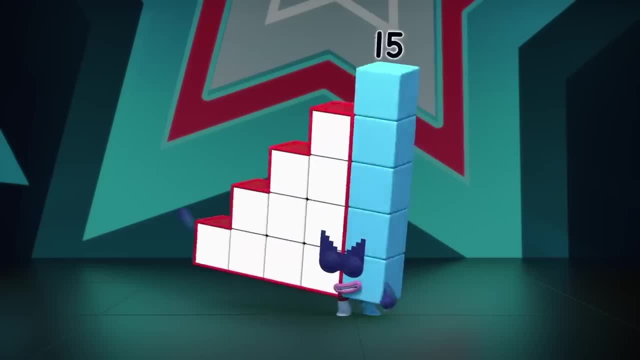 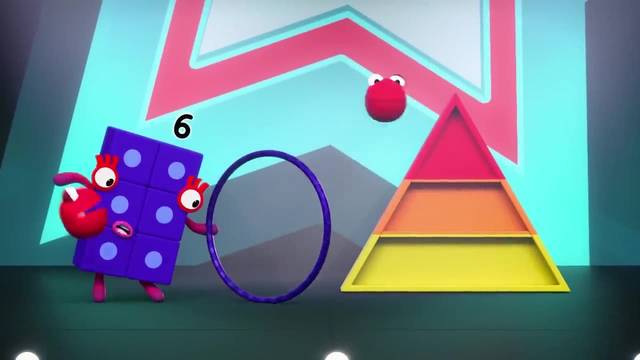 Four, five six triangle: Yay. And now the number blocks: One, two, three triangle. Four five six triangle: Yay. One, two, three triangle Four five six triangle. 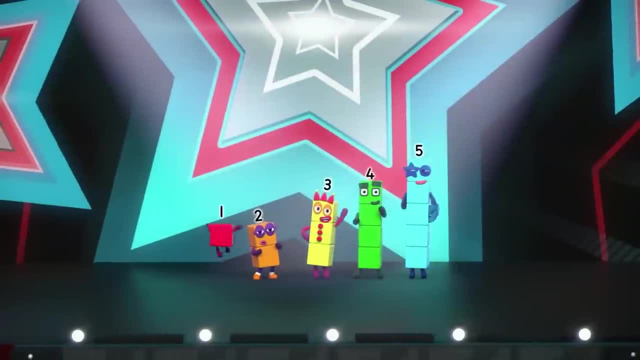 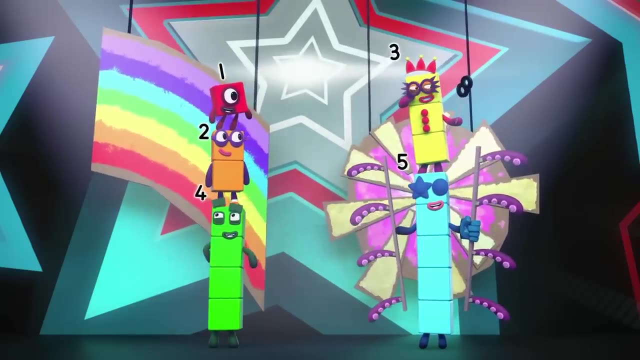 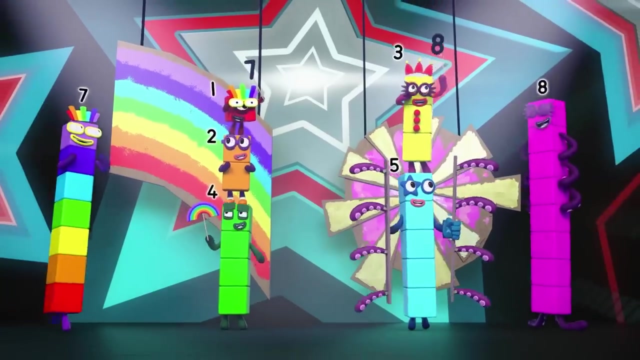 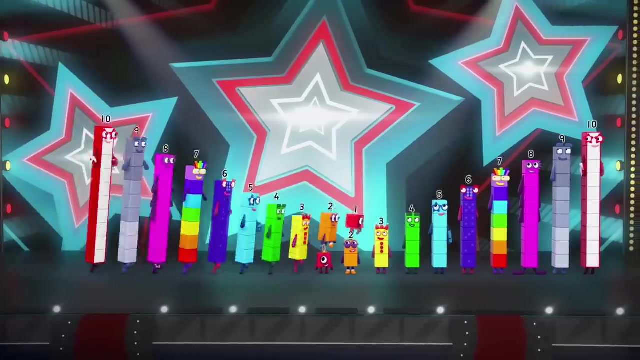 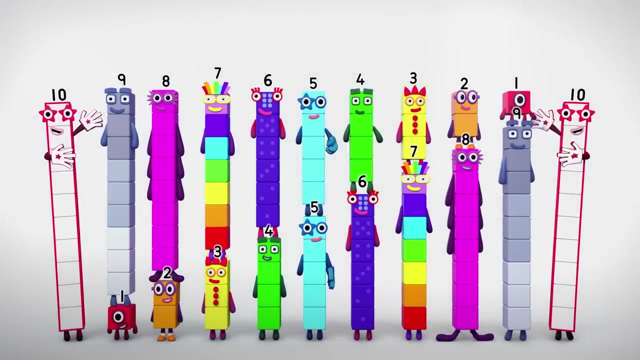 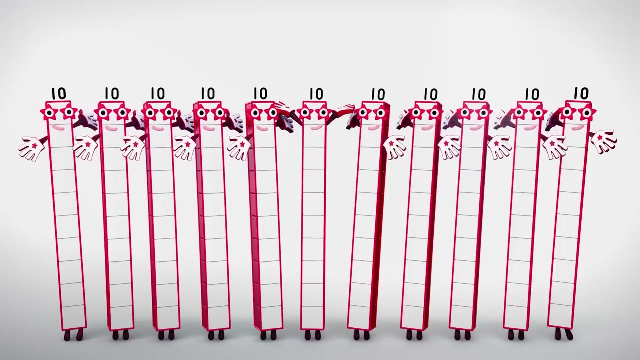 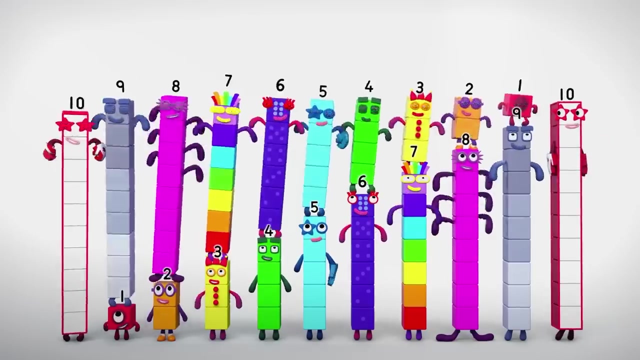 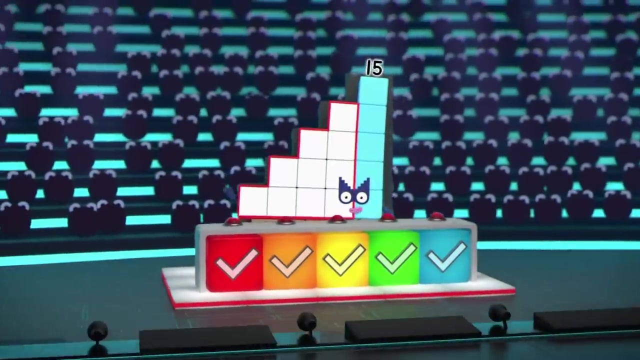 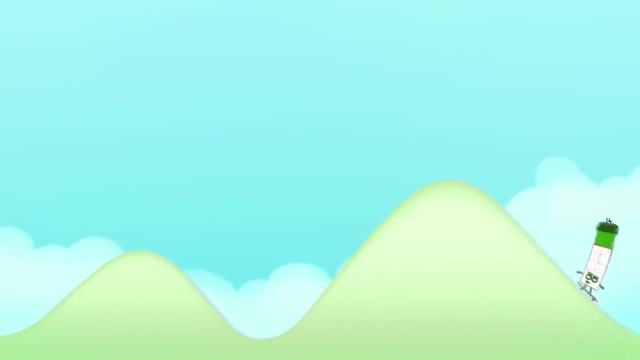 Yay. Impressive impressions, Octoblock to the rescue- Oh, that's lucky. Oops, Ooh, And mystical magic acts. Now it's time to see what some of our bigger numbers have in store. For as long as I can remember, I've always wanted to skate. 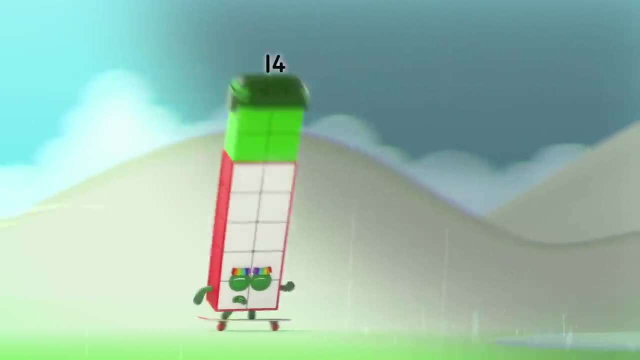 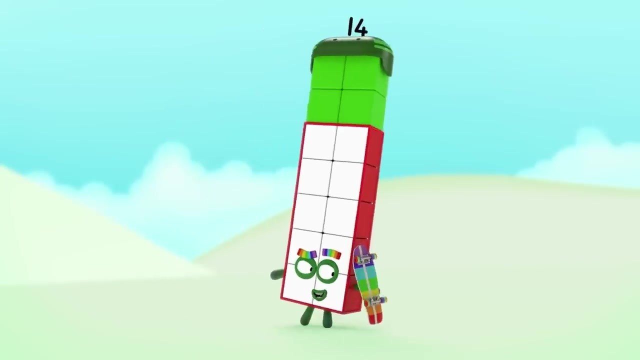 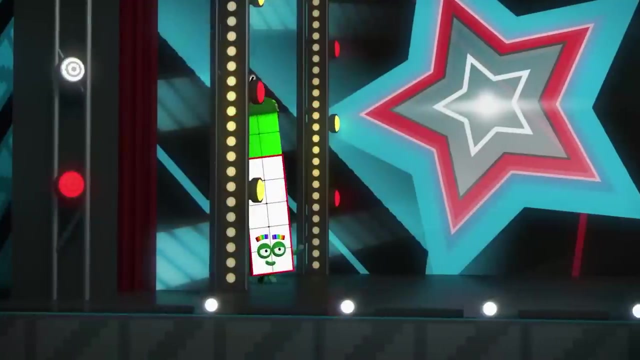 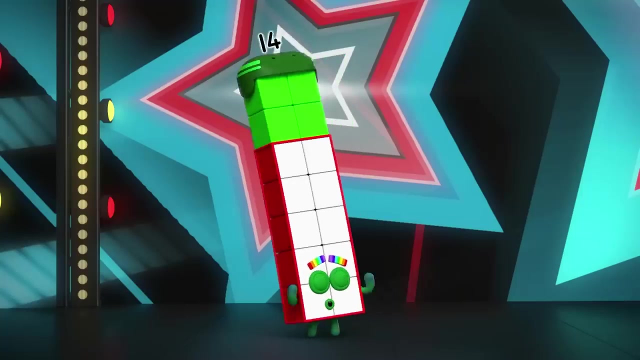 In wind, rain and snow, No matter how gnarly it gets. I put in the hours, Cos. practice makes perfect. Welcome to 15's Minute of Fame. Show us what you've got 14. No problemo, but I need a volunteer for this trick. 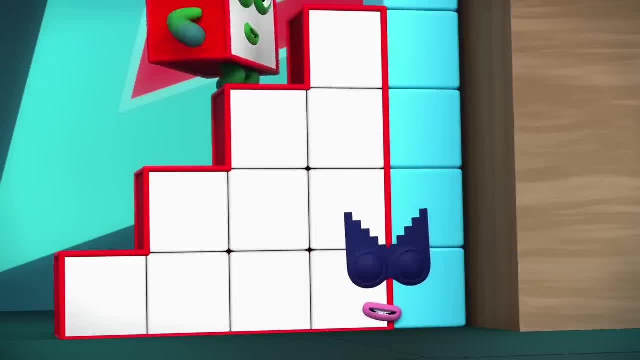 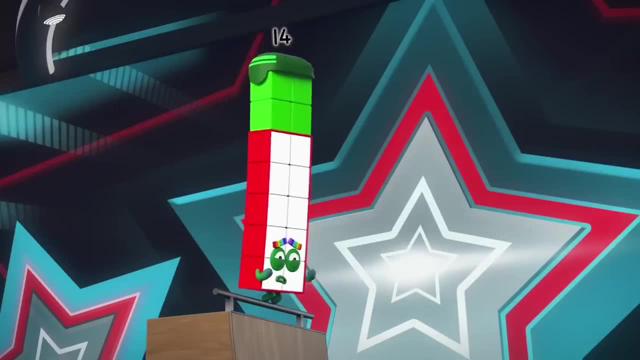 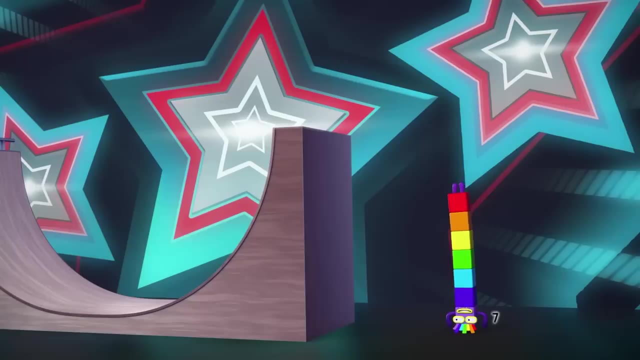 15. No, no, I'm not the act he is, I'm just helping him take it to the next level. 14. Oh no, I forgot my skateboard. Whoa, Wow, Yep, that was lucky, double lucky. 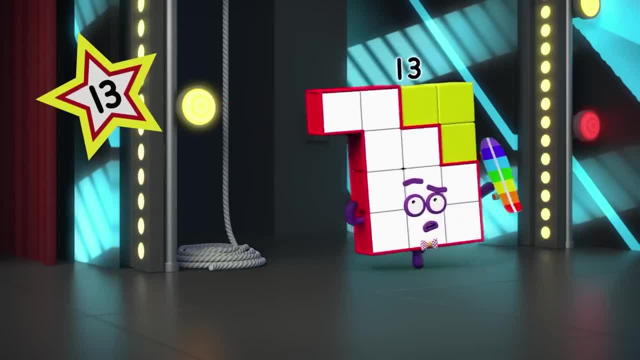 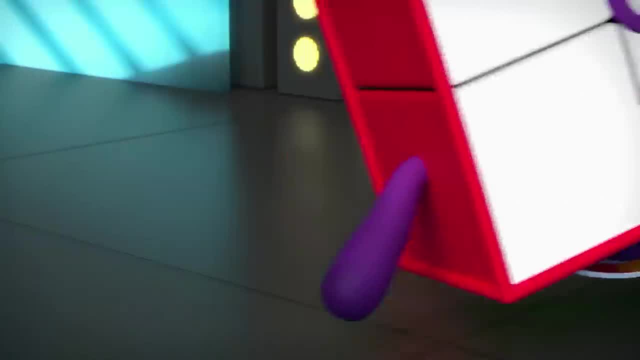 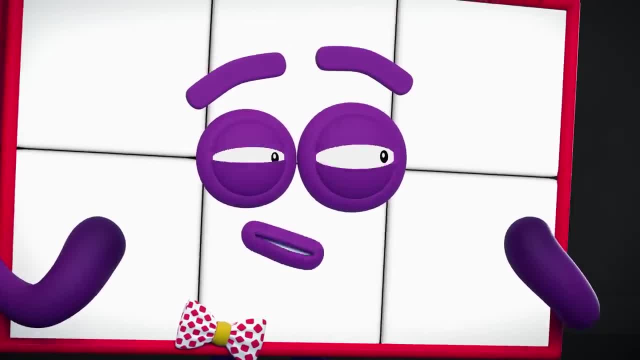 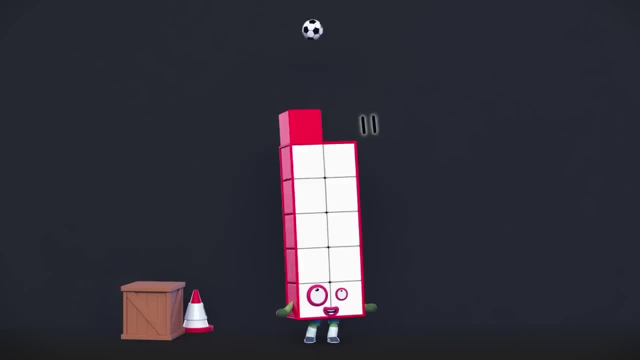 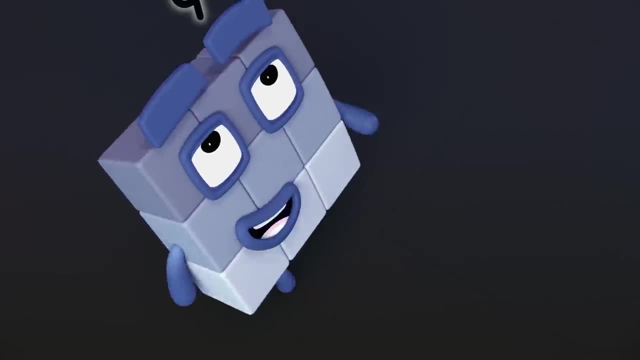 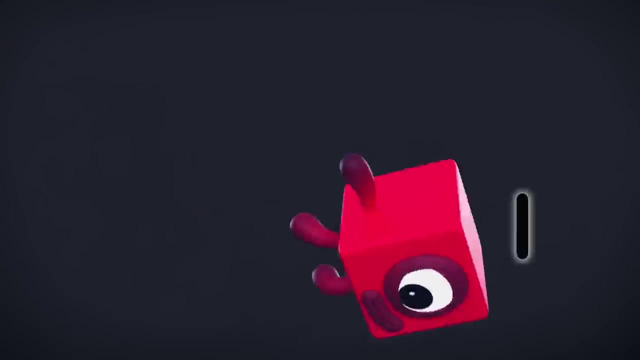 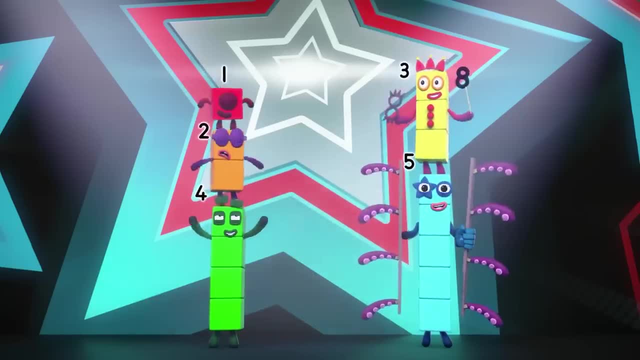 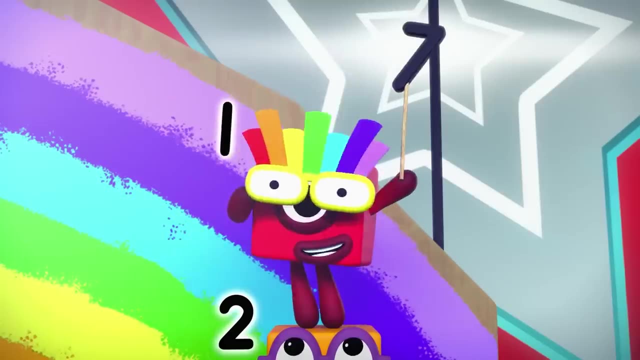 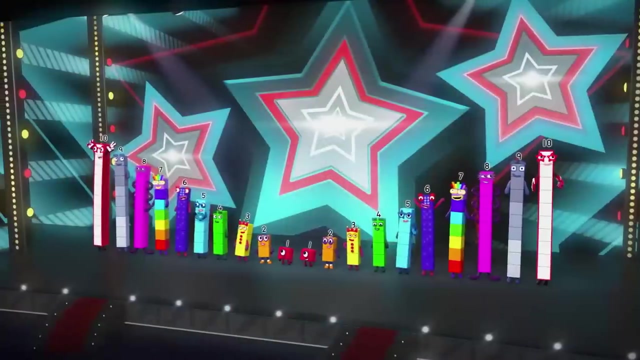 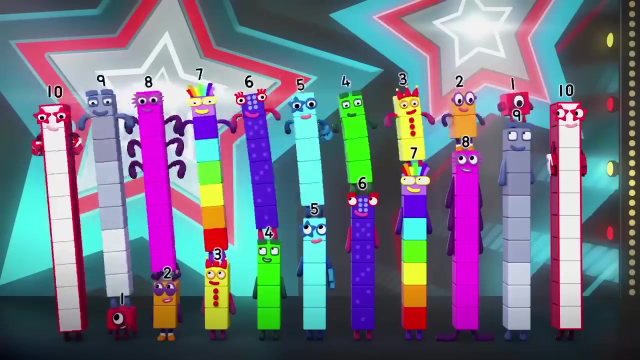 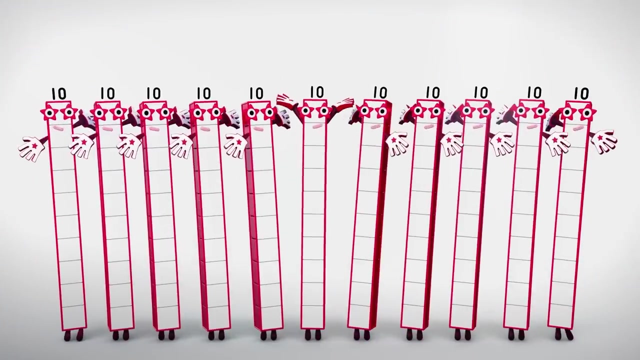 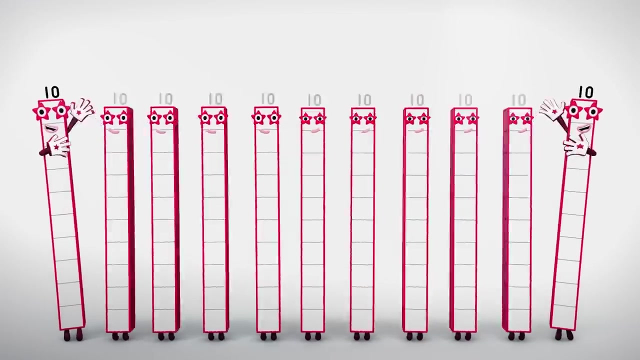 Impressive impressions. Octoblock to the rescue- Oh, that's lovely. Oops And mystical magic acts. Let's make her big again. Vroom, vroom, vroom. Numbraillcadabra 11 tenths. 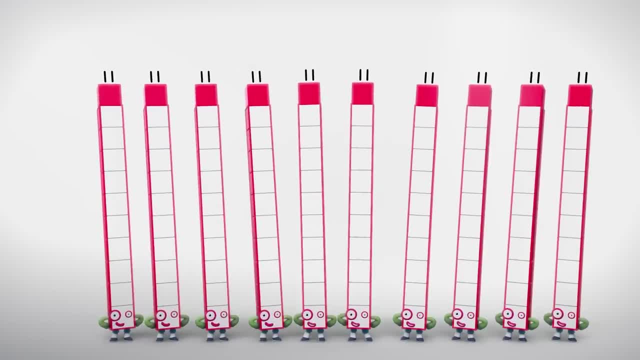 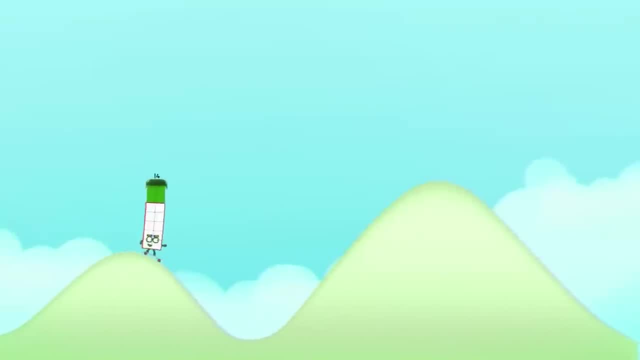 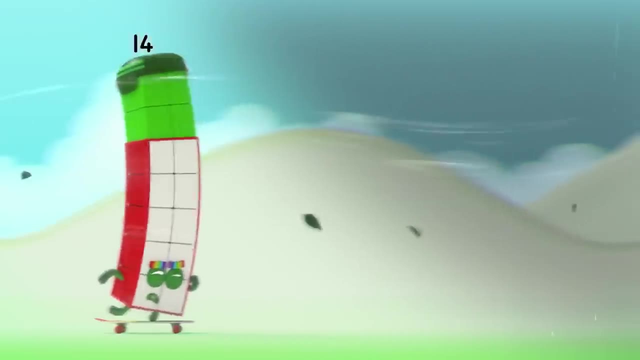 Vroom. Vroom Numbraillcadabra: Nope 7-11! Numbraillcadabra 7-11! ba-tient. As long as I can remember, I've always wanted to skate in wind, rain and snow. 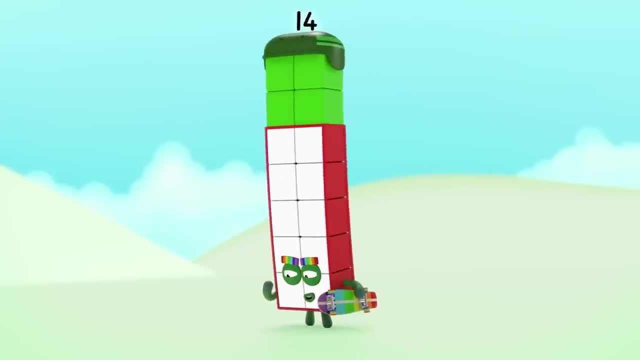 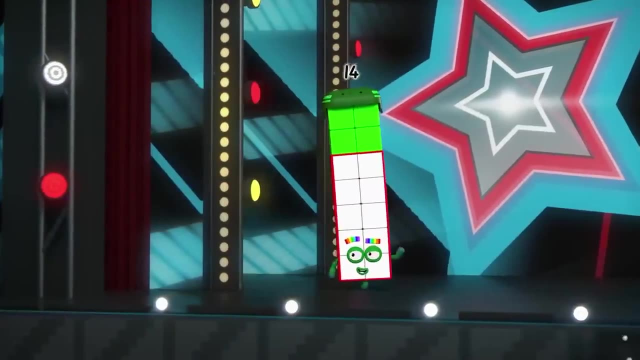 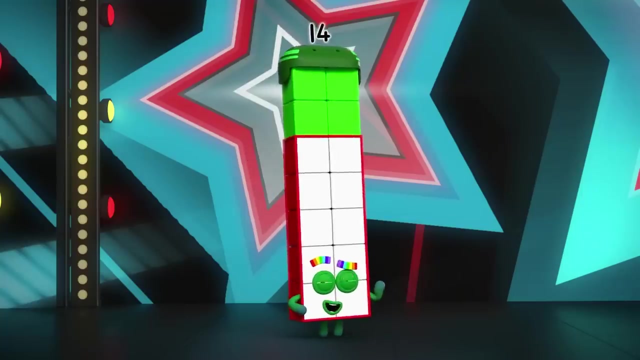 No matter how gnarly it gets. I put in the hours, cos practice makes perfect. Welcome to Fifteen's Minute of Fame. Show us what you've got. Fourteen, No problemo, But I need a volunteer for this trick. 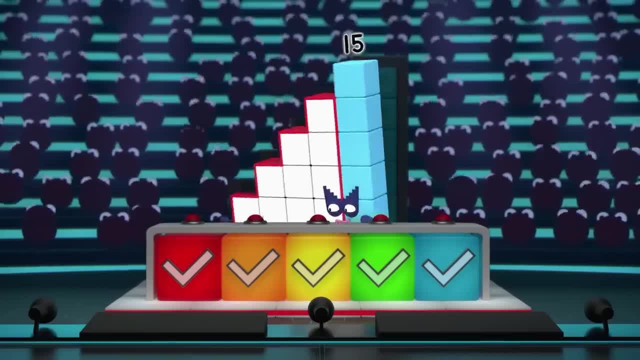 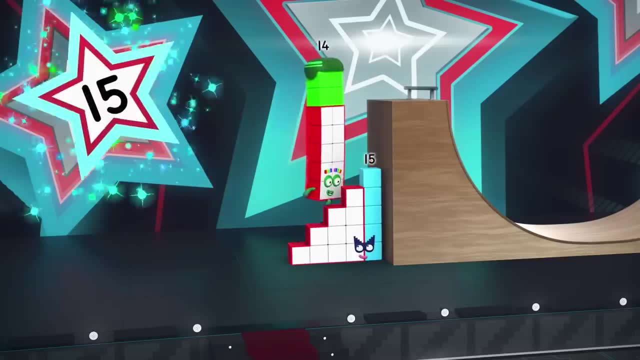 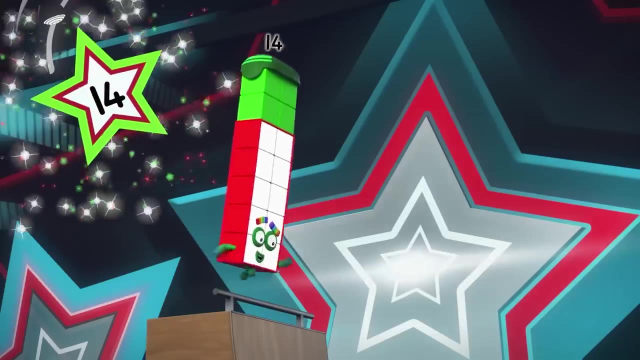 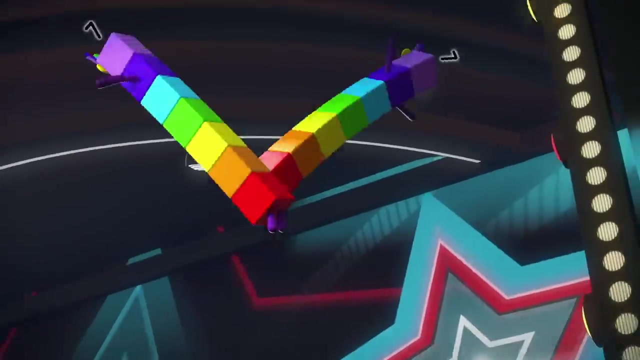 Fifteen: No, no, I'm not the act he is, I'm just helping him take it to the next level. Fourteen: Oh no, I forgot my skateboard. Whoa, Whoa, Whoa, Whoa. 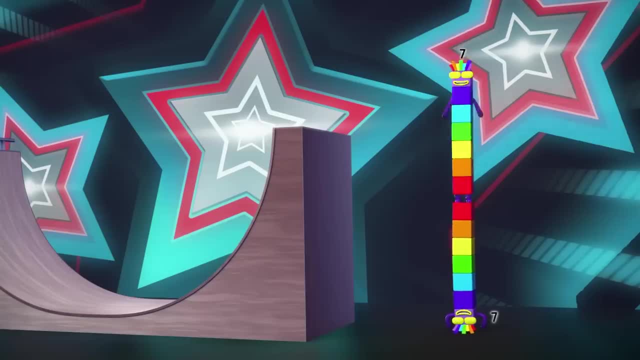 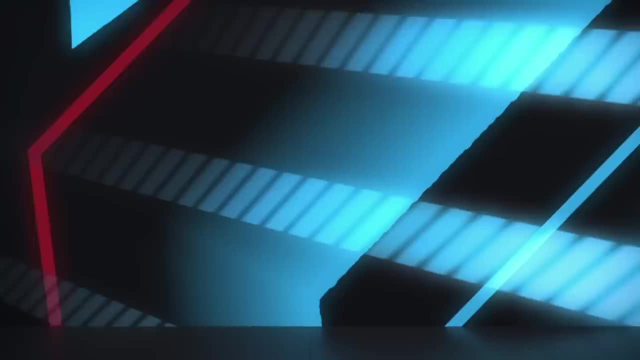 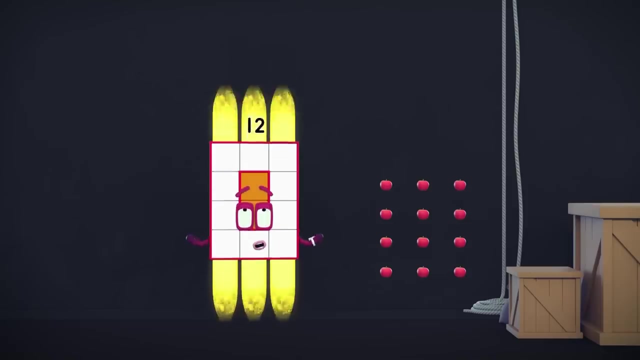 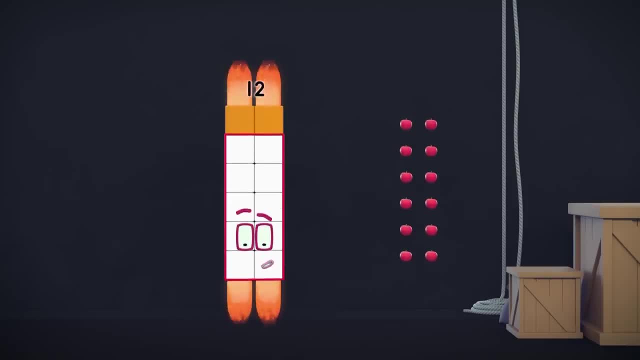 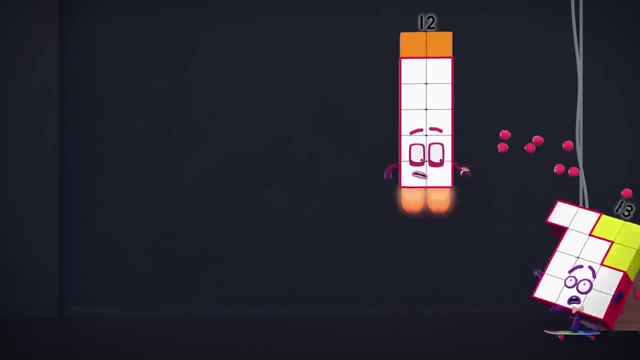 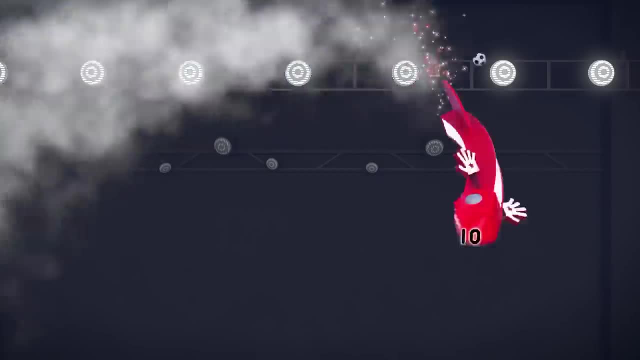 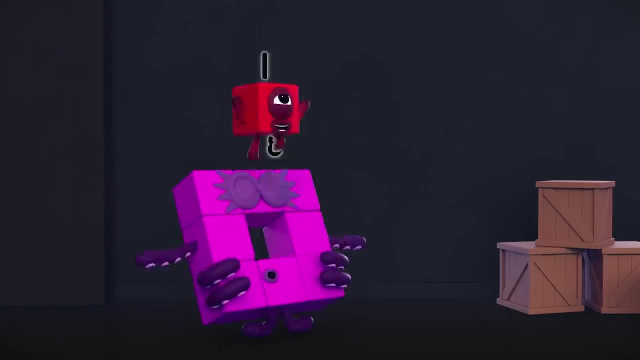 Nine, Achoo, Oh, my Eight Octoblock, Pirouette One, two, three, four, five, six, seven, eight. Pirouette Oh, Seven, Oh, Oh, Oh Oh. 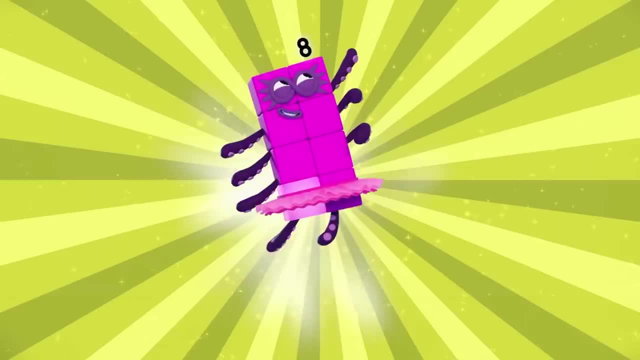 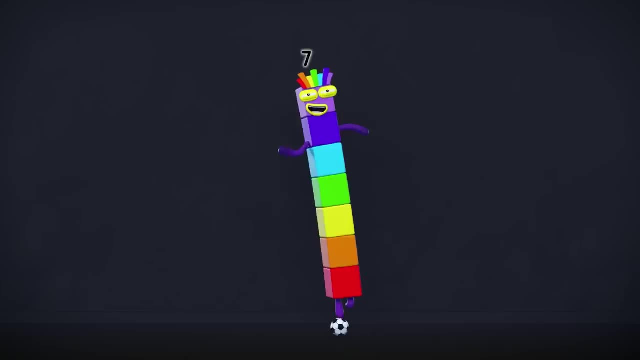 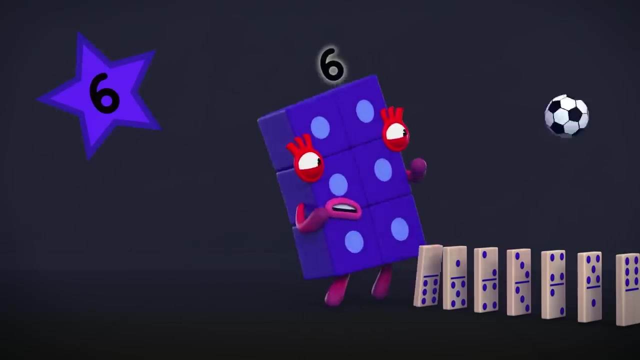 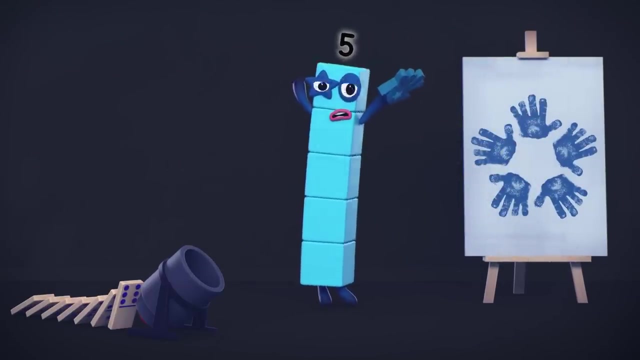 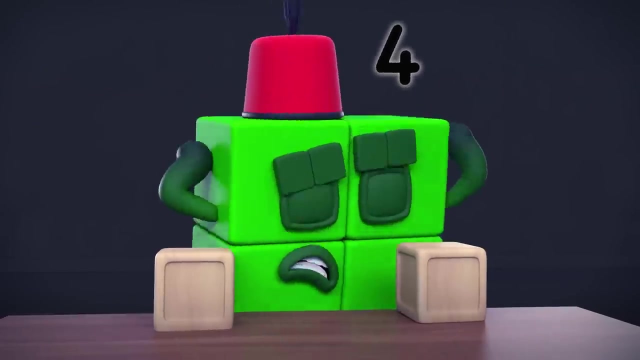 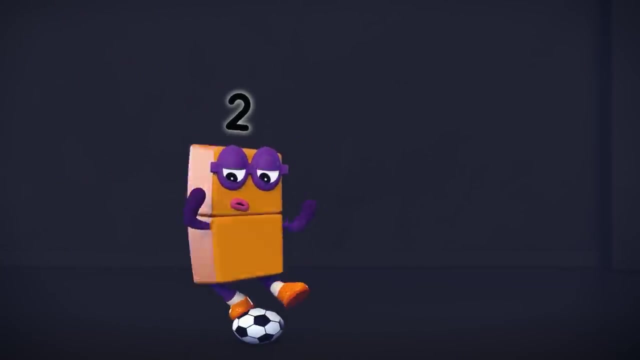 9! airs A-chooo, Ah, Ah, Lucky me. Six, Five, Four, Screw, screw Round thing Three. Look at me. Two, One oops, Two, oops, One oops. 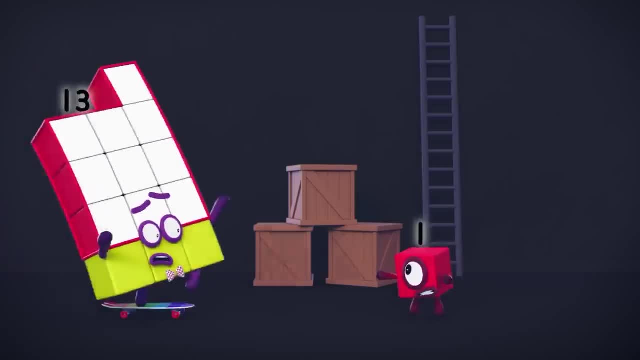 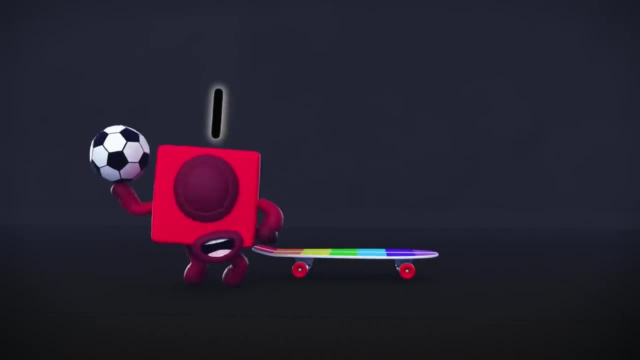 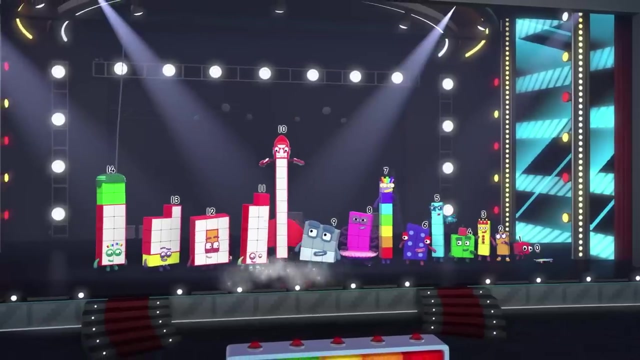 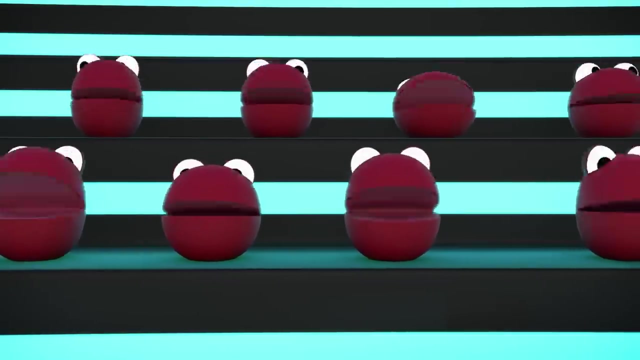 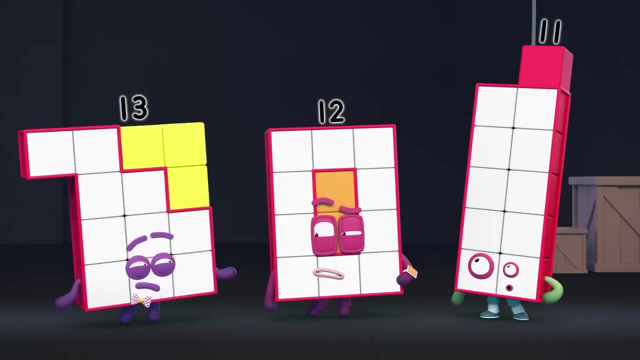 Two, oops, One Ta-da. Anyone lost a football Or a skateboard. Zero, Nothing to it. Ha-ha. Oh, a beauty, A beauty, Yay, Hooray, That is made of that, Ah-tush. 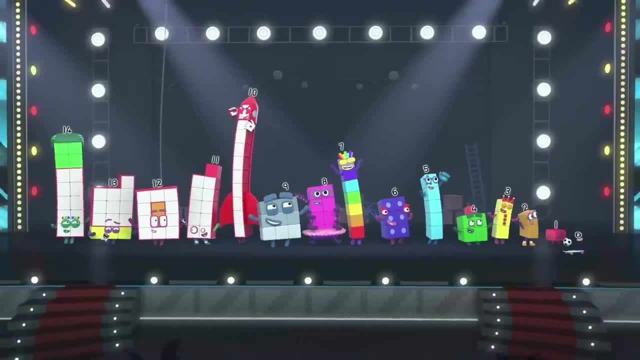 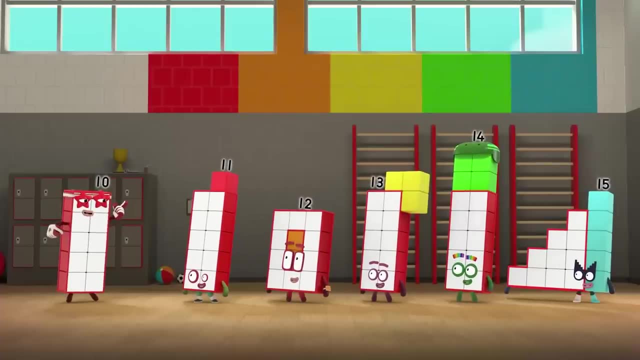 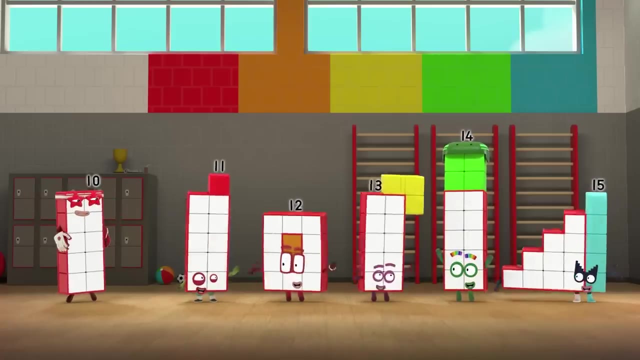 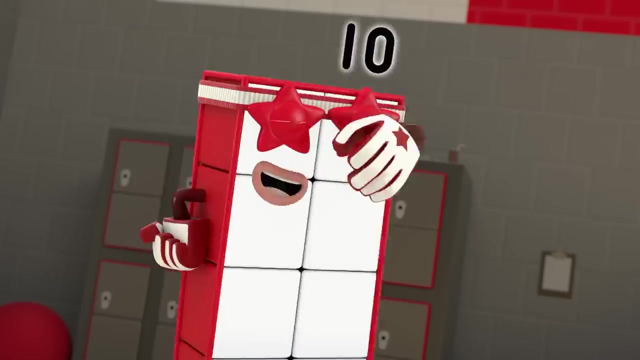 Everyone's a winner. Yay, Welcome to Ten's Place. All of you are bigger than me. That means each of you has a ten inside. you See, You are greater than ten Subtitles by SteamTeamExtra and you've got big dreams. you want fun? well, fun it is. right. now is where you start playing. 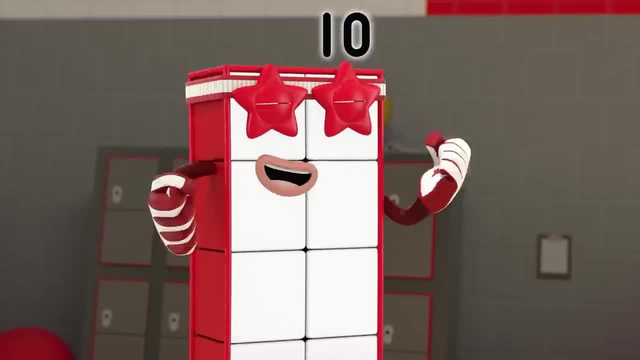 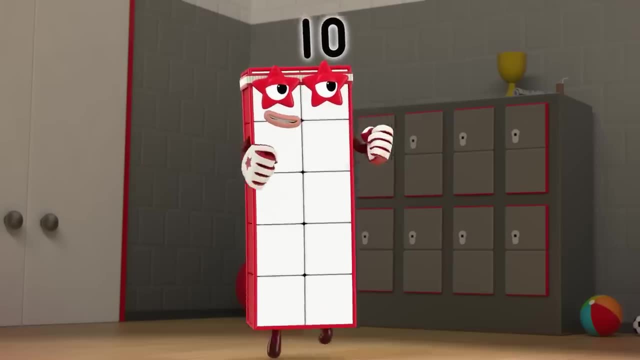 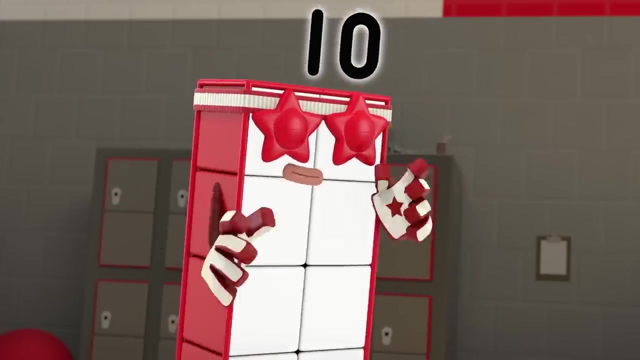 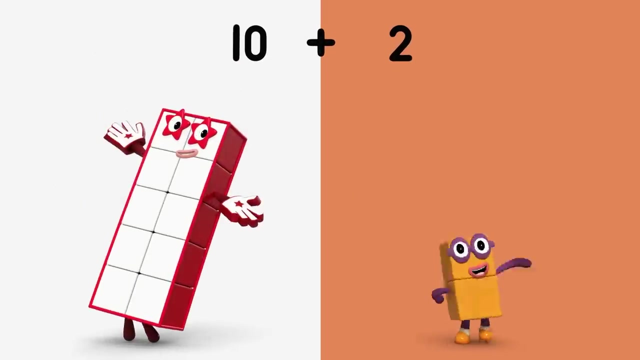 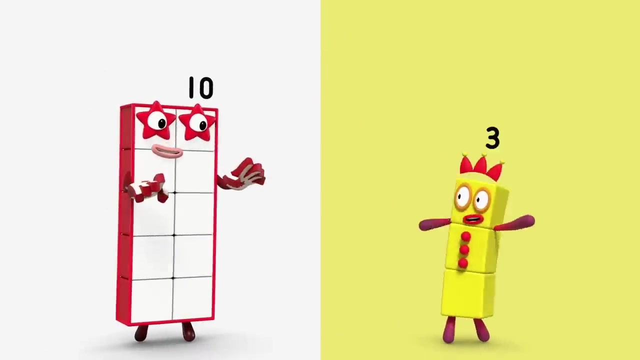 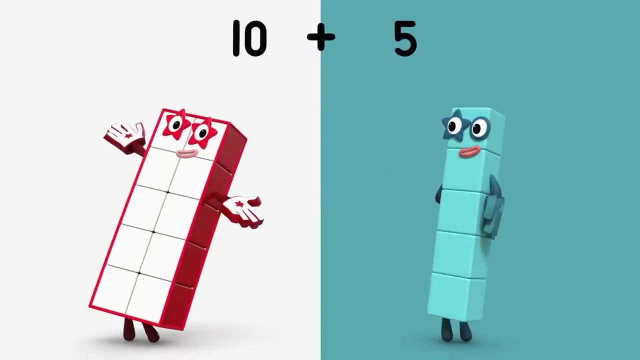 that's right now. give me some squats. let me see you do the jump and bump. 10 plus 1 is 11, 10 plus 2 is 12, 10 plus 3 is 13, 10 plus 4 is 14, 10 plus 5 is 15. 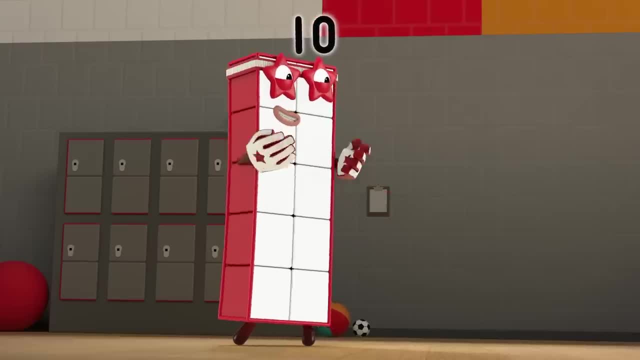 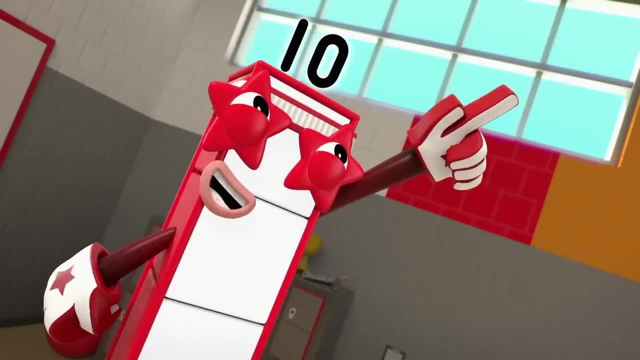 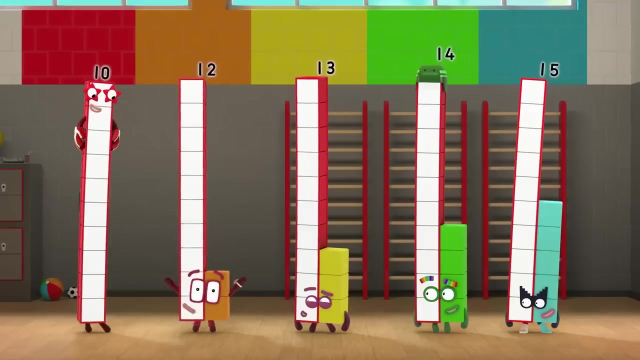 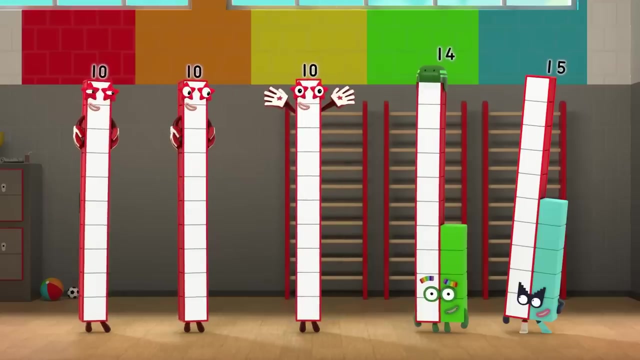 terrific. now let's stretch our 10s, nice and tall, bling those ones high in the air. take it away: 11 minus 1 is 10, 12. minus 2 is 10. 13 minus 3 is 10, 14.. minus 4 is 10. 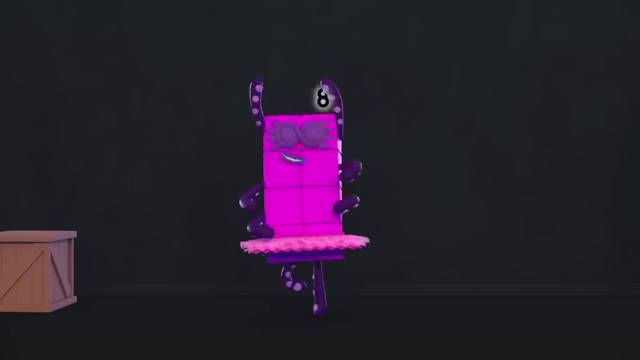 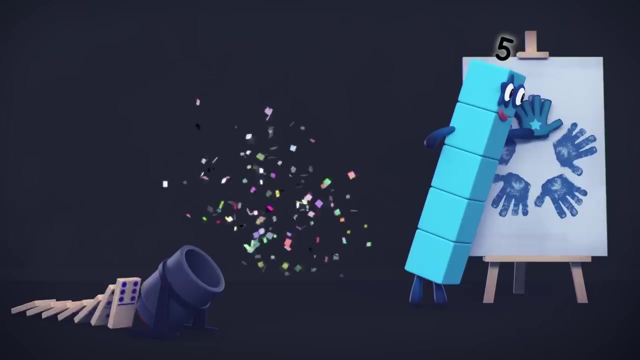 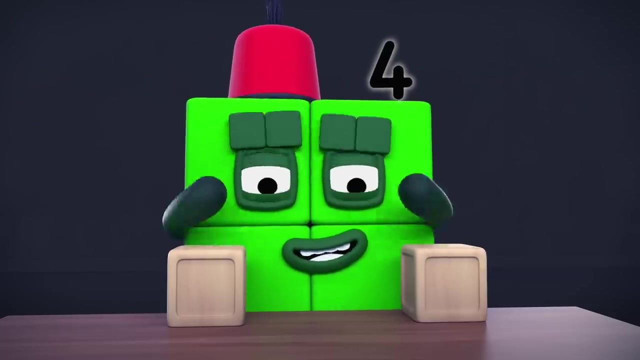 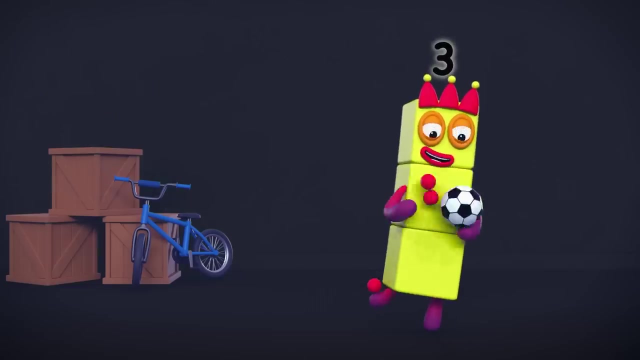 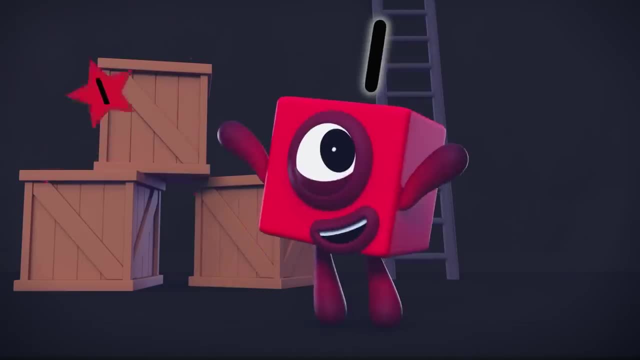 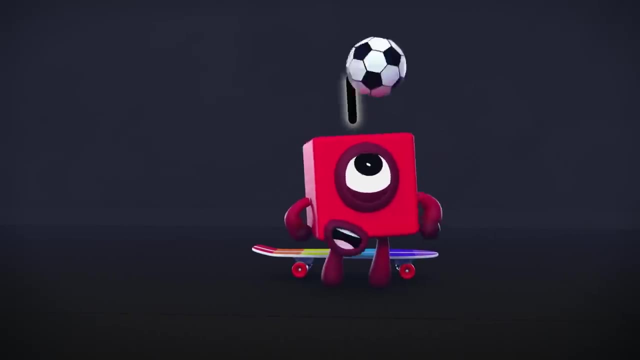 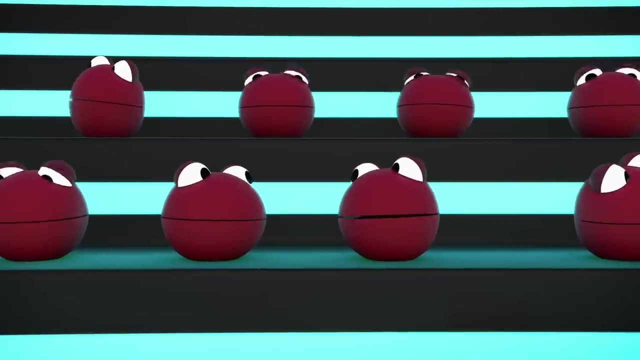 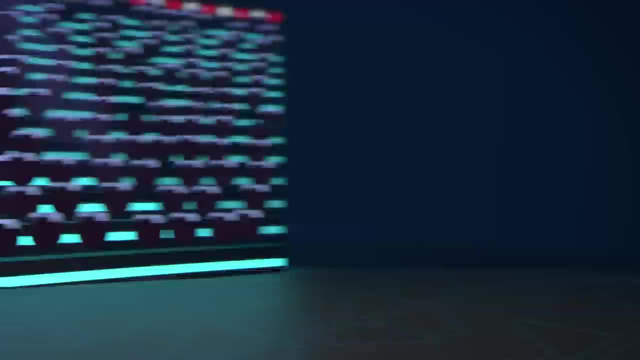 One ups, Two ups. Anyone lost a football Or a skateboard. Zero, Nothing to it. Yay Hooray. Let's see what our judges made of that. Oh, Oh, Oh Oh. What is made of that? 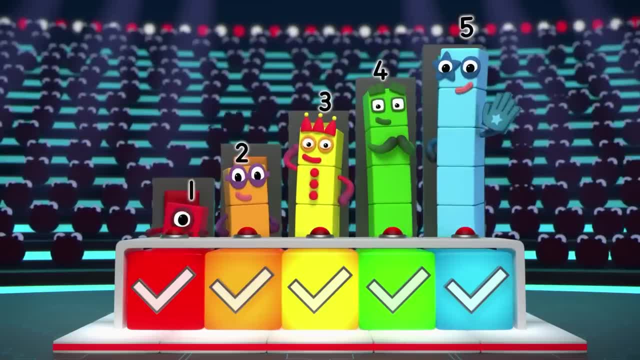 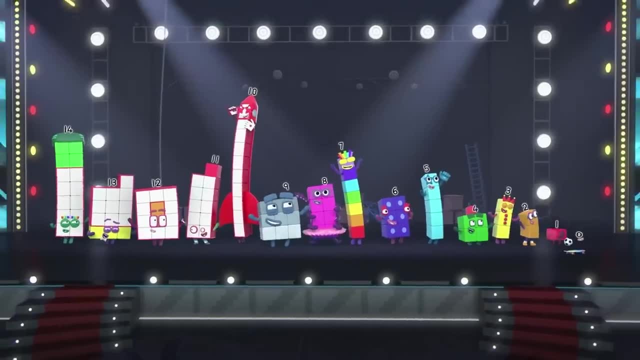 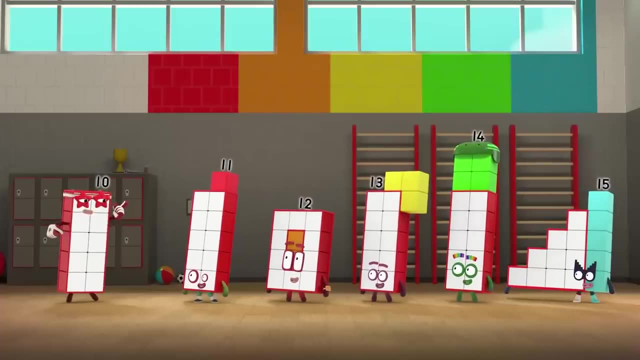 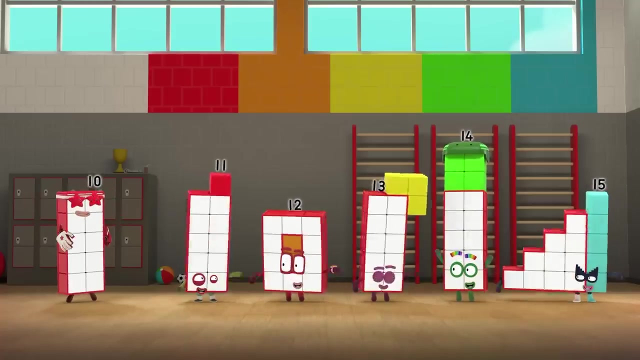 Hush-hush, Everyone's a winner. Yay, Welcome to Ten's Place. All of you are bigger than me. That means each of you has a ten inside you. You see, You are greater than Ten. Oh, And you've got big dreams. 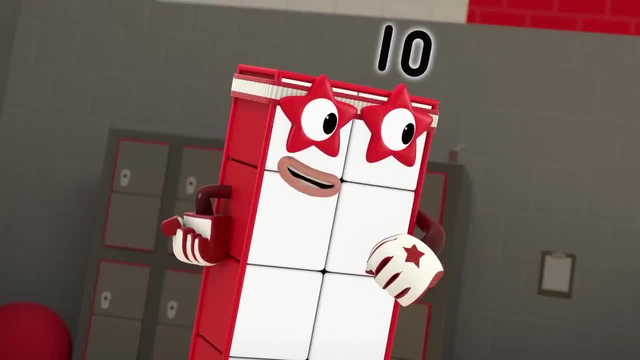 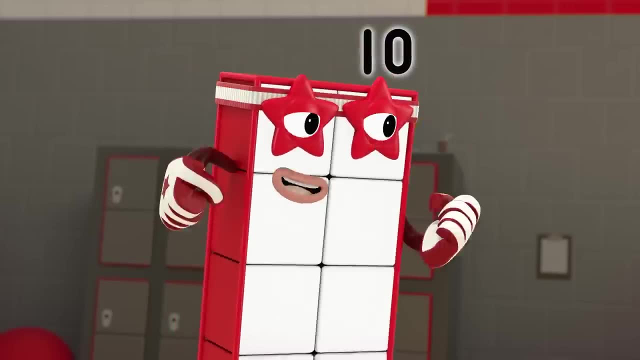 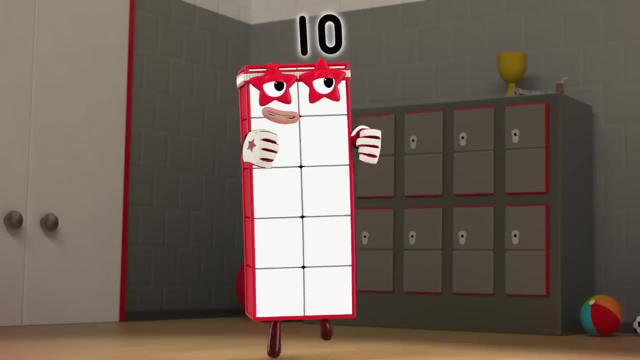 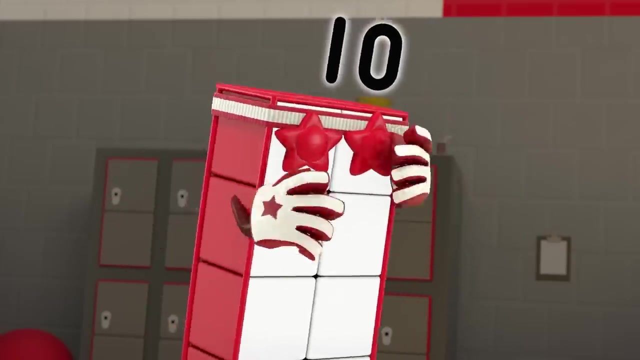 You want fun? Well, fun it is. And right now is where you start playing Wow. OK, let's pump those numbers. That's right Now. give me some squats. Let me see you do the jump and bump. 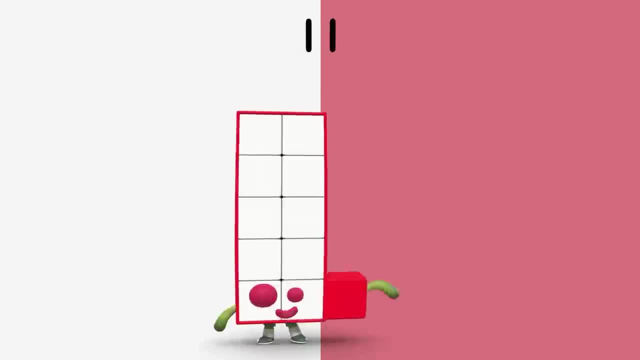 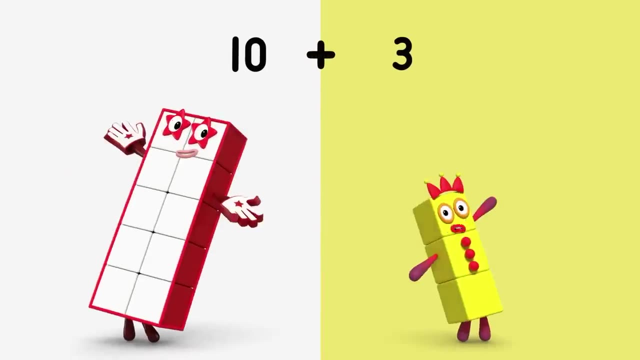 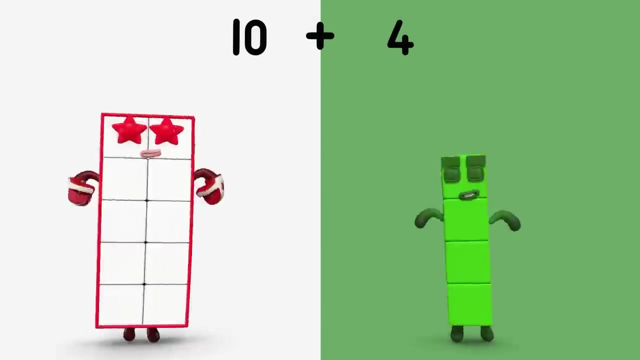 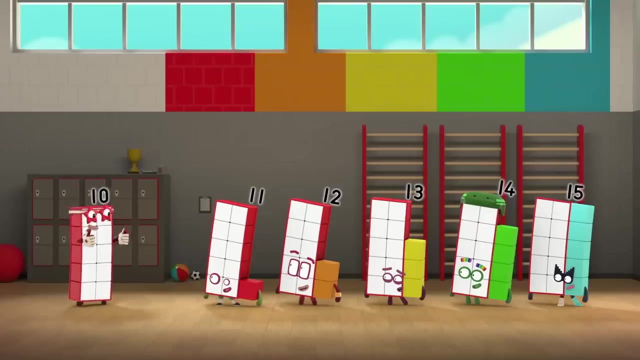 Ten plus one is eleven. Ten plus two is twelve. Ten plus three is thirteen. Hooray, Ten plus four is fourteen. Ten plus five is fifteen. Terrific, Now let's stretch our tens. Nice and tall Hoop. 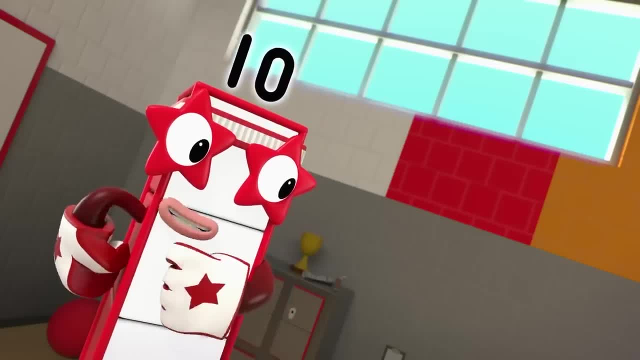 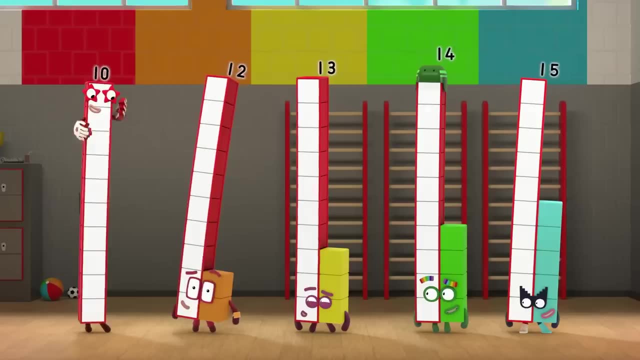 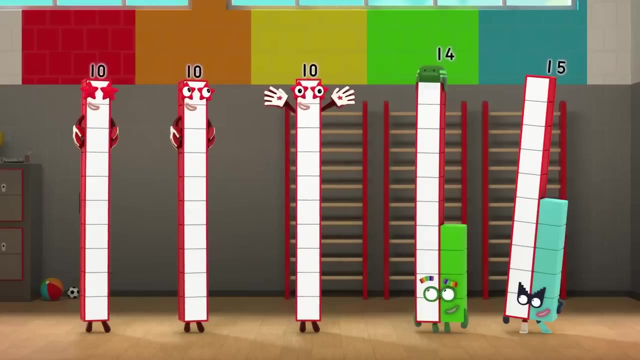 Hoop, Hoop, Hoop. Blink those ones high in the air. Take it away. Eleven Minus one Is ten Twelve. Minus two Is ten Thirteen. Minus three is ten Fourteen. 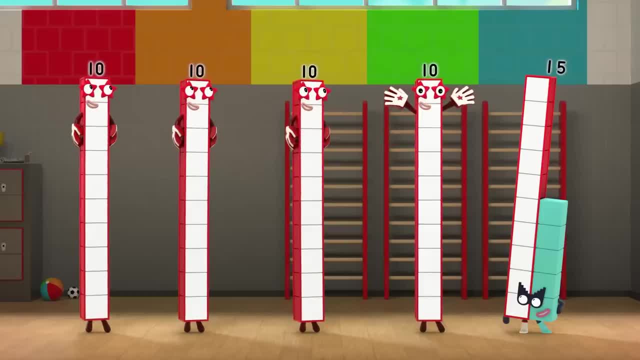 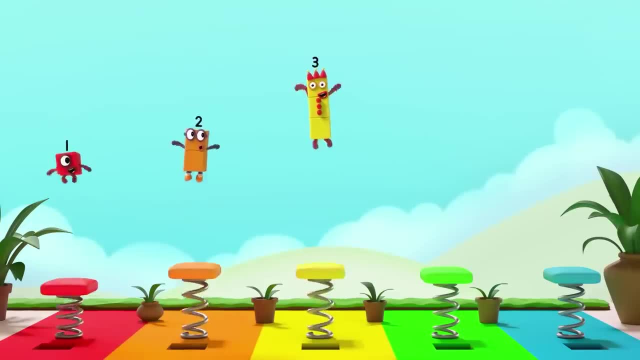 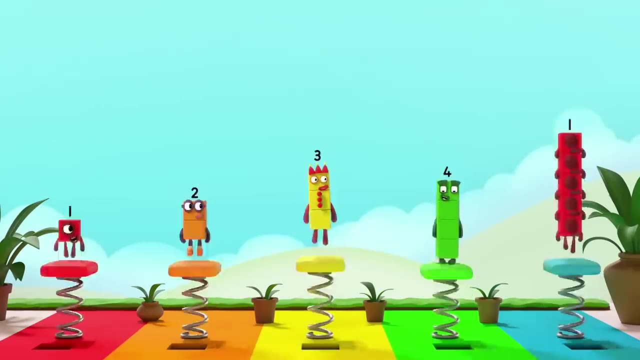 Minus four Is ten. Fifteen Minus five is ten. Bye-wee, Bye-wo, Bye-wo, Boing, boing, boing, boing, boing, boing. One, two ones, three ones, four ones, five ones. 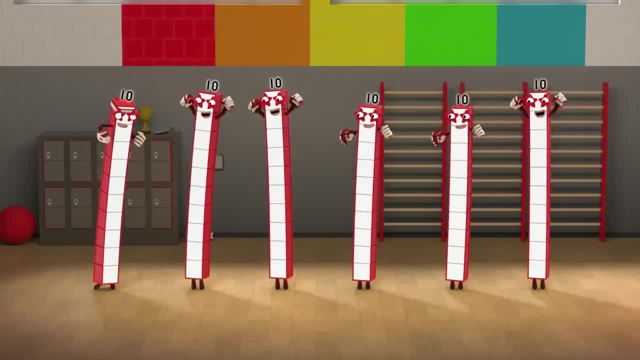 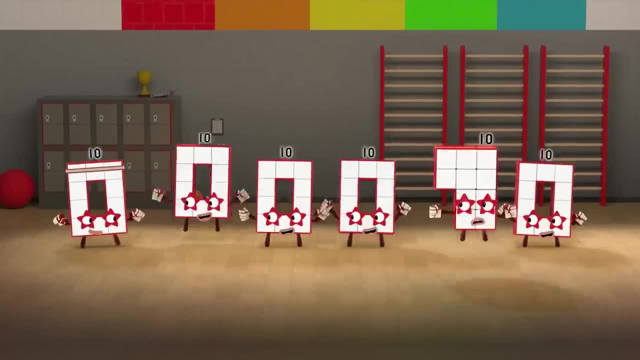 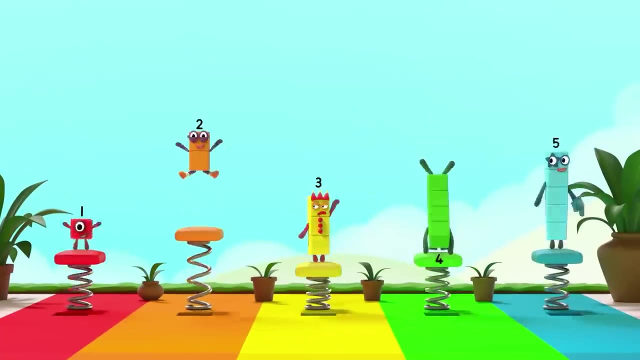 Ready, Let's work those tens. Yeah, Tall slide, two eyes Slide and go low rectangle with a hole And freestyle. Yeah, Ha, ha, ha, ha, ha ha. Boing, boing, boing, boing, boing, boing. 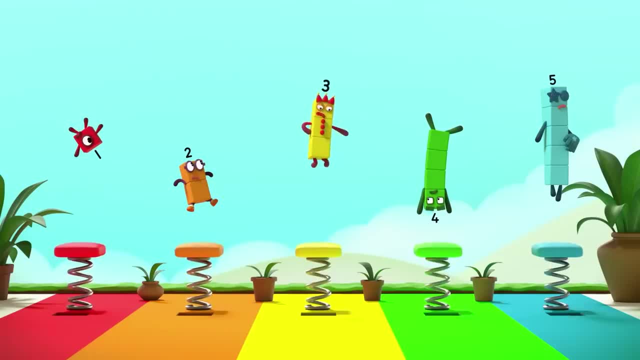 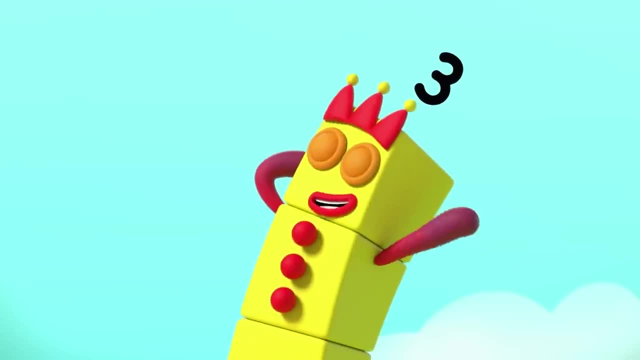 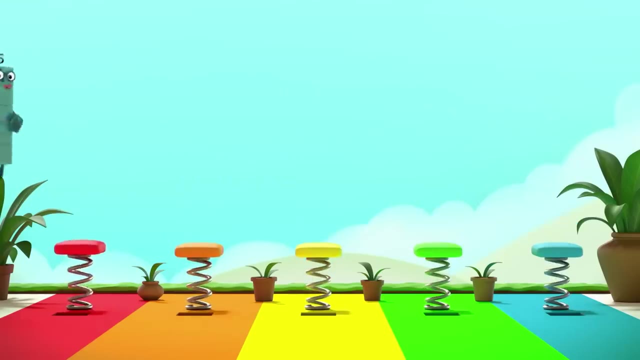 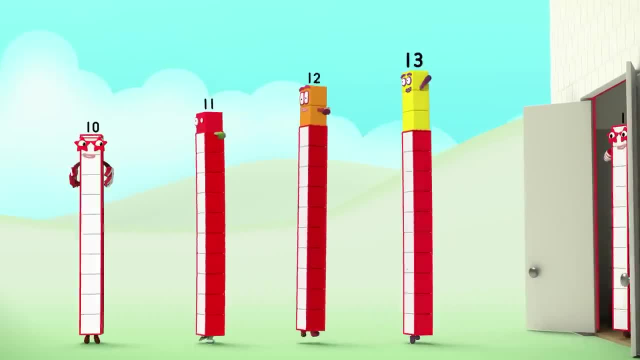 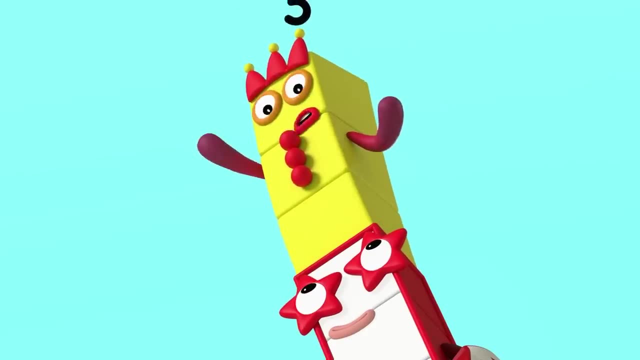 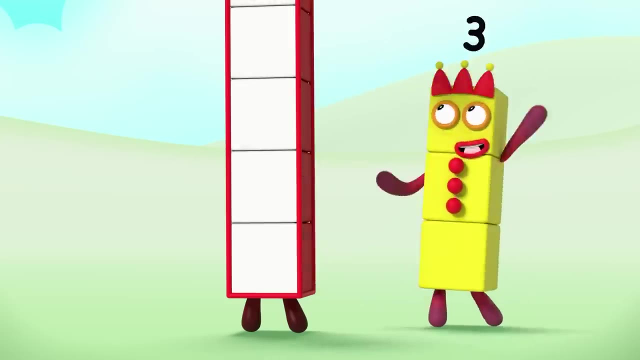 Ten, Eleven, Twelve, Thirteen, Woo-hoo, Fourteen, Fifteen, Welcome to. Oh, it's a bit high up here, Uh, put me down. All of you are bigger than me, Uh, so make yourself shorter. 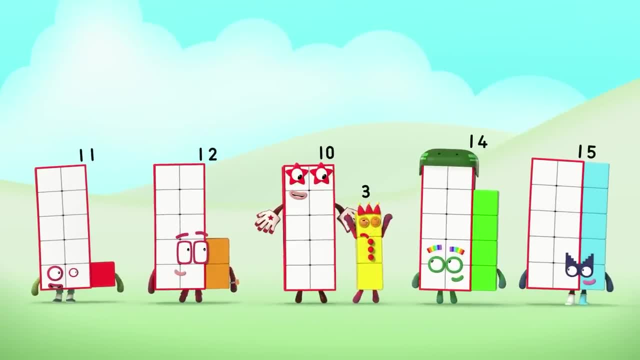 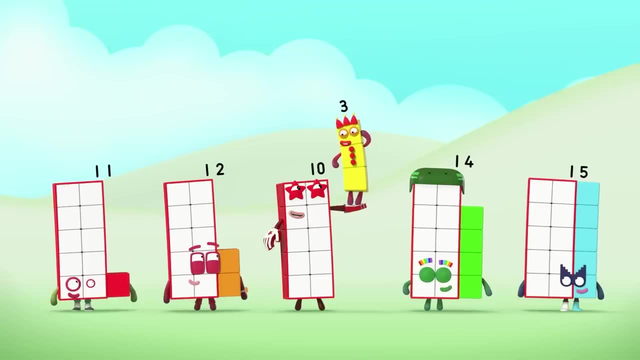 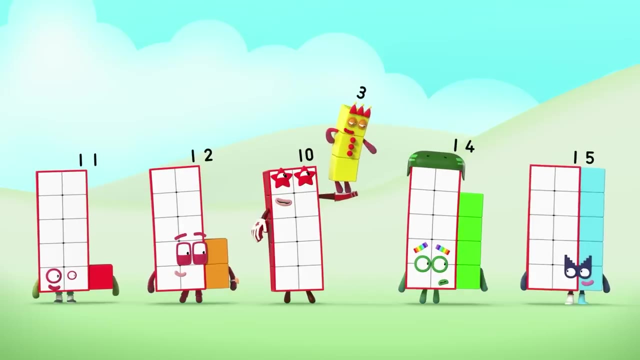 Even shorter. You've all got a three inside you. Well, except for thirteen. He already pinged a part into ten and me: Oh, fourteen, You're one more than thirteen. Extreme fourteen Minus one Equals thirteen. And for my next trick, twelve. 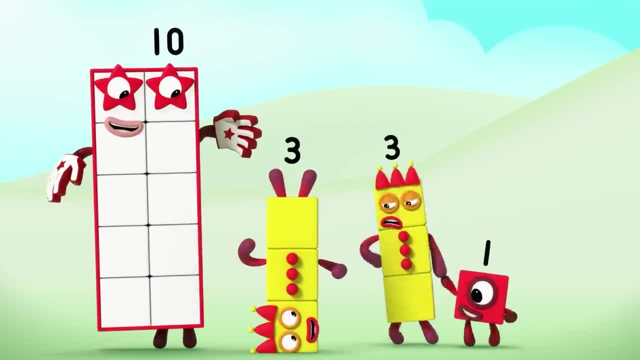 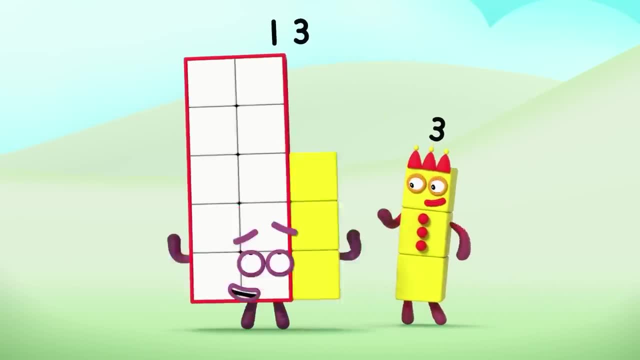 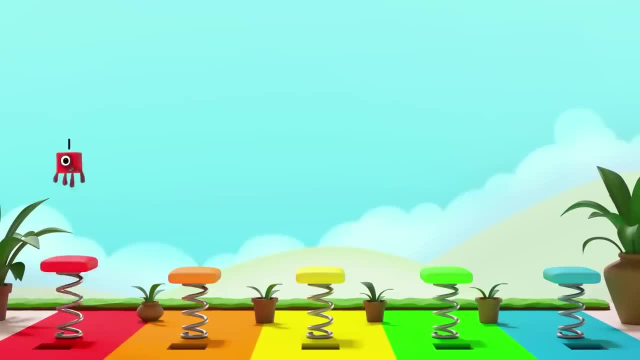 15. One, two ones, three ones, four ones, five ones. Ready, Let's work those tens. Yeah, Tall, slide two eyes. Slide and go low rectangle with a hole And freestyle. Yeah, Tall, slide two eyes. 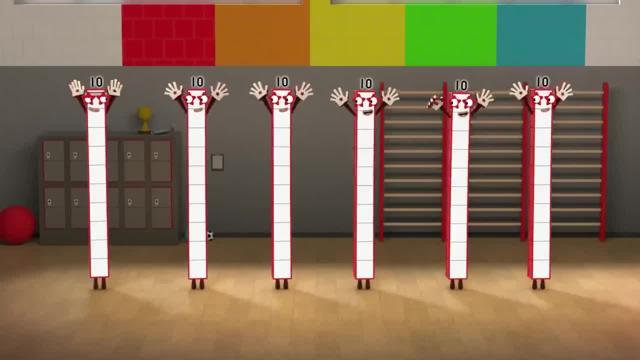 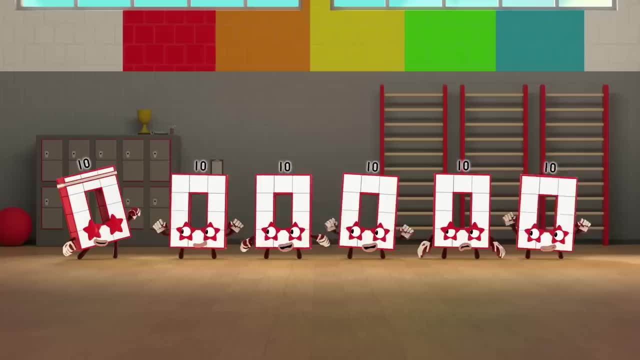 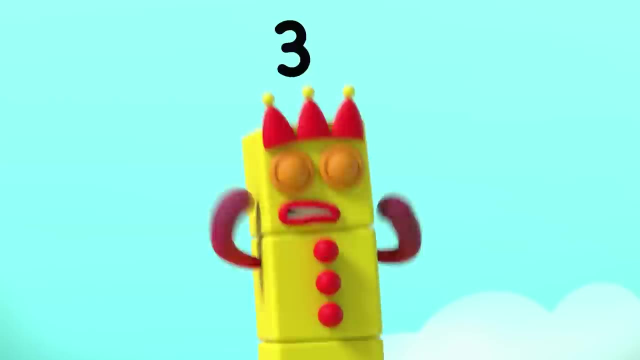 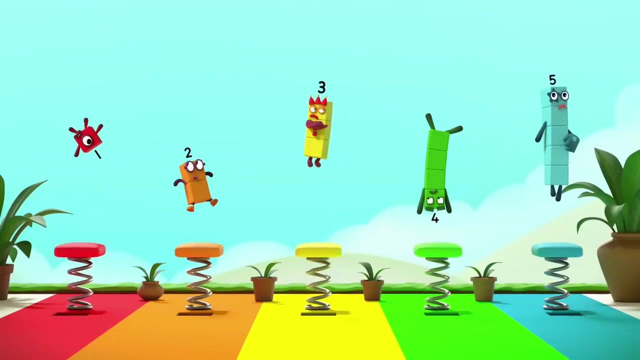 Slide and go low rectangle with a hole And freestyle: Yeah, Boing, boing, boing, boing, boing. Stop, stop, stop. If this is tens place, where are the tens? Err, I say we make this floor threes place. 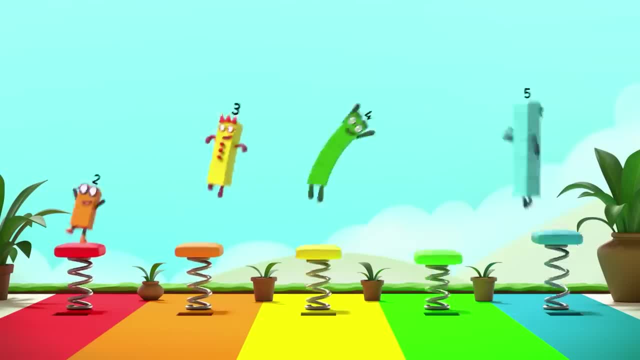 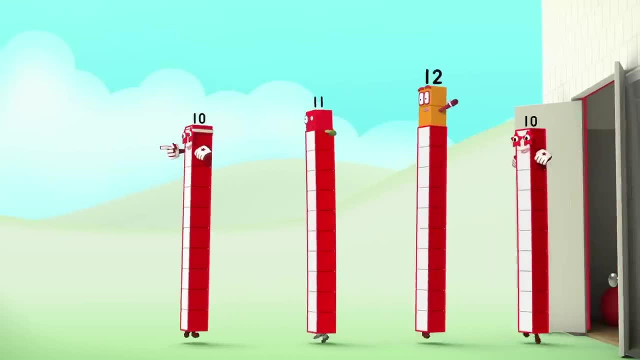 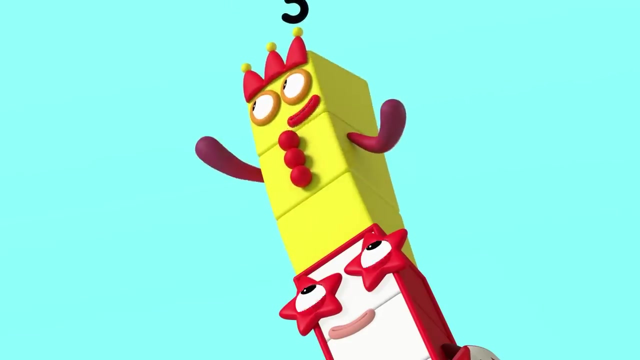 Everyone off. Boing, boing, boing, boing, boing. Ten, Eleven, Twelve, Thirteen, Wahoo Fourteen, Fifteen, Welcome to. Oh, It's a bit high up here. Put me down. 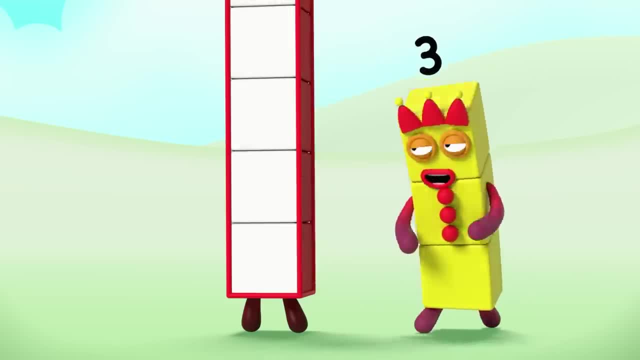 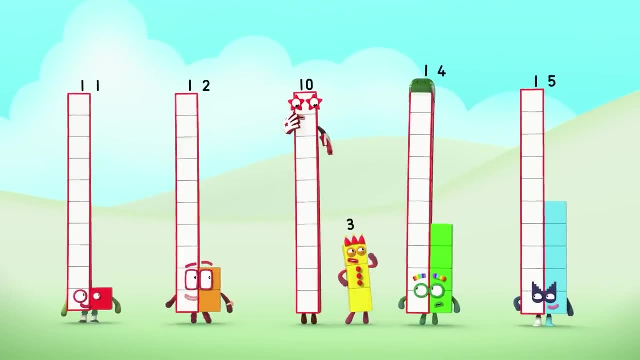 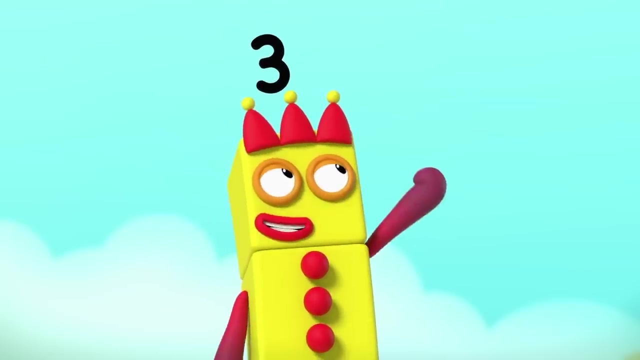 All of you are bigger than me, So make yourself shorter, Even shorter. You've all got a three inside you. Well, except for thirteen. He already pinged the part into ten and me, Oh, Fourteen, You're one more than thirteen. 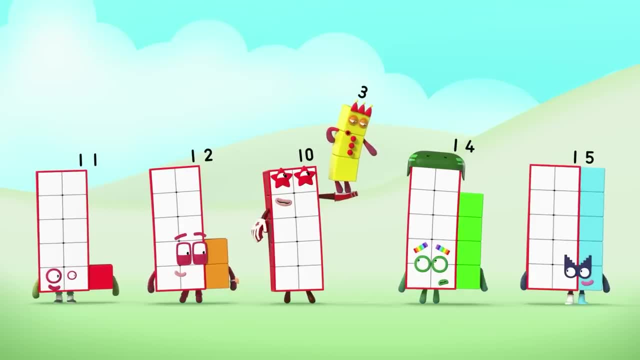 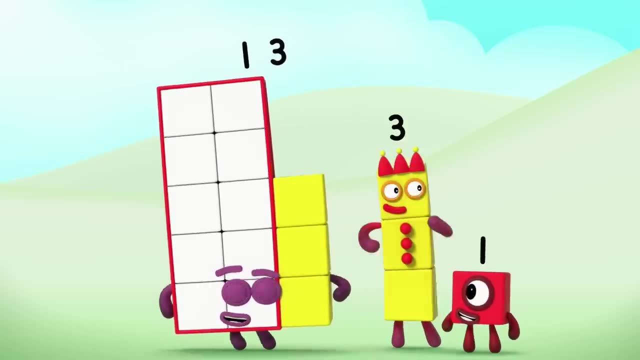 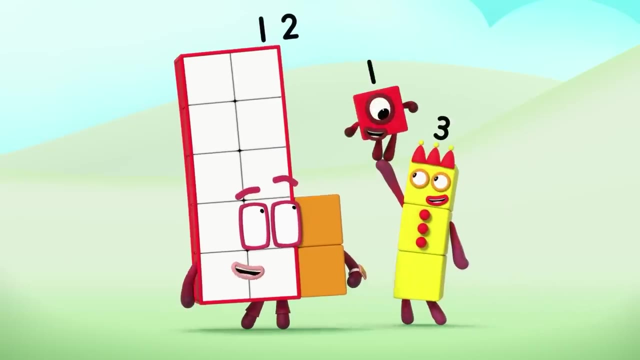 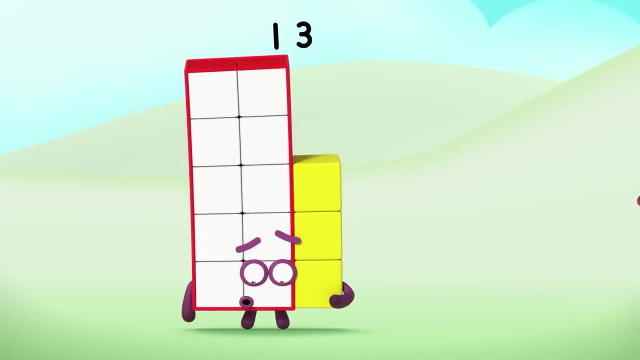 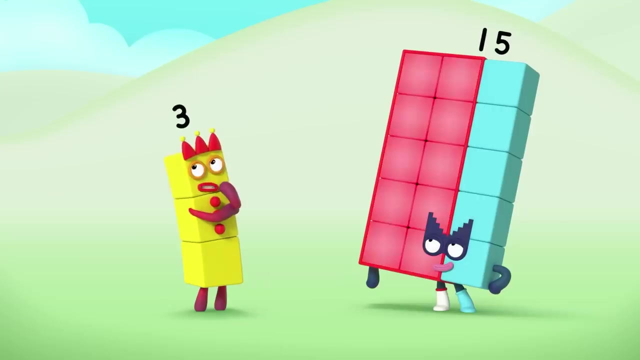 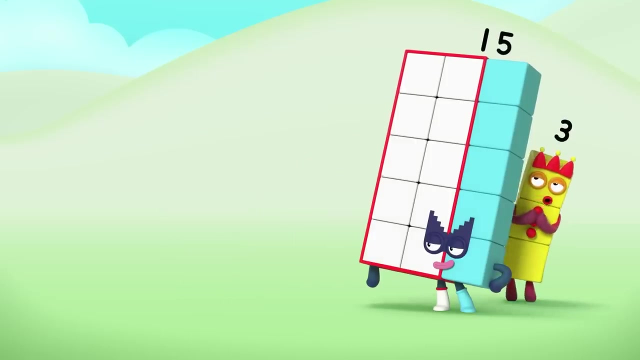 Extreme: fourteen Minus one Equals thirteen. Oh, Oh, Oh, Oh. And for my next trick, Ten and three. Oh, Your turn fifteen, Let's say ten and five, But I want ten and three, And three is two less than five. 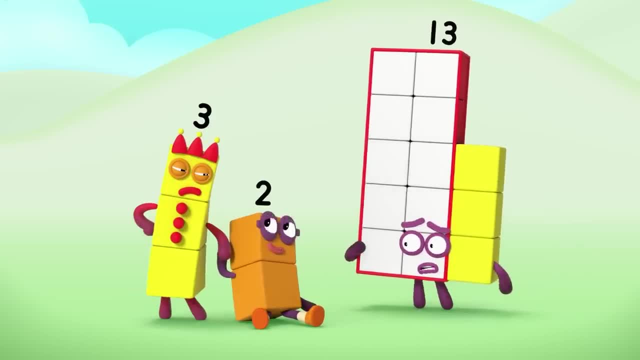 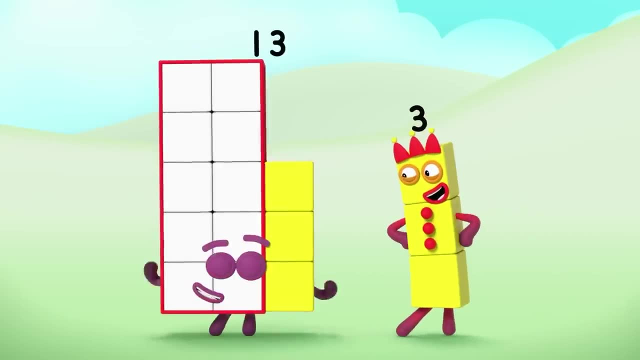 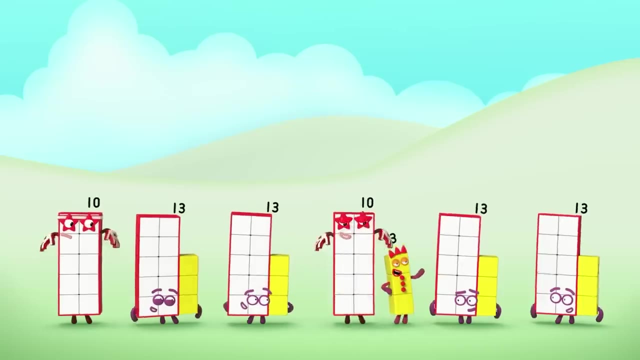 So let's pop off a two, Ten and five. Ten and one plus two equals, Sir, only joking- Ten and three There. Now everybody stand tall, Go When I say go, go, Go, my lovely 13.. 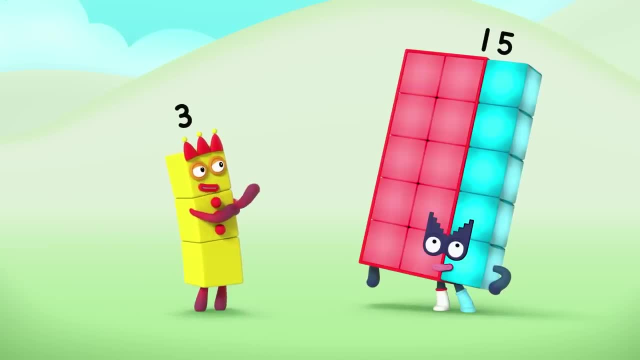 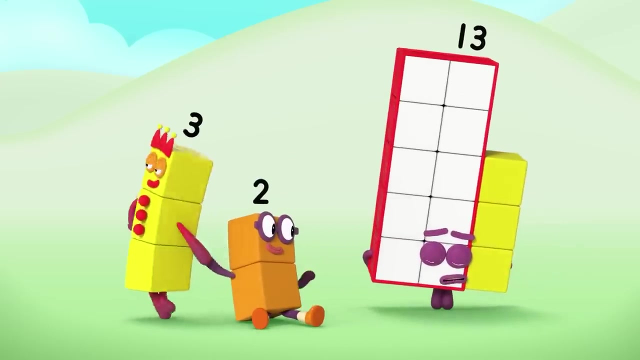 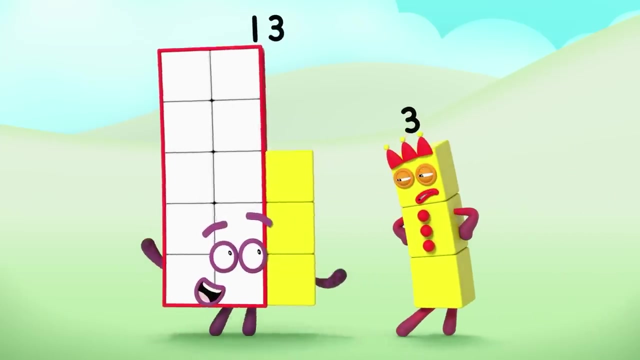 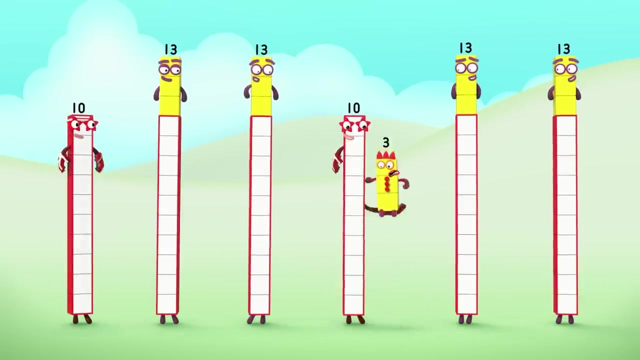 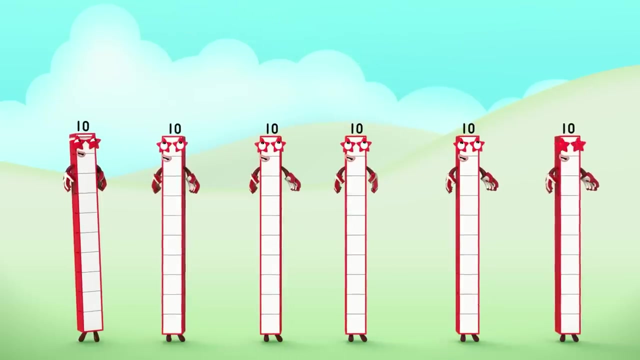 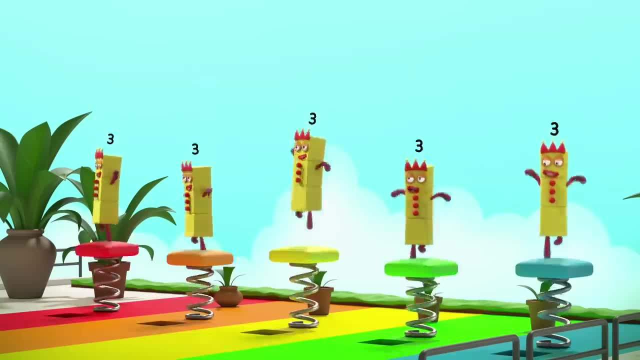 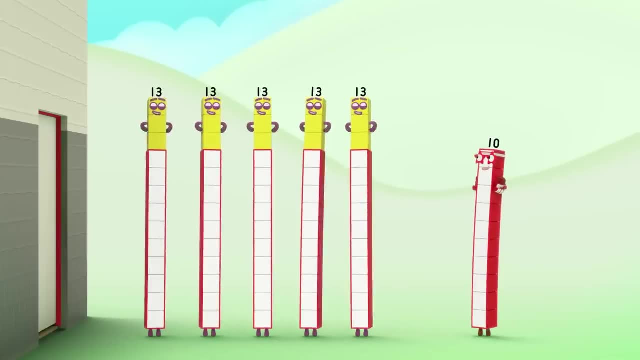 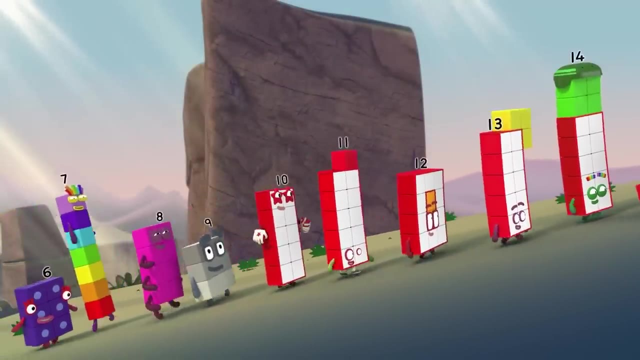 Welcome to Three's Place. Bolly-ha, bolly-hoo, bolly-ha. Never mind Tenth Place or Three's Place, We should call this Thirteen. I can't wait to visit the Patton Palace. Is it far? 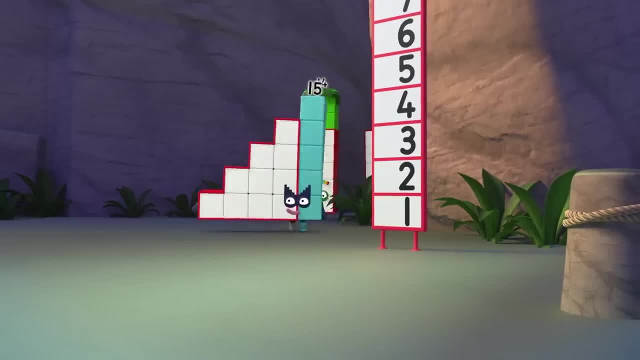 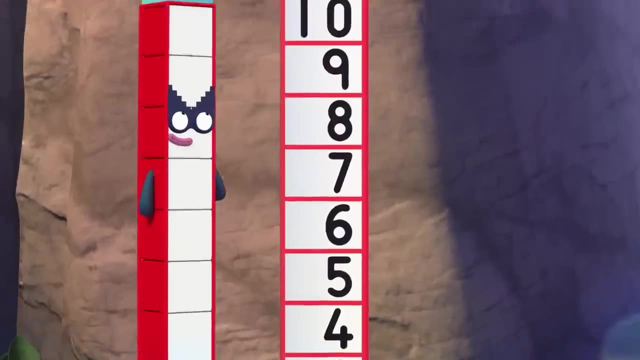 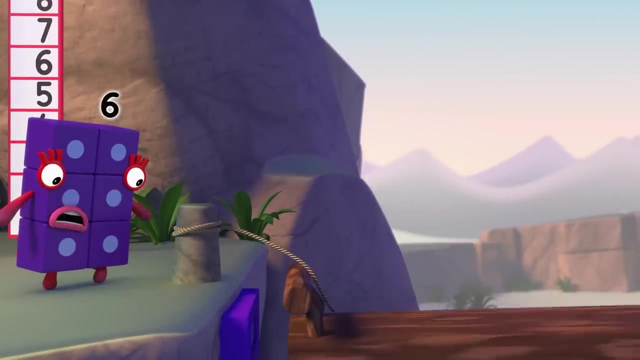 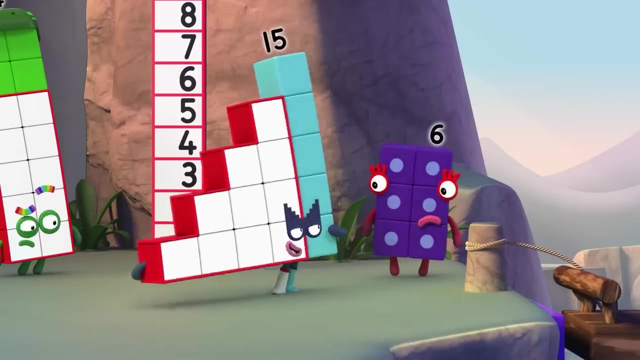 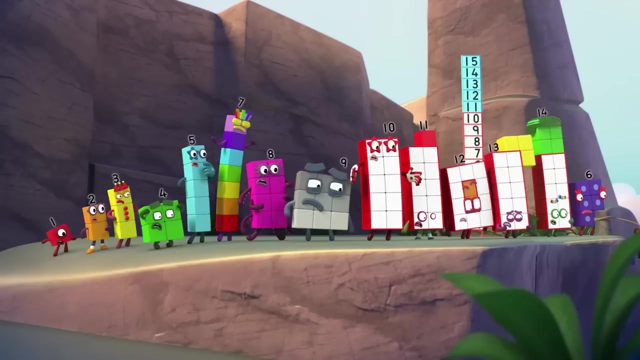 There's a shortcut round this ridge. if you can cross the balancing bridge, Wow, Ta-da, Whoops, Guess I forgot to put the safety locks on. I say we go softly, softly, Like this, Yipe Ooh, Oh, my God. 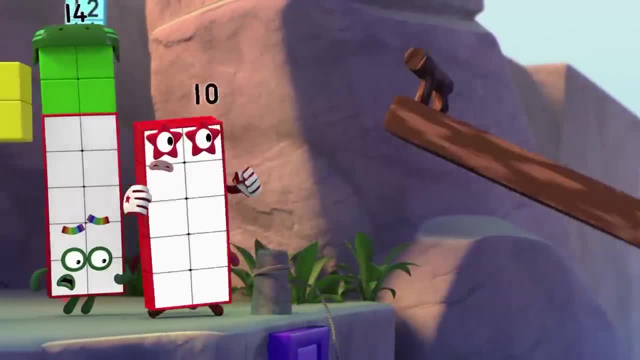 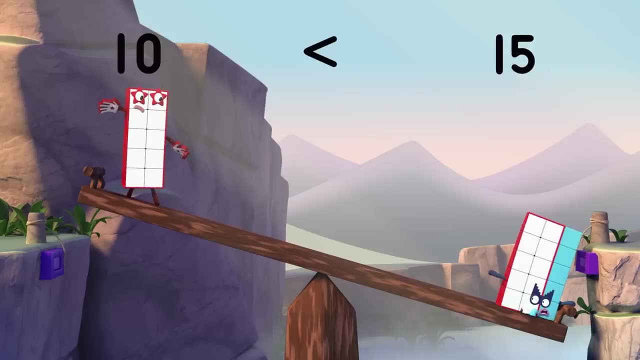 See, We need to balance the bridge out before 15 falls off, But I'm not big enough to do it alone. 10 is less than 15.. You need 15 blocks to balance me out, But 15 is 10 and 5.. 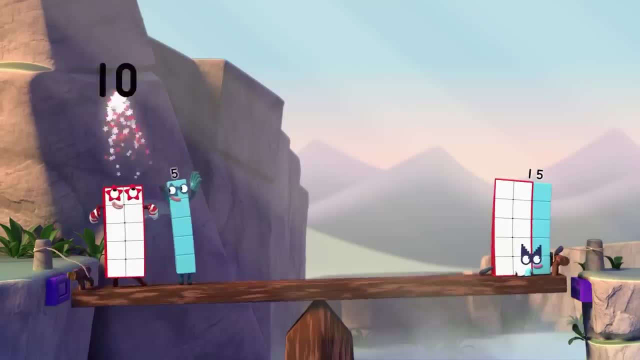 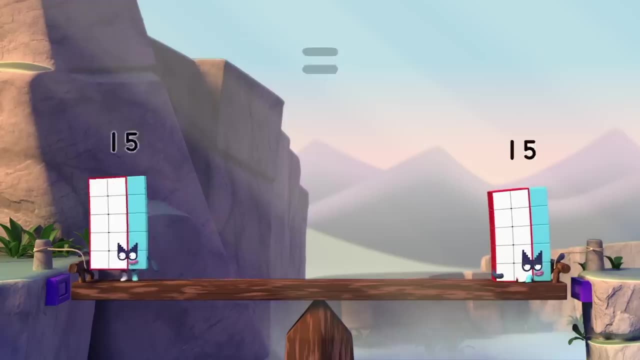 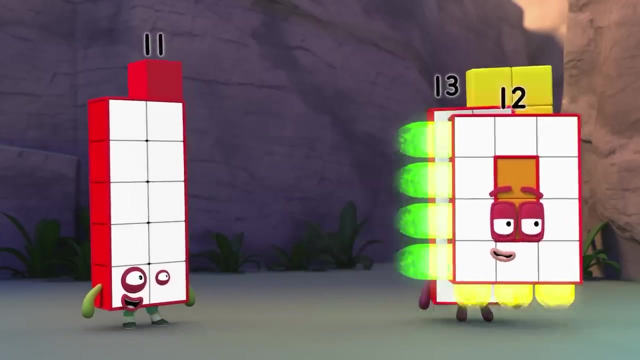 So if I land a hand Hoo, 2 plus 5 equals 15!. Grab hold. We need to reach the far side So we can lock the bridge. I can do this. I am 3 by 4.. 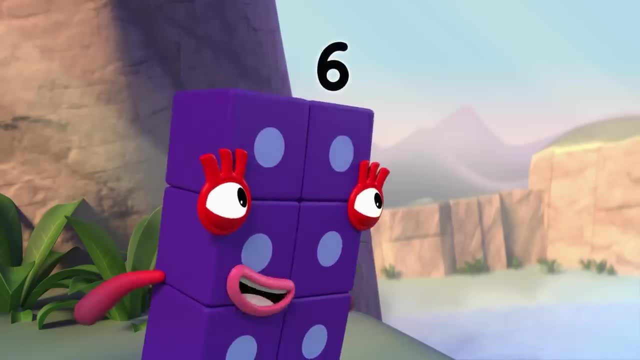 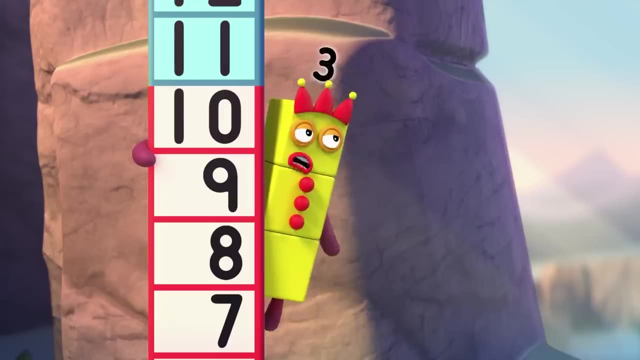 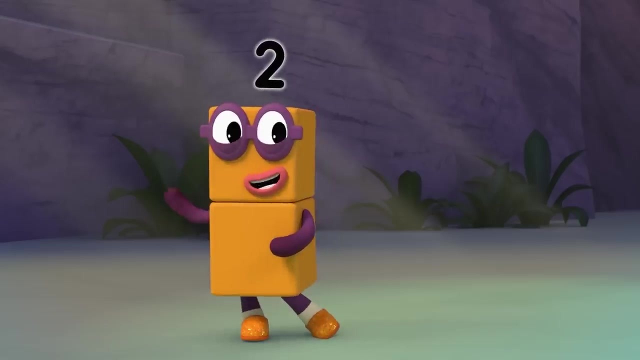 I am a rectangle. Wow, That is so cool. Thanks, What's going on? 12 needs balancing And 12 is 10 plus 2.. Come on 10!. Wait, Where's 10? Bit busy, Sorry. 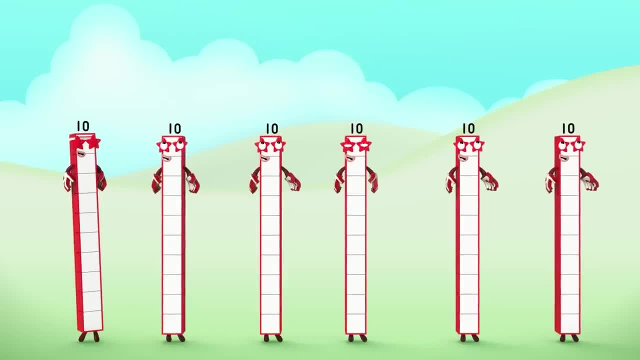 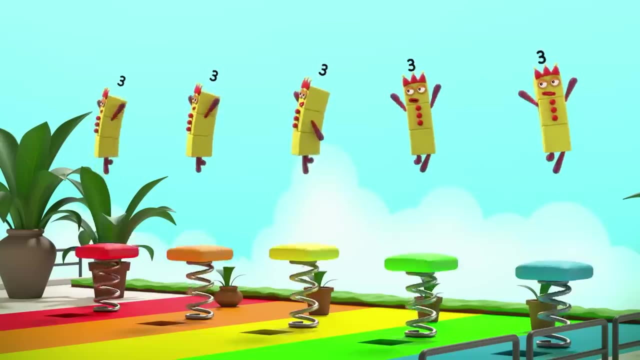 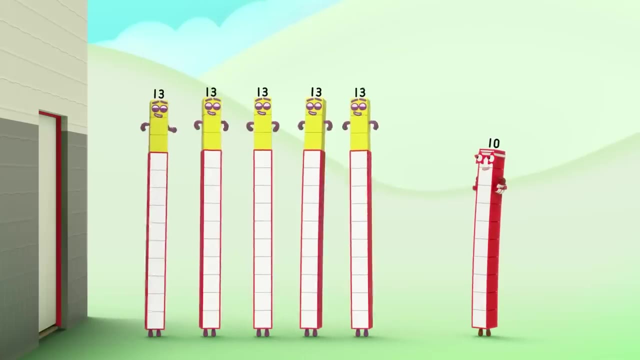 Woo Bolly ho bolly ha. Welcome to Three's Place. Bolly ha bolly ha, Bolly ho, bolly ha. Never mind 10's place or Three's Place, We should call this 13.. 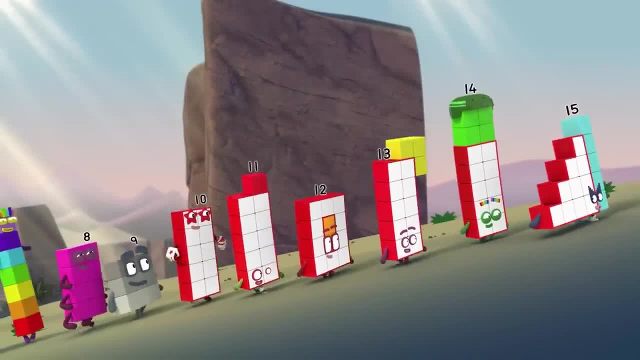 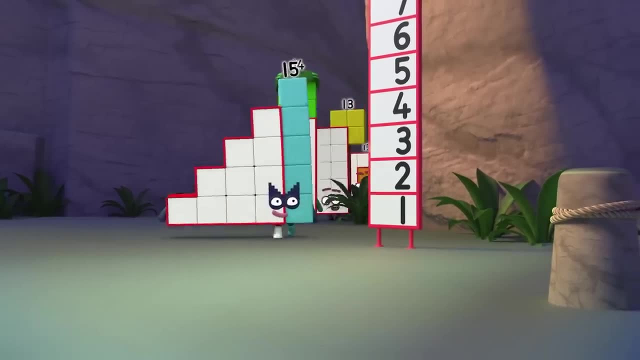 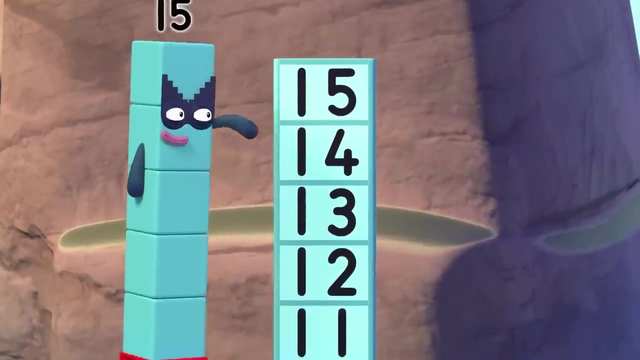 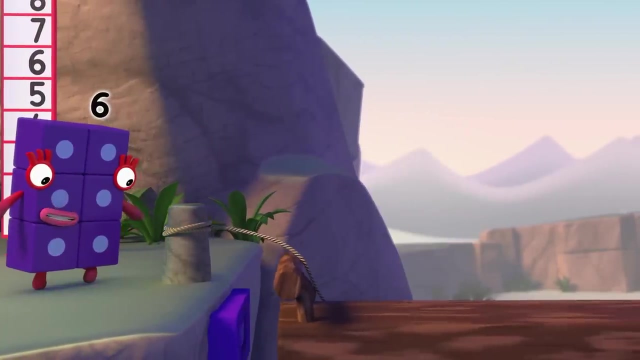 Woo, I can't wait to visit the Patton Palace. Is it far? There's a shortcut round this ridge, if you can cross the balancing bridge. Hmm, Oh, Oh, Wow, Ta-da Woo, Whoops, Guess I forgot to put the safety locks on. 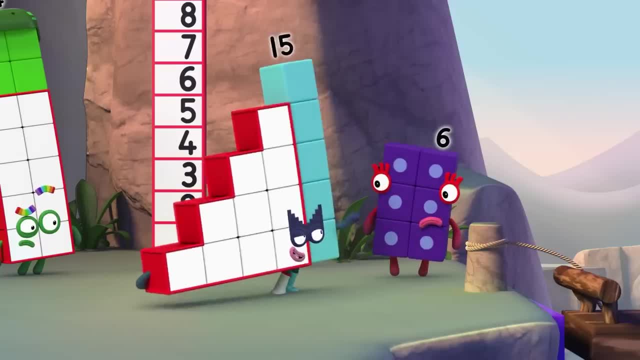 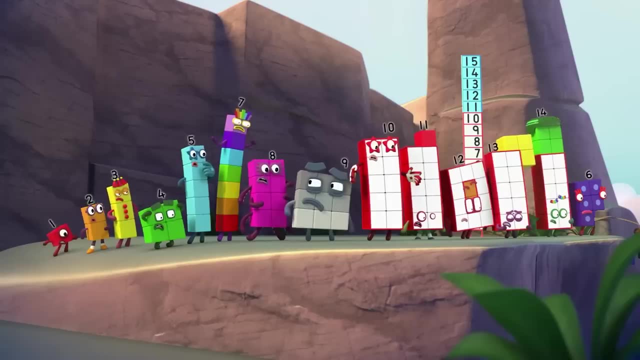 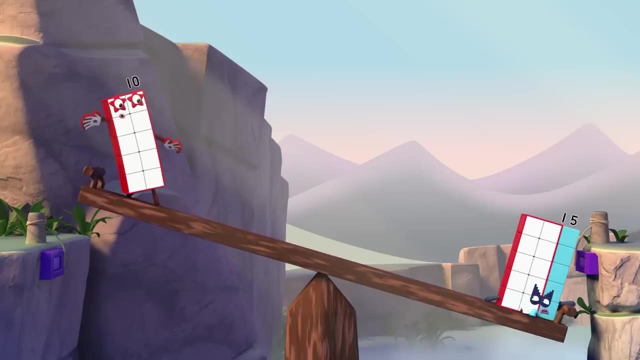 I say we go softly, softly, Like this: Yipe, Woo Woo. Oh, my God, We need to balance the bridge out before 15 falls off, But I'm not big enough to do it alone. 10 is less than 15.. 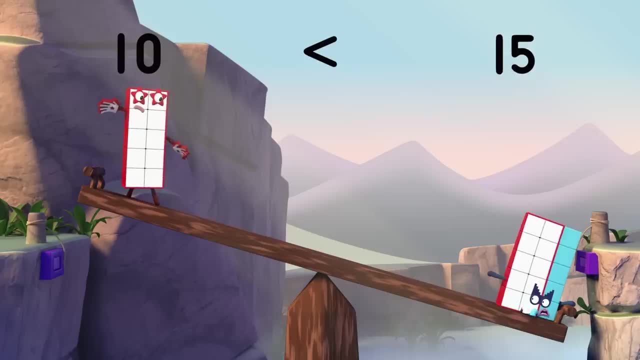 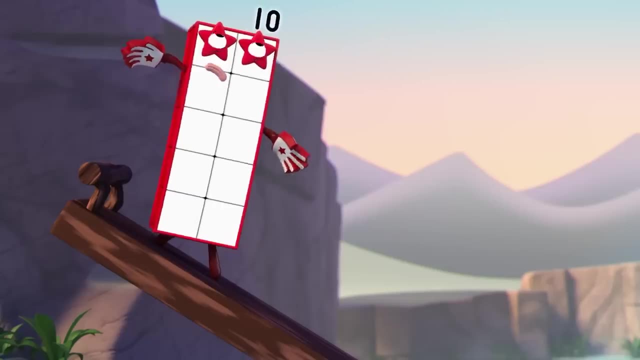 You need 15 blocks to balance me out. Oh no, Oh no, Oh no, But 15 is 10 and 5.. So if I lend a hand, Ha Hoo, 2 plus 5 equals. 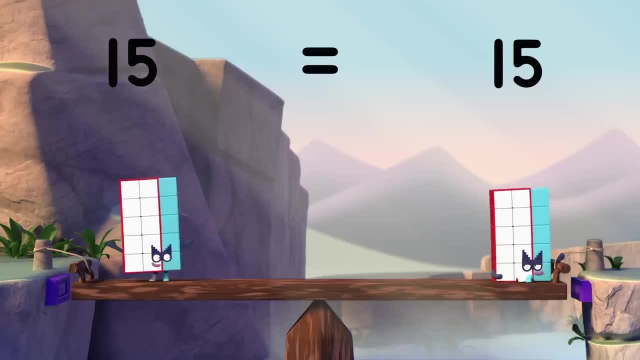 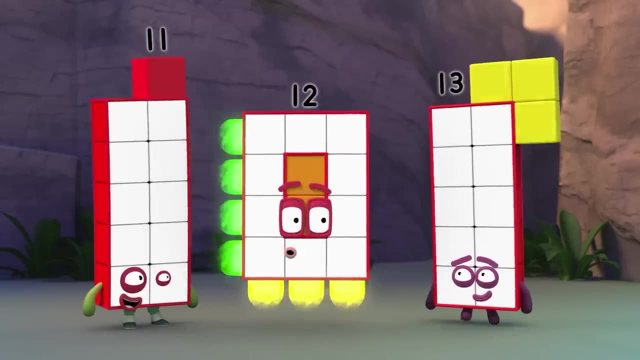 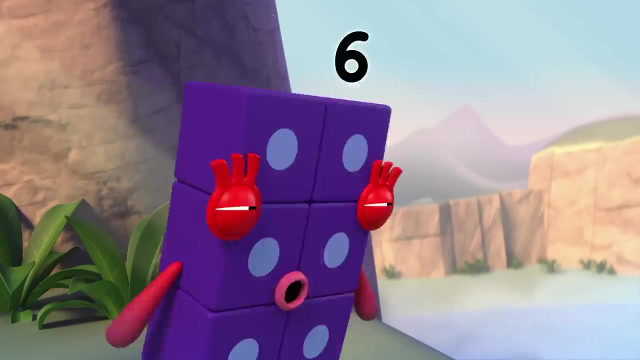 15!. Grab, hold. We need to reach the far side so we can lock the bridge. I can do this. I am 3 by 4.. I am a rectangle. Wow, That is so cool. Thanks, Six Oh. 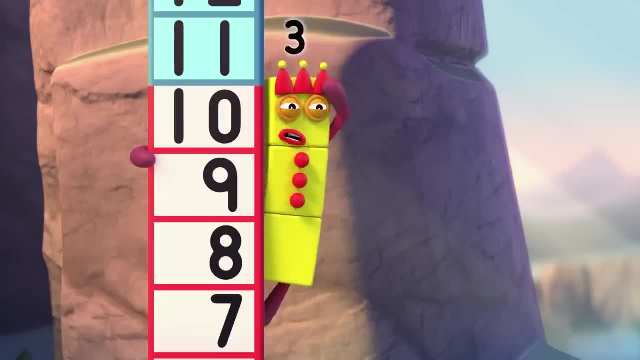 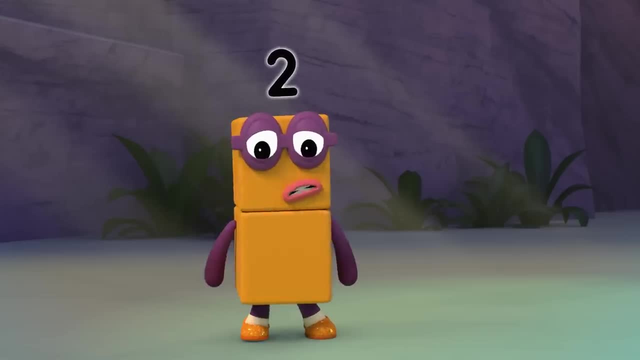 Oh, Oh, Oh. What's going on? Oh, 12 needs balancing And 12 is 10 plus 2.. Come on 10!. Wait, Where's 10?? Oh Bit busy, Sorry. Then we need another 10.. 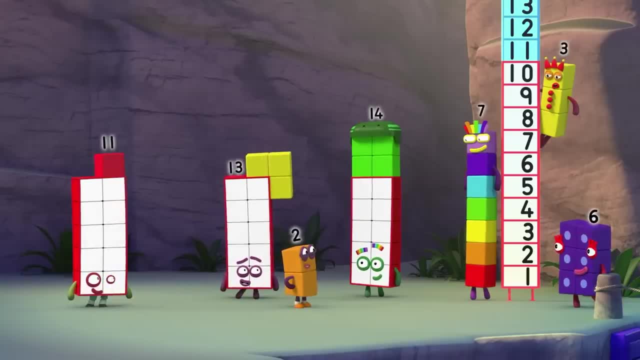 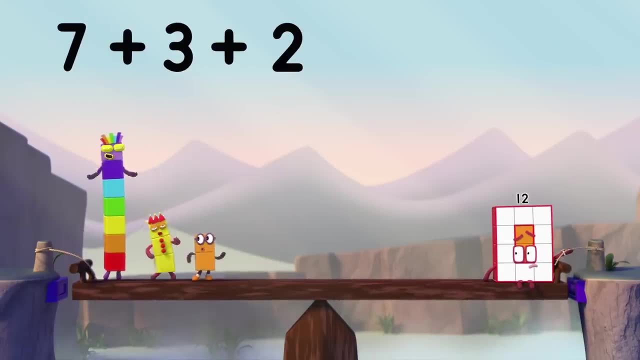 Oh, 7, 3. You can make 10.. Oh, That's lucky. 7 plus 3. Plus 2. Equals 10! 10! Plus 2. Equals 12! 12!, Grab hold. 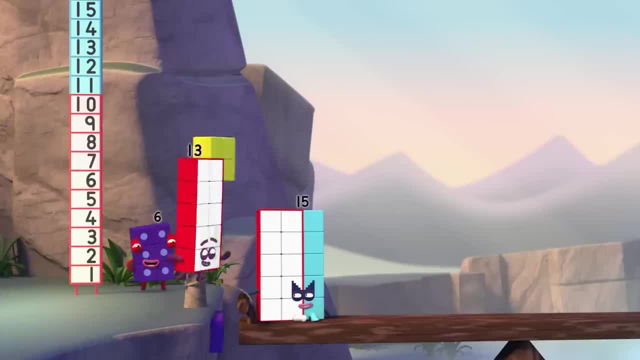 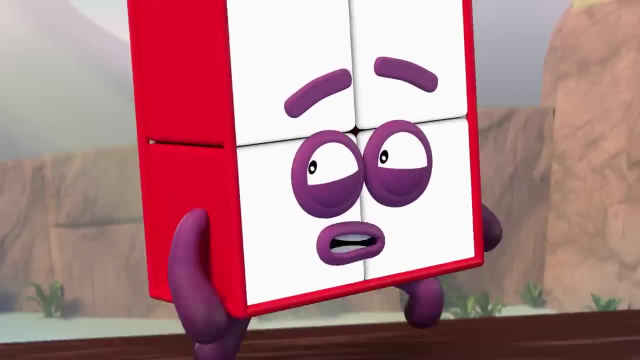 Hooray, We're halfway there. What could possibly go wrong? What could possibly go wrong? What could possibly go wrong? Ooh, Look out 13!. Who said it? Oh, What We need to balance 13.. 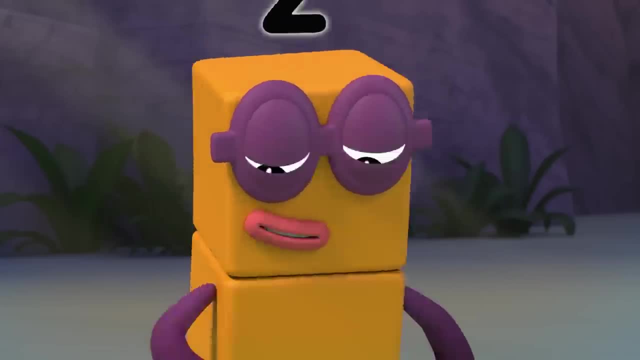 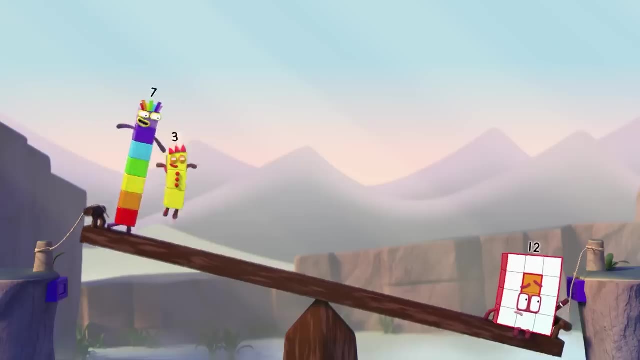 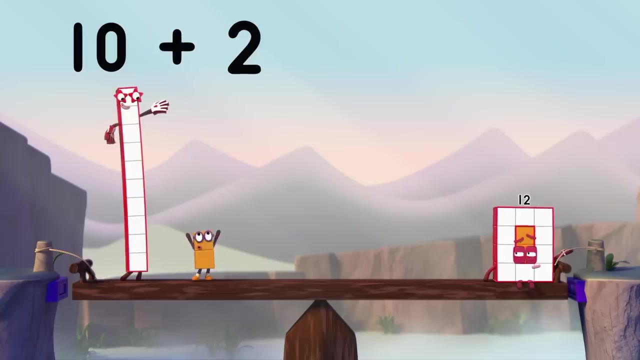 Then we need another 10.. 7,, 3. You can make 10.. Hoo-hoo, That's lucky. 7 plus 3. Plus 2. Equals 10!. Plus 2 equals 12!. 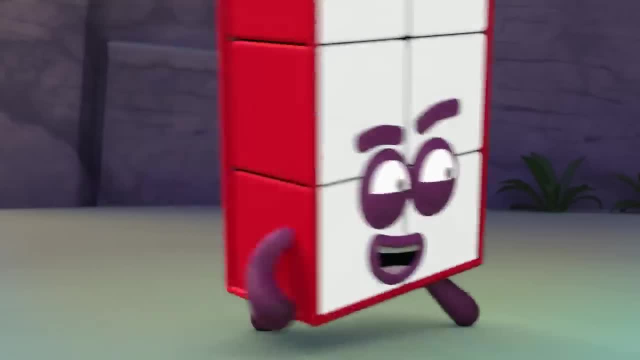 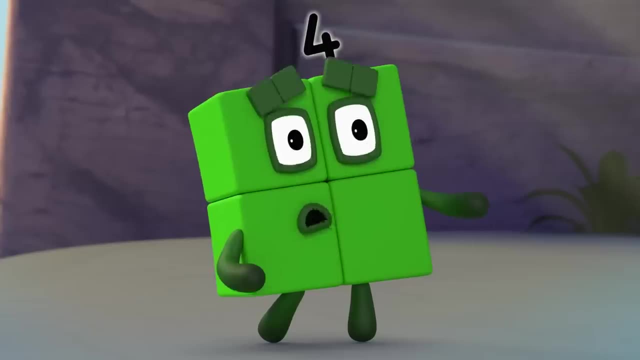 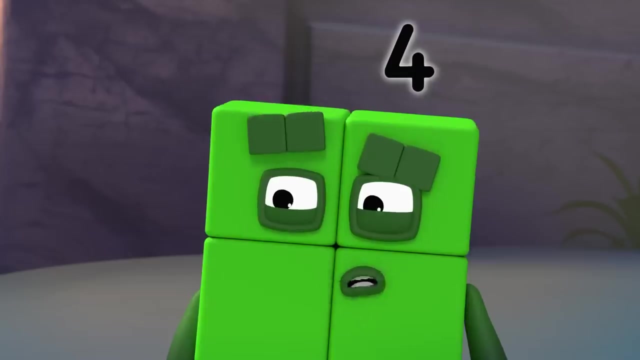 Grab hold. Yay, We're halfway there. What could possibly go wrong? Ooh, Look out 13!. Who says it? We need to balance 13. But we haven't got a 3 or a 10.. Maybe I can help. 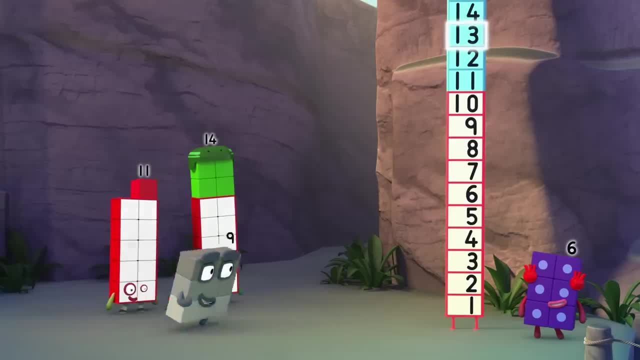 I'm only one, less than 10.. That's close, And after that we need 3 more blocks, So that adds up to 1,, 2,, 3, 4.. 4 blocks, Oh, Square power. 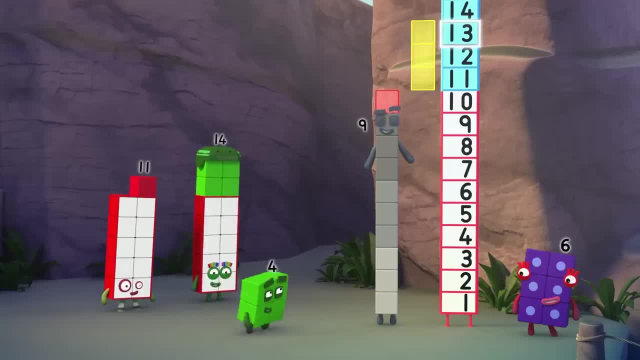 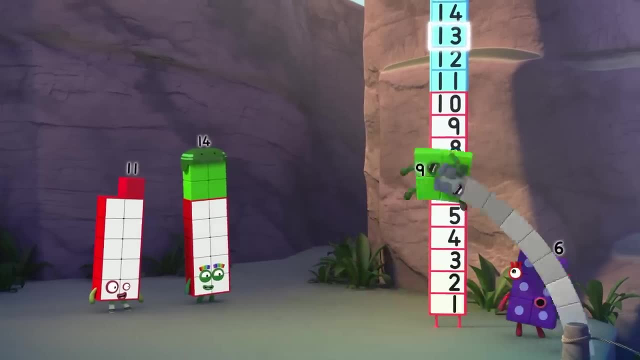 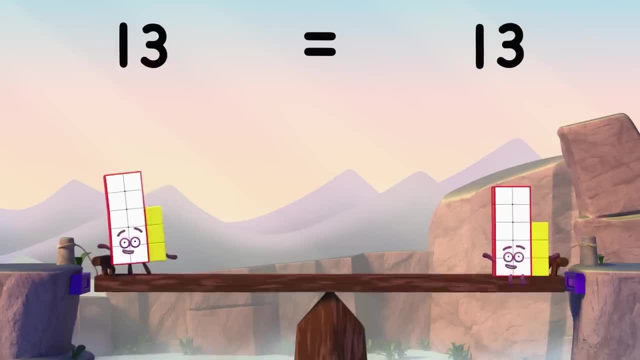 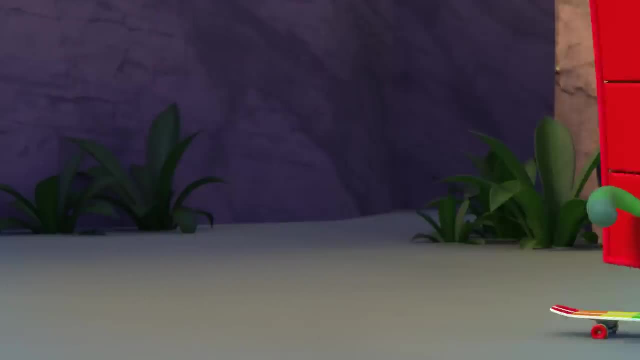 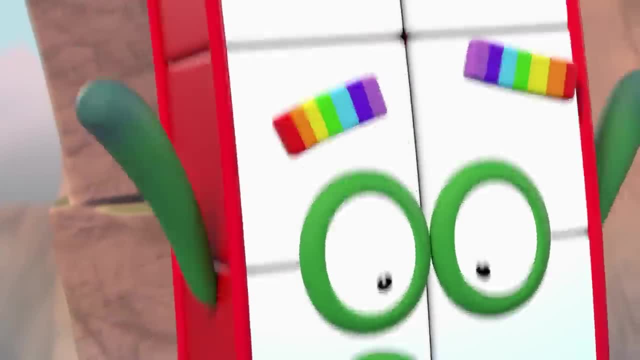 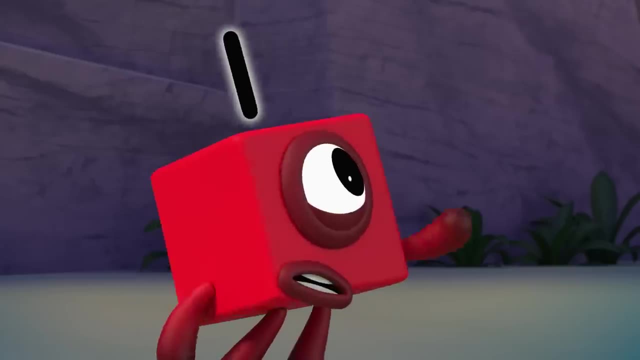 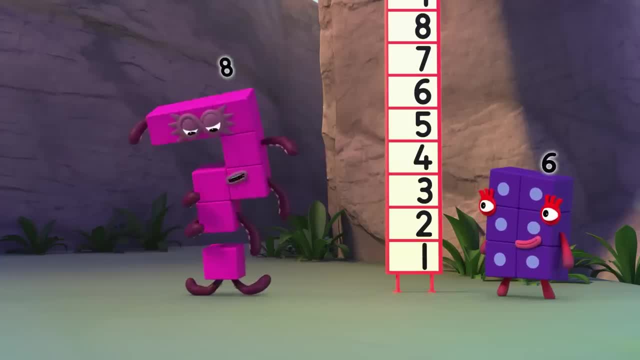 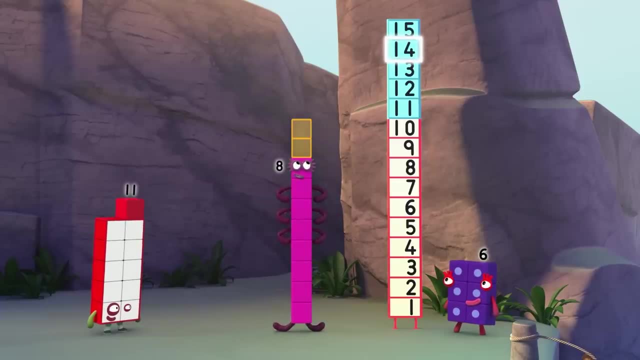 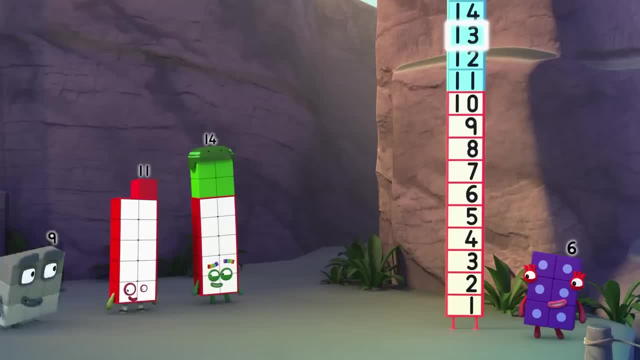 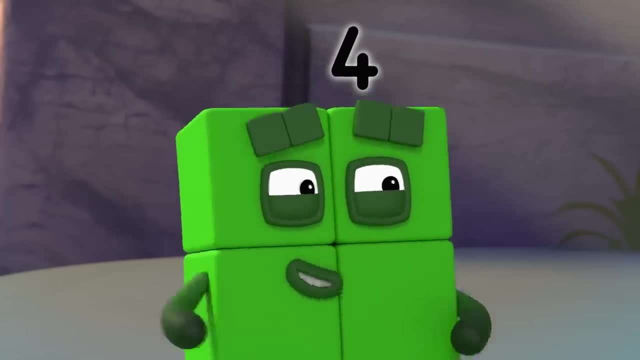 But we haven't got a 3 or a 10. Maybe I can help. I'm only one less than 10.. That's close, And after that we need 3 more blocks, So that adds up to 1,, 2,, 3,, 4.. 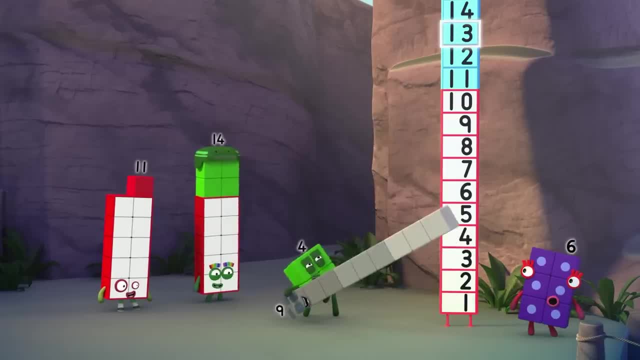 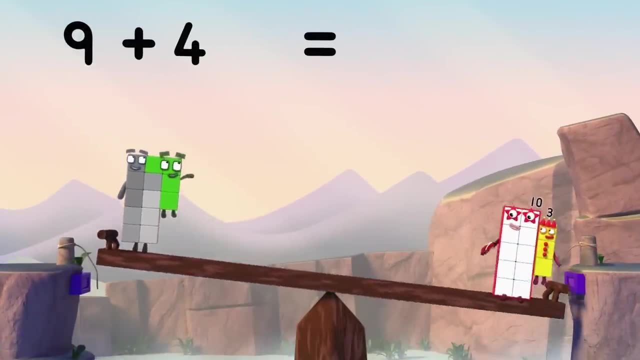 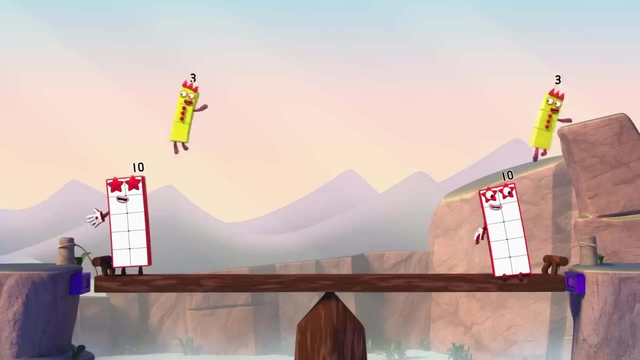 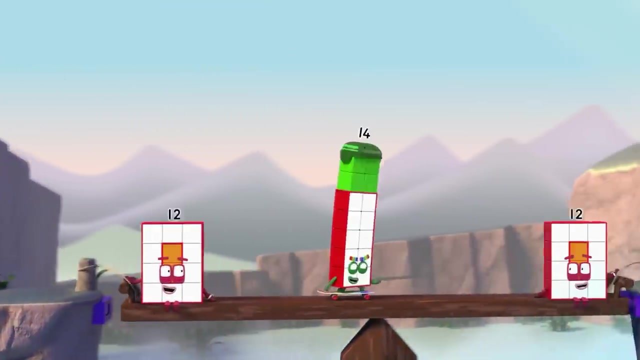 4 blocks, Oh, Square power. 9 plus 4 equals 10 plus 3.. And both sides equal 13!. Whee, Grab, hold One more bridge to go Ready. 2!, 1!, 2!. 1!, Okay, Two, 3!, 5!, 6!, 7!, 8!, 9!, 10!, 1!, 3!, 2!, 3!, 2!, 3!, 4!, 1!. 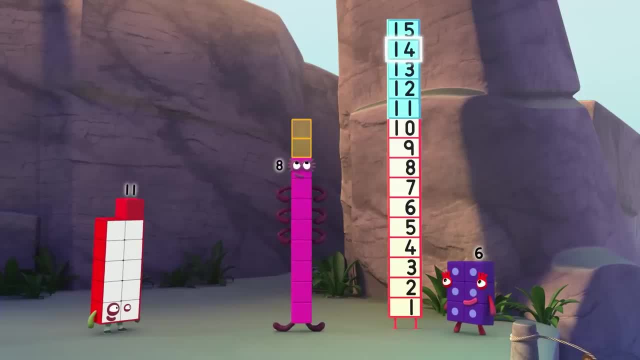 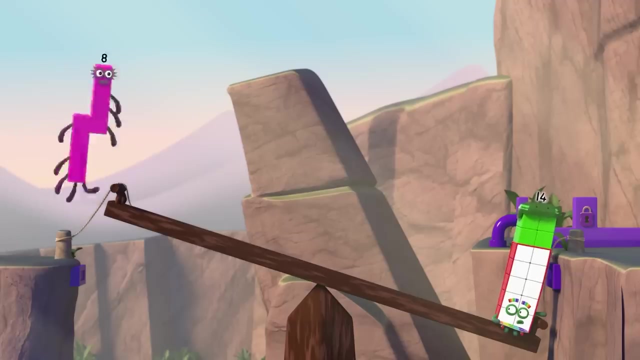 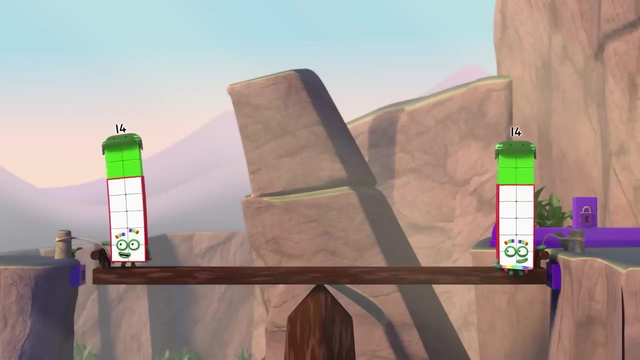 1!. From eight to ten takes two blocks, and fourteen is ten and four. So I need four blocks more, which makes one, two, three, four, five, six. Eight Plus six Equals fourteen Grab hold. Thanks to our team, we've got a clear run at goal. 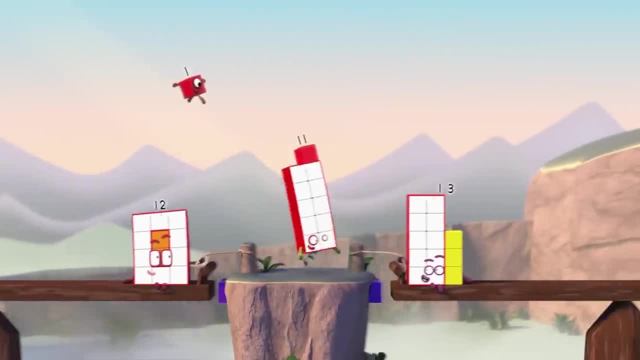 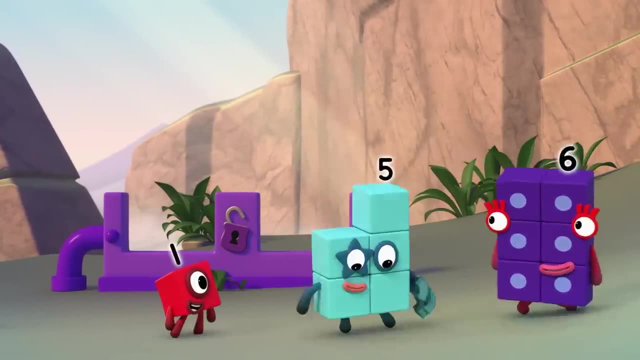 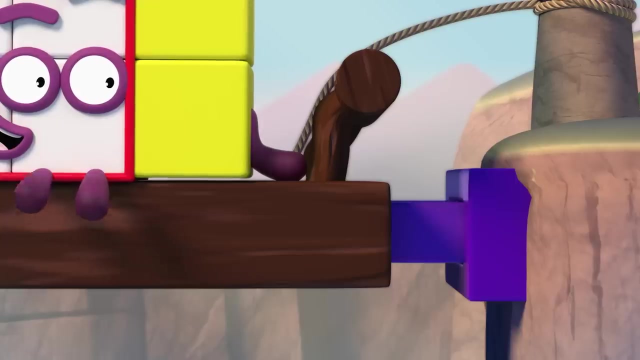 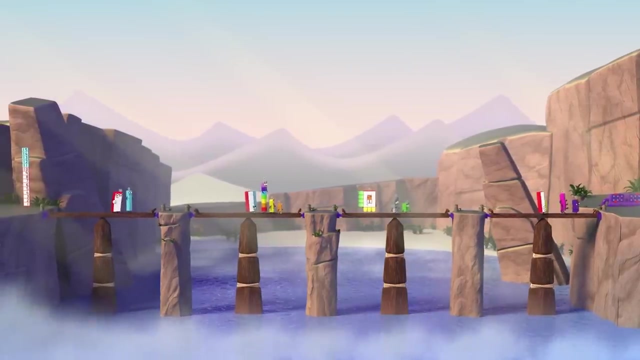 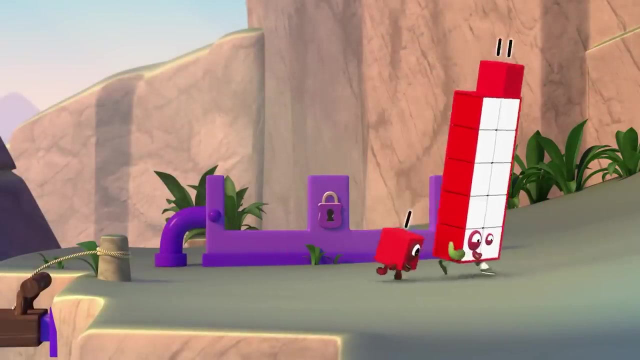 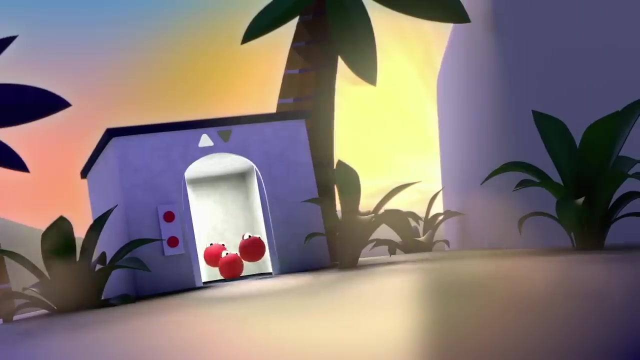 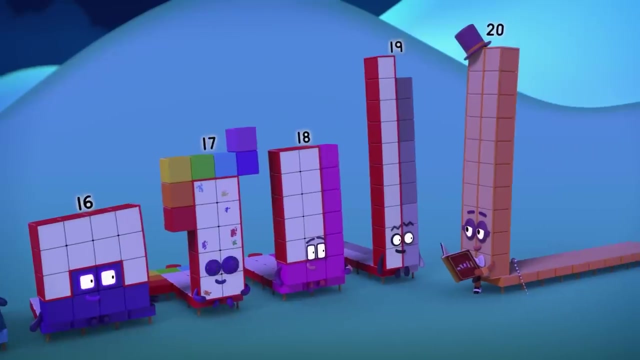 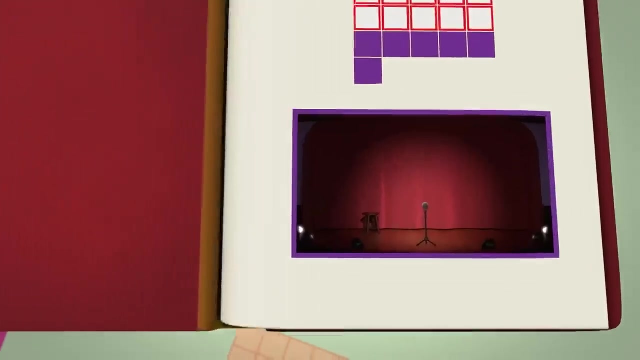 Double six bridge is fixed. I guess this shortcut's not so swift. Next time we can take the lift. There's a lift Sit, If you're sitting comfortably. then I'll begin Chapter 16, a six walks into a ten. 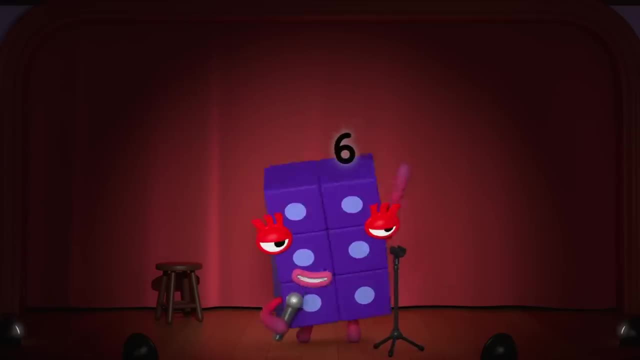 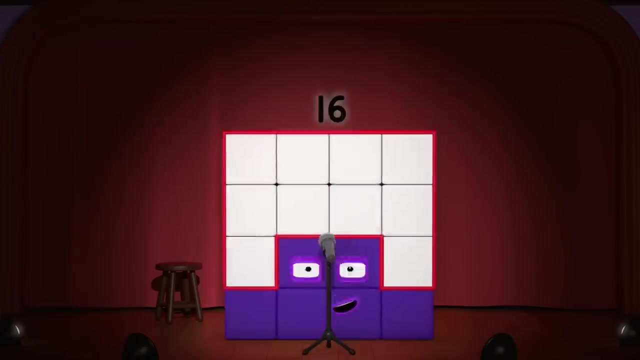 Ow. Now it's time to introduce you to an act who will amuse you. She knows how to make a scene. Give it up now for Sixteen. Hi Ten, They're Sixteen. Right here, I'm Sixteen. 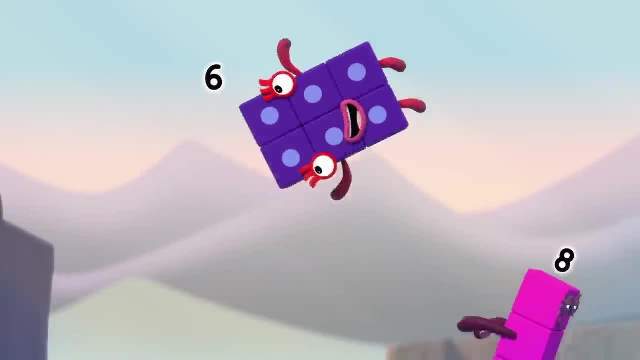 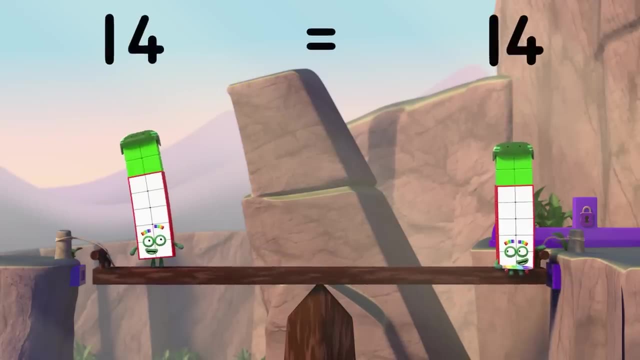 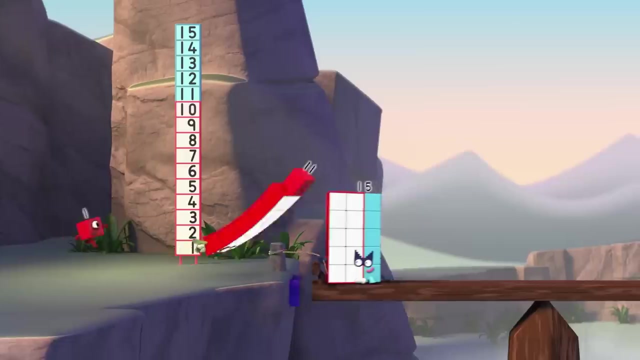 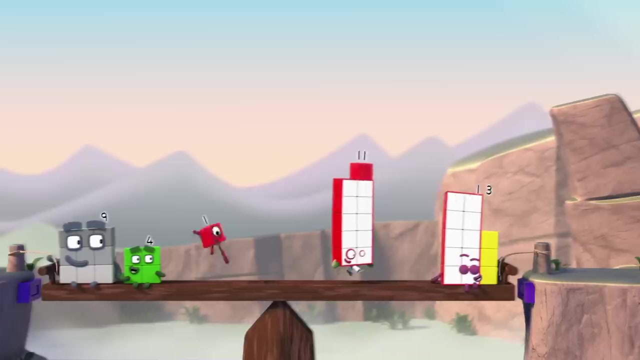 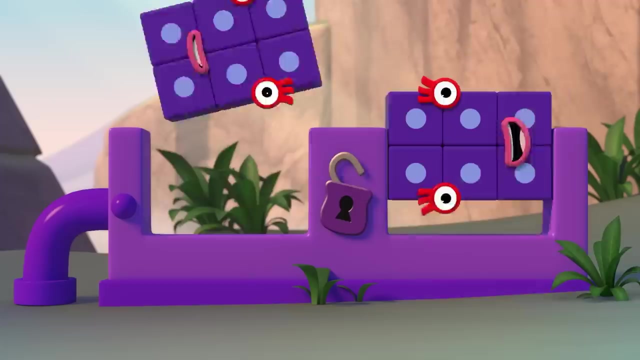 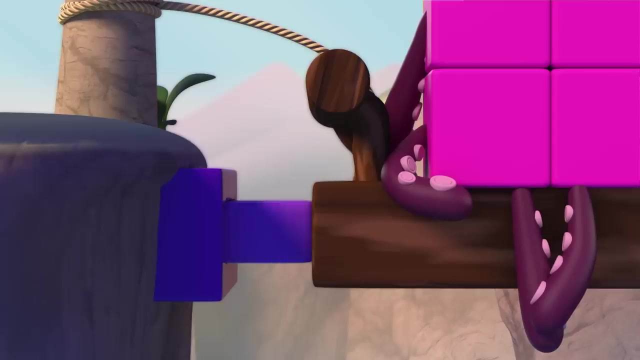 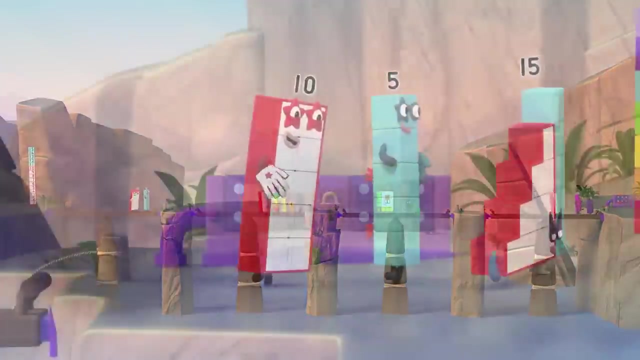 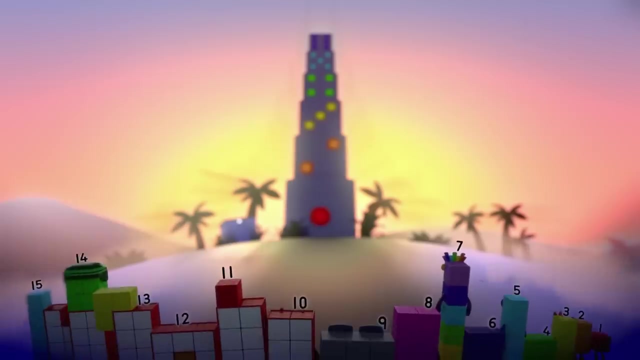 Square power, Square power. Eight plus six equals 14! Grab hold. Thanks to our team, we've got a clear run at goal. Double six bridge is fixed. Hooray, I guess this shortcut's not so swift. Next time we can take the lift. 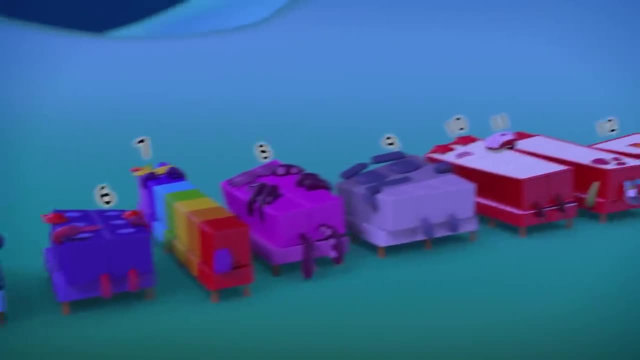 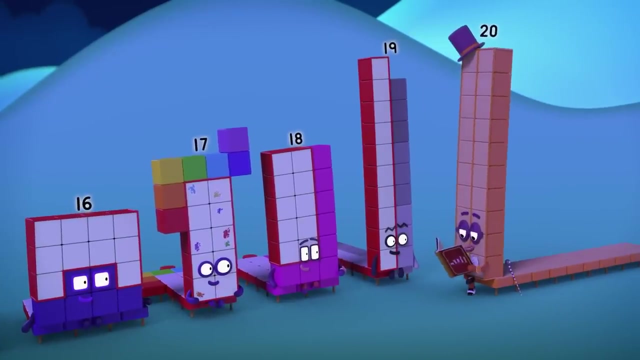 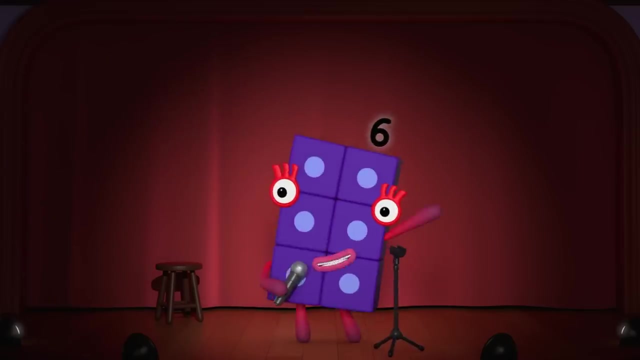 There's a lift Sick. Thank you. If you're sitting comfortably, then I'll begin Chapter 16, a six walks into a ten Ow. Now it's time to introduce you to an act who will amuse you. She knows how to make a scene. 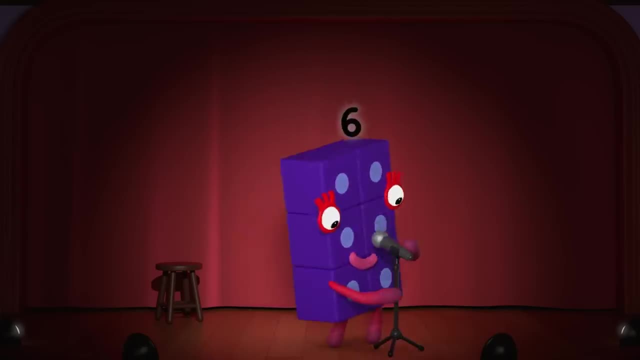 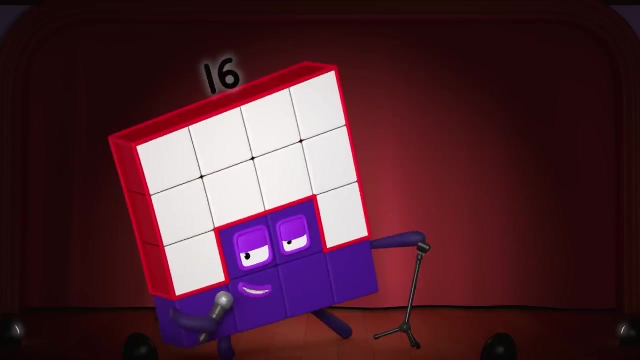 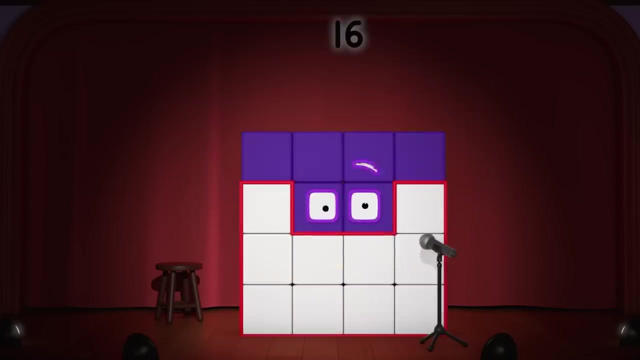 Give it up now for 16!. Um, hi Ten, They're 16.. Right, here, I'm 16.. Let's get this party started. It's nice to be here And here And here And here. Oh, look at that. 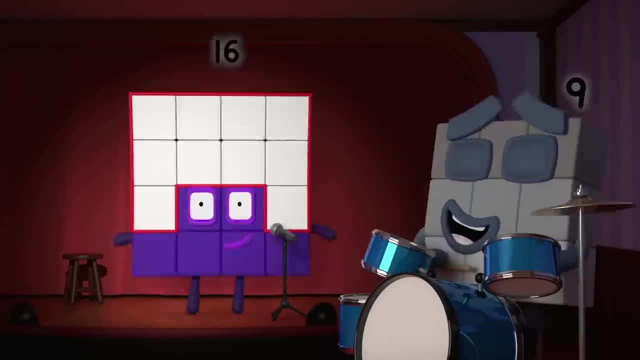 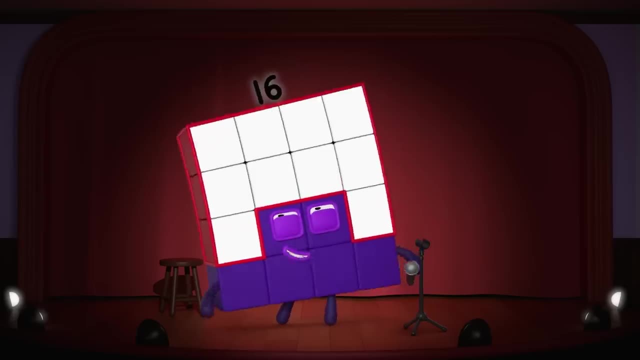 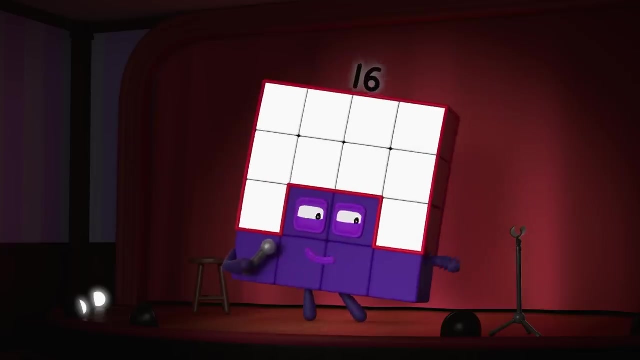 I'm a square turning round. Hey, you know what nine's favourite story is: Goldilocks and the three squares Squares. And if you're after a square deal, here I am. I'm a square, Mega squares With a-. 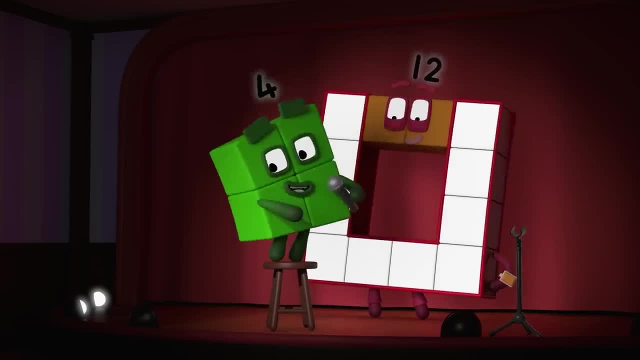 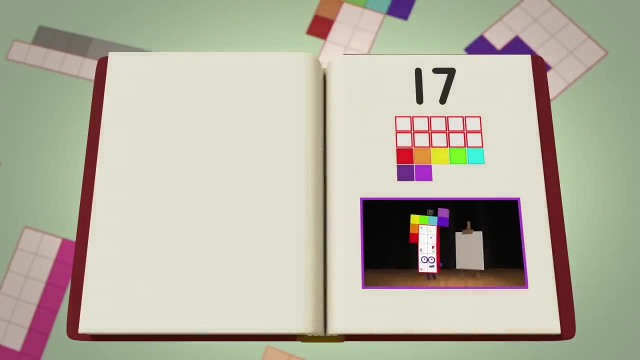 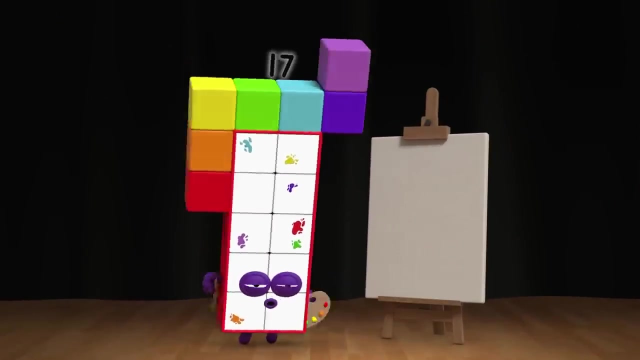 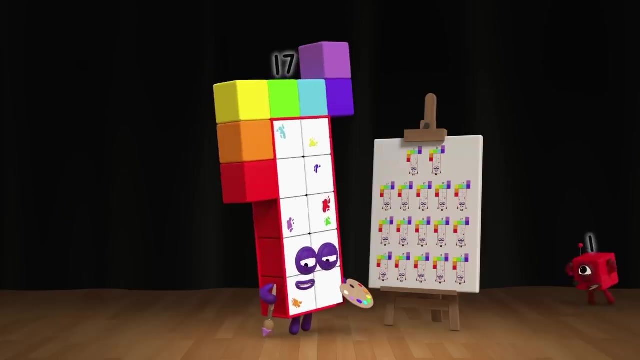 A square in the middle, Chapter 17,. portrait of the artist in his prime. How do 17 here? Today I'm going to show you how to paint a self portrait. Here goes Deary me. That's 17 self-portraits. 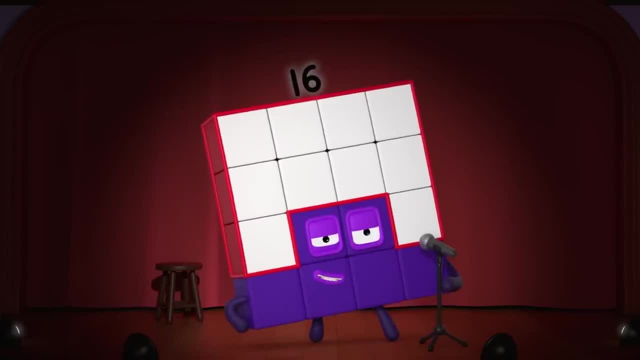 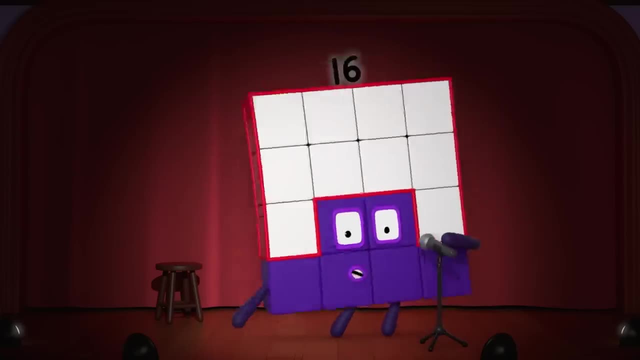 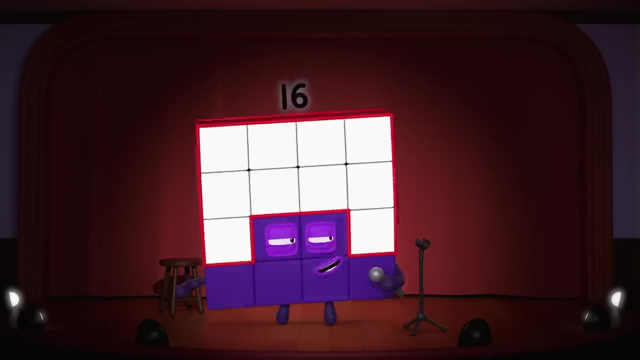 Let's get this party started. It's nice to be here And here And here And here. Look at that, I'm square turning round. Hey, you know what nine's favorite story is? Goldilocks and the Three Squares. 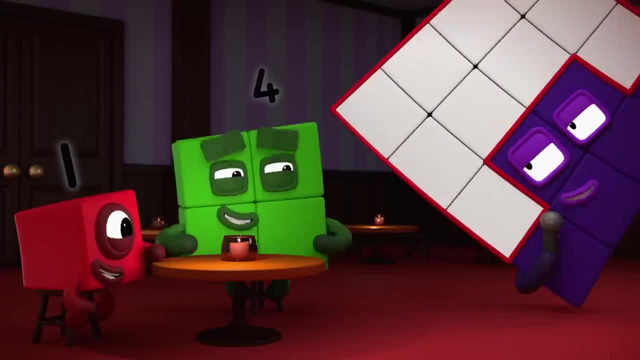 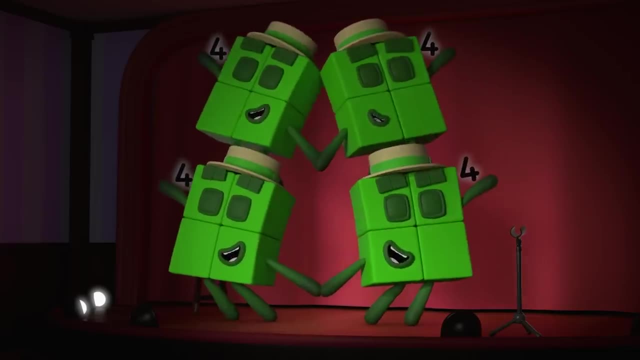 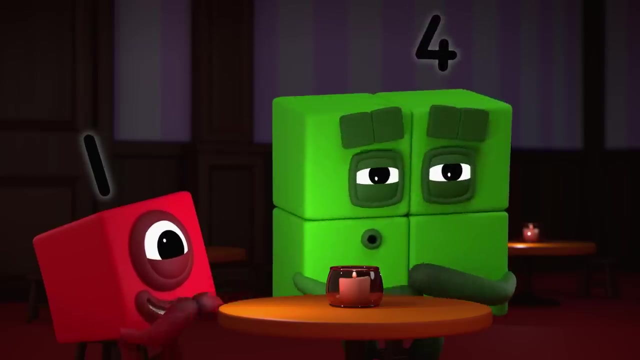 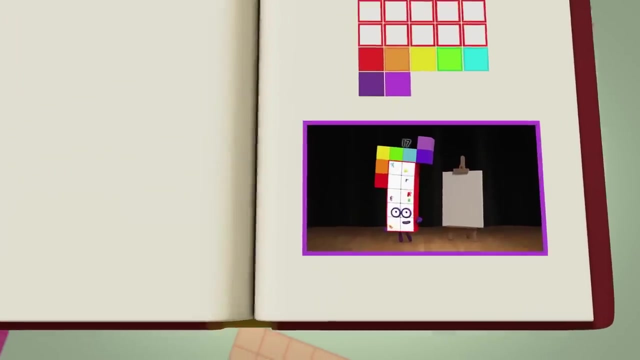 Squares, And if you're after a square deal, here I am. I'm a square Made of squares, With a A square in the middle. Chapter 17, Portrait of the Artist in His Prime. How do, How do I paint a self-portrait? 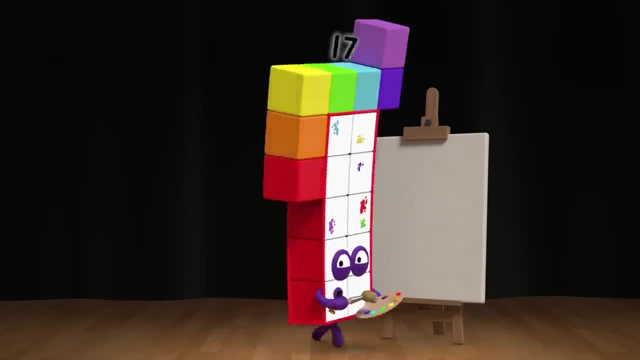 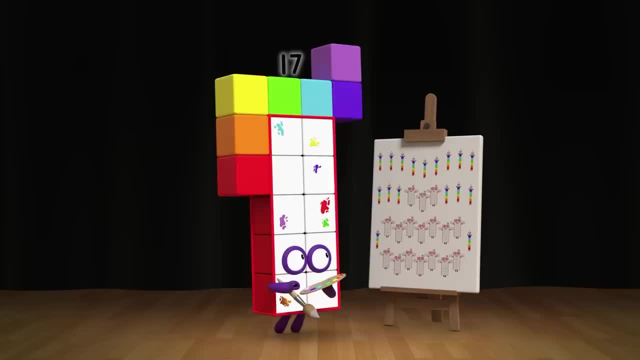 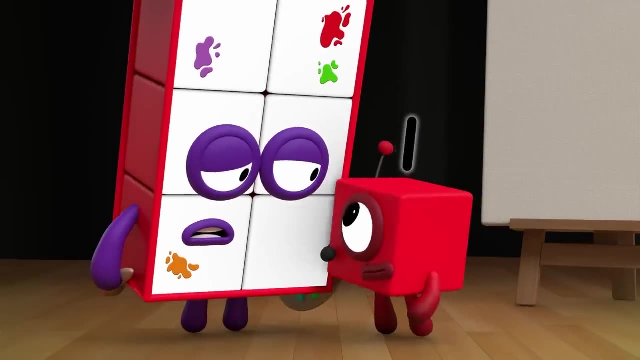 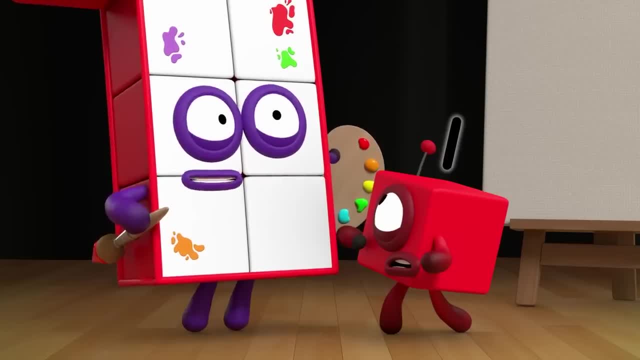 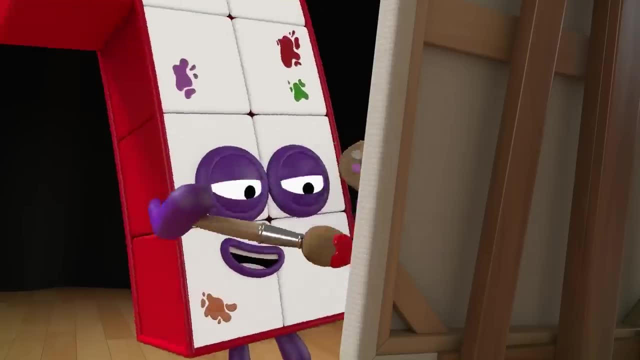 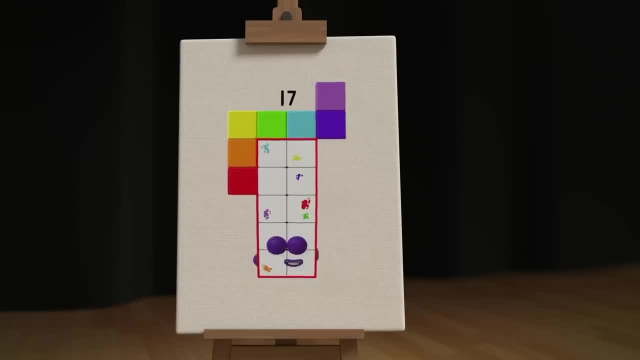 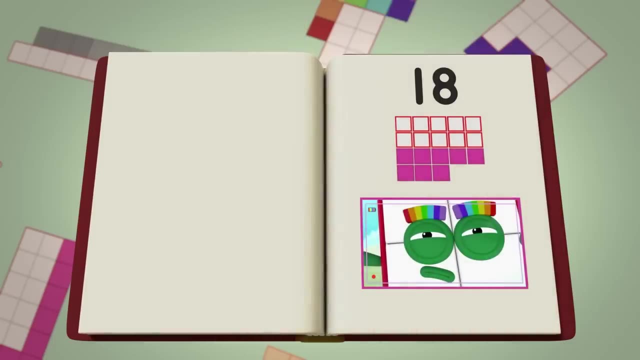 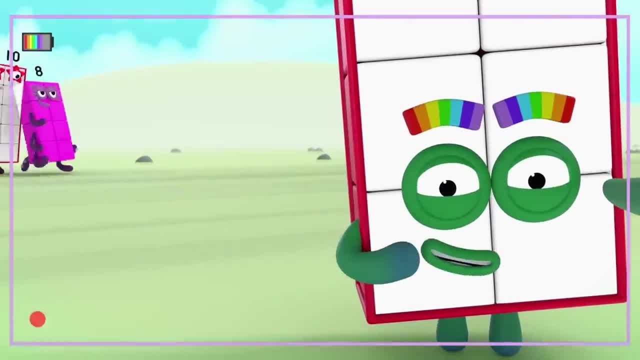 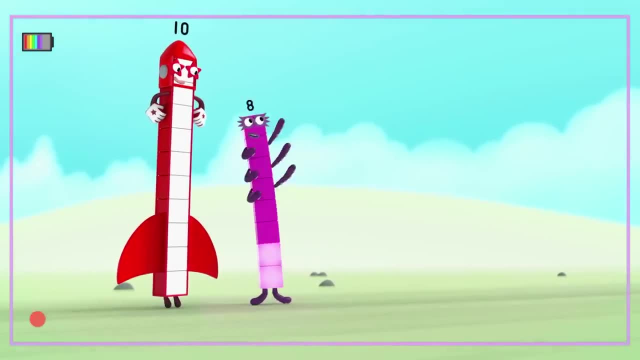 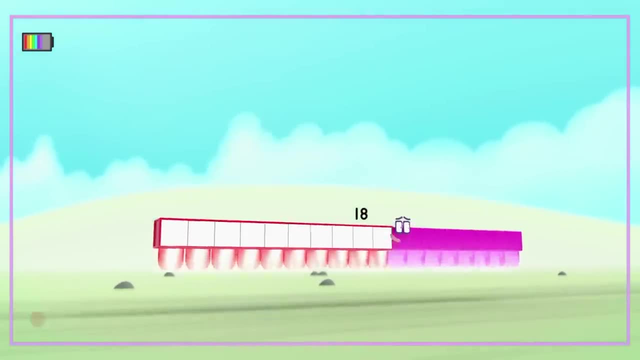 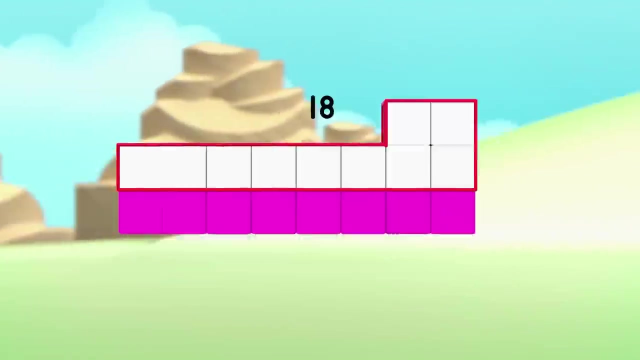 Super speedy, don't be late. Then somebody say speed 18, speed machine- One ray and away. Whoa Wanna see me go faster? Two rays and away, Three rays and away, Six rays and away, Nine rays and away. 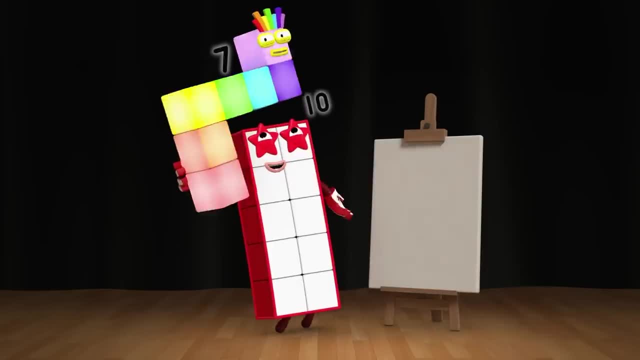 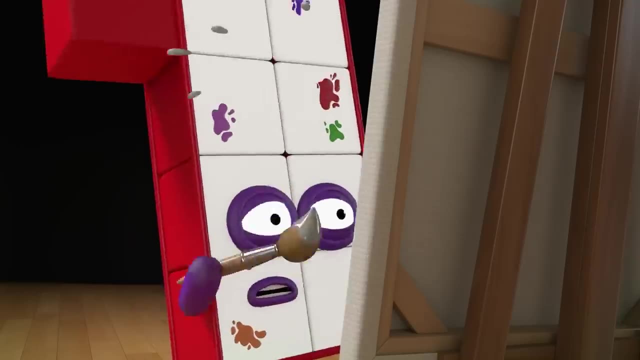 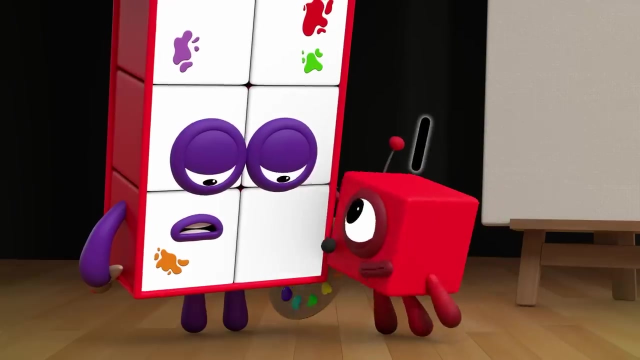 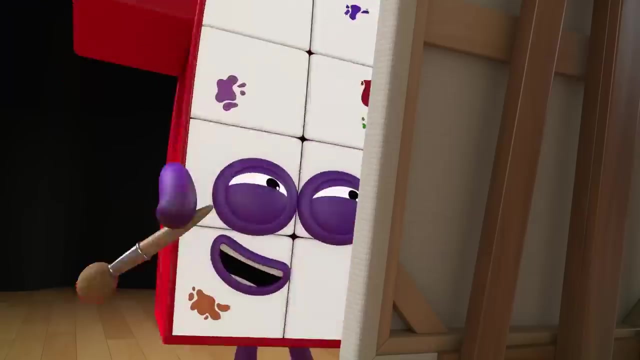 Let's try again. I'm ten and seven. So if I paint ten and then seven, Oh, 17 of each, Oh, I'm never going to get this right. Take some deep breaths. One, That's it. one. Stay there And there and there and there. 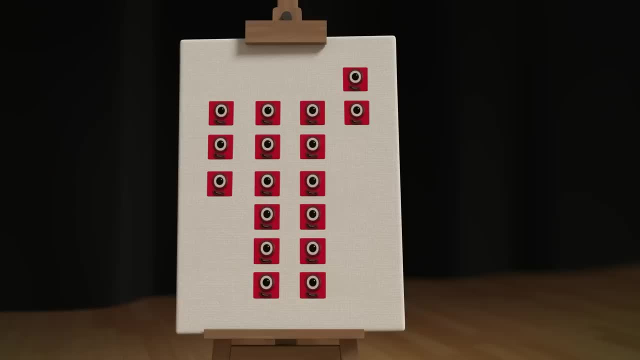 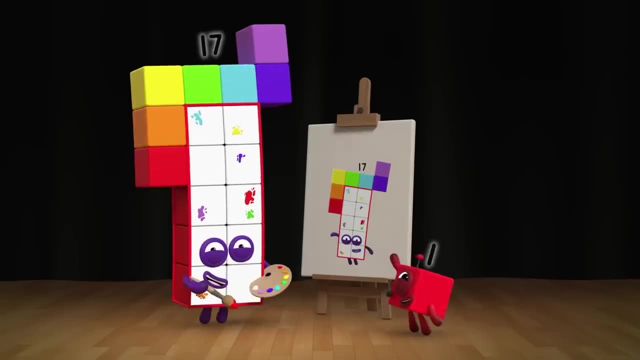 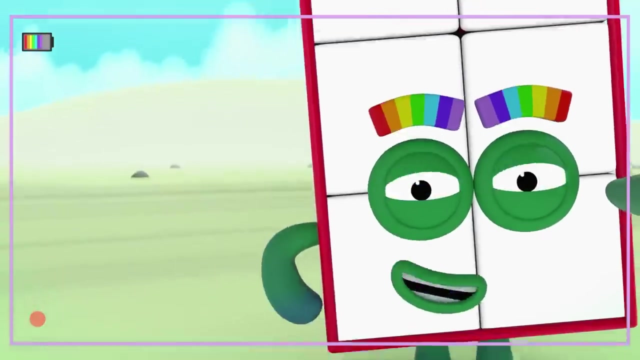 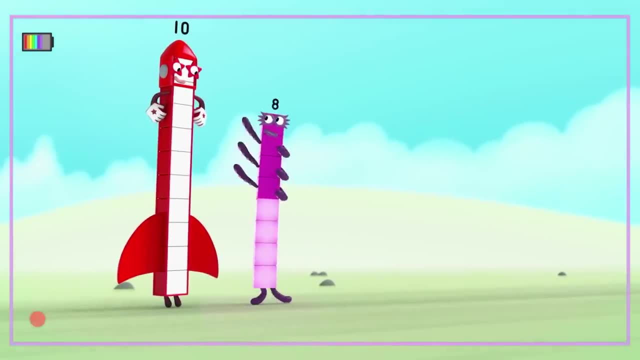 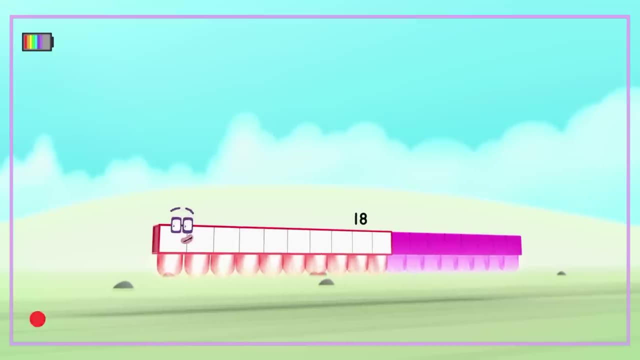 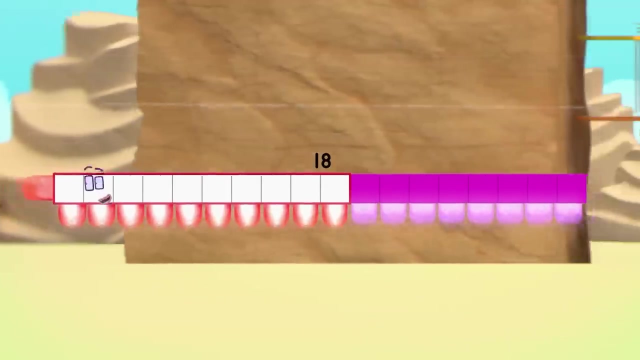 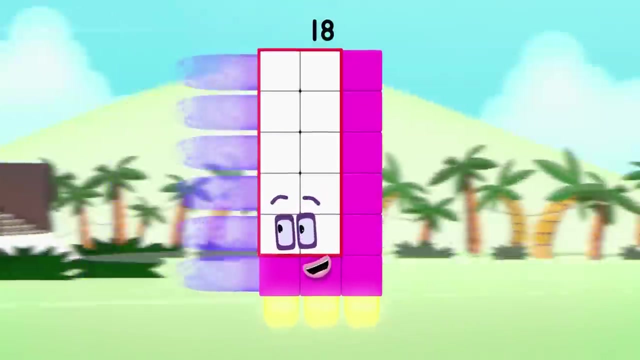 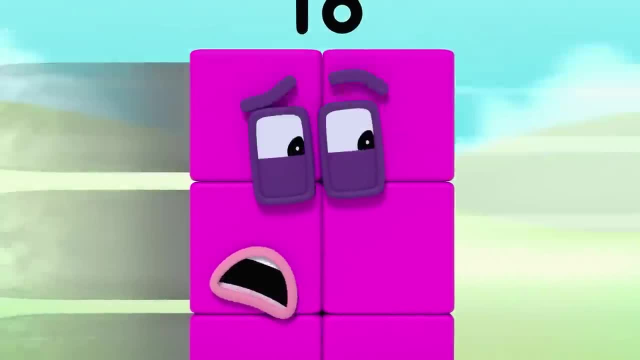 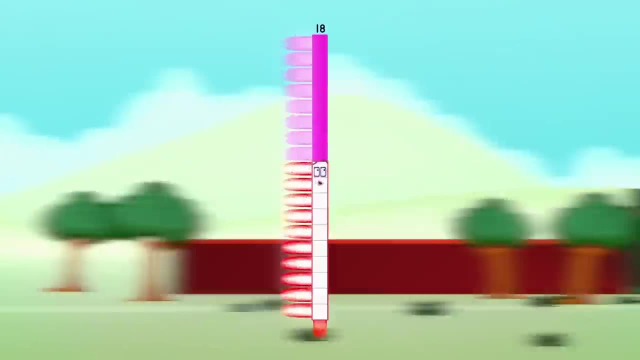 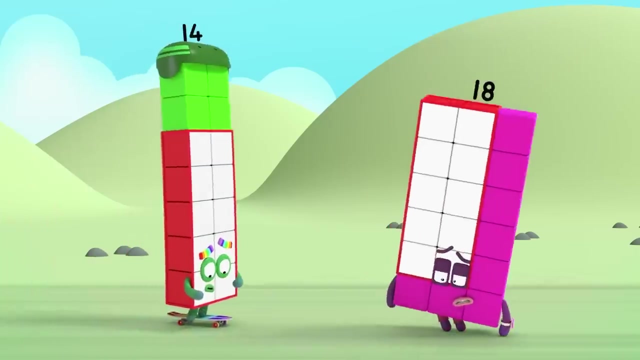 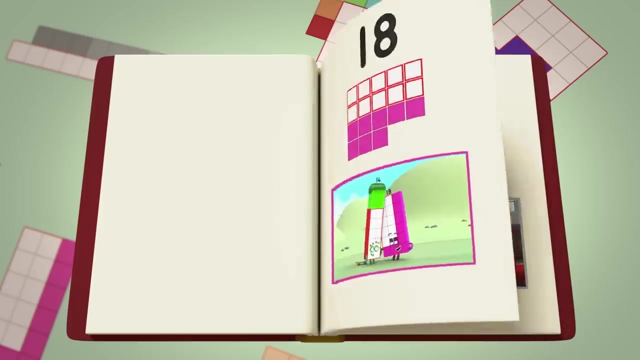 Nine rays and away. Super Sonic 18,, 18. Good call, compadre, 18 rays. Go dude, Look out Tunnel. Uh-oh, Now that was a speedy escape. Phew, Chapter 19.. Flex-ability. 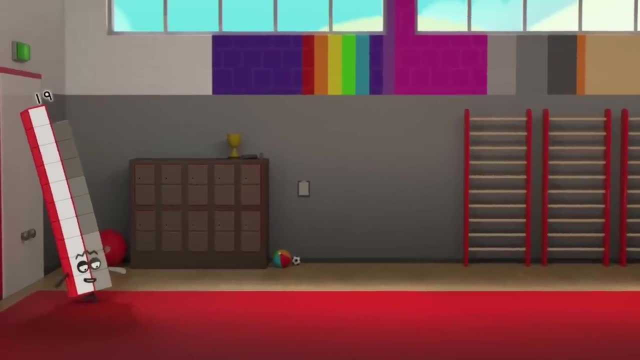 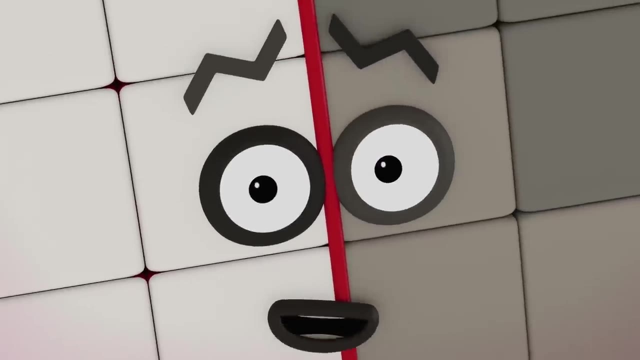 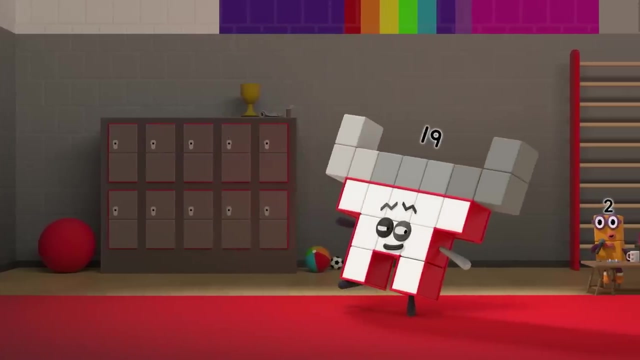 I'm 19.. When I try to make a rectangle, I'm always one block off. Oh, but who needs rectangles when you can make shapes? I can make shapes like these. Ah Whoop, So many shapes, So versatile. 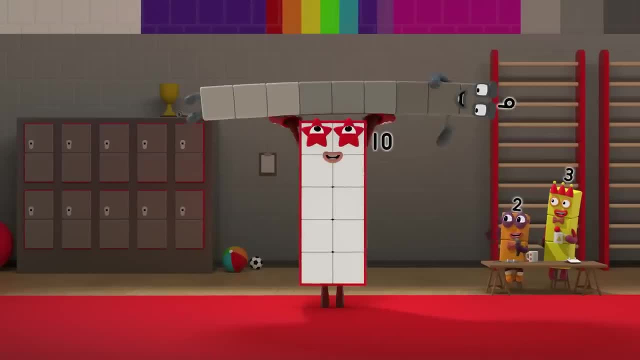 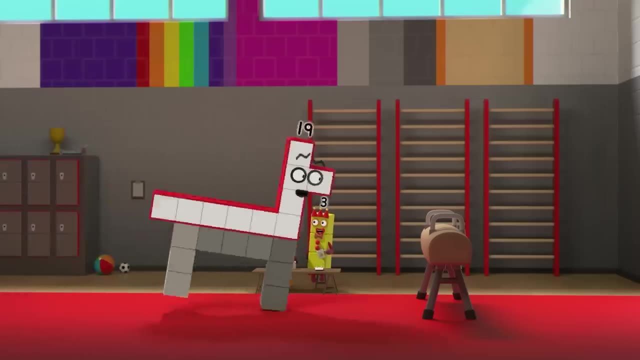 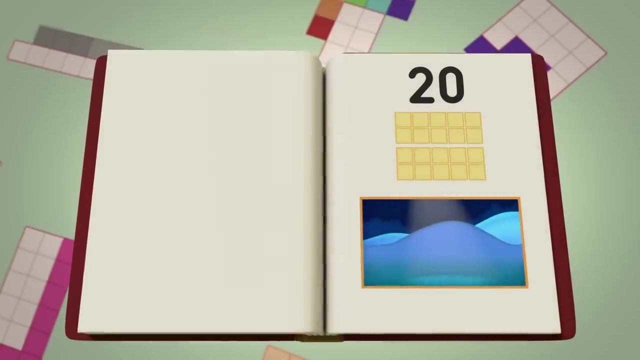 The plant pot, the helicopter, Lovely Letting us see the ten and the nine there, Magnificent Finishing with the horse. I'm a one-off Whoop. I go my own way. Chapter 20. Making friends. 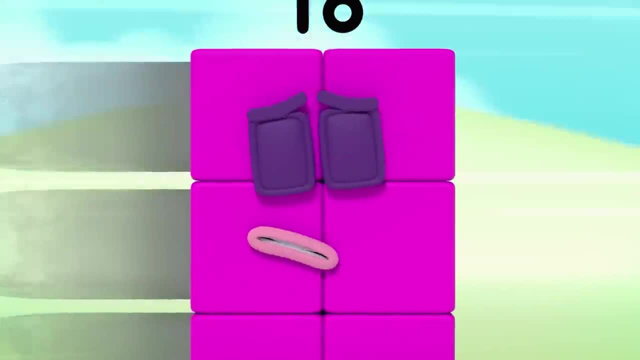 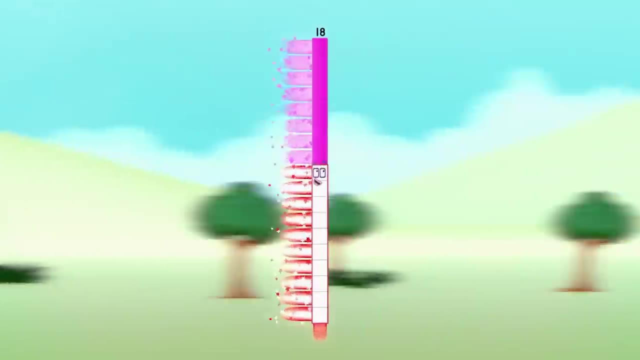 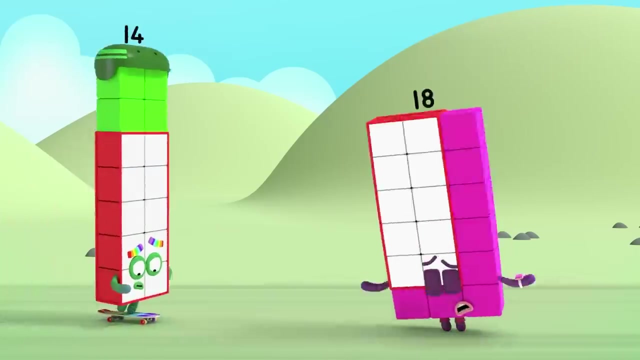 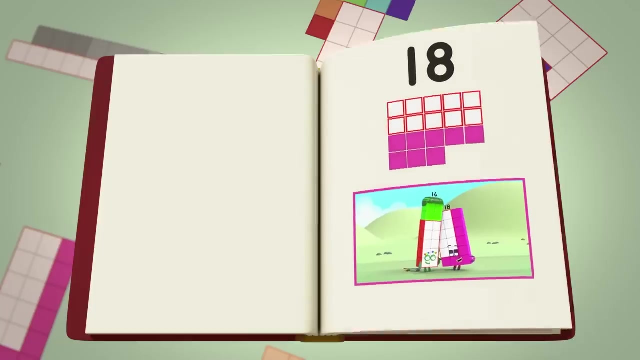 Nine rays and away. Supersonic 18,, 18!, Good call, compadre. 18 rays and away. Go dude, look out Tunnel. Uh-oh, Now that was a speedy escape, Chapter 19.. 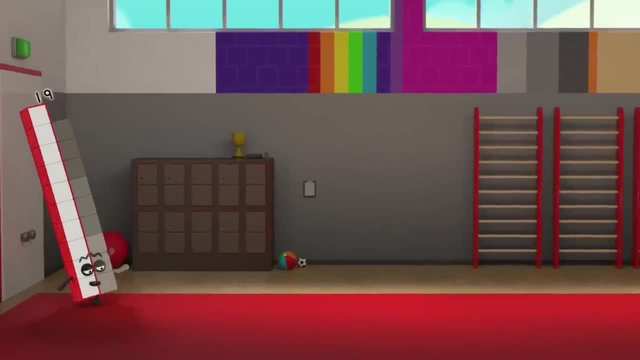 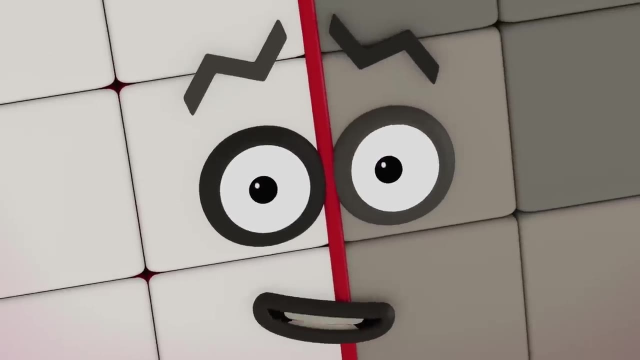 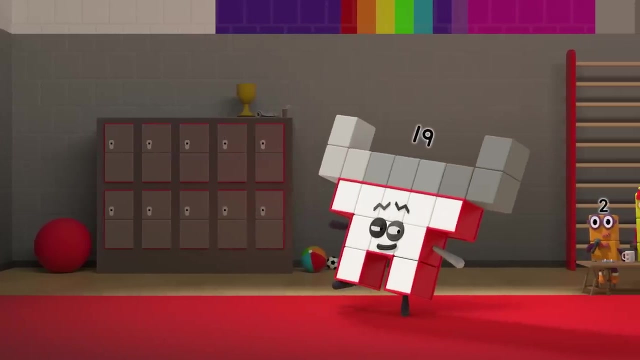 Flexibility. I'm 19.. When I try to make a rectangle, I'm always one block off. Oh, but who needs rectangles when you can make shapes like these? Ah, So many shapes, So versatile: The plant pot, the helicopter, lovely. 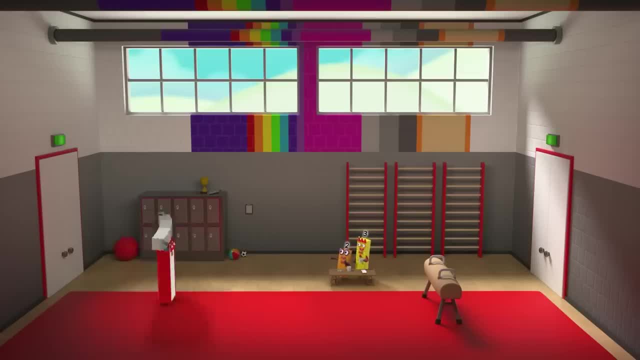 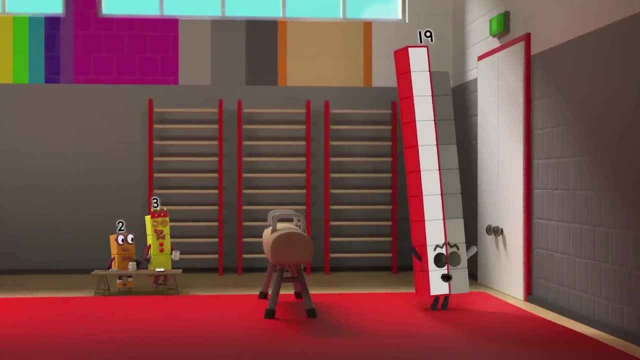 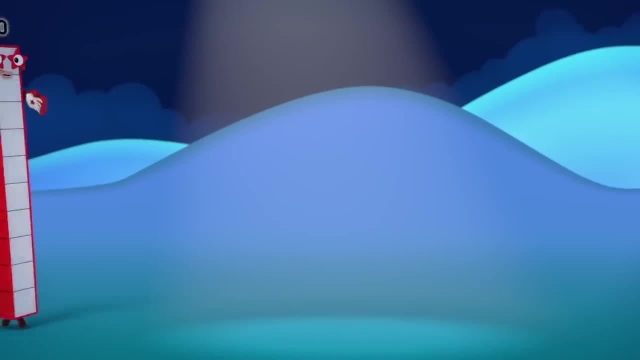 Letting us see the 10 and the 9 there. Magnificent, Finishing with the horse. I'm a one-off. I go my own way, Chapter 20. Making friends. Hello, I'm 10.. I'm another 10.. 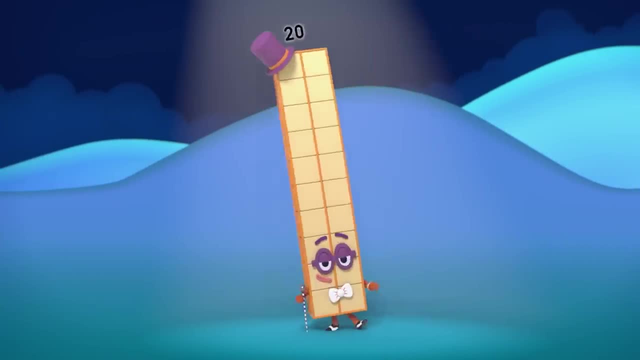 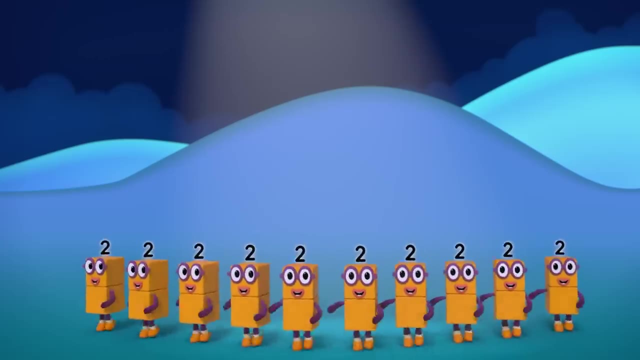 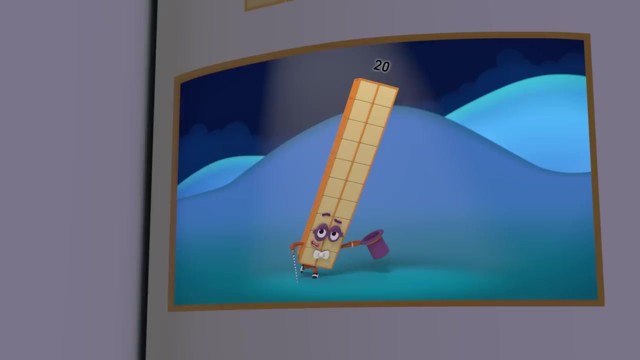 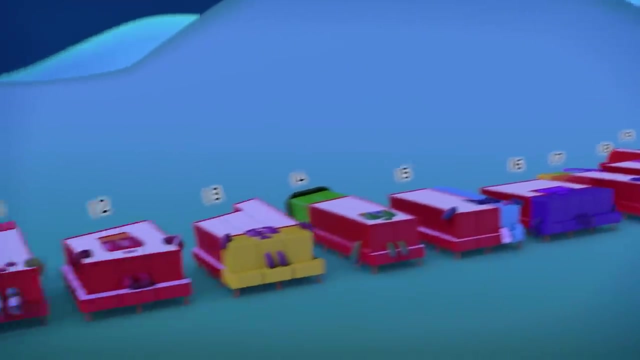 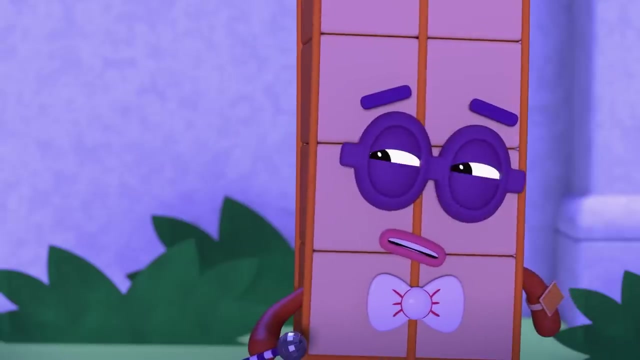 Let's be friends. I'm 20. And I'm good at making friends. I'm a 10-pack of twos. Thank you, Numberland. And sweet dreams, Sweet dreams all of you. Oh, Hello, friends. 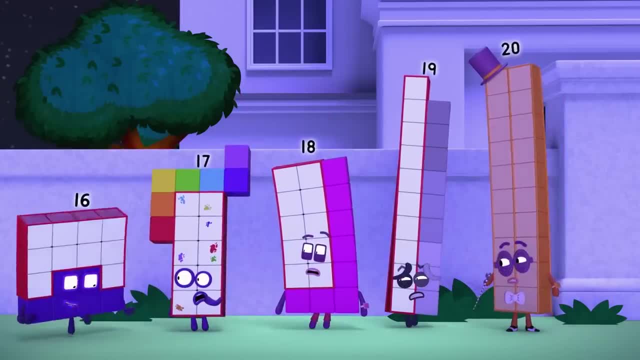 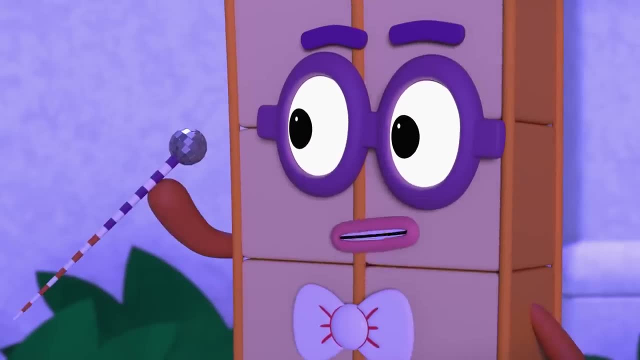 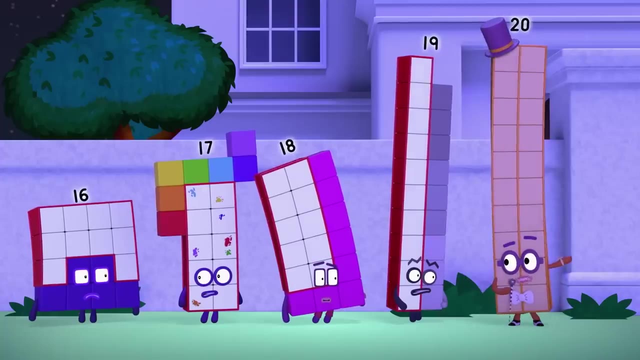 Glad you could make it The Museum of Numbers. I love this place. The museum's closed. There are robot guards everywhere. grab what we came for and get out, or a certain someone's not going to be happy. now we need to get through this big square, gate 16- you're up. 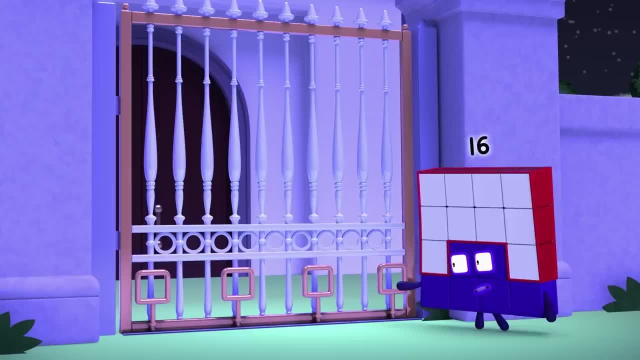 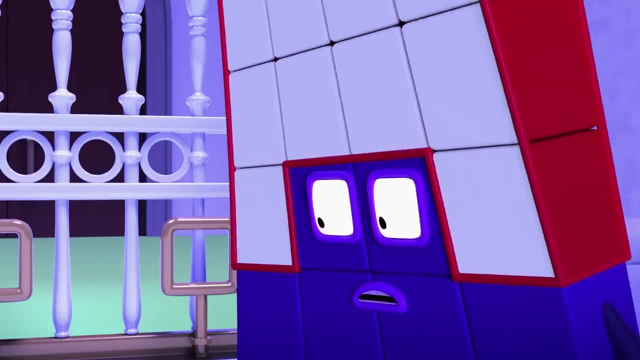 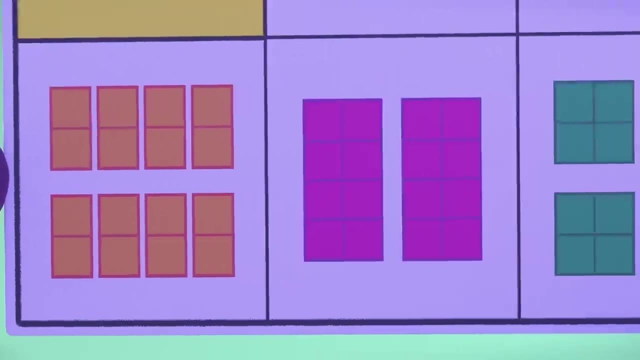 there is a problem, boss. there are four bolts. i can't lift them all at the same time. don't panic, it's time for a backup plan. use your skill sheet. four heavy bolts: what would help? eight, twos? twos aren't strong enough. two, eights, not enough of them. 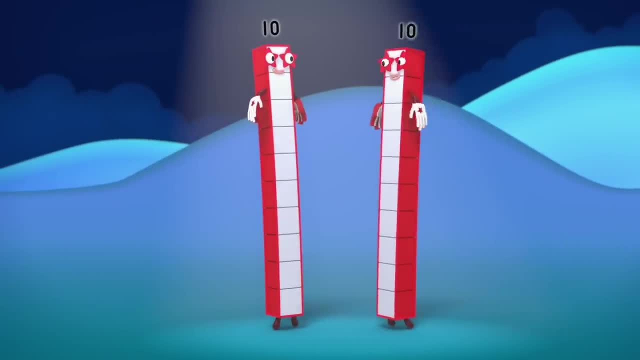 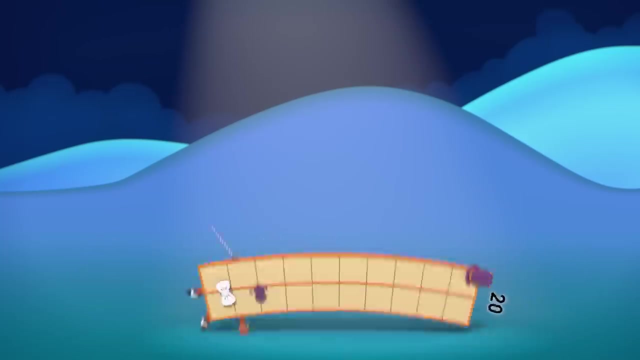 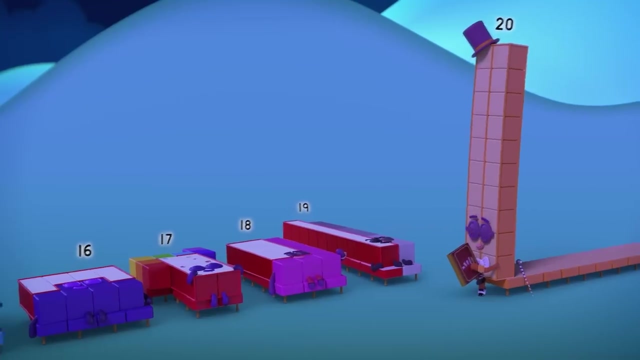 Hello, I'm ten. I'm another ten. Let's be friends. I'm 20, and I'm good at making friends. I'm a ten-pack of twos. Thank you, Numberland, And Good night, Sweet dreams, all of you. 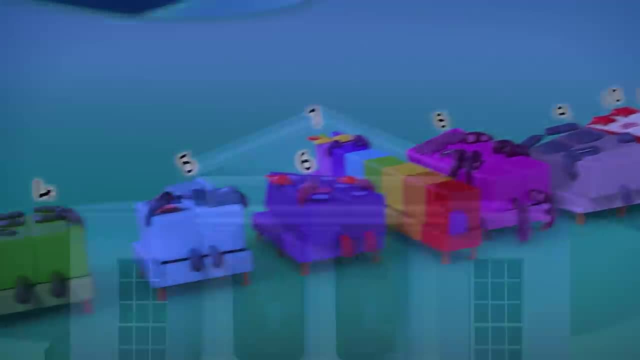 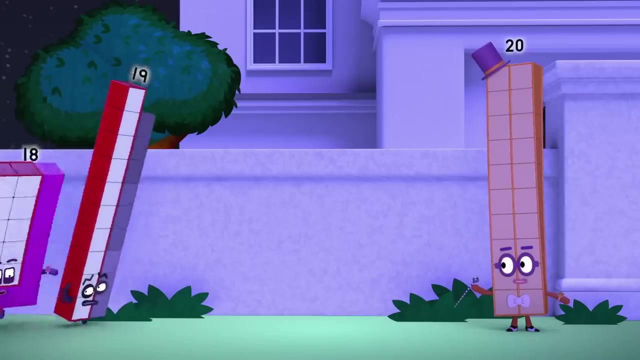 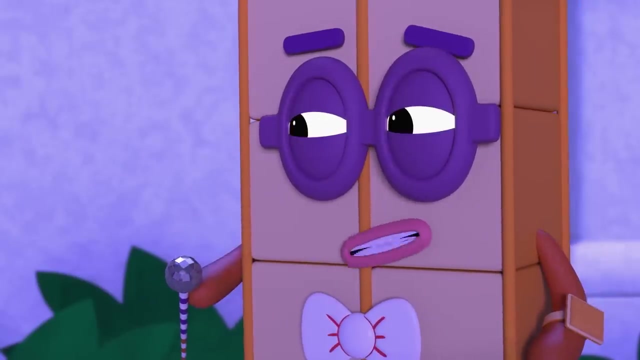 Brrr, Brrr. Hello friends, Glad you could make it The Museum of Numbers. I love this place. Shhh, The museum's closed. There are robot guards everywhere. We need to get in, grab what we came for and get out. 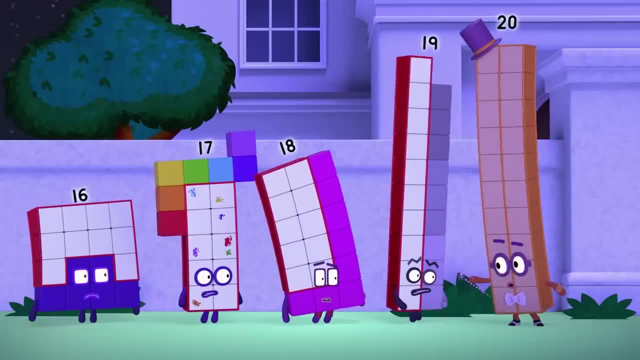 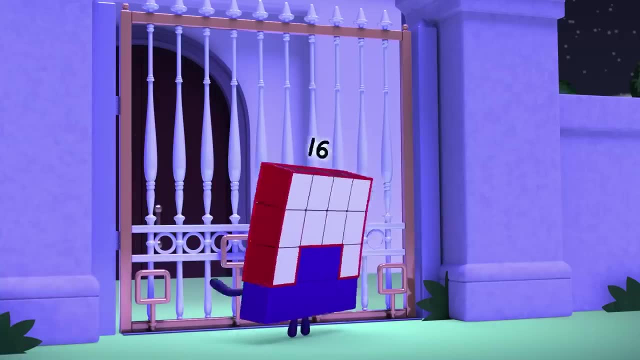 Or a certain someone's not going to be happy. Now we need to get through this big square gate Sixteen, you're up. There is a problem, boss. There are four bolts. I can't lift them all at the same time. 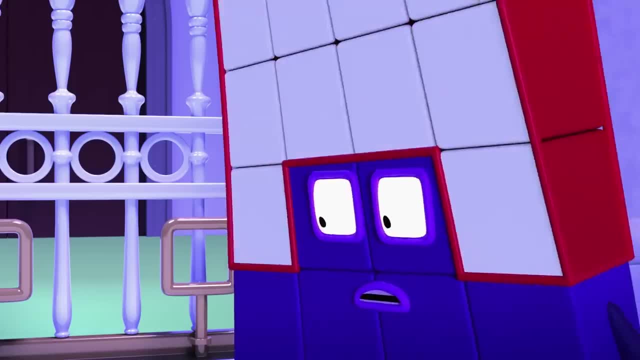 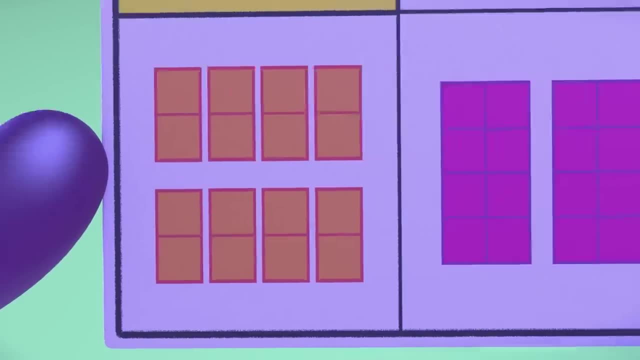 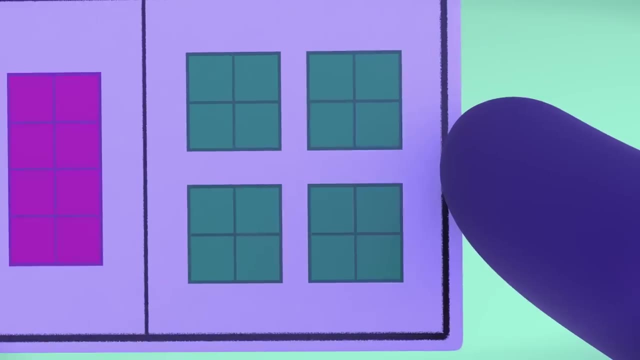 Don't panic. It's time for a backup plan. Use your skill sheet. Four heavy bolts. What would help? Eight, twos, Twos aren't strong enough. Two, eights, Not enough of them. Aha, I can be four square fours. 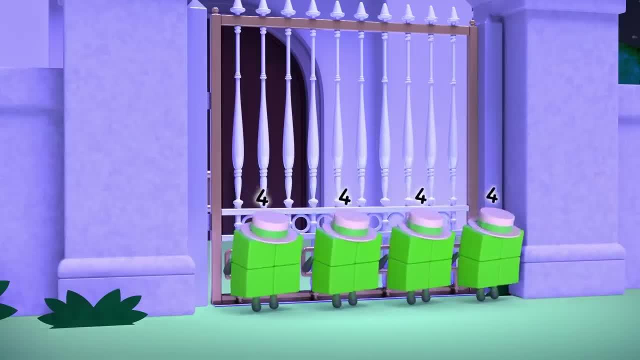 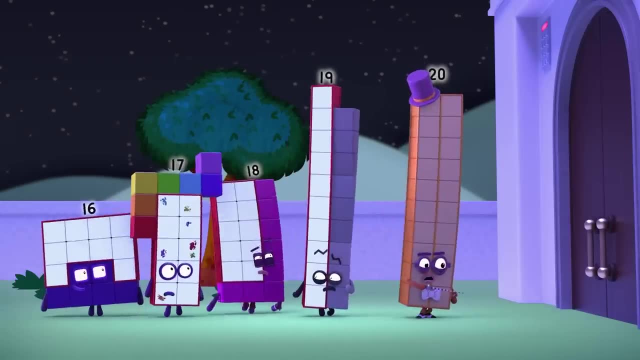 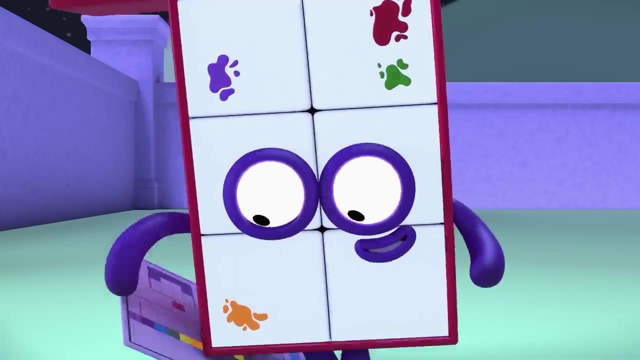 Squares are strong. Oop, Oop. The plan says there's a keypad for the main door Way up there, But we don't know the code. Hmm, How can we get up high? We could climb up a stepshape fifteen. 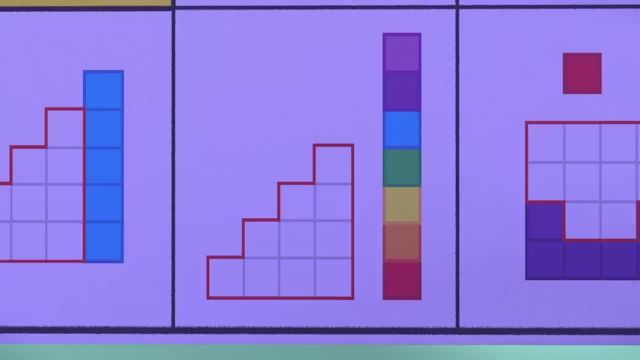 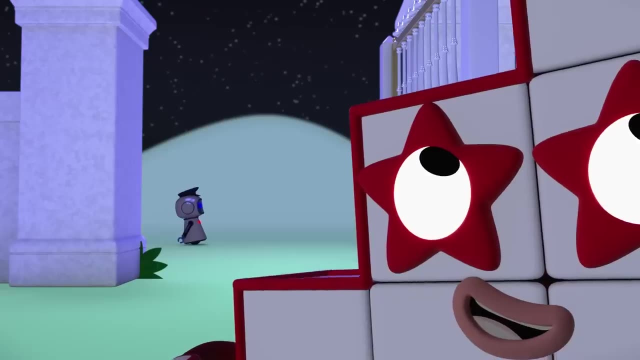 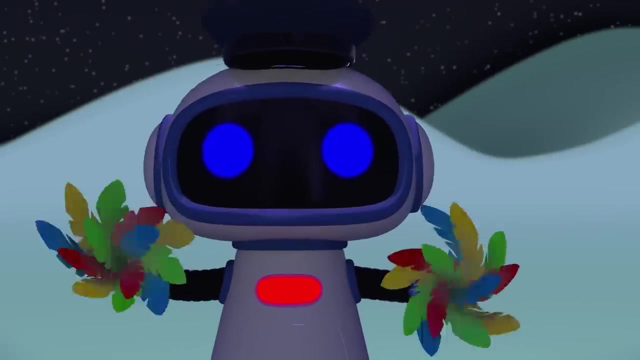 But we need a lucky guess to crack that code. Aha, Stepshape ten and lucky seven. Ooh, Ooh, Intruders, Intruders, Tickle, Tickle, Tickle, Tickle, Tickle, Tickle, Tickle. 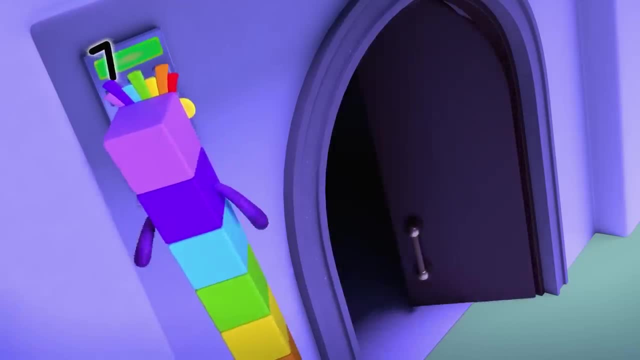 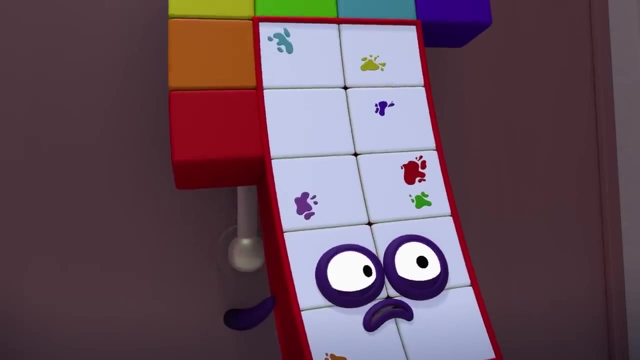 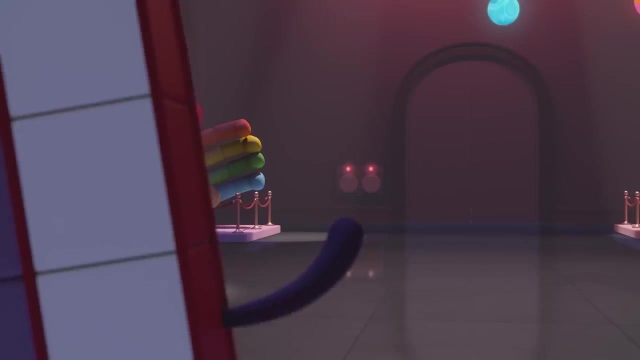 That was lucky. Intruders, Intruders. The floor past that line is alarmed. If anything touches it, we'll all get caught. Those buttons turn the alarms off. But how come Tickle, Tickle, Tickle? 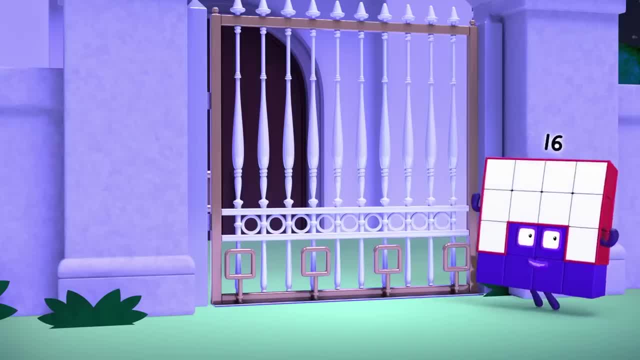 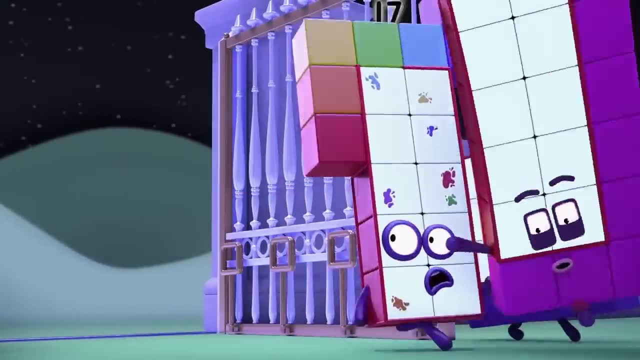 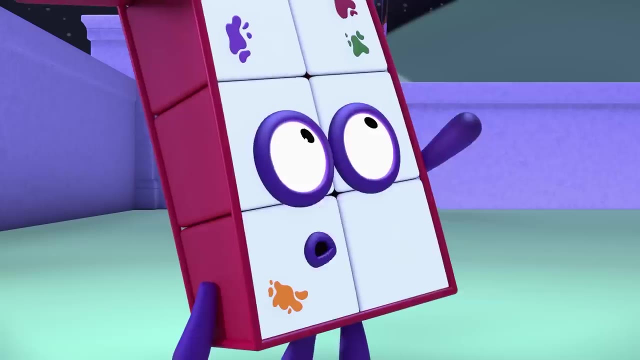 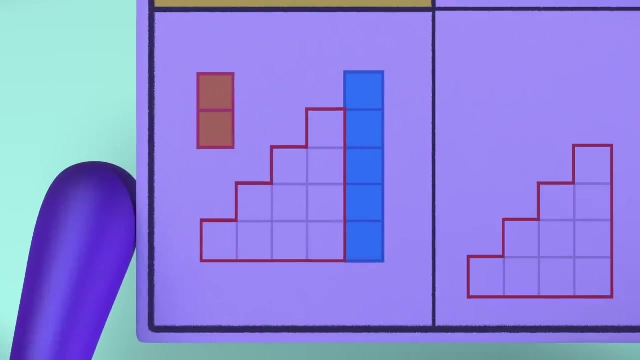 i can be four square. fours squares are strong. the plan says there's a keypad for the main door way up there, but we don't know the code. how can we get away? hi, we could climb up a step- shape 15- but we need a lucky guess to crack that code. 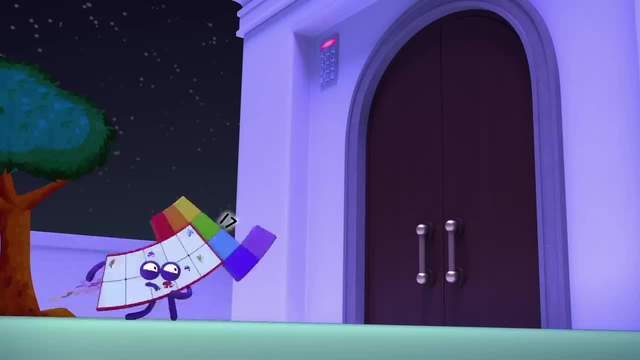 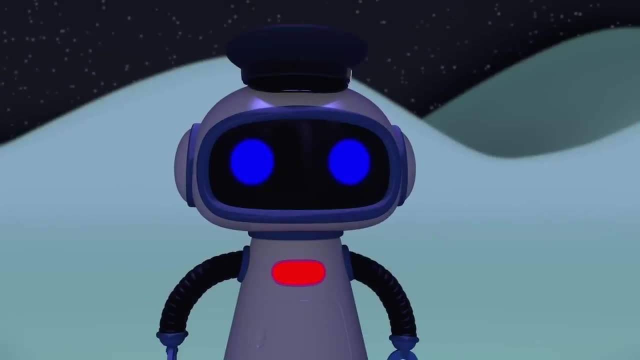 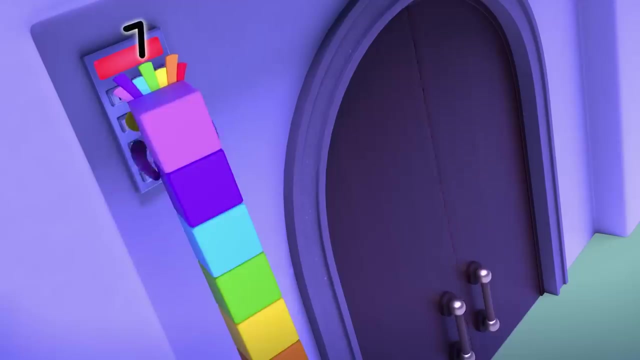 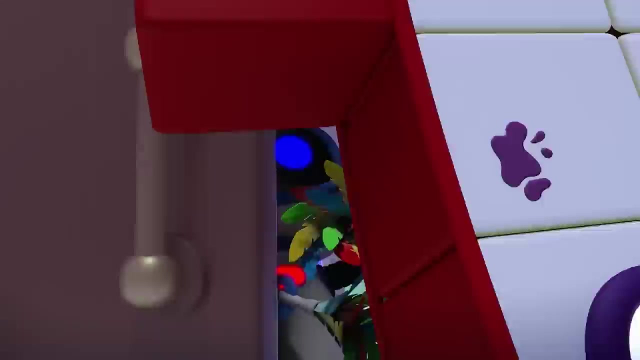 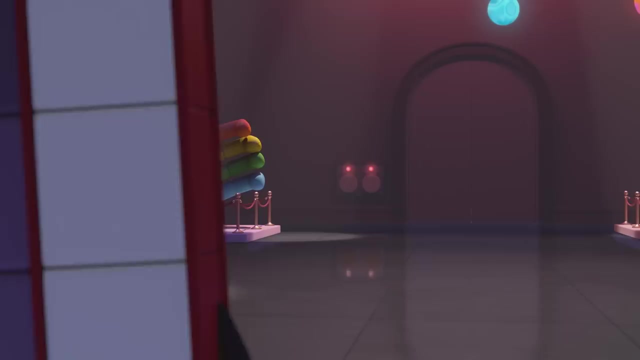 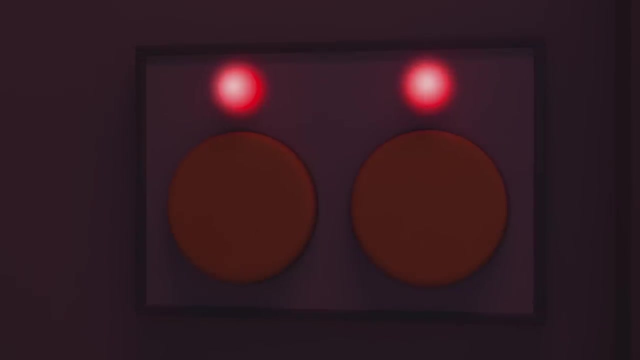 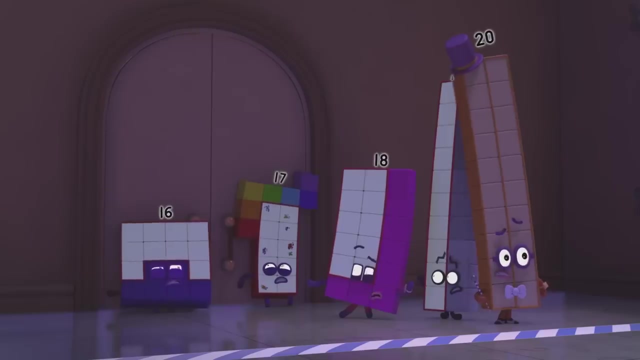 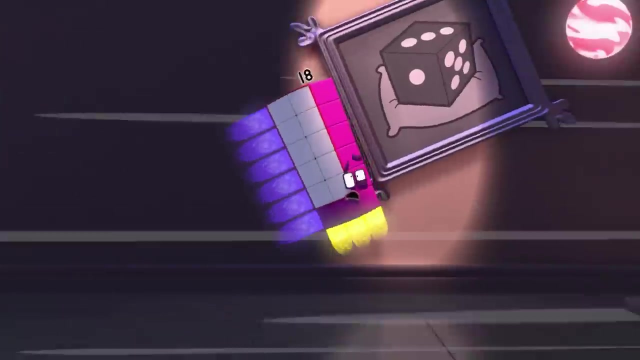 those buttons turn the alarms off, but how can we get to them? tickle, tickle, tickle, tickle. quickly, i can't hold the door much longer. and power, i don't believe this car's fast. the speed sticks raise and away. be careful, friends, Watch out for that. 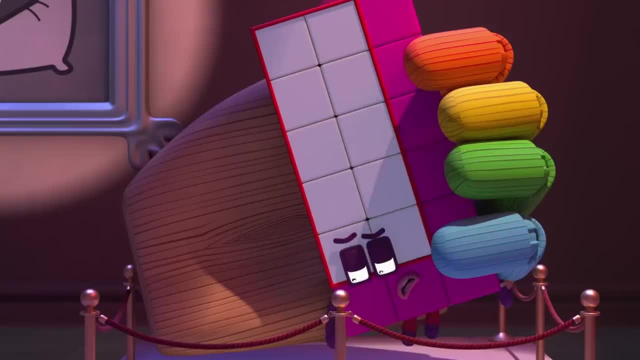 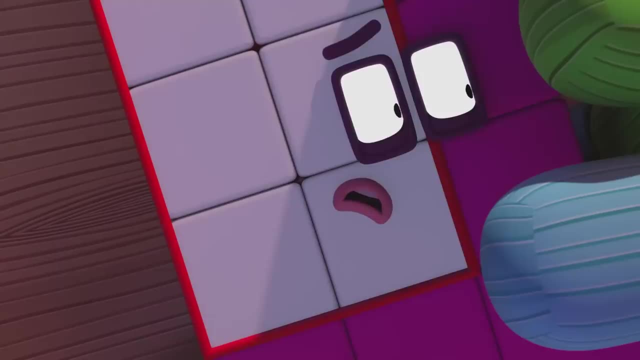 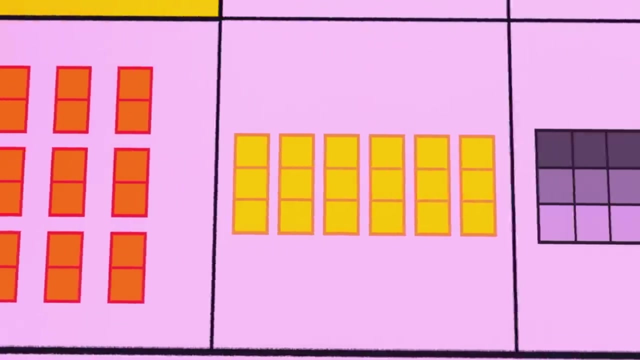 Inconvenient. I'm stuck: Tickle, tickle, Tickle, tickle, Do something. Hmm, how can I reach both those buttons while still stuck here? Nine, twos, No use. Six, threes, Please, Two, nines Ding. 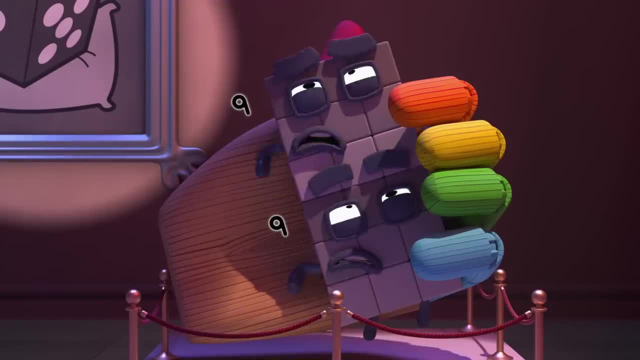 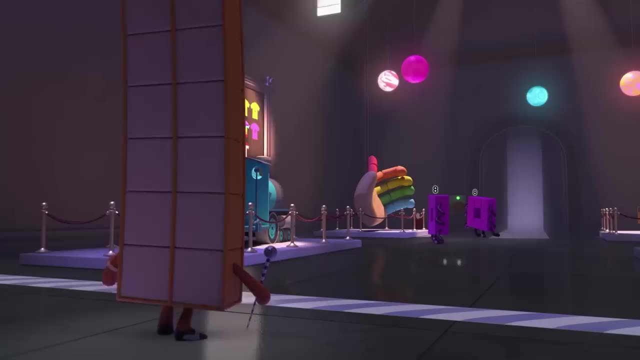 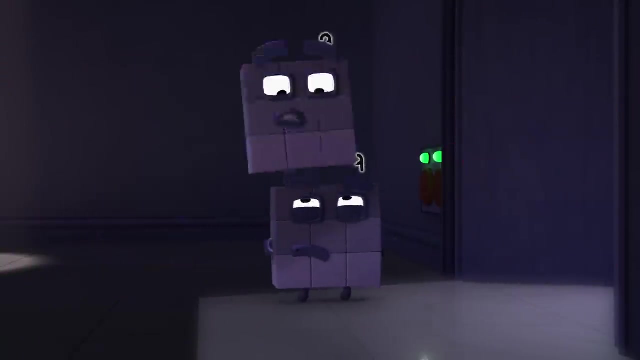 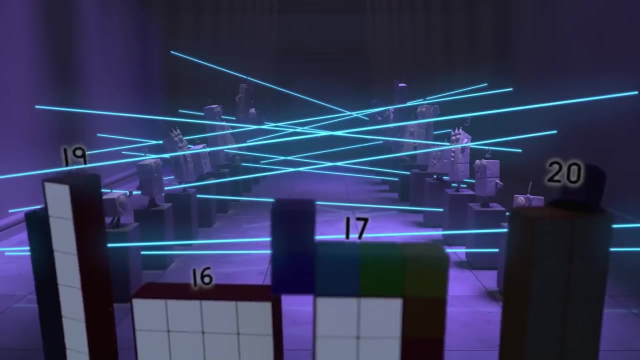 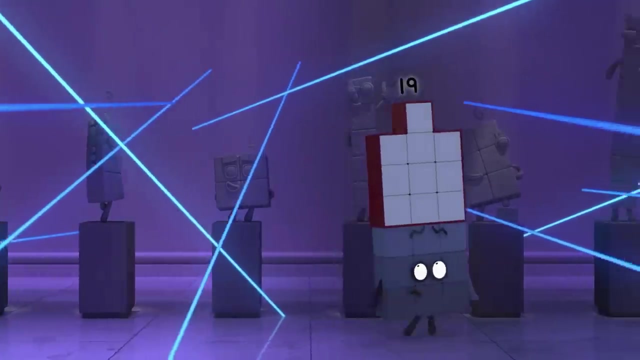 We have a winner. Er er, Alarm off. Follow me, friends Nearly there now. Tickle, tickle, Tickle, tickle. A laser maze- The perfect job for a one-off like me. Tickle, tickle, Tickle, tickle. 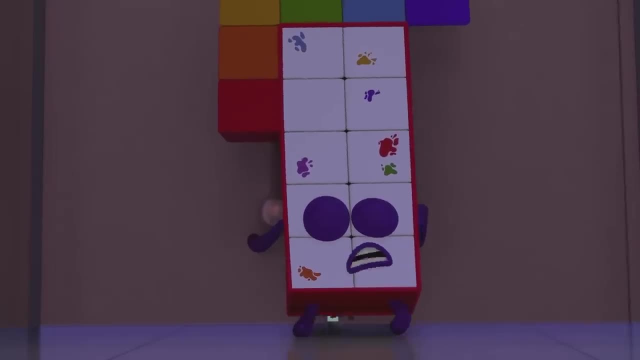 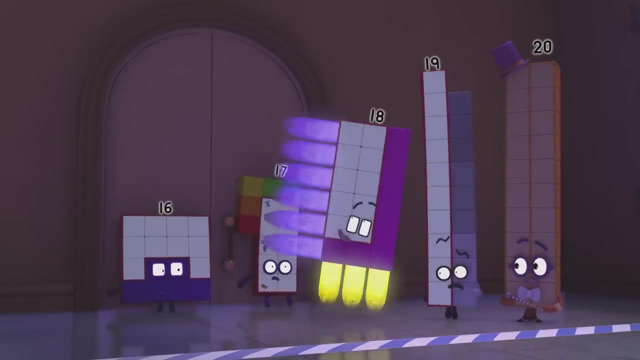 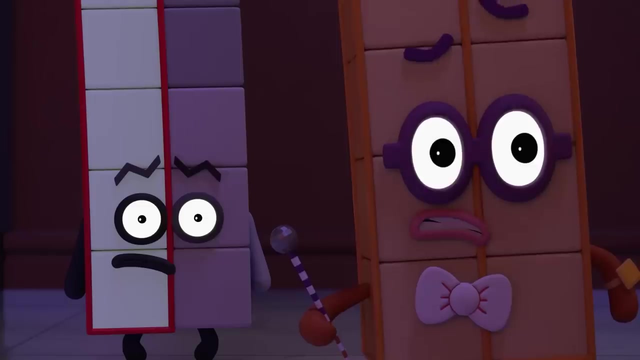 Quickly, I can't hold the door much longer. Spare power. I don't believe this calls for speed. Six rays and away. Careful friend, Watch out for That Inconvenient, I'm stuck. Tickle, Tickle, Tickle, Tickle. 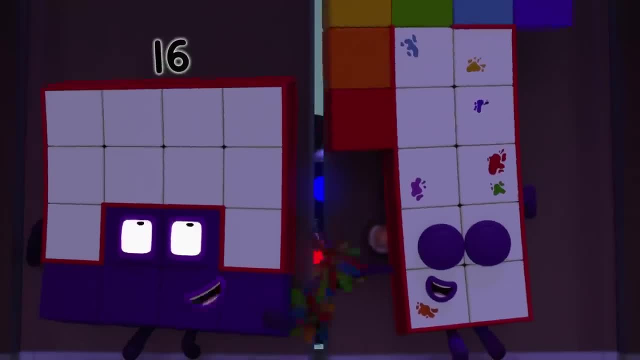 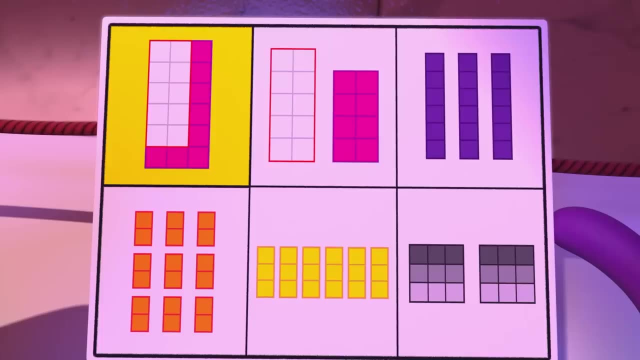 Do something: Tickle, Tickle, Tickle, Tickle, Tickle, Tickle, Tickle. Hmm, How can I reach Both those buttons while still stuck here? Nine, twos, No use. Six, threes, Please. 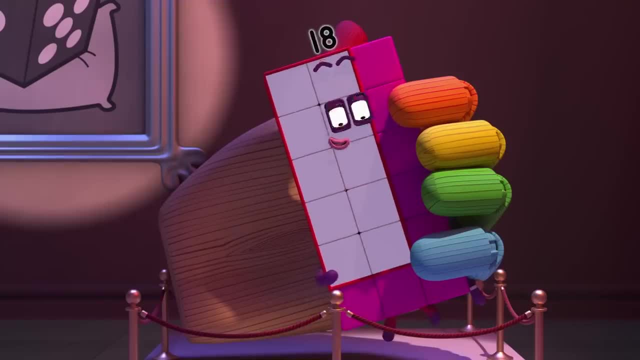 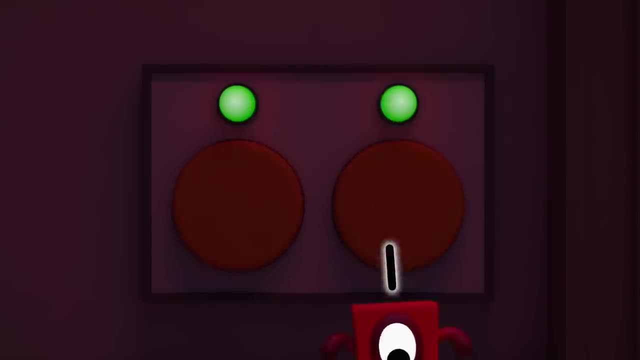 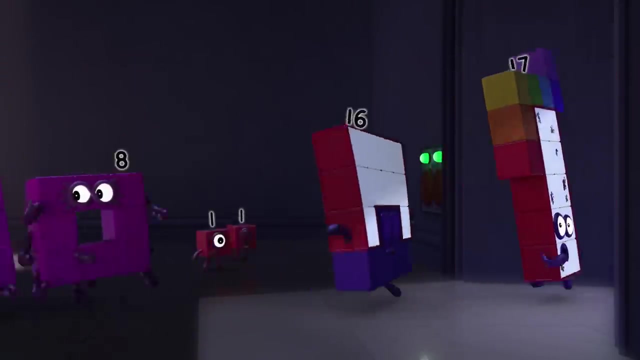 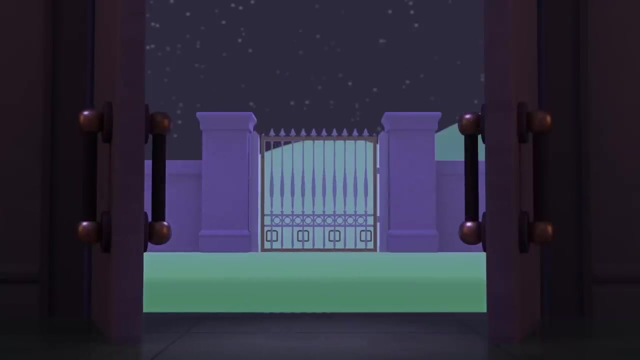 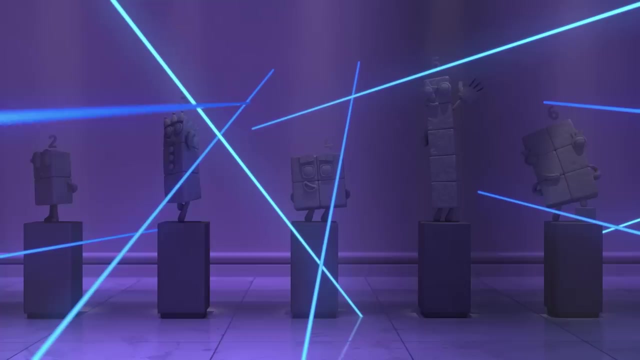 Two nines Ding, We have a winner. Alarm off. Follow me, friends Nearly there now. Ooh Oh, Tickle, tickle, Tickle, tickle. A laser maze- The perfect job for a one-off like me. 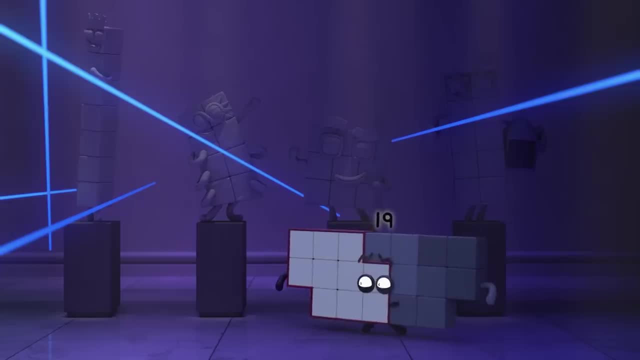 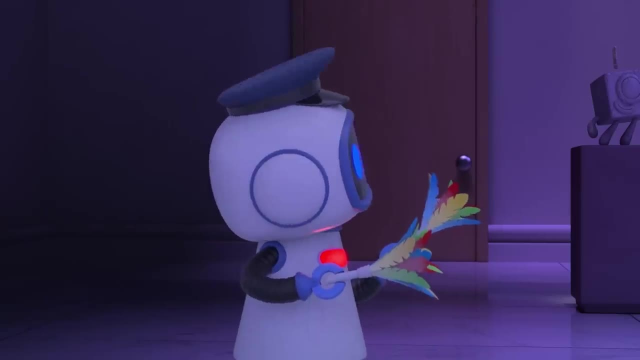 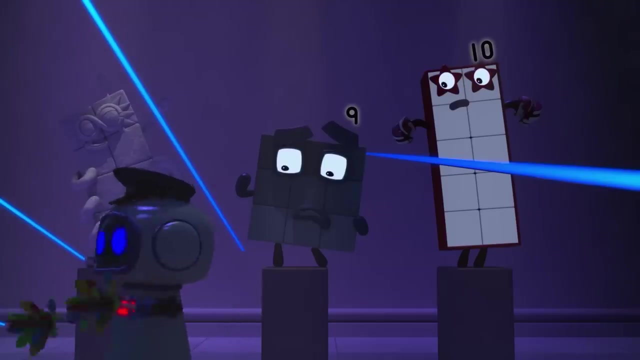 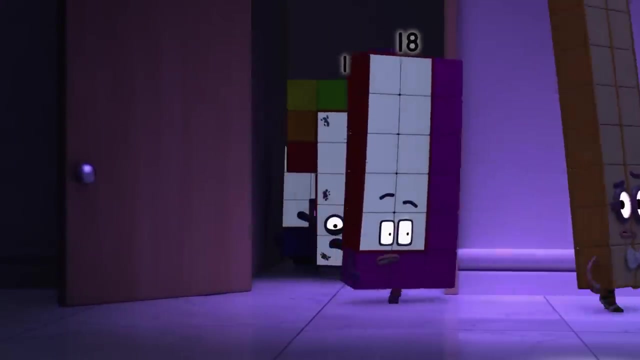 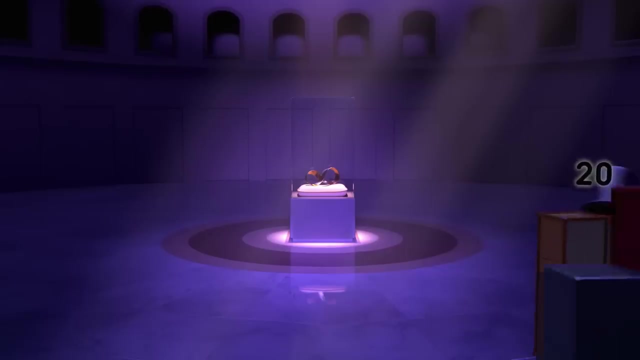 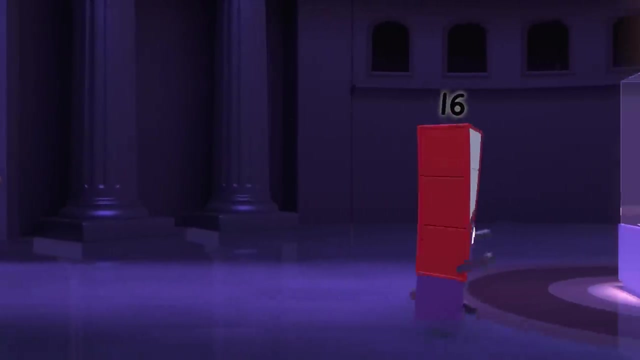 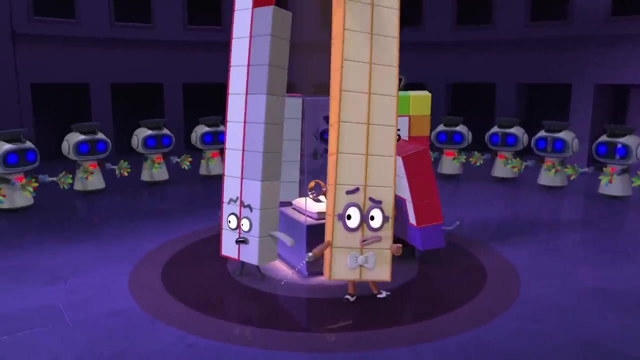 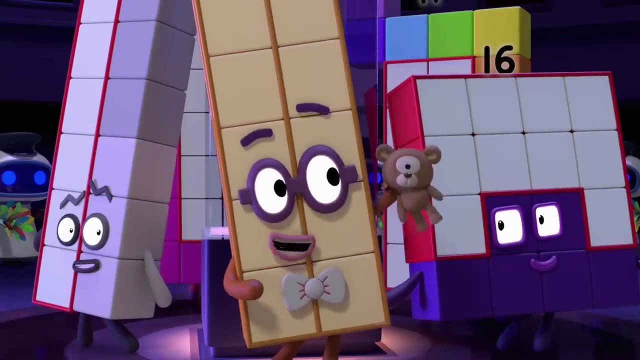 Tickle, tickle, Tickle, tickle The guard Hide. For once, I need to blend in, not stand out. Hmm, Oh There, it is the golden infinity Time to grab it. 16 wait, Wait. we're not stealing anything. We came for this one's teddy bear. 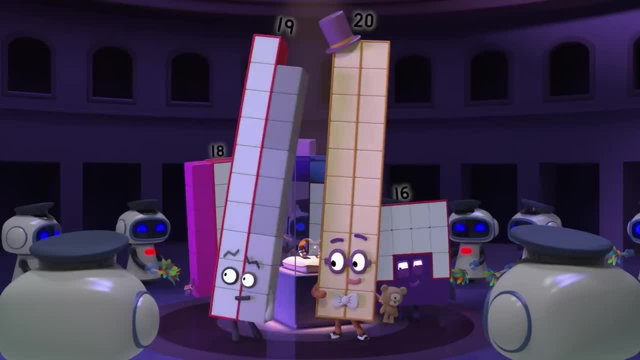 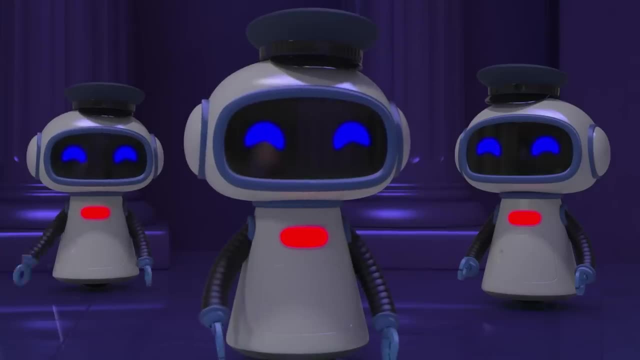 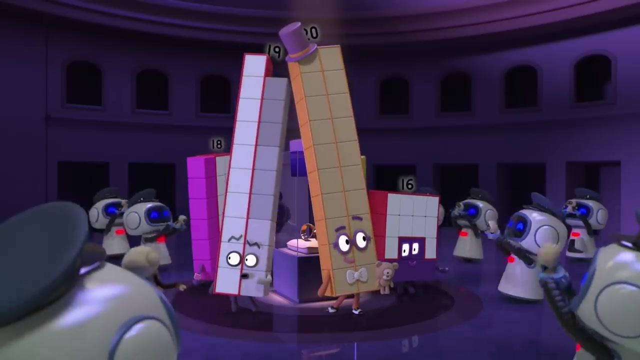 She left it behind at closing time. we did come back in the morning, but she can't sleep without it. We're very sorry. No need to apologize. We can't sleep without ours either, You.